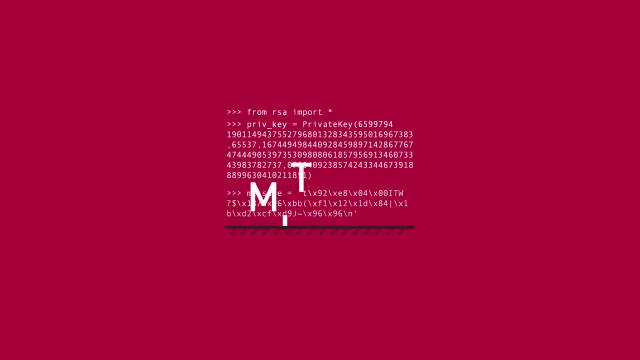 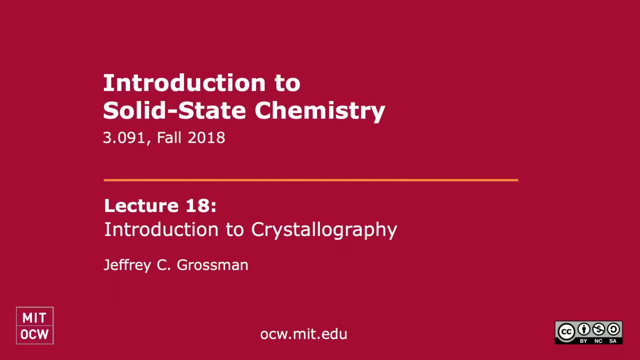 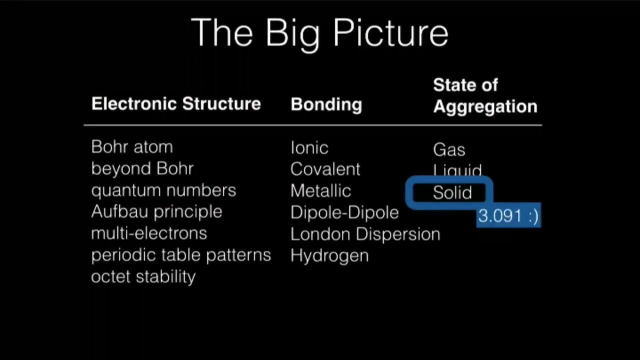 Big picture. I showed you this big picture before We're now going to add to it. Look at what we've done: Electronic structure all the way up through, you know, octet, stability, Lewis, molecular orbital theory, how to handle multi-electrons, all these different kinds. 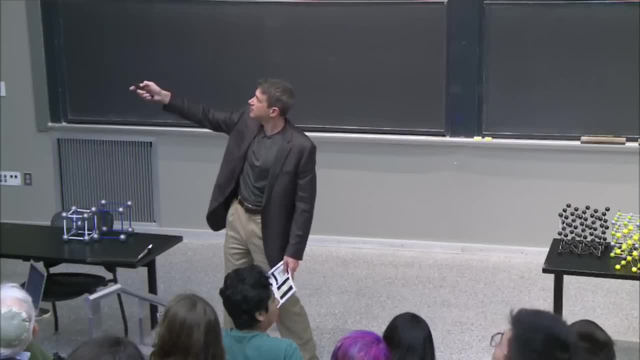 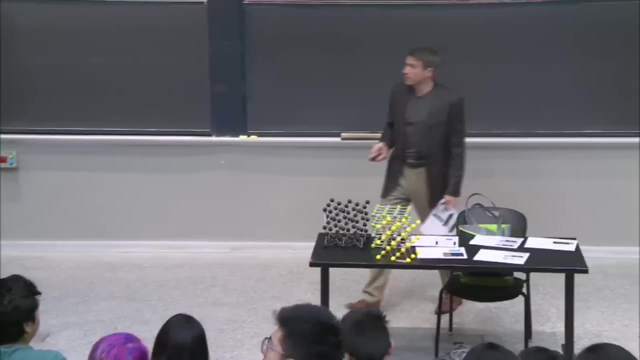 of bonding Check. We've covered every single one of these, And this is solid state chemistry. OK, but now here we are, right Now. OK, remember, we also talked about this in the very first lecture. When you classify solids, there are two things. 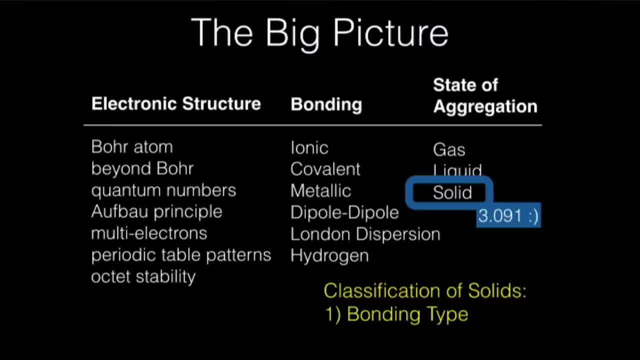 that are really important. One is the bonding type. How do the atoms in the solid want to talk to each other, How do they interact? And that is something that we have covered in a lot of different ways. But the next is how they come together. 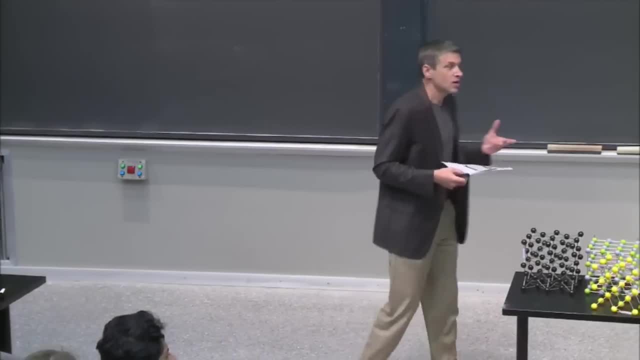 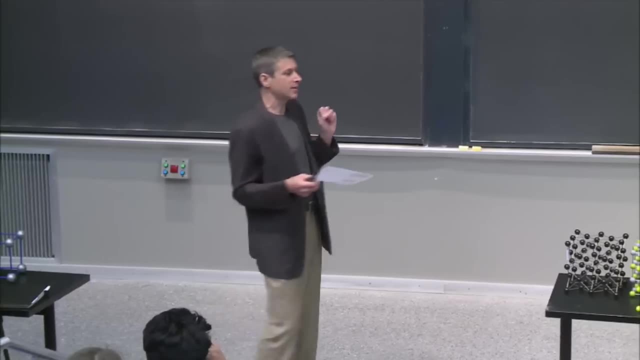 the actual arrangement of those atoms And that is what we're going to talk about today and on Wednesday, And then as we learn after Exam 2, as we learn about X-rays. that's a way to characterize the arrangement so that you can see how they're ordered. 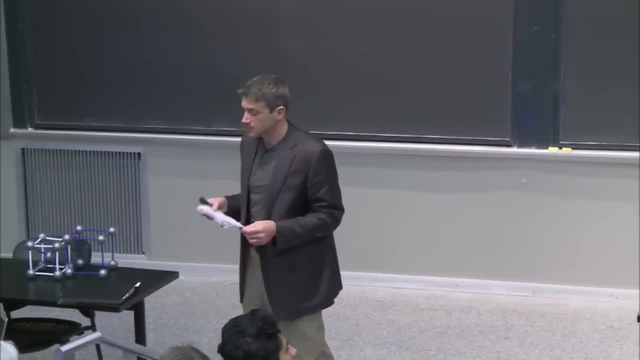 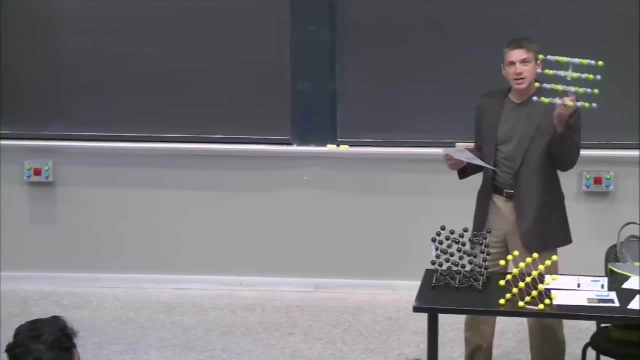 OK, we're going to use X-rays and do something called X-ray diffraction, But for this week. for this week, I want to just classify. I want to talk about the things, the tools that we use to understand how a solid forms. 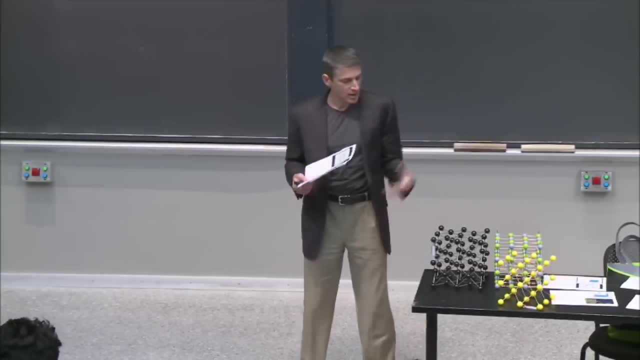 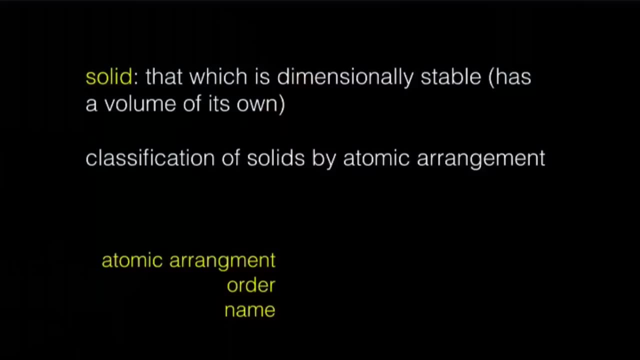 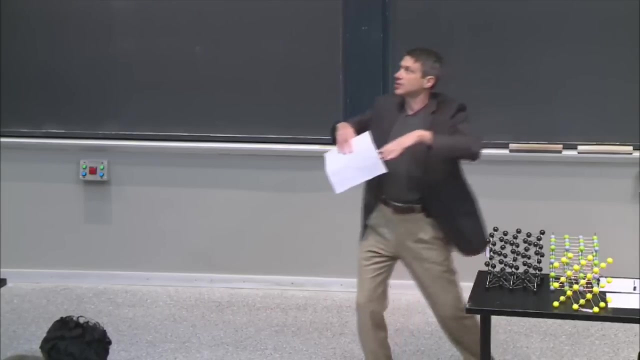 how to describe the formation of a solid, how the atoms can be described. So, of course, a solid is that which is dimensionally stable. Simple definition, right. But we can break down how these atoms arrange into two basic categories: the atomic arrangement, the order. 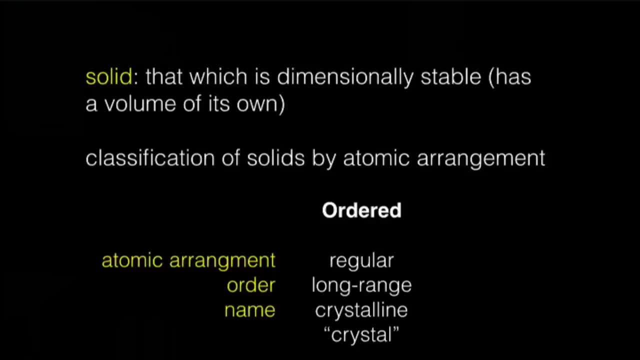 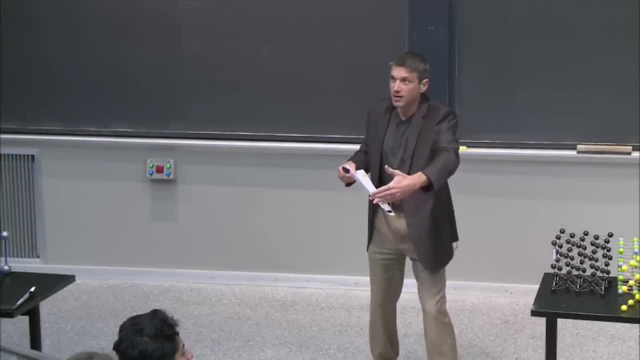 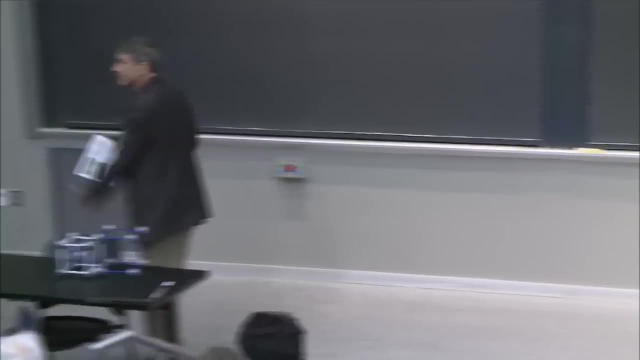 and what we call it In the first category, it's regular. So what that means is that everywhere I look, I have the same thing repeating, And you know what It repeats over a long, long way- like really long OK. 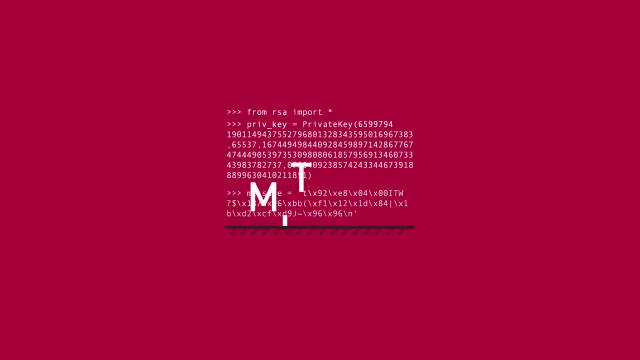 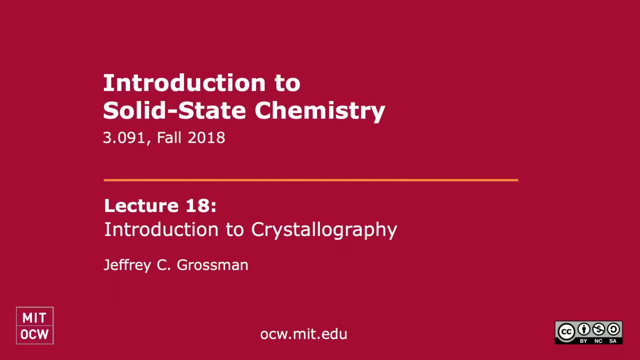 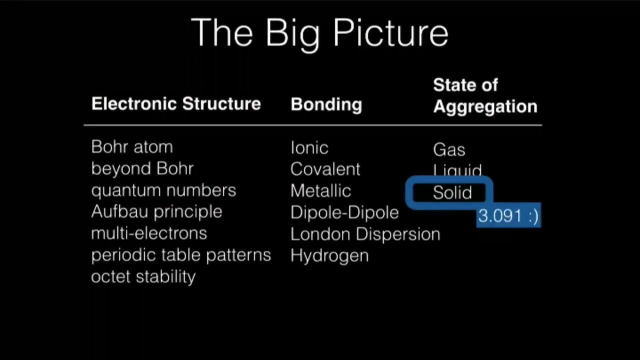 Big picture. I showed you this big picture before We're now going to add to it. Look at what we've done: Electronic structure all the way up through, you know, octet, stability, Lewis, molecular orbital theory, how to handle multi-electrons, all these different kinds. 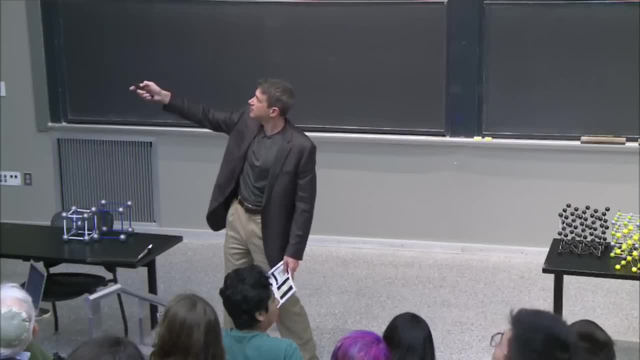 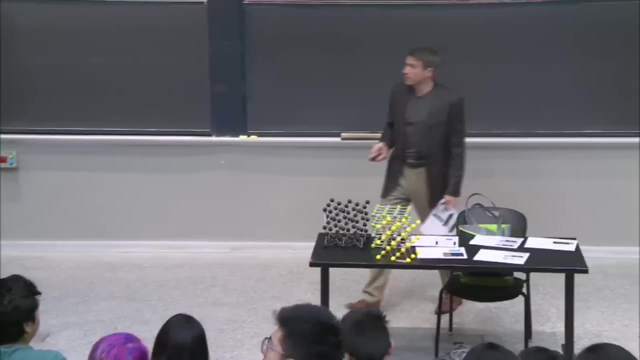 of bonding Check. We've covered every single one of these, And this is solid state chemistry. OK, but now here we are, right Now. OK, remember, we also talked about this in the very first lecture. When you classify solids, there are two things. 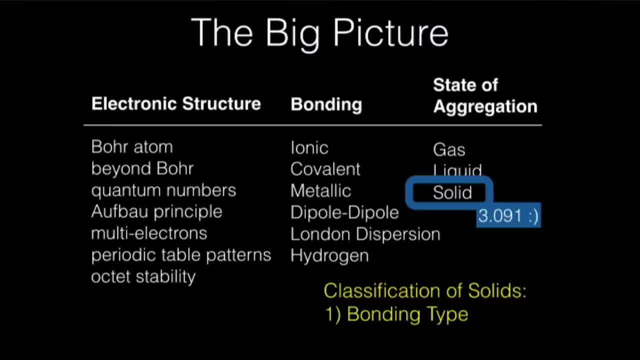 that are really important. One is the bonding type. How do the atoms in the solid want to talk to each other, How do they interact? And that is something that we have covered in a lot of different ways. But the next is how they come together. 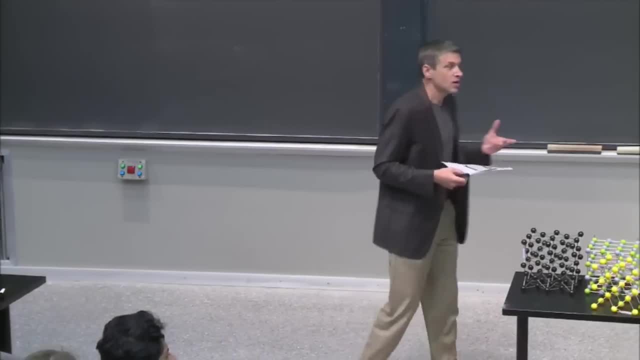 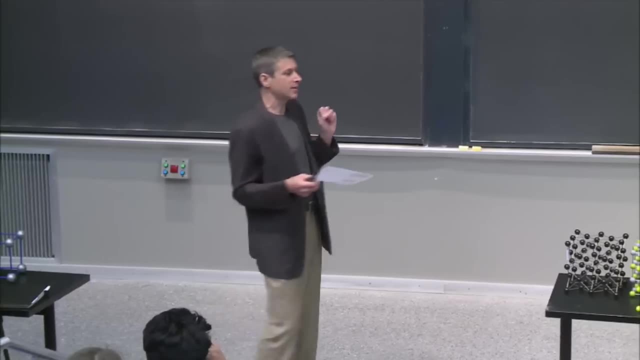 the actual arrangement of those atoms And that is what we're going to talk about today and on Wednesday, And then as we learn after Exam 2, as we learn about X-rays. that's a way to characterize the arrangement so that you can see how they're ordered. 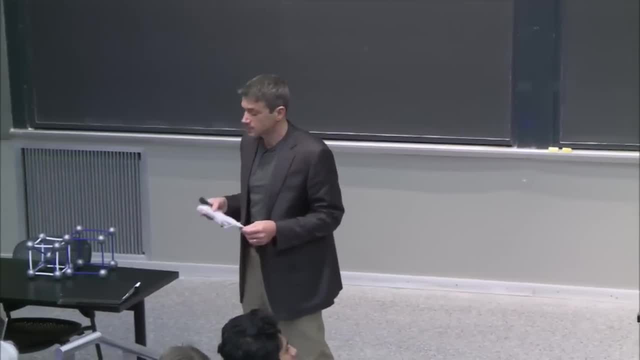 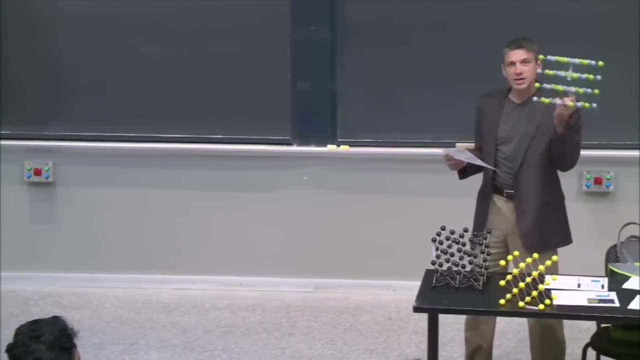 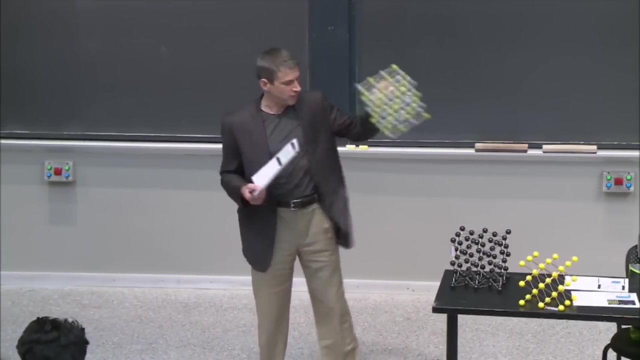 OK, we're going to use X-rays and do something called X-ray diffraction, But for this week I want to just classify. I want to talk about the things, the tools that we use to understand how a solid forms, how to describe the formation of a solid, how 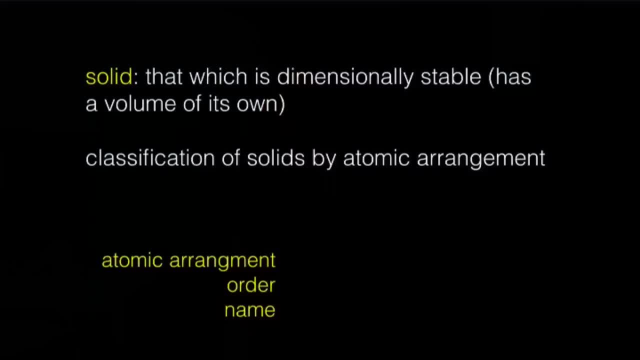 the atoms can be described. So, of course, a solid is that which is dimensionally stable. Simple definition, right. But we can break down how these atoms arrange into two basic categories: the atomic arrangement, the order, and what we call it. 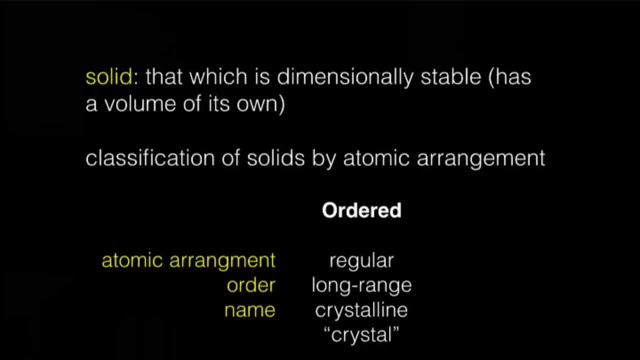 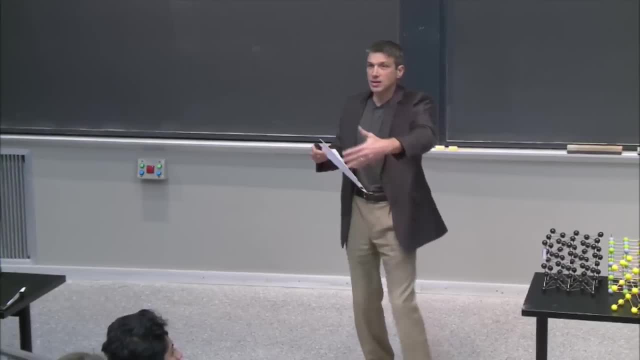 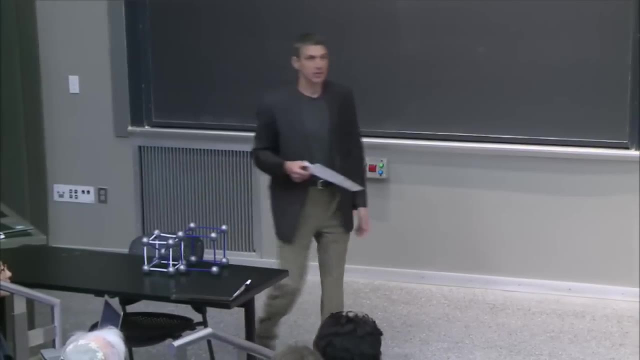 In the first category it's regular. So what that means is that everywhere I look, I have the same thing repeating, And you know what It repeats over a long, long way, like really long. OK, So that kind of regular, long range order is a crystal. 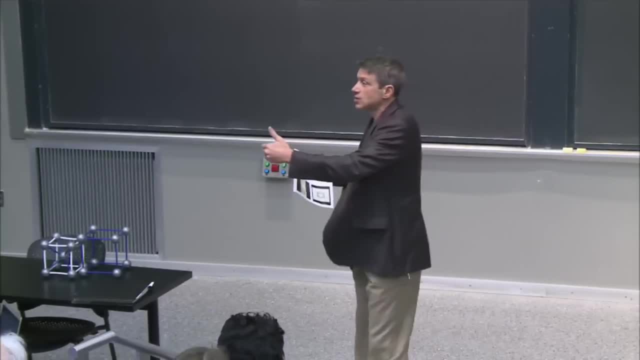 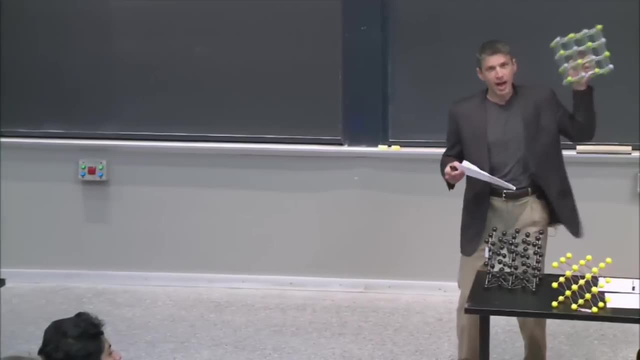 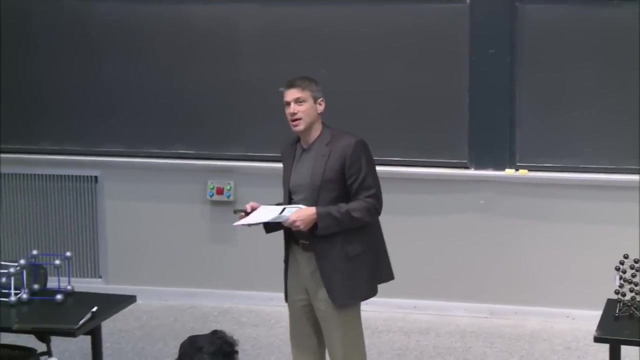 So that kind of regular long range order is a crystal, That's a crystalline solid, And that is going to be the topic of this week: crystalline solids. Now there are also solids that you can make where there isn't order. 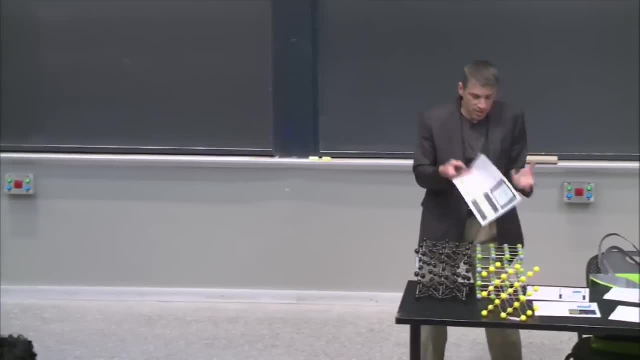 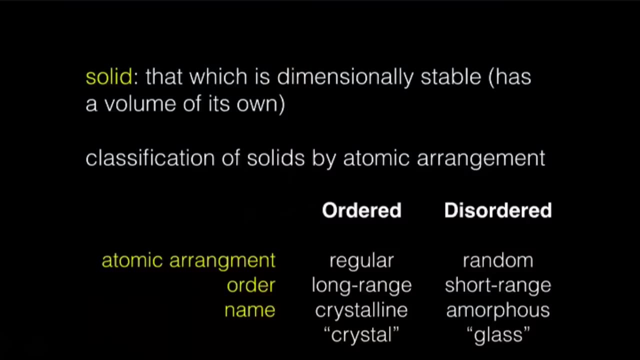 Or maybe there's some, but not much. So things are kind of jumbled up. They're not regularly repeating. They might be random, the atomic arrangement, Or maybe there's repetition, but it's very short range. So things look ordered, but only for a few bond lengths. 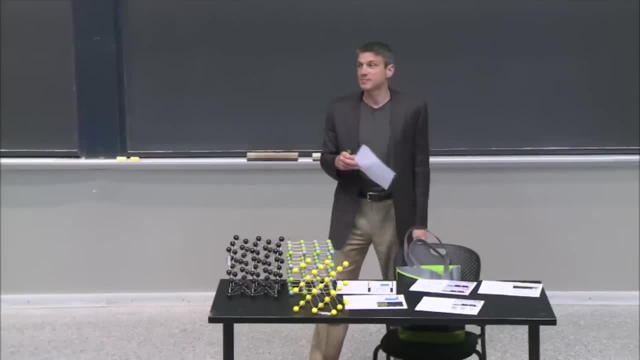 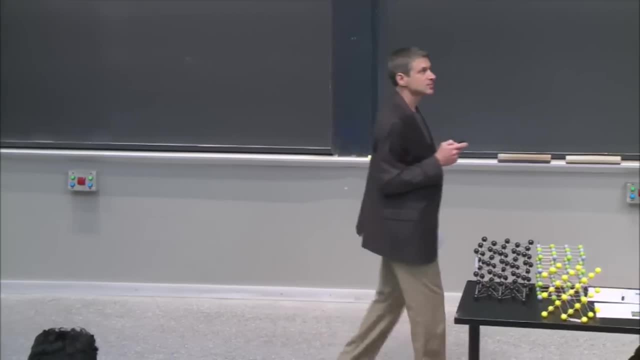 not 10 to the 23rd bond lengths- right, Those are regular. They are called amorphous solids or also glass. Now, as I mentioned, this is the topic of this week And this will be covered on exam two. 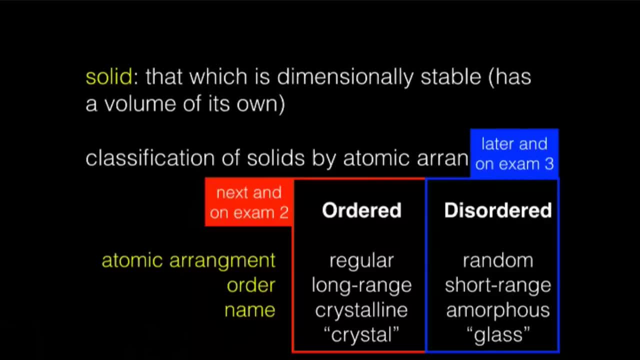 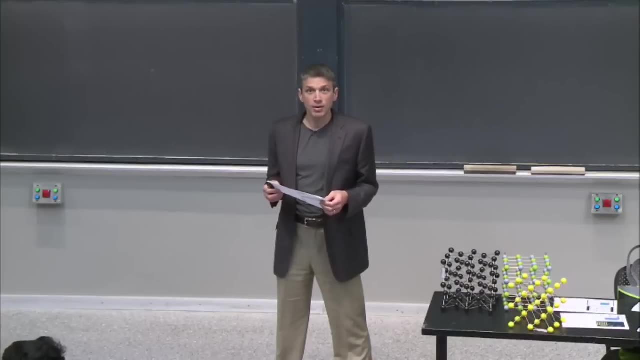 This is the topic of after exam two next week, So we'll talk about both of these types of solids as we go. All right now. OK, It turns out that nature has been thinking about order for a long, long time, And there's a reason for this. 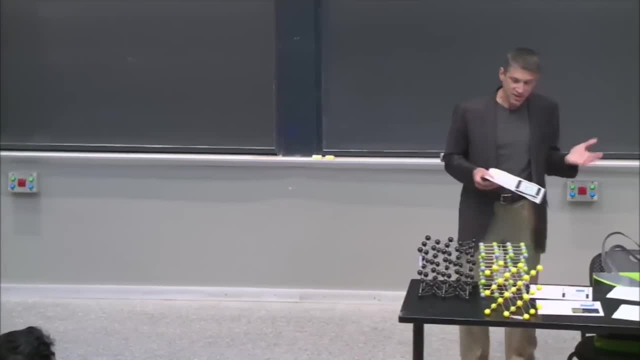 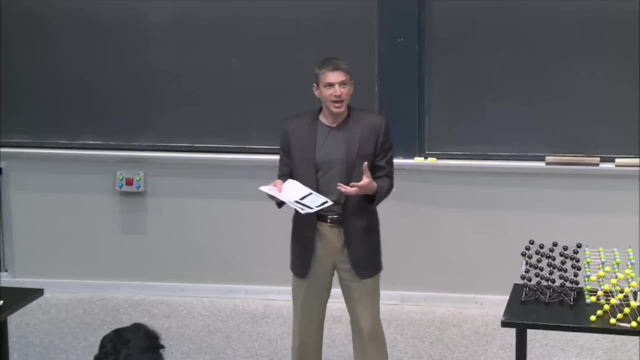 Nature, because nature wants to be efficient. This plant is like: well, I'm only going to grow this big And I got to put as many seeds as I can on the surface of this thing. How do I fit them? How do I pack them in? 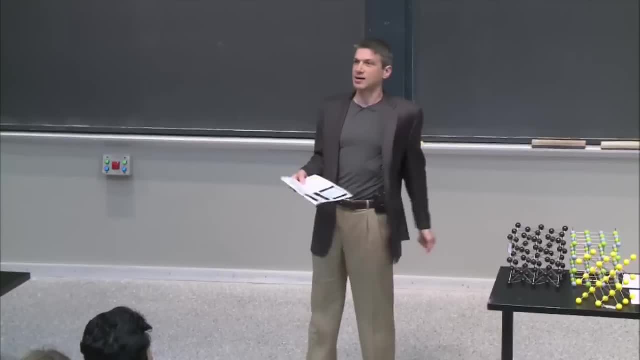 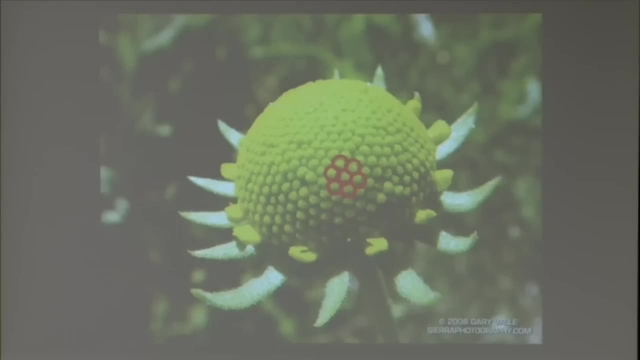 Well, I could fit them randomly, but it doesn't seem like I could get as many seeds on there. What if I packed them in in some regular pattern? What if I packed them in in some regular way? Oh well, you can pack a lot more in. 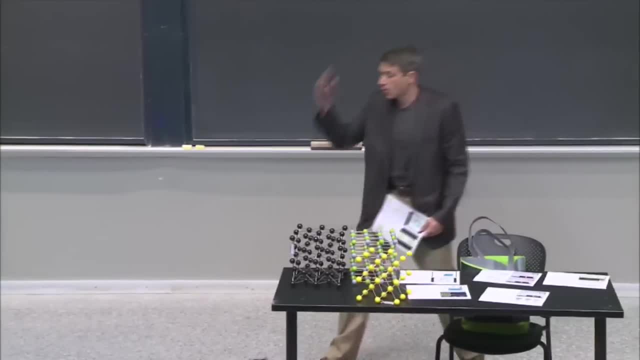 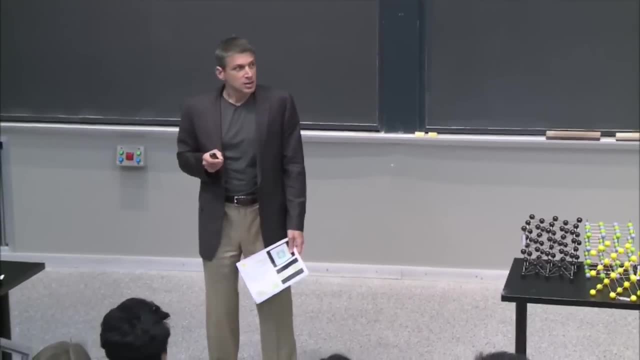 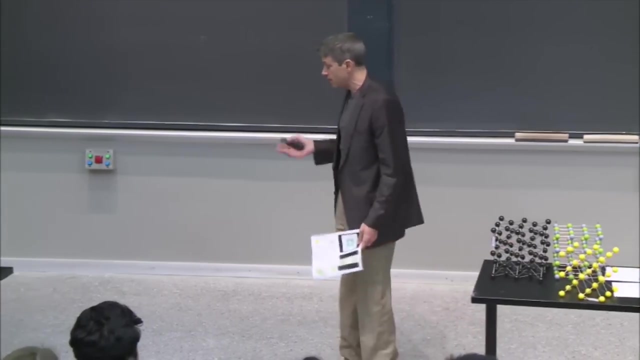 And so nature has already been thinking about symmetry and order and even long range order for a long time. People have been thinking about this too. Robert Hooke, the same person from Hooke's law in the 1600s. he was all about cannonballs. 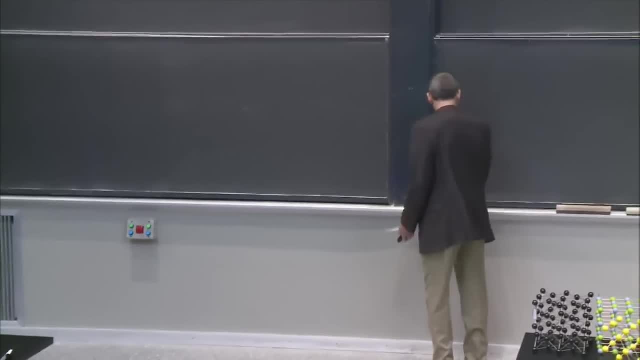 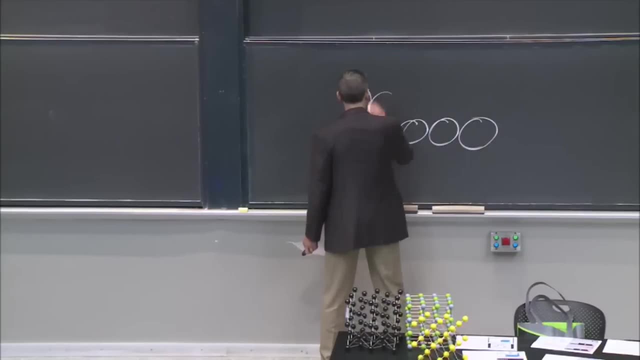 And he was like: how can I stack cannonballs? And you know he tried this right. He's like, well, maybe if I just put them like this, Is that a good way to stack them. I don't know. 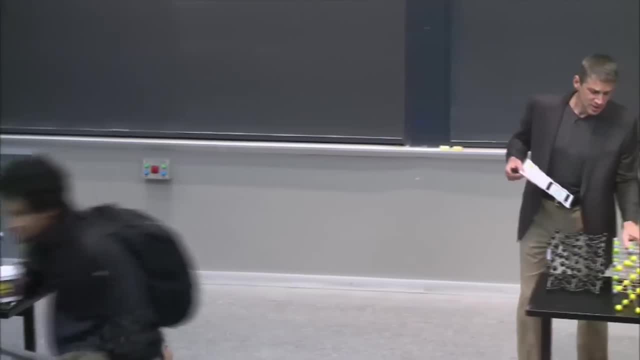 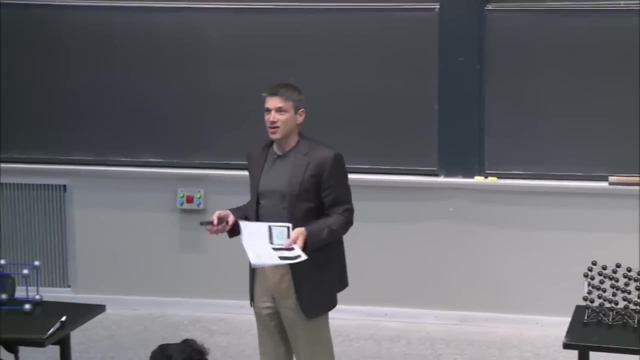 That's a crystalline solid And that is going to be the topic of this week: crystalline solids. Now there are also solids that you can make where there isn't order, Or maybe there's some, but not much, So things are kind of jumbled up. 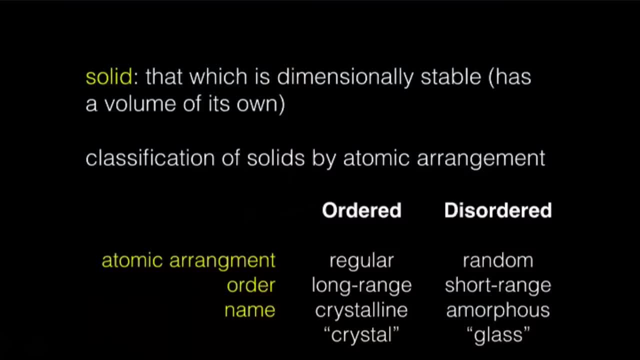 They're not regularly repeating. They might be random, the atomic arrangement, Or maybe there's repetition, but it's very short range. So things look ordered, but only for a few bond lengths, not 10 to the 23rd bond lengths, right? 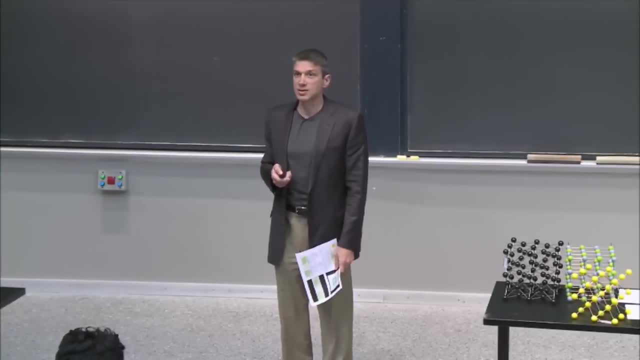 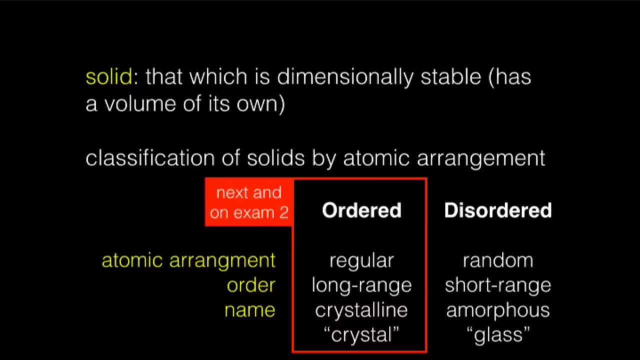 Those are regular. They are called amorphous solids or also glass. Now, as I mentioned, this is the topic of this week And this will be covered on exam two. This is the topic of after exam two next week. So we'll talk about both of these types of solids as we go. 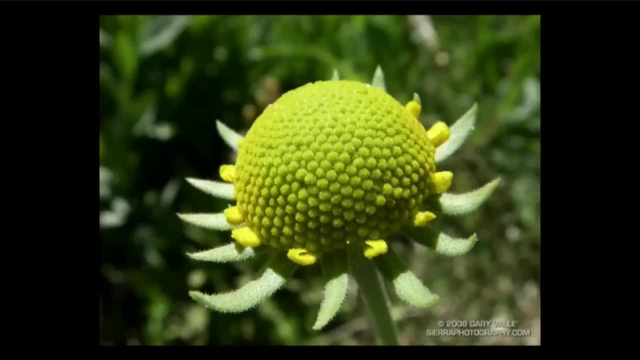 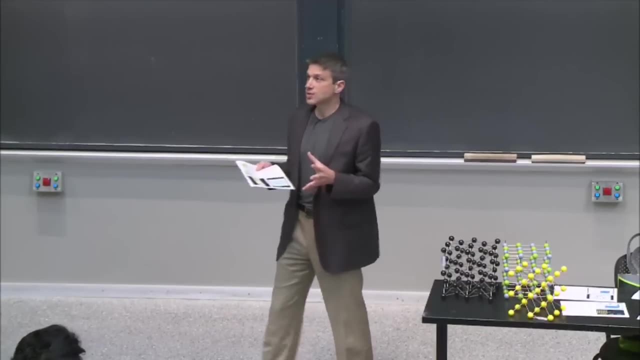 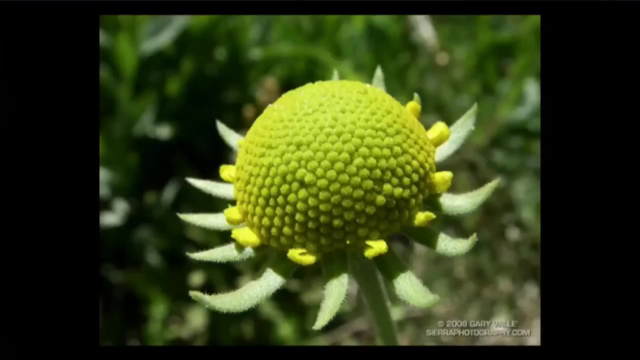 All right now. OK, It turns out that nature has been thinking about order for a long, long time. And there's a reason for this Nature: because nature wants to be efficient. This plant is like: well, I'm only going to grow this big. 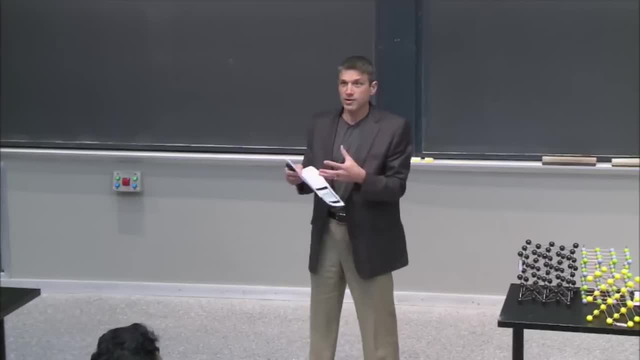 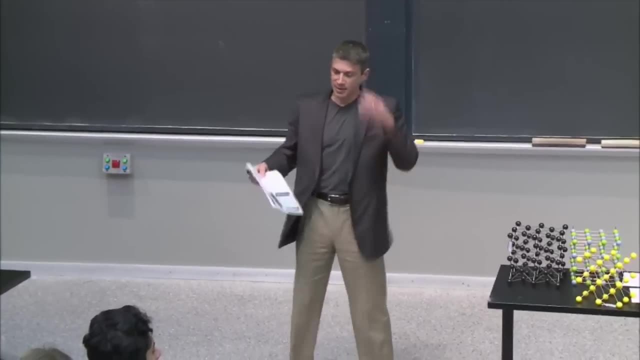 And I got to put as many seeds as I can on the surface of this thing. How do I fit them? How do I pack them in? Well, I could fit them randomly, but it doesn't seem like I could get as many seeds on there. 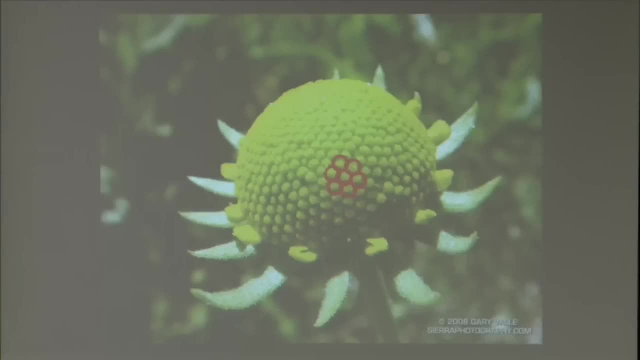 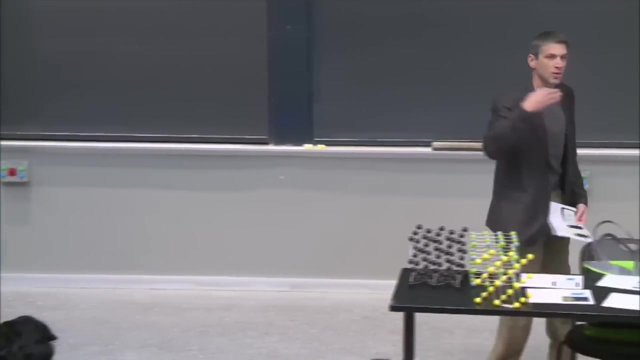 What if I packed them in in some regular pattern? What if I packed them in in some regular way? Oh well, you can pack a lot more in. And so nature has already been thinking about symmetry and order, and even long range order for a long time. 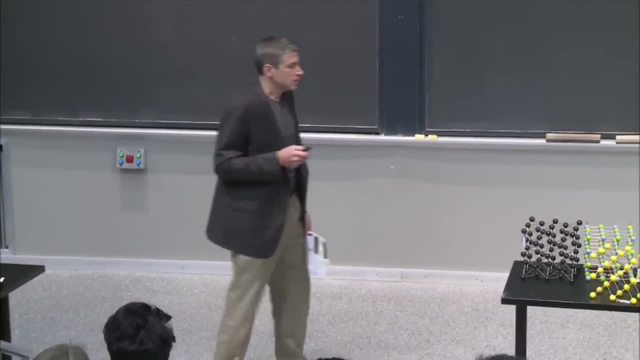 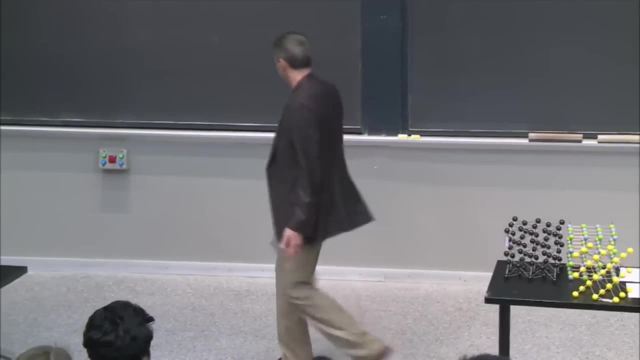 People have been thinking about this too. Robert Hooke, the same person from Hooke's Law in the 1600s. he was all about cannonballs And he was like, how can I stack cannonballs? And you know, he tried this right. 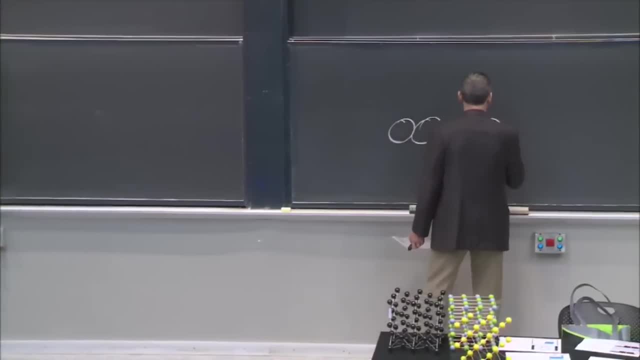 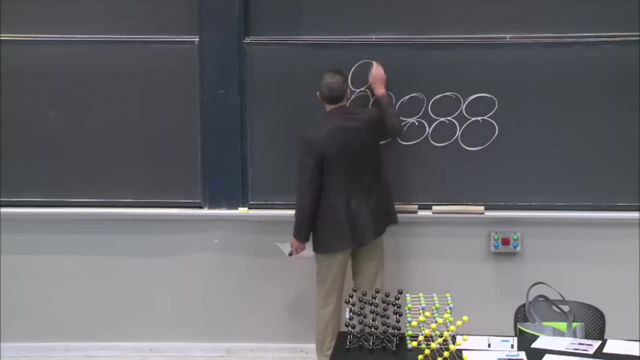 He was like: well, maybe if I just put them like this, is that a good way to stack them, I don't know. And then he sort of put them all together, But now he tried this and then he tried another arrangement. 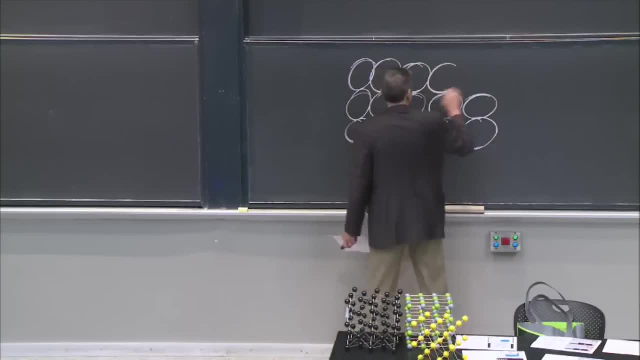 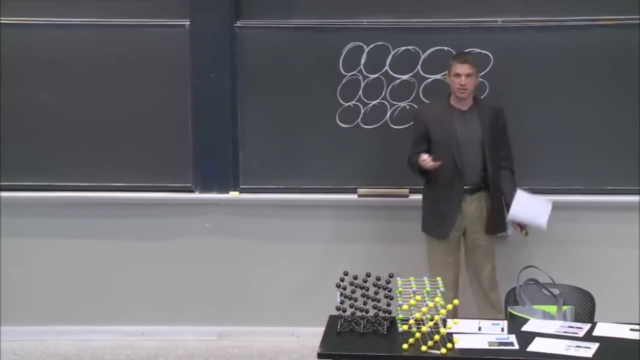 And then he sort of put them all together. But now he tried this and then he tried another arrangement And he'd be like: well, but how? First of all, are they stable? Do they fall over easily? because you don't want cannonballs falling all over the place. 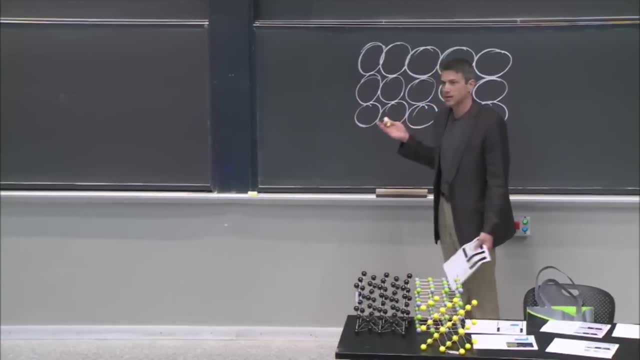 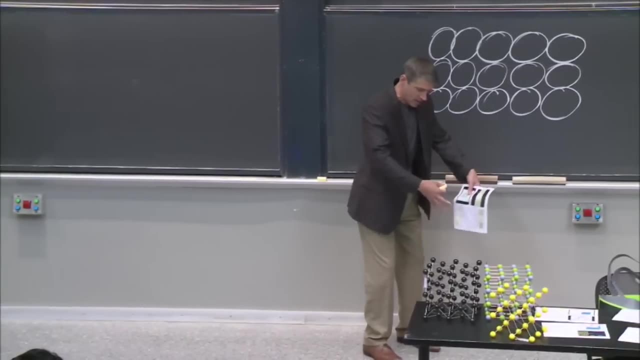 But then also did you pack as much in this way as another way? So he was thinking about it and he figured out that you could pack more cannonballs in for the same area or volume if you sort of switched it up, right. 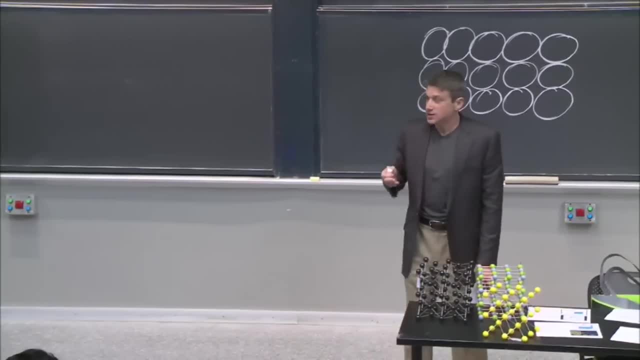 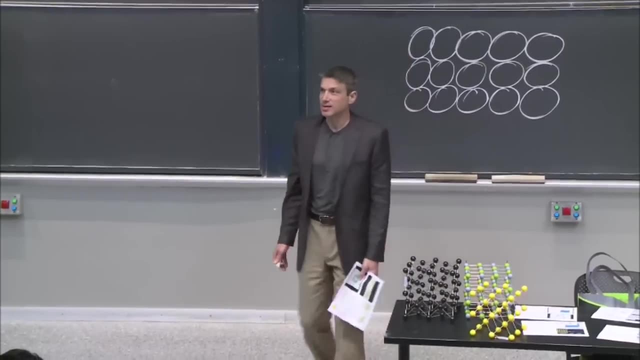 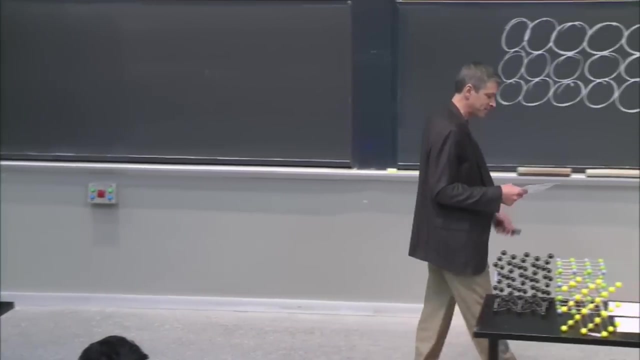 And then he thought, well, maybe other things have packing too. And he thought about all sorts of things. He looked at salt crystals and he said they must also pack in some way, because cannonballs do. So people have been thinking about this for a long time. 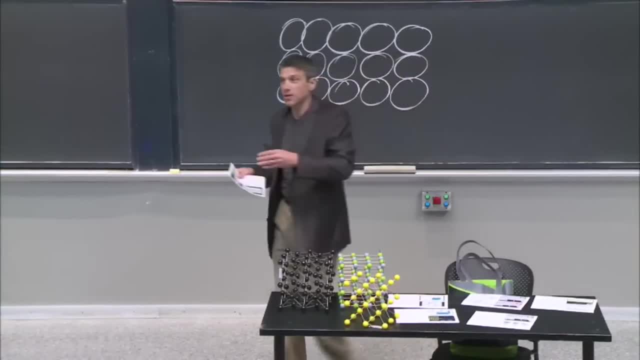 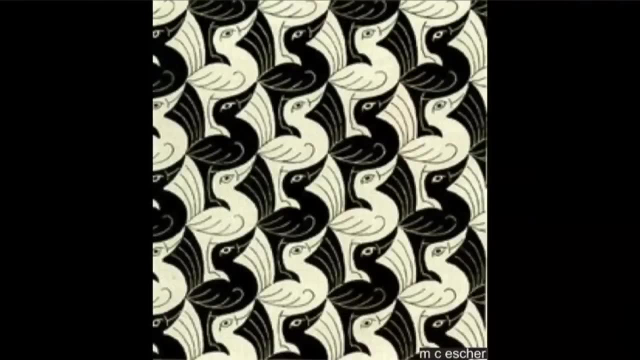 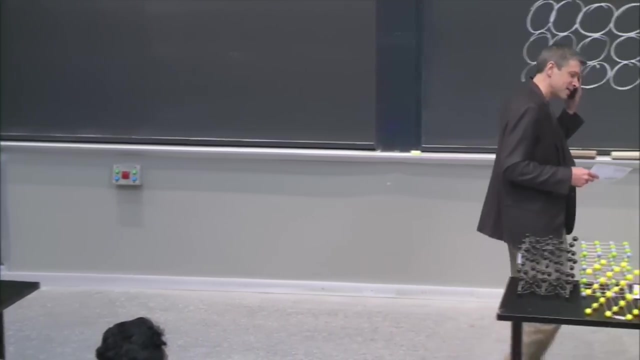 Now, people are also inspired by regular order, right. So If you look at, for example, an Escher painting, you can see that there is a repetitive pattern here. This is a crystal of ducks right Now. when you look at patterns like this, you have to well. 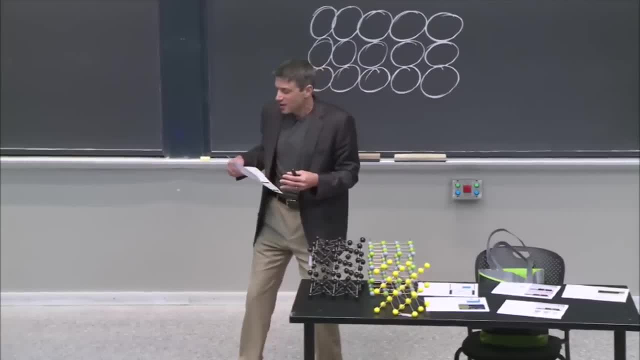 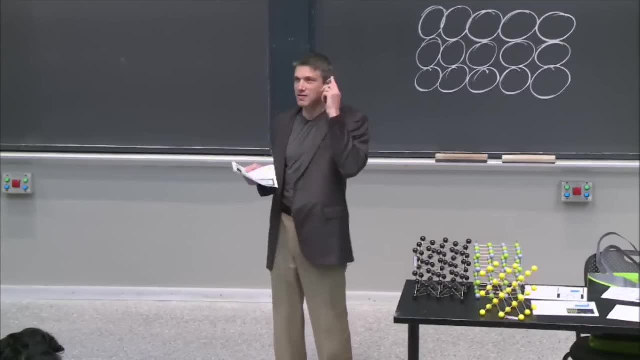 you don't have to, but we have to. in this class We've got to figure out what is the repeating unit. What is it that is repeating everywhere? So that's the first question we need to ask, And you can see if you look at this picture. 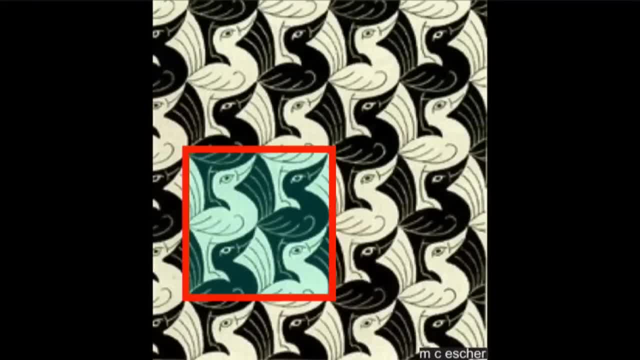 you can draw a box like that: There's a box around a light-colored, dark-colored duck, And now you see, if you take this box and you move it over, you translate it over there, you get exactly the same thing. 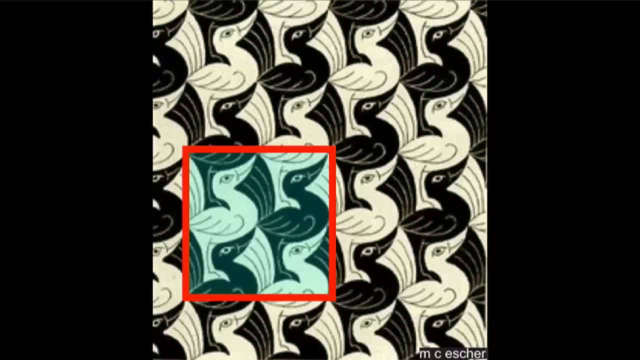 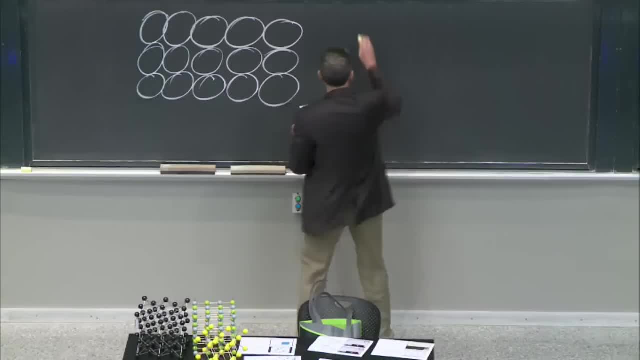 What if you take that box and you put it up there? you get exactly the same thing. So that is a repeating unit. That is a repeating. Oh, we have a definition. It's a unit cell. It's called a unit cell. 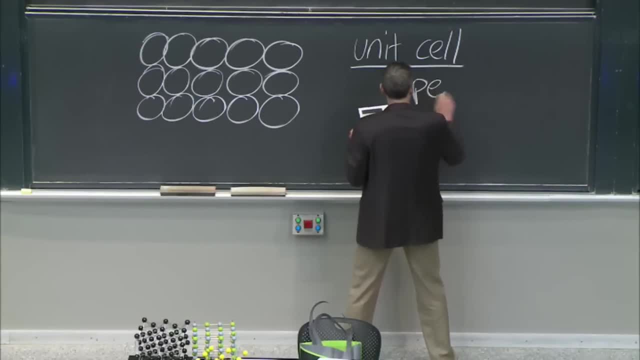 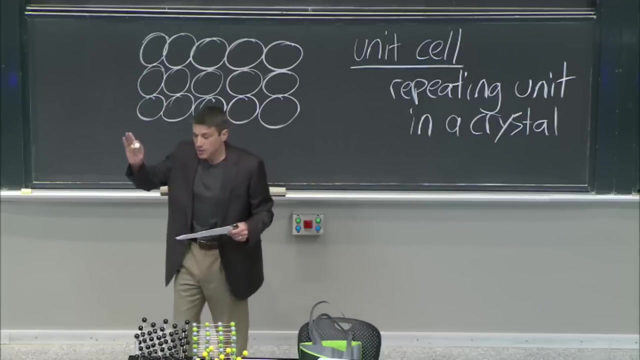 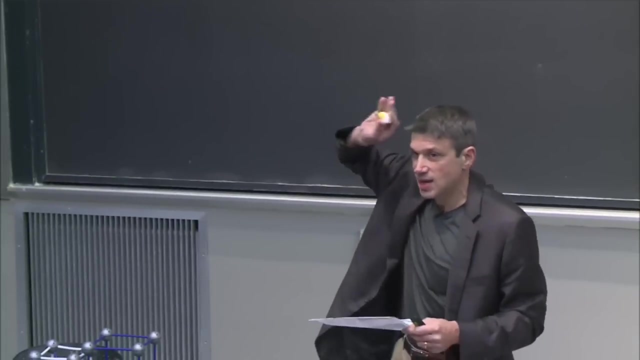 And it's the repeating unit in a crystal. It's a repeating unit. Now, it's not always obvious, So there's one way that I could repeat and take this and make the picture by repeating it everywhere. But check this out, I could have done that. 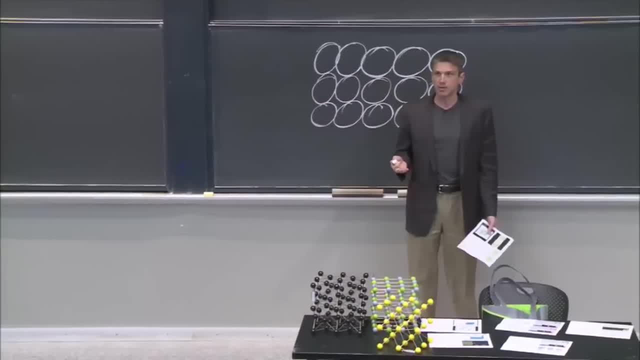 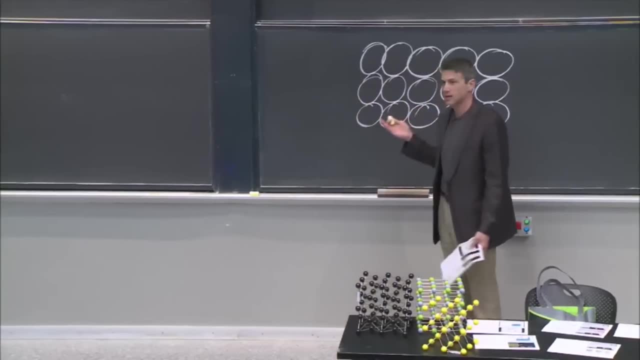 And he'd be like: well, but how? first of all, are they stable? Do they fall over easily? because you don't want cannonballs falling all over the place. But then also, did you pack as much in this way as another way? 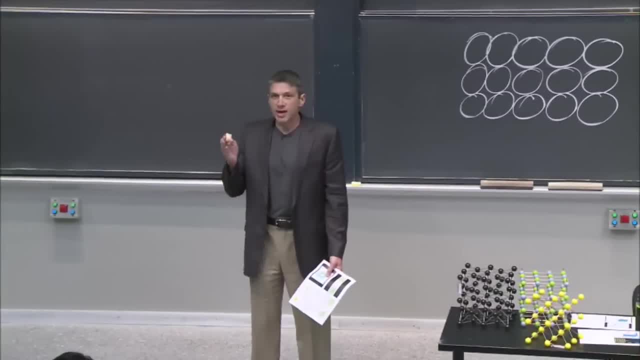 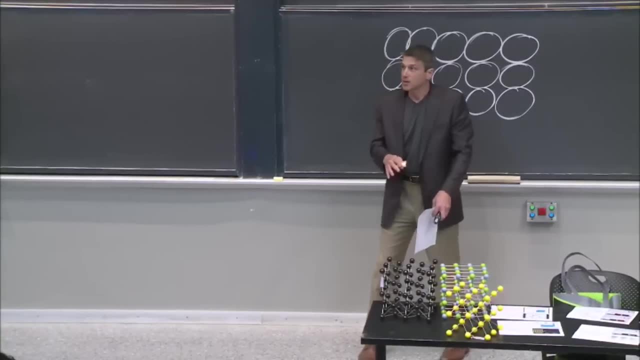 So he was thinking about it And he figured out that you could pack more cannonballs in for the seeds. You'd have the same area or volume if you sort of switched it up right. And then he thought, well, maybe other things have packing too. 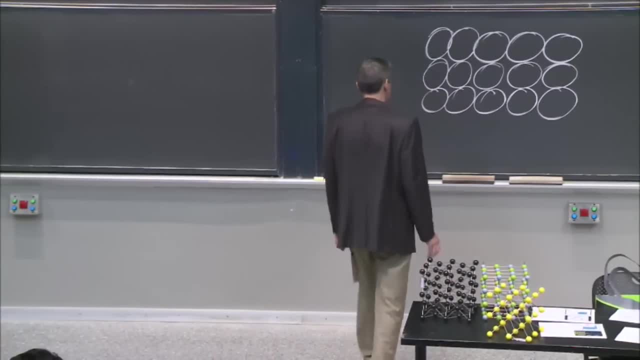 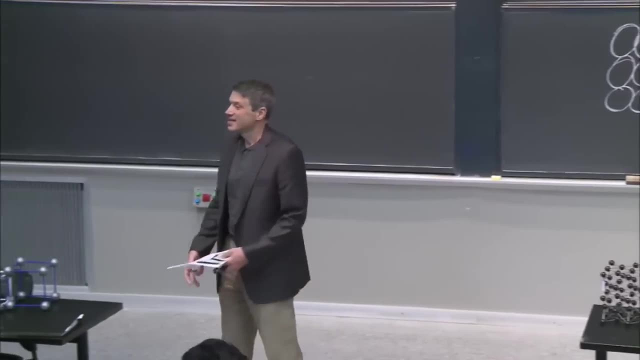 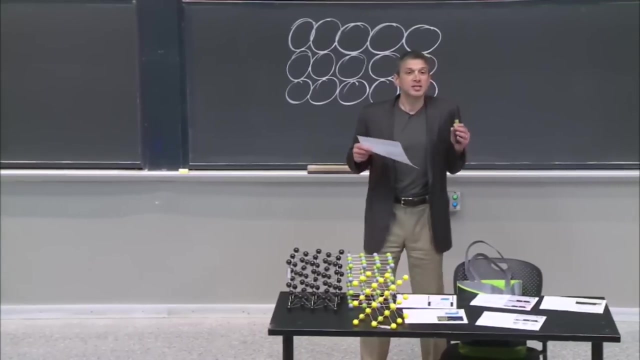 And he thought about all sorts of things. He looked at salt crystals and he said they must also pack in some way, because cannonballs do. So people have been thinking about this for a long time Now. people are also inspired by regular order, right? 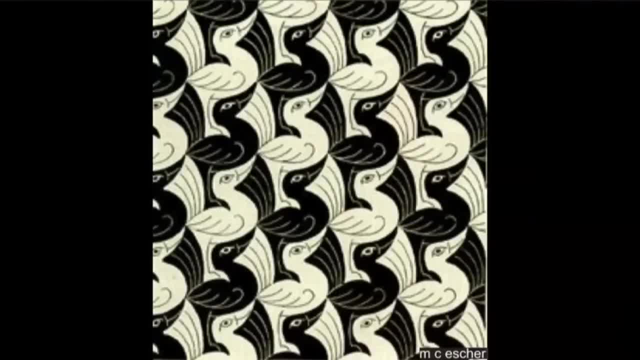 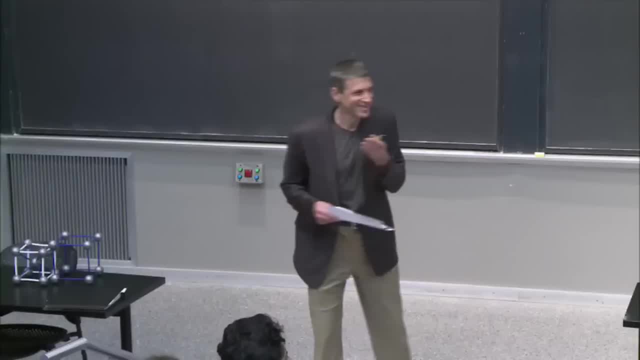 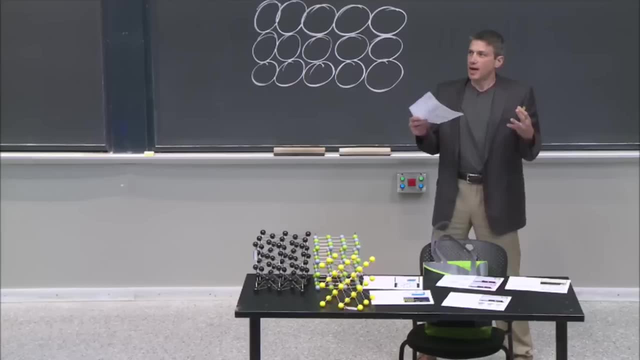 So if you look at, for example, an Escher painting, you can see that there is a repetitive pattern here. This is a crystal of ducks right Now. when you look at patterns like this, you have to. Well, you don't have to, but we have to in this class. 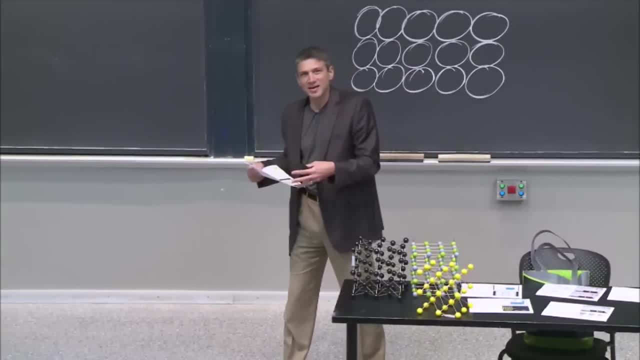 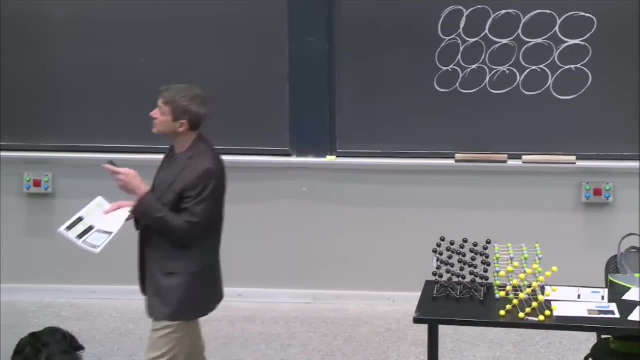 We've got to figure out what is the repeating unit? What is it that is repeating everywhere? So that's the first question We need to ask. And you can see if you look at this picture, you can draw a box like that. 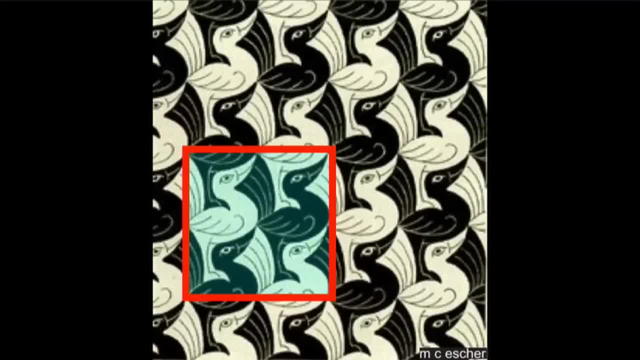 It's a box around a light-colored, dark-colored, duck and down. You see, if you take this box and you move it over, you translate it over there, you get exactly the same thing. What if you take that box and you put it up there? 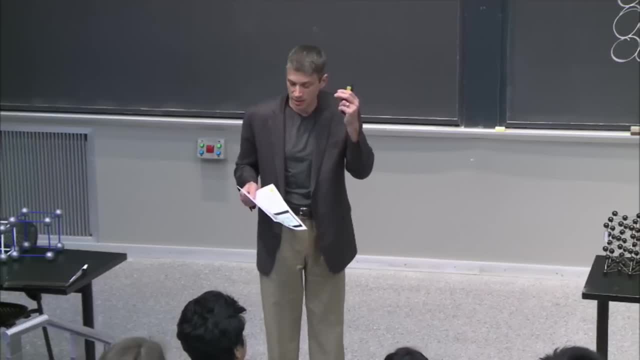 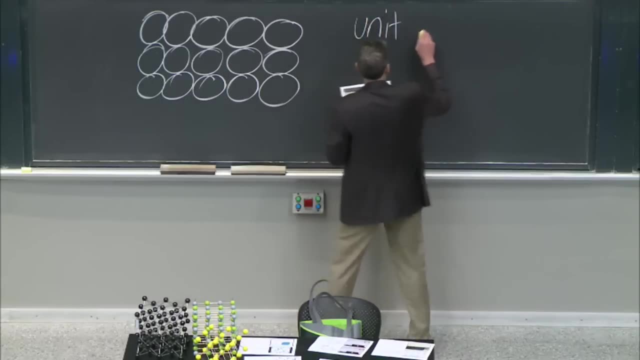 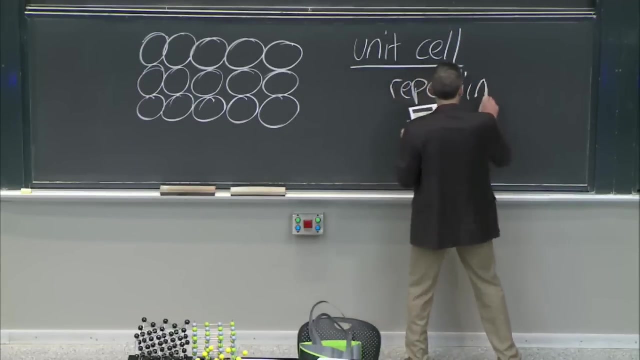 you get exactly the same thing. So that is a repeating unit. That is a repeating. Oh, we have a definition. It's a unit cell, It's called a unit cell And it's the repeating unit in a crystal. It's a repeating unit. 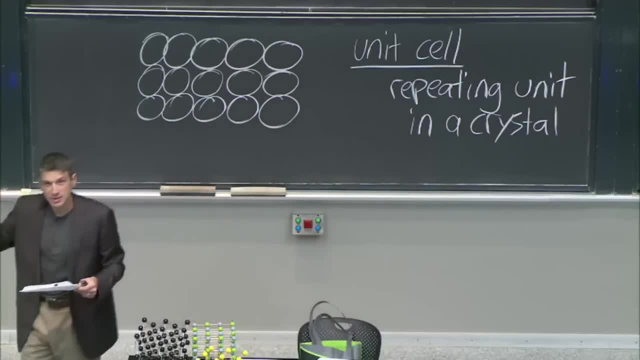 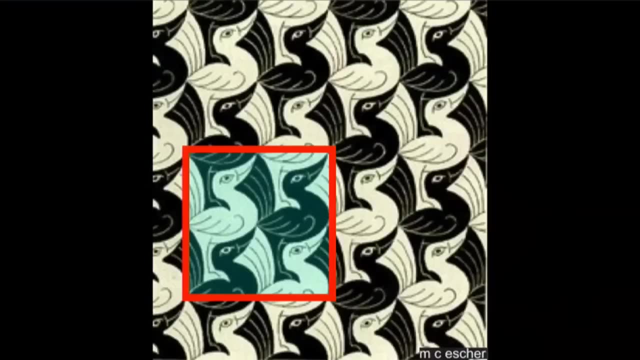 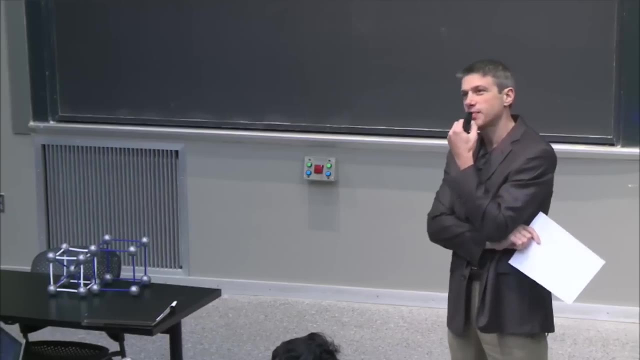 Now it's not always obvious. So there's one way that I could repeat and take this and make the picture by repeating it everywhere. But check this out, I could have done that. If you stare at that, you can see that that is also a repeating unit. 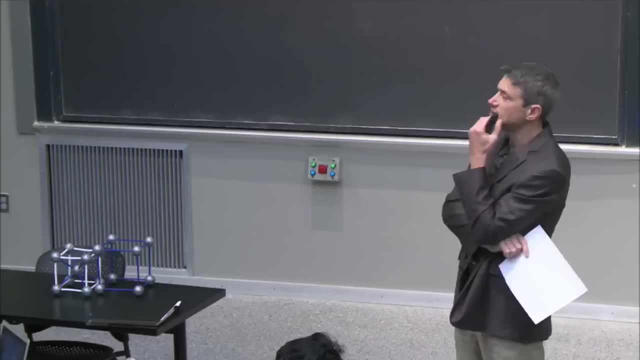 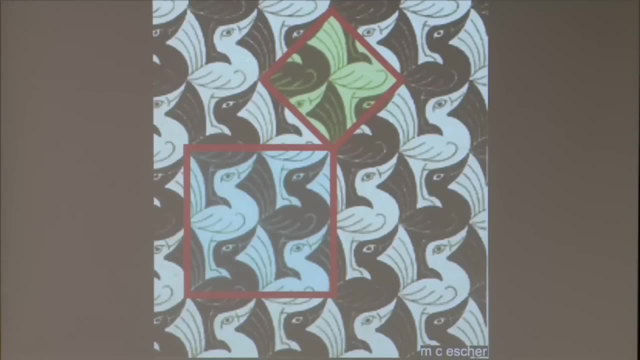 Why don't you do that? All right, If you stare at that, you can see that that is also a repeating unit. That is also a repeating unit That if I take this and I move it down here, I get exactly the same thing. 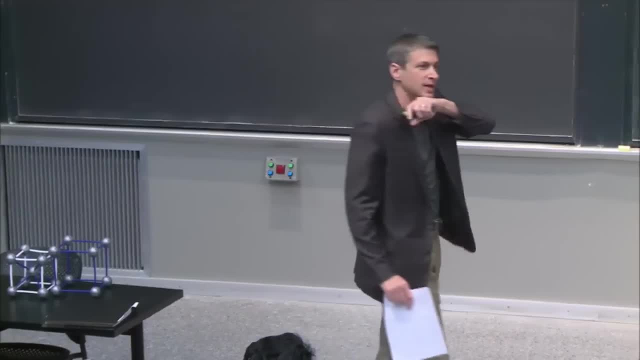 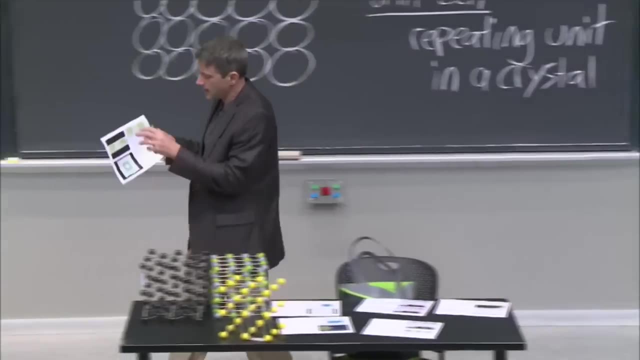 And I move it over there And I can tile all of space. I can tile all of space And something is really important here: I can take these repeating units and stamp them- Oh, I like that word- And I can tile. 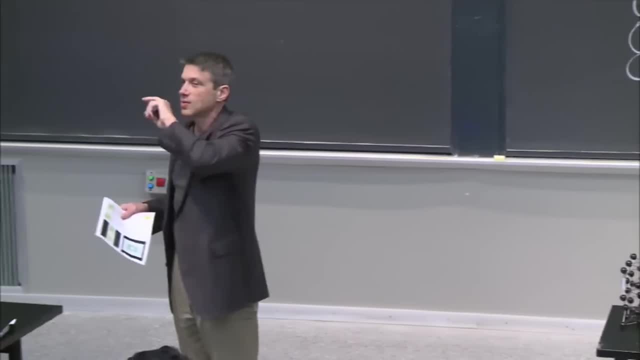 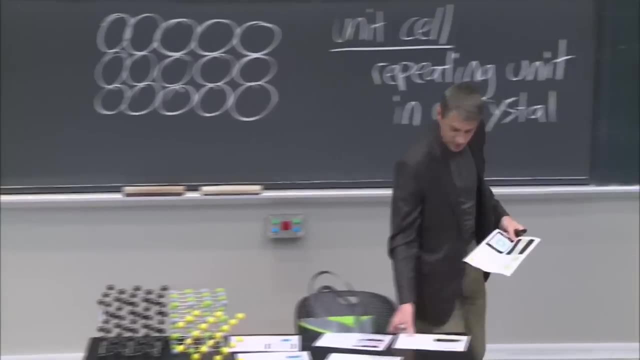 And I can tile all of space and recreate this picture without any voids. I didn't miss anything. I filled all of space. I filled all of space, And that is what a crystal system is: A crystal system. Let's write it here. 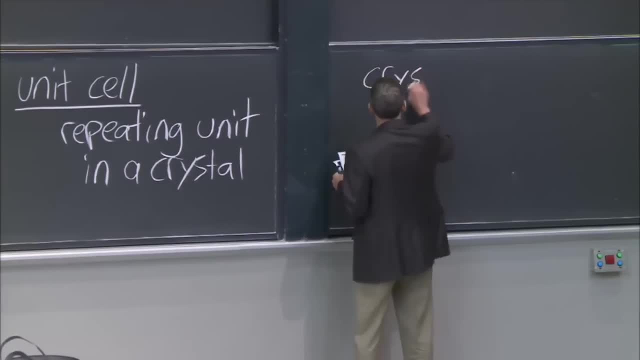 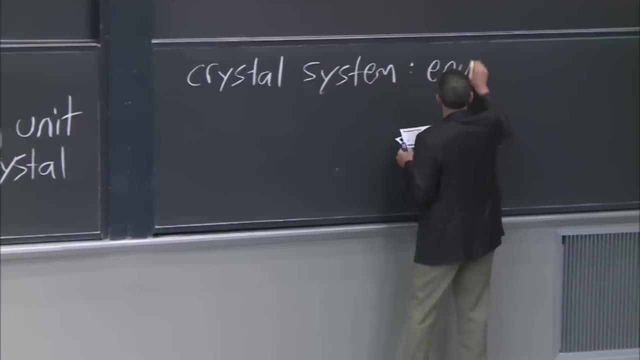 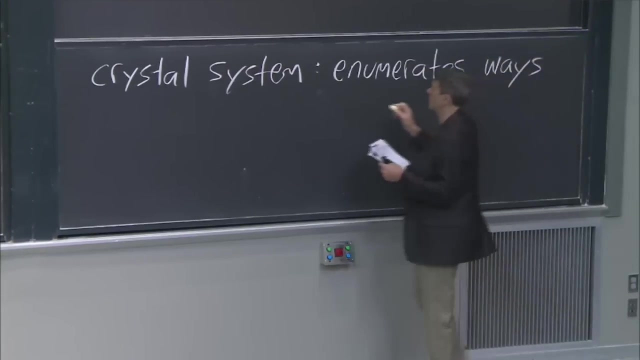 A crystal system. Crystal system- That is a way of enumerating Enumerates. Enumerates ways that space can be filled. Enumerates ways that space can be filled with no voids. Enumerates ways that space can be filled with no voids. 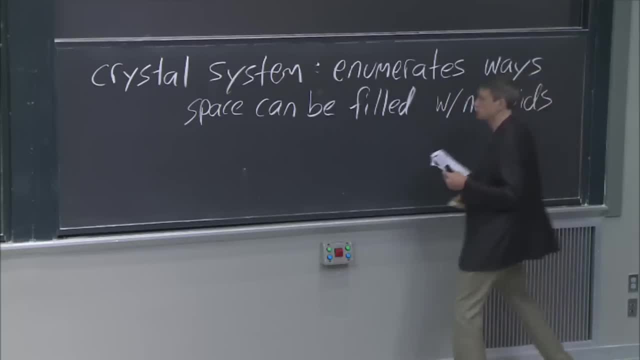 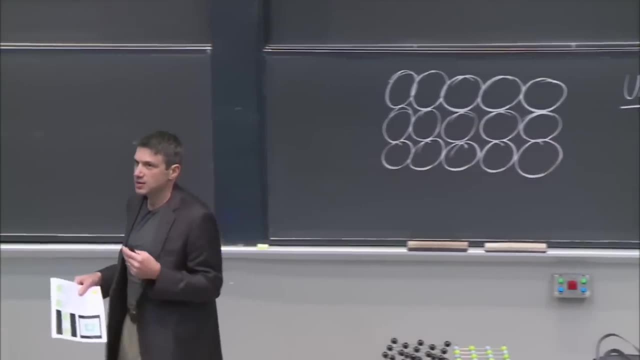 Enumerates ways that space can be filled with no voids. That's a crystal system, OK, Well, let's go back to the canons for a minute, Because we can think about this first in 3D, before we were just warming up. 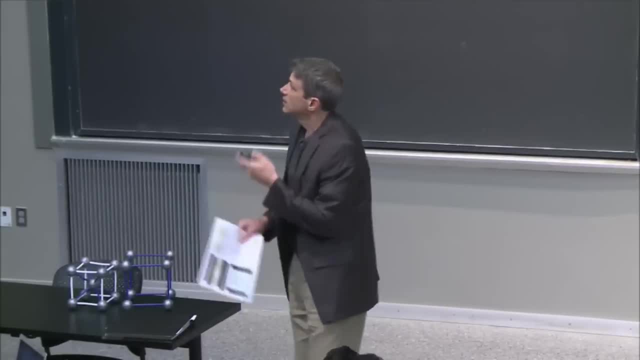 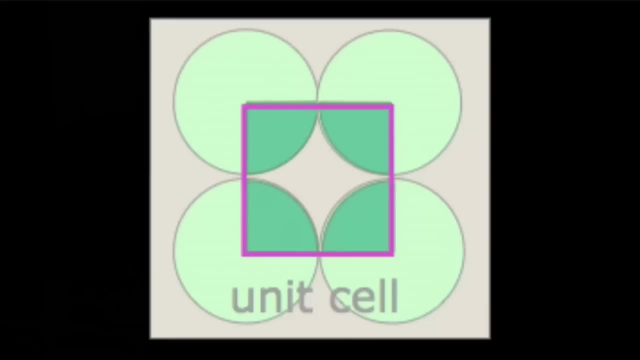 Before we get to 3D: OK, Now, OK, So, oh, there it is, That's a unit cell. OK, Now, the thing is so I've drawn a unit cell And notice what I've done. 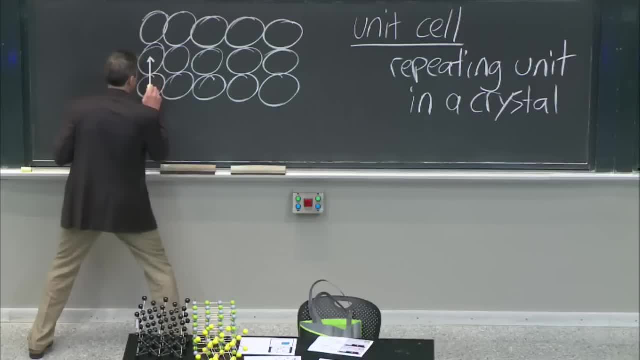 I've taken this And I'm drawing it this way. OK, And those vectors define the unit cell, Those vectors define the unit cell. So those are my stamps, The vectors there, So these things here. well, they went a little. 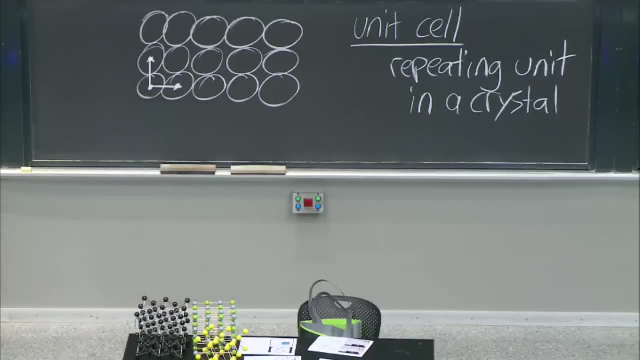 far there, but they should go to the center of the next cannonball. So now these are vectors. If I just take these and I put them Now, if I translate them over to there, then I get the next unit cell and the next one. 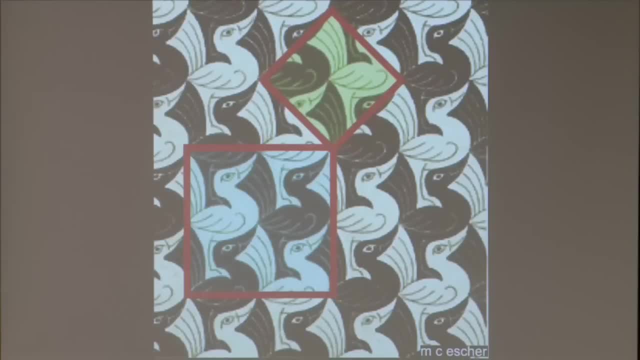 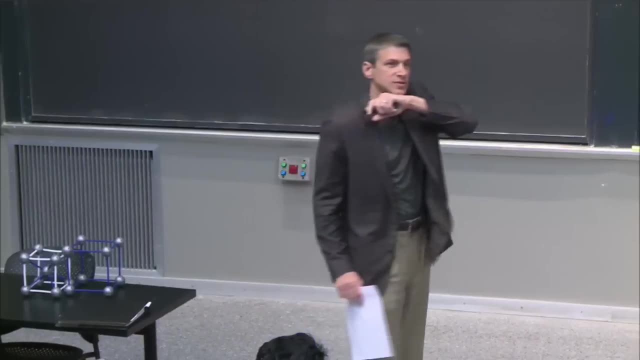 That is also a repeating unit, That if I take this and I move it down here, I get exactly the same thing, And I move it over there and I can tile all of space. I can tile all of space. And something is really important here: 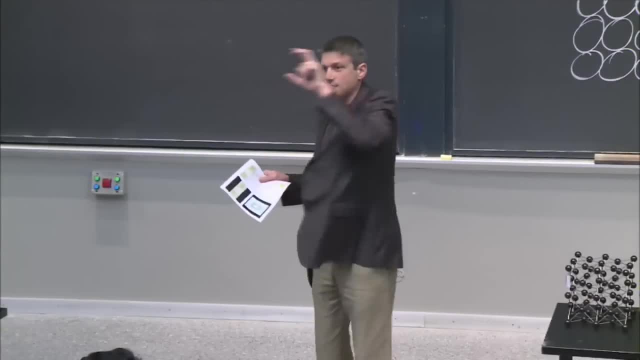 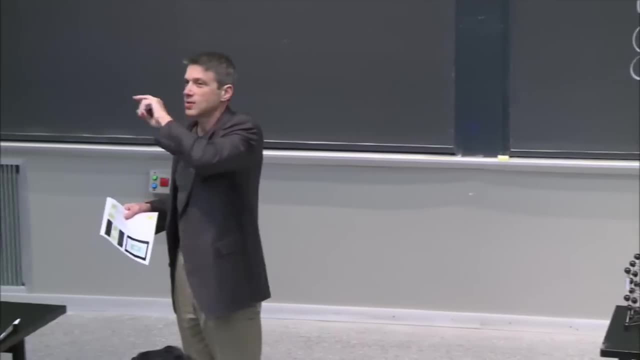 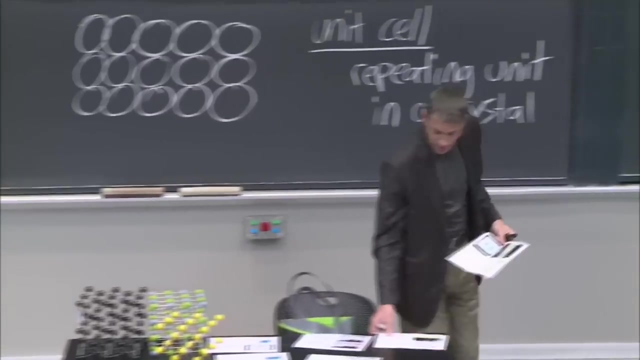 I can take these repeating units and stamp them- Oh, I like that word- And I can tile all of space and recreate this picture without any voids. I didn't miss anything. I filled all of space. I filled all of space. 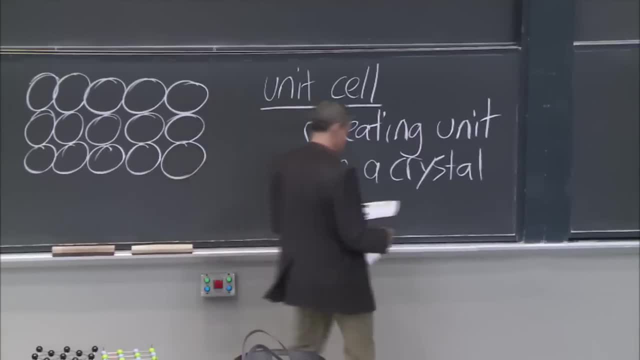 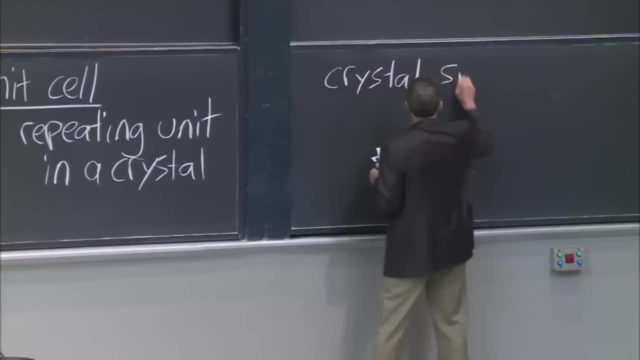 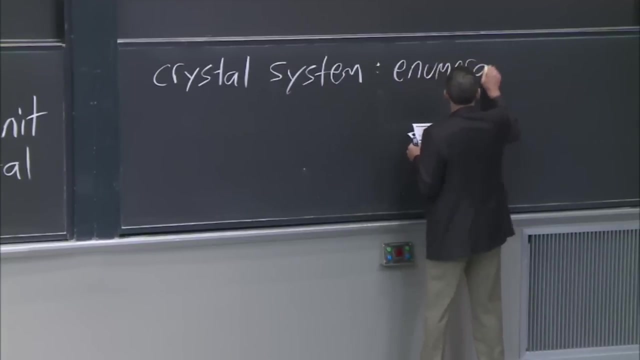 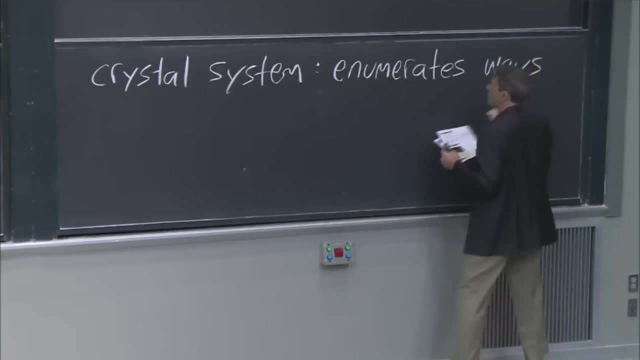 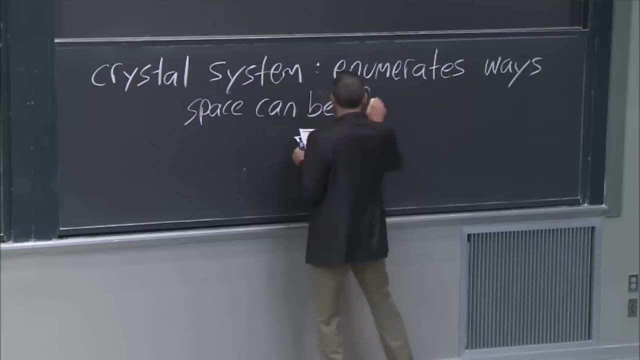 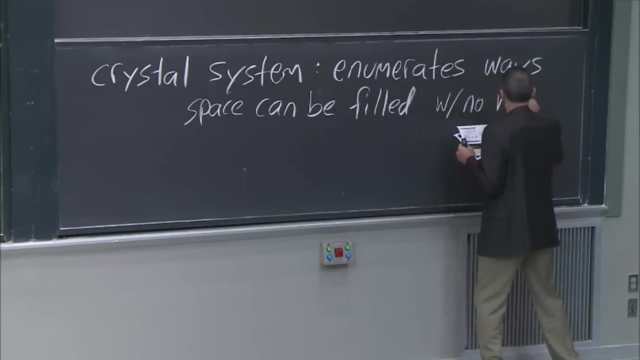 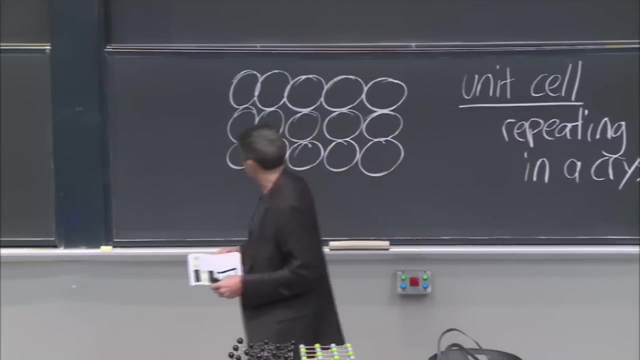 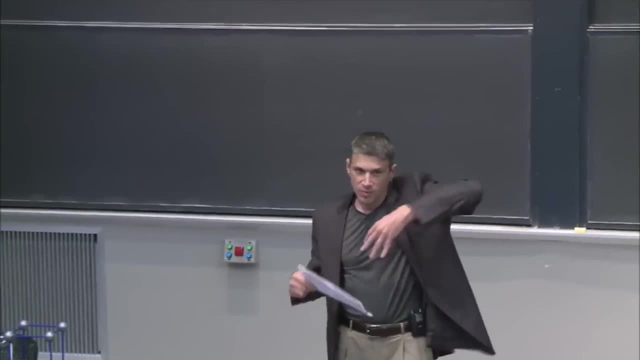 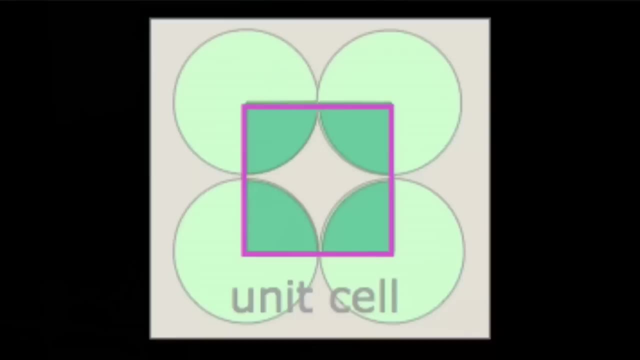 because we can think about this first in 3D, before we were just warming up, before we get to 3D. OK, Now, OK, so there it is. That's a unit cell. OK, now the thing is so. I've drawn a unit cell. 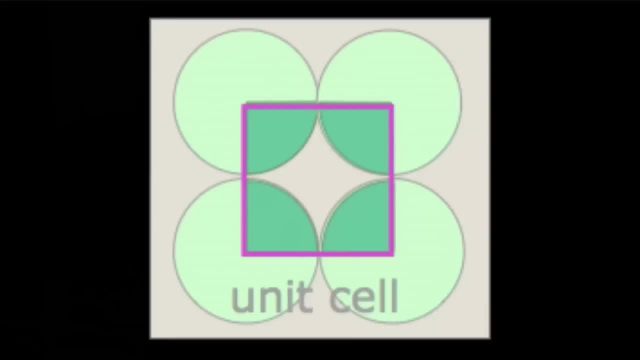 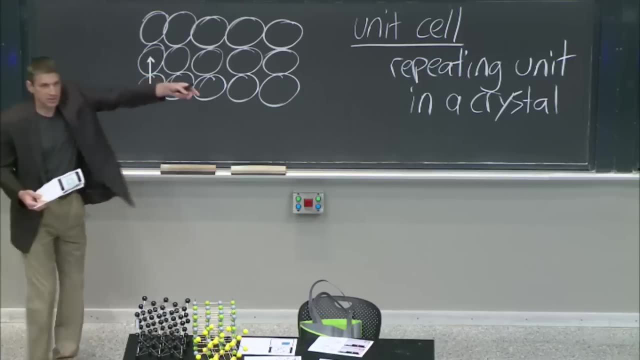 And notice what I've done. I've taken this and I'm drawing it this way. OK, And those vectors define the unit cell right. Those vectors define the unit cell. So those are my stamps, the vectors there, So these things here. well, they went a little far there. 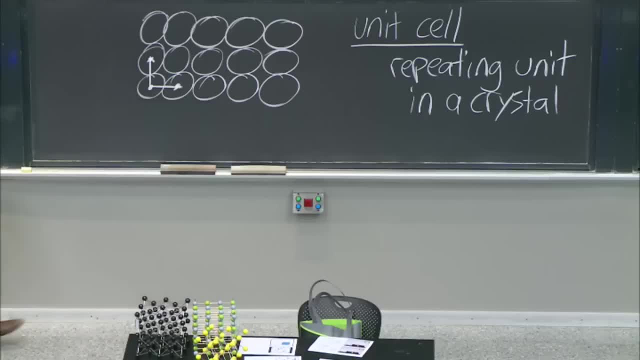 but they should go to the center of the next cannonball. So now these are vectors. If I just take these and I put them now, if I translate them over to there, then I get the next unit cell and the next one. 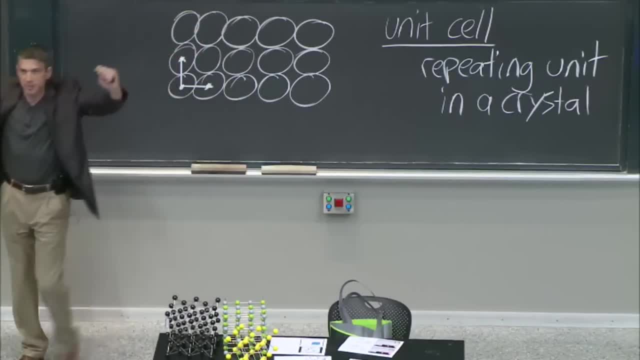 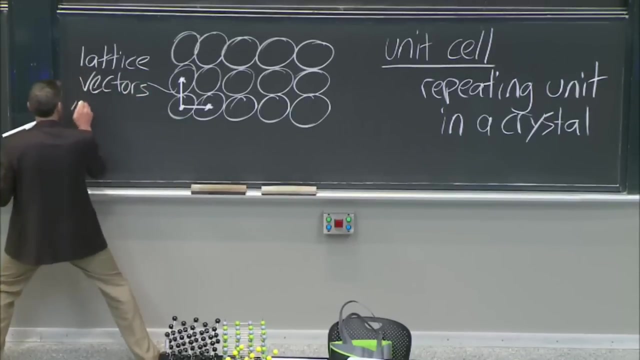 And I go up and I go over and I get all the tiling of all space, And so those vectors are really important and they have a name. Those are called the lattice vectors. Those are the lattice vectors. I really like to think of them as my stamps or my stamp. 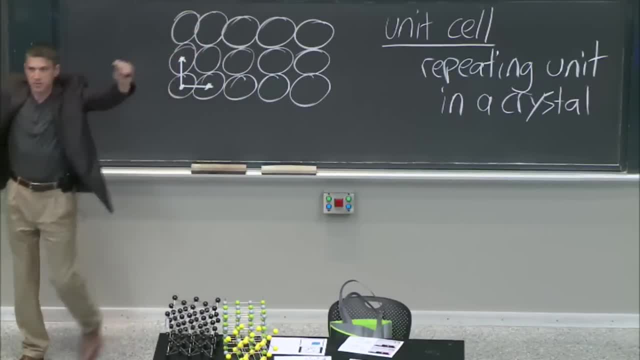 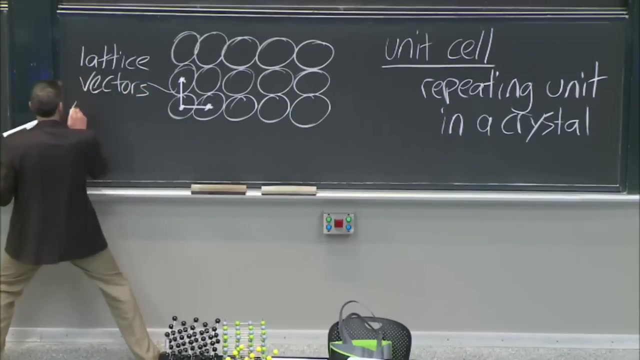 And I go up and I go over and I get all the tiling of all space, And so those vectors are really important and they have a name. Those are called the lattice vectors. Those are the lattice vectors I. I really like to think of them as my stamps or my stamp. 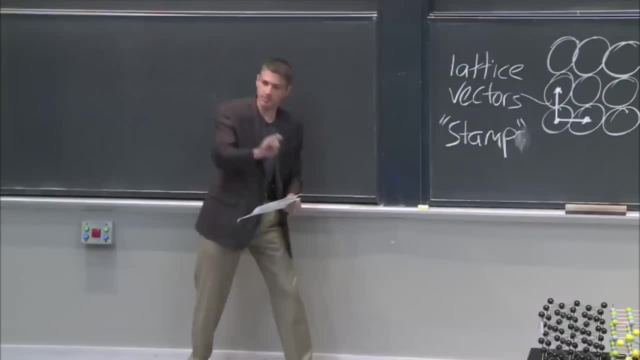 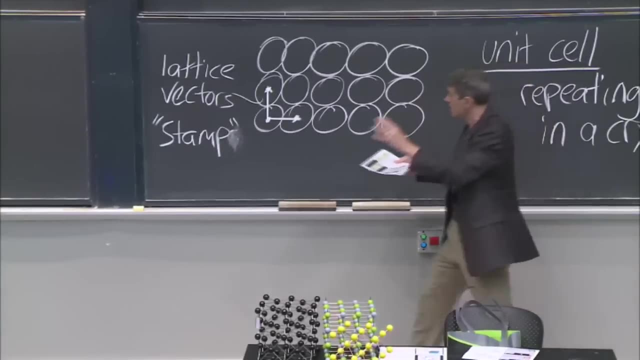 It is a stamp And no voids. These vectors are my stamp. Now I'm stamping all of space. I didn't really say what I'm putting there. I mean here there's cannonballs, In Escher there's ducks. 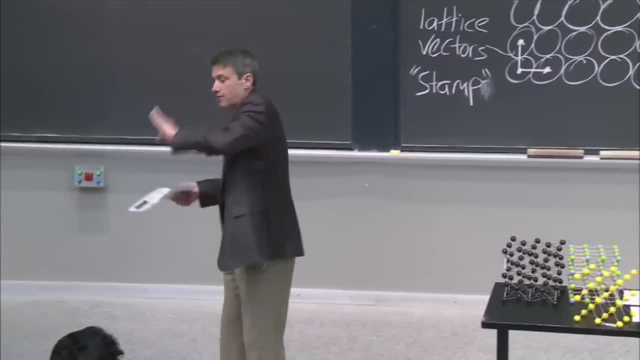 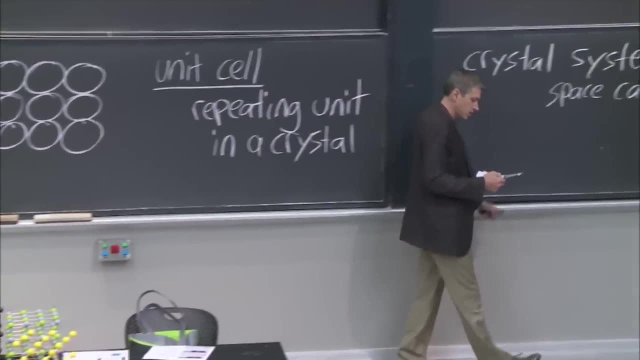 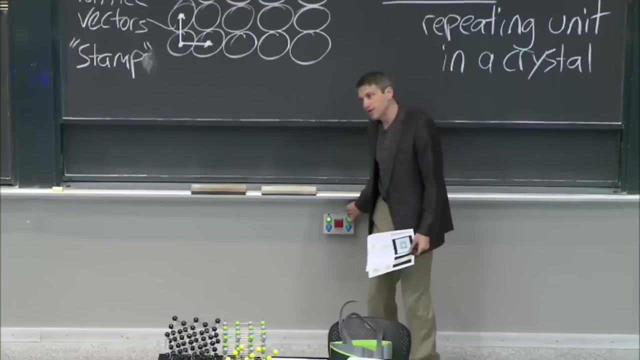 Doesn't matter right now. It's a stamp that fills all of space. That is how we're building up our knowledge- Knowledge of crystals. OK, Well, you can also ask the question which is: how much could you fill in there? 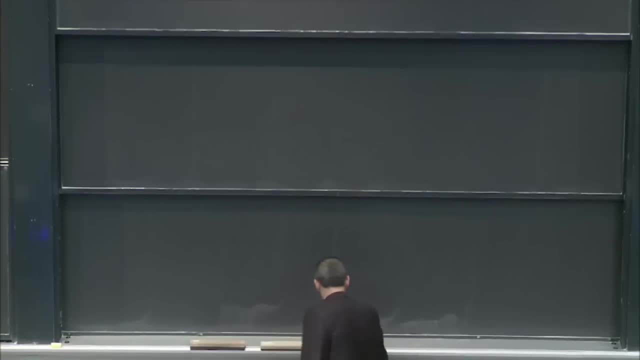 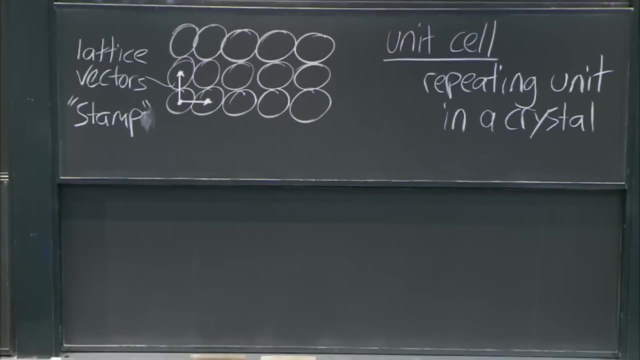 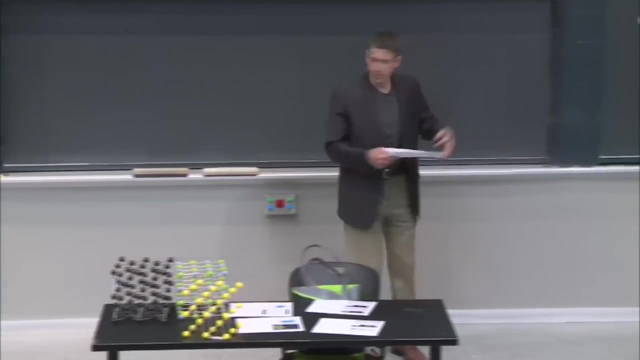 And that's a very important question that we want to know. OK, OK now. so I've got my lattice vectors, But I want to know now, what am I put? Because I could put there, I could you know. look at this. 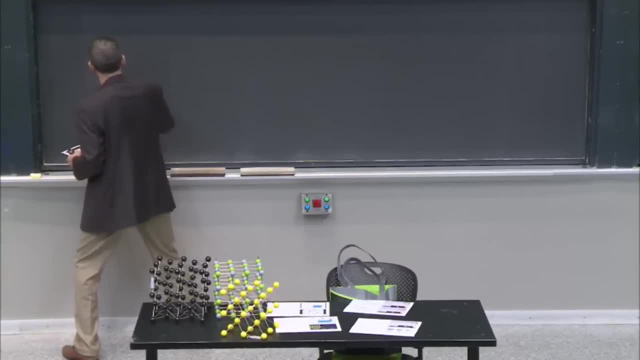 I'm going to take a lattice vector like this. This is a square lattice. OK, if this is a square lattice, then those are the same length. right. A is like the length of the. this is like the length of the lattice vector. 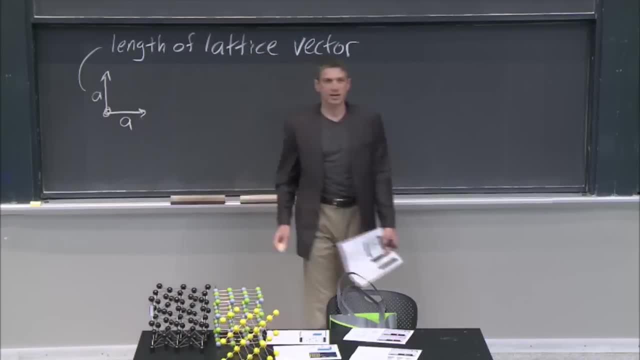 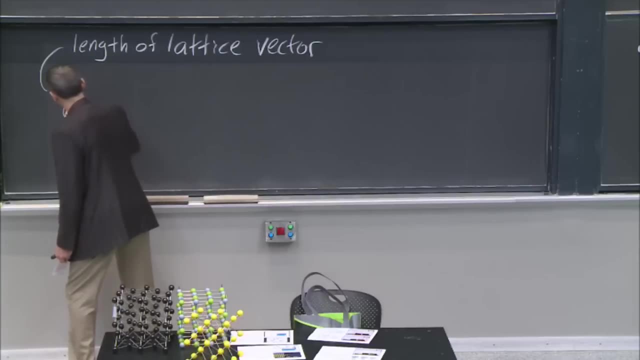 Now, if I took this lattice, this stamp, and I say, OK, now I'm going to decide what to put there. I'm going to put circles, OK, OK, Circle there, circle there, And what you do then is you put a circle everywhere. 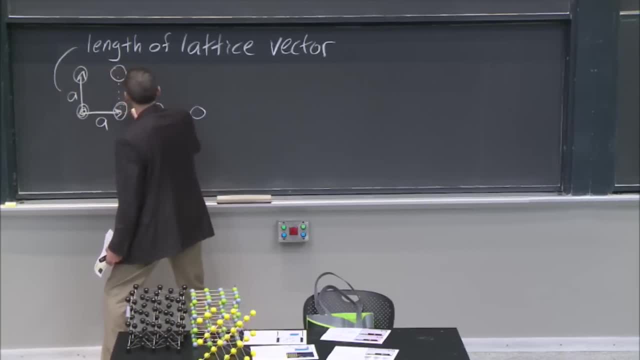 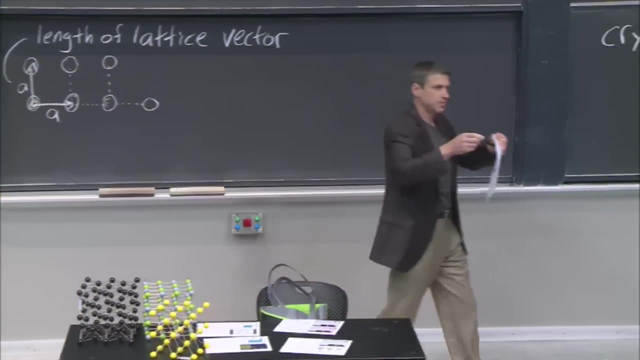 that you stamp, right, OK, So I have now. I've now taken my stamp And I've stamped everywhere And I've put something at each place- a circle. But I might ask a question, And this is a very important question, which? 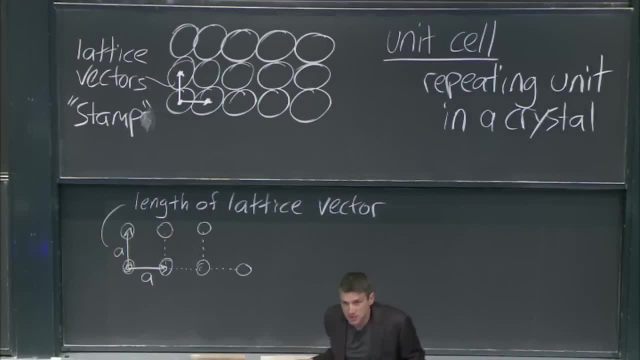 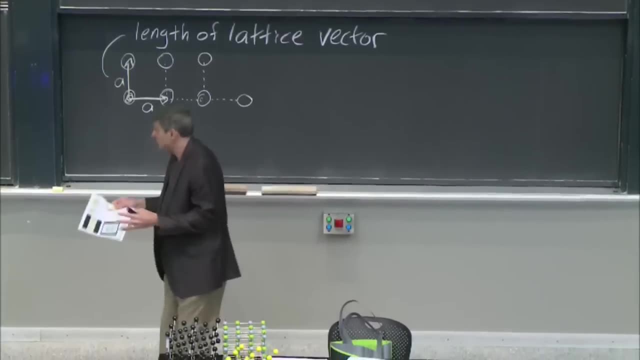 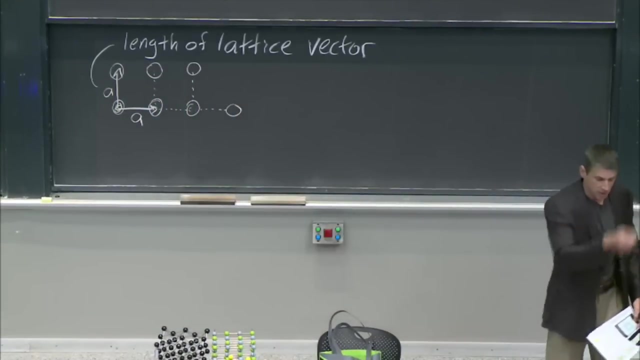 is: what is the maximum? if I have circles, what is the maximum that they can pack in for this lattice? How much can I pack the? well, you can just visualize that. now Let's grow them. A stamp means it's the same thing everywhere, right? 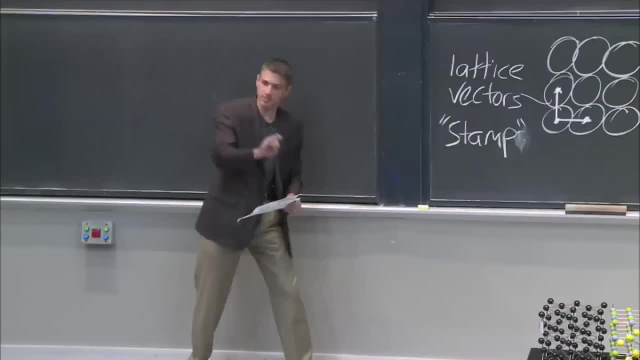 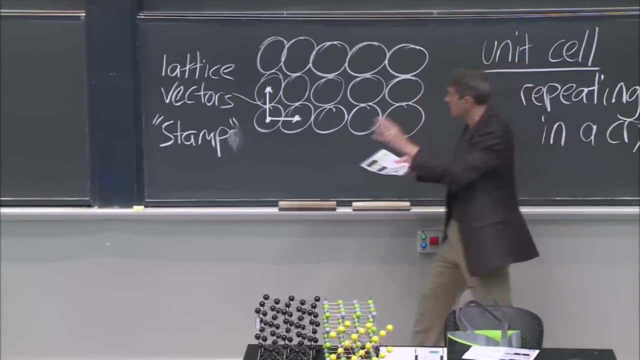 It is a stamp And no voids. These vectors are my stamp. Now I'm stamping all of space. I didn't really say what I'm putting there. I mean here there's cannonballs, In Escher there's ducks. 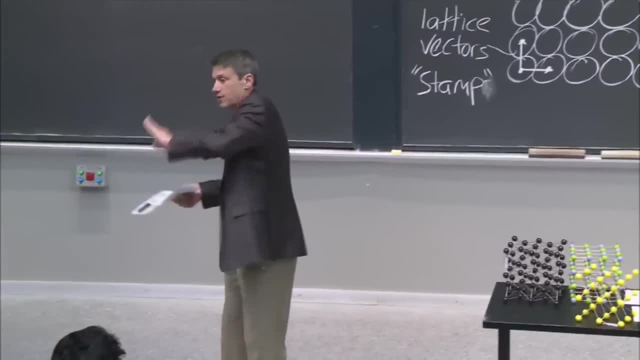 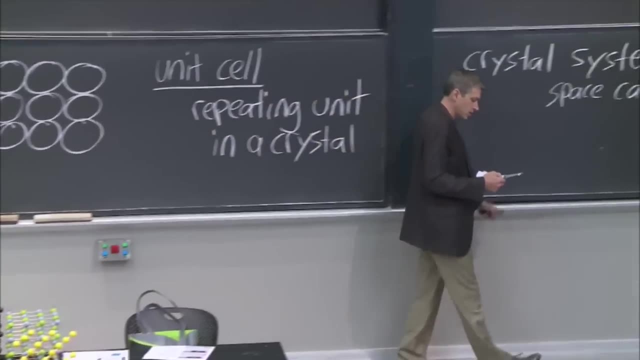 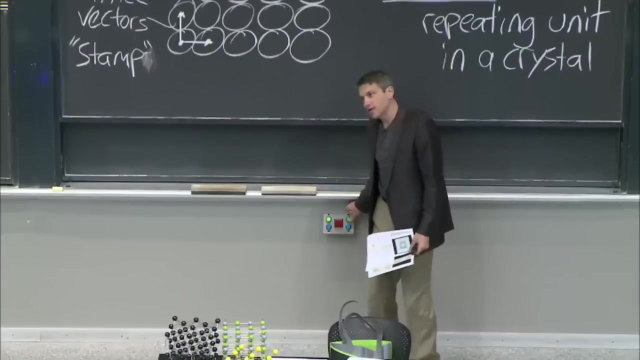 Doesn't matter right now. right, It's a stamp that fills all of space. That is how it works. That's how we're building up our knowledge of crystals. OK, Well, you can also ask the question, which is: how much could you fill in there? 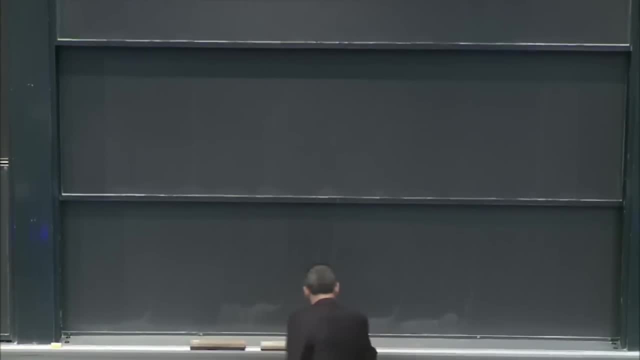 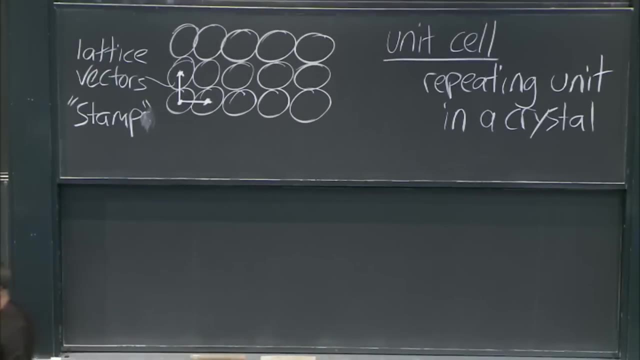 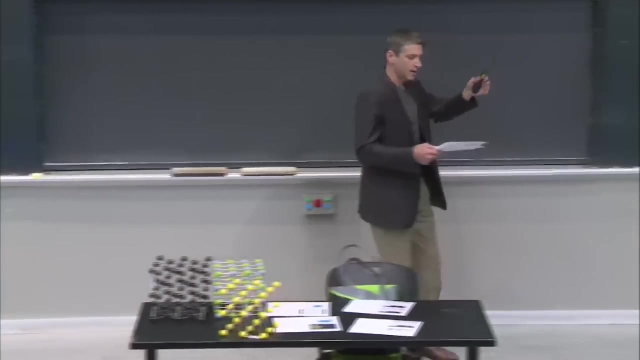 And that's a very important question that we want to know. OK now, so I've got my lattice vectors, But I want to know now, what am I put? Because I could put there, I could, you know. look at this. 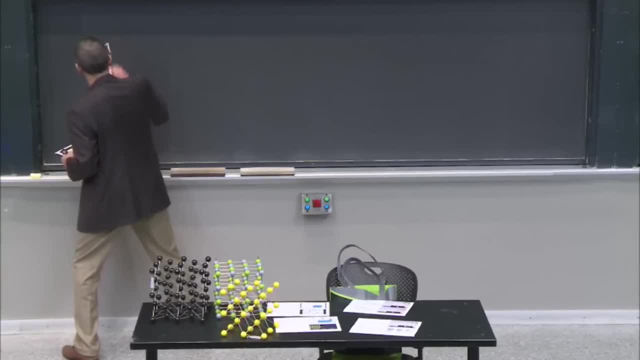 I could take a lattice vector like this that this is a square lattice. OK, if this is a square lattice, then those are the same length. right A is like the length of the. this is like the length of the lattice vector. 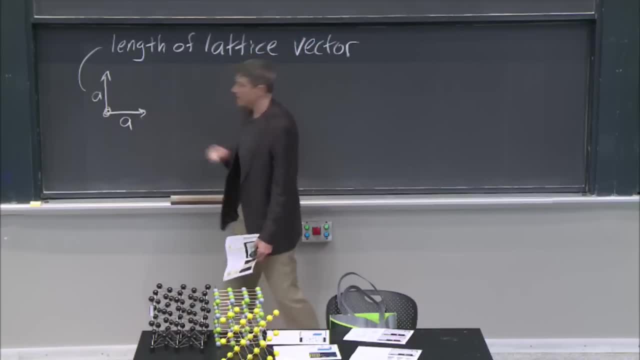 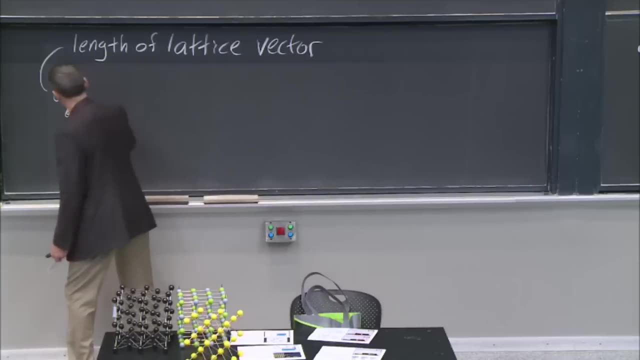 Now, if I took this lattice, this stamp, and I say, OK, now I'm going to decide what to put there. I'm going to put circles, OK, so I'm going to put a circle there, circle there, And what you do then is you put a circle everywhere. 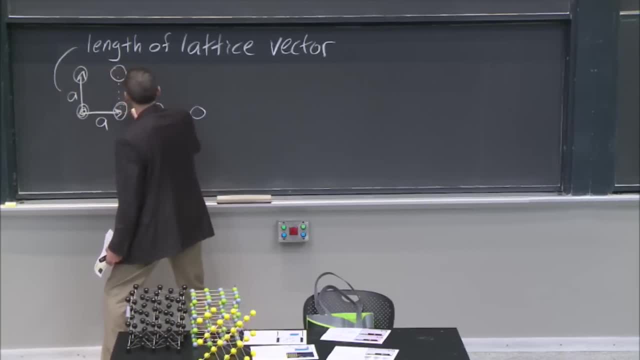 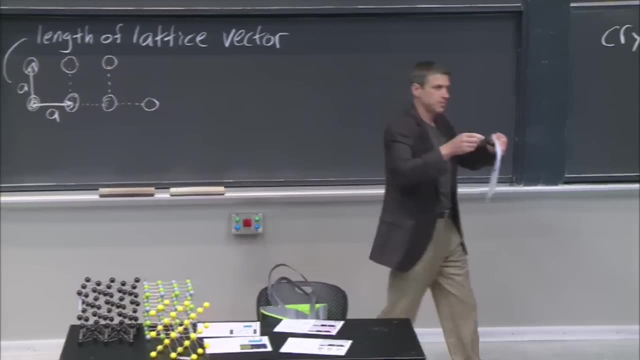 that you stamp, right, OK, so I have now. I've now taken my stamp and I've stamped everywhere And I've put something at each place- a circle. But I might ask a question, And this is a very important question, which is: 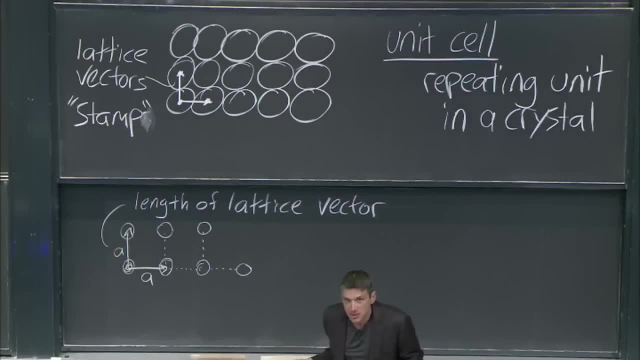 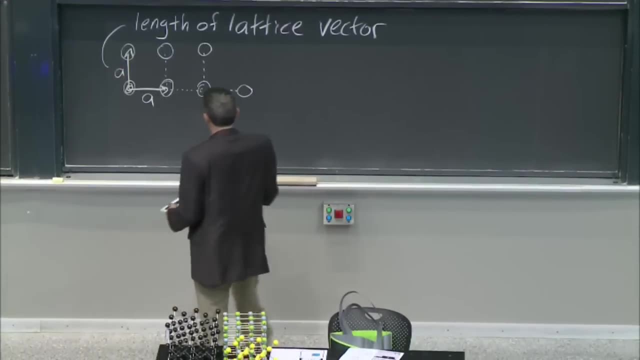 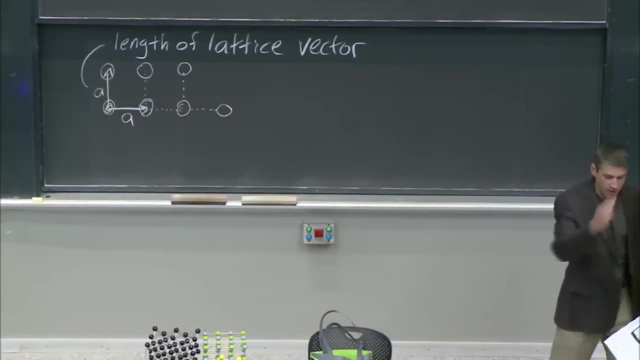 what is the maximum? if I have circles, What is the maximum that they can pack in for this lattice? How much can I pack the? well, you can just visualize that. Now let's grow them. A stamp means it's the same thing everywhere, right? 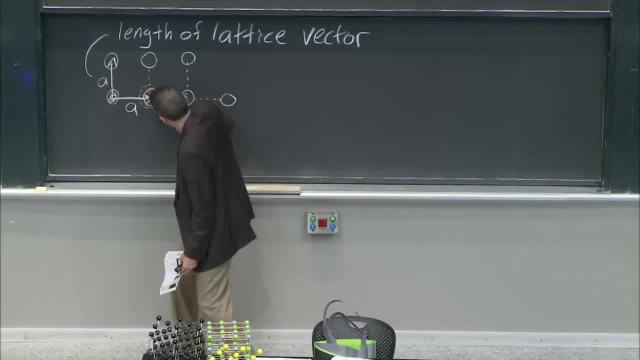 So now, if I make one of them bigger, well, I've made them all bigger, right, Because they're all the same everywhere, And if I make them all big enough, eventually they're going to touch like that. That's a special thing. 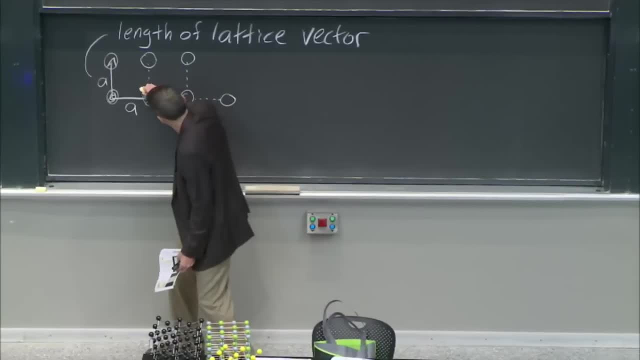 So now if I make one of them bigger, well, I've made them all bigger, right, Because they're all the same everywhere, And if I make them all big enough, eventually they're going to touch like that. That's a special thing, because now I've 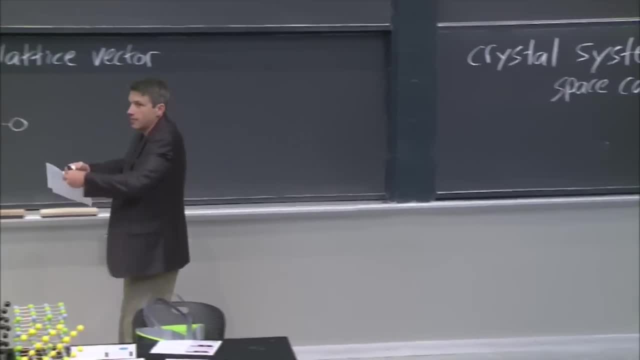 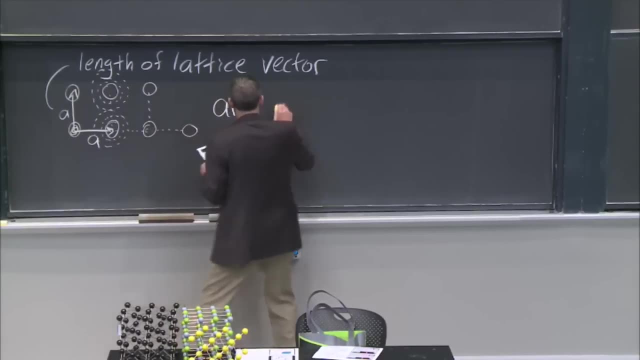 grown the shape that I'm putting there, OK, OK, To the point where it's the maximum packing right, And so you can imagine this. The area of maximum packing is a very important parameter, And it's something that we'll talk about today. 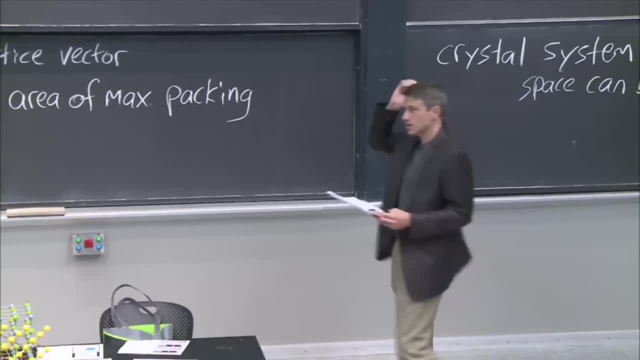 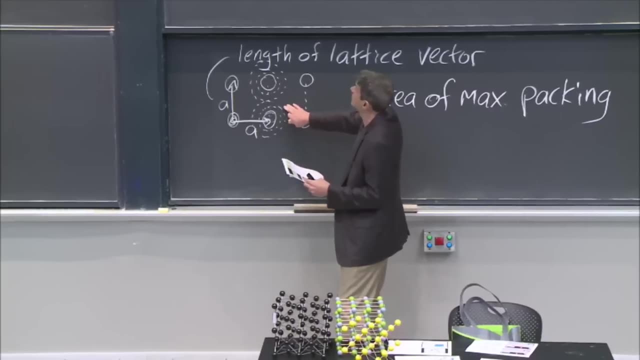 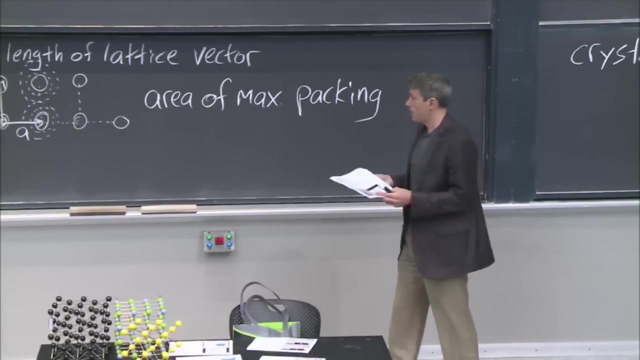 with 3D crystals, which is the solids of elements in the periodic table. But if you stay with this square analogy, so my lattice is a square, My stamp is a square, My sides are equivalent And what I put there is a circle. 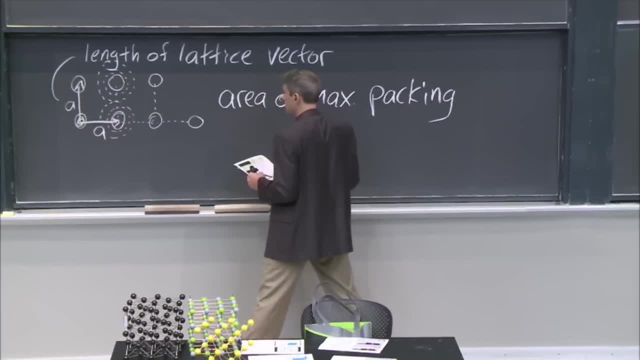 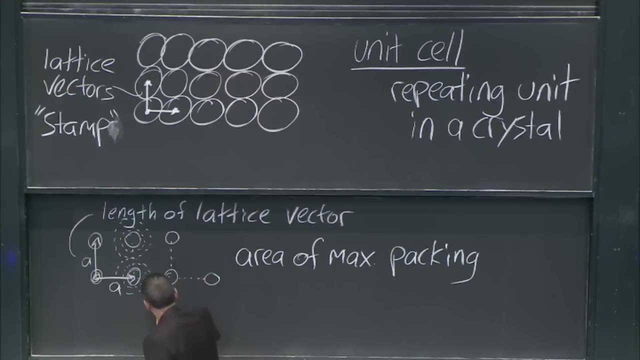 Then the area of maximum packing is something you can calculate right, Because the circle itself, in this case, if I look at it, then oh, that's not a good circle. But anyway, you'll get the point here, which is that, oh boy. 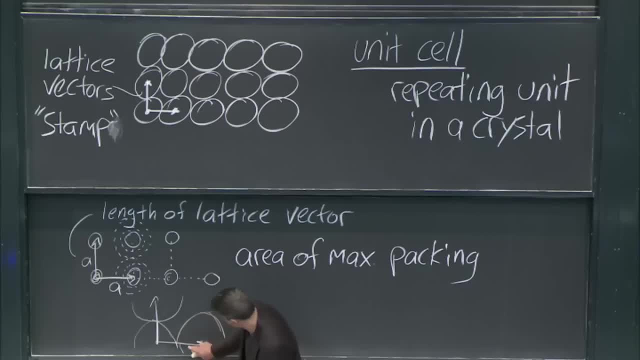 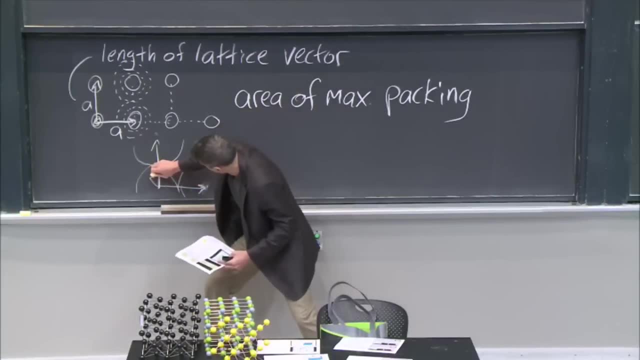 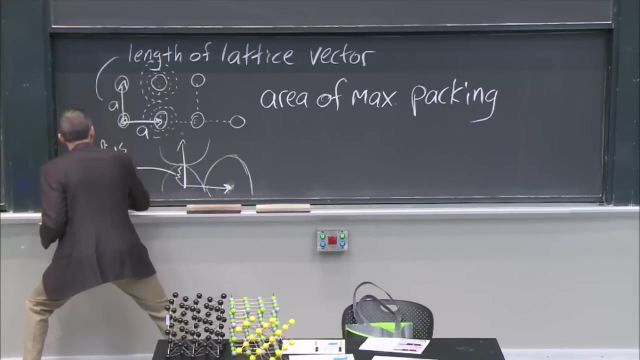 Which is that you know if this is the lattice vector, is a a right, like I drew there and I'm looking at the maximum packing, then you know already that the radius of the circle is a half a, So radius equals 1 half a right. 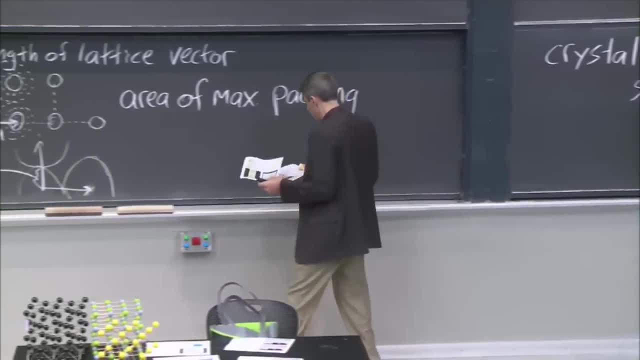 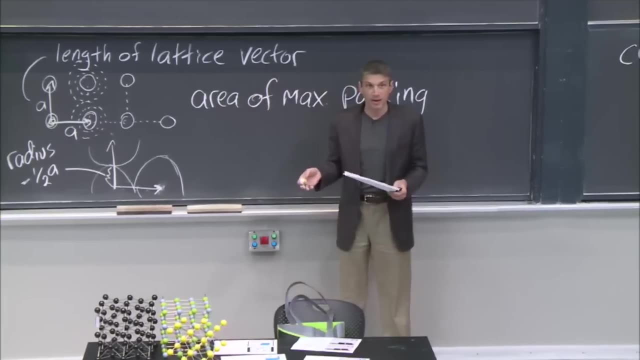 I mean, if the radius of the circle is a half a, OK, if the radius of a circle is a half a, then you also know what the area is. I'm in 2D right now. I'm in 2D. 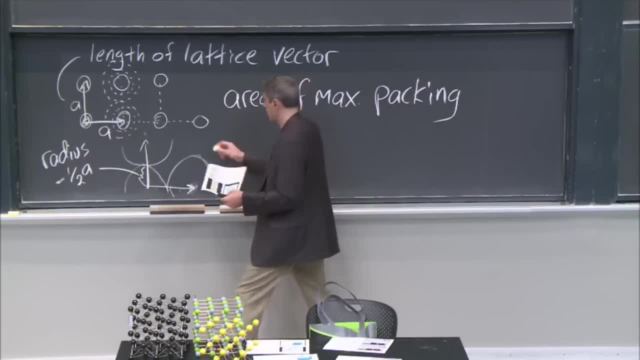 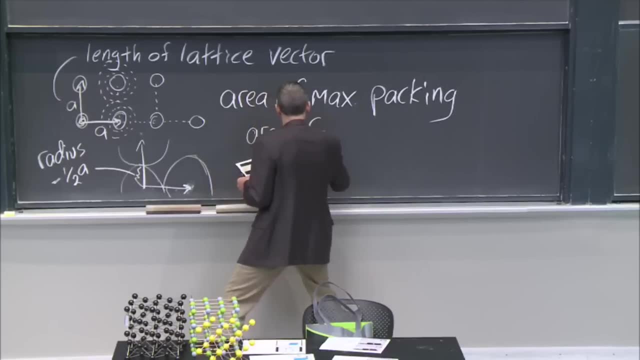 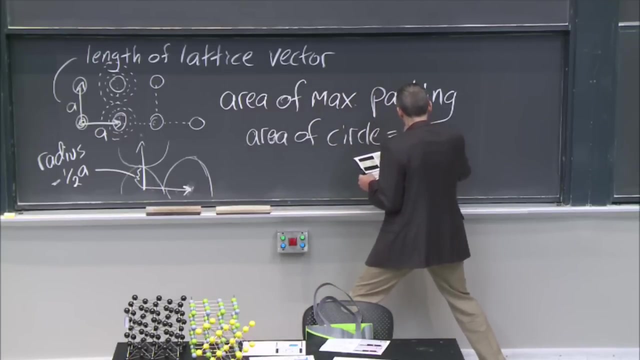 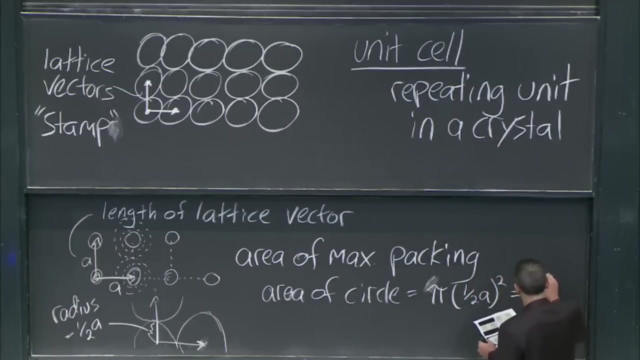 So if I've maximized the packing of these circles on the square lattice, then the area, then the area area of the circle is 1 half. that's a pi times r squared. So 1 half a squared equals all right pi a squared. 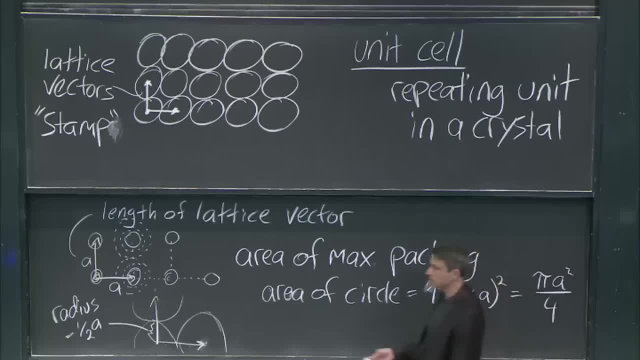 All right, Pi squared over 4.. But see, I also know how much I packed it in, right? I'm doing this slowly on purpose, because we'll go faster when we do some of the other ones, But I want to do the first one slow. 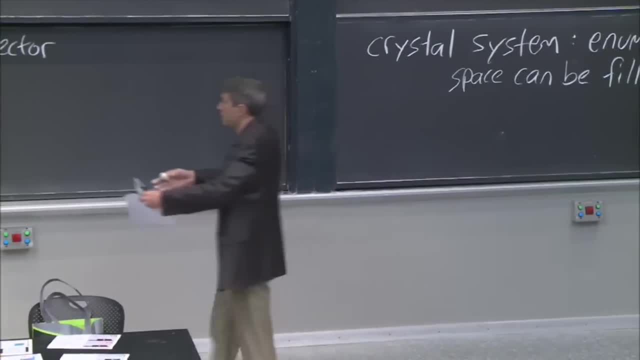 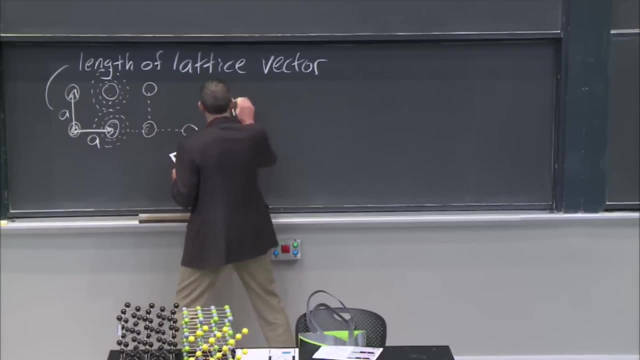 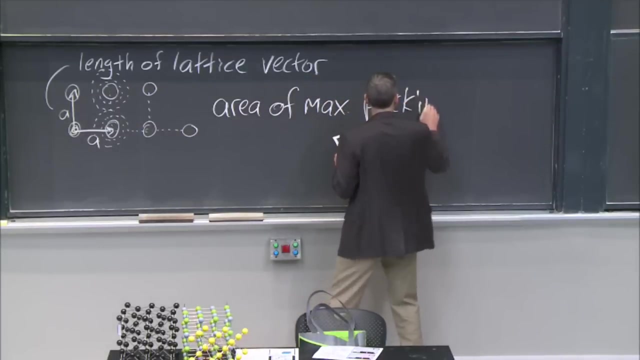 Because now I've grown the shape that I'm putting there to the point where it's the maximum packing right, And so you can imagine this. The area of maximum packing is a very important parameter, And it's something that we'll talk about today. 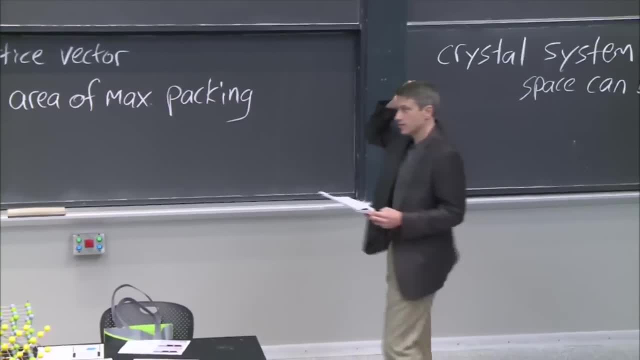 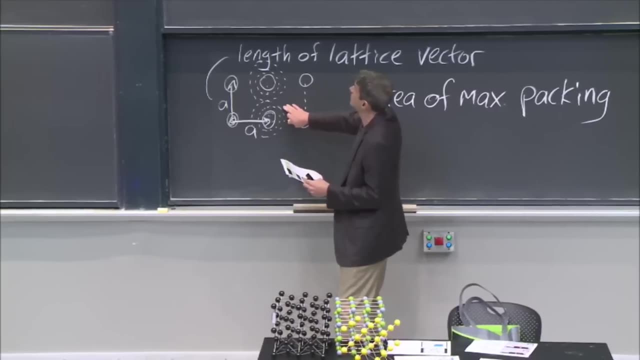 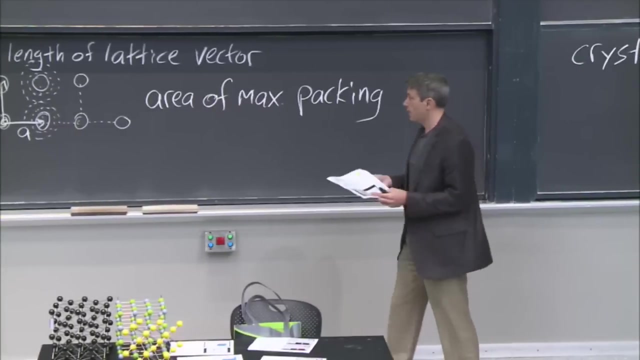 with 3D crystals, which is the solids of elements in the periodic table. But if you stay with this square analogy, you can see that the area of maximum packing is the area of maximum packing. So my lattice is a square, My stamp is a square. 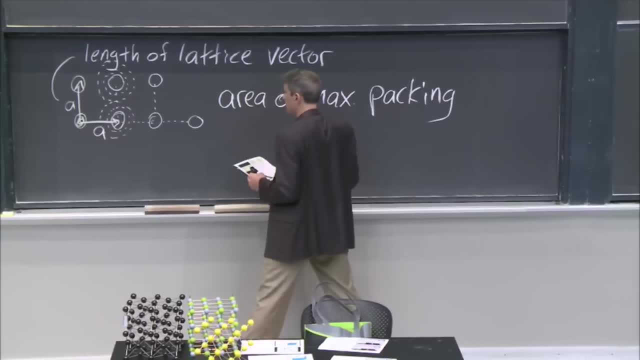 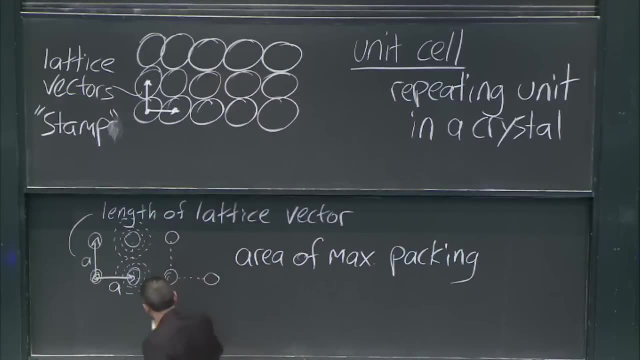 My sides are equivalent And what I put there is a circle, Then the area of maximum packing is something you can calculate right, Because the circle itself, in this case, if I, because it's in tight, if I look at it, then oh, 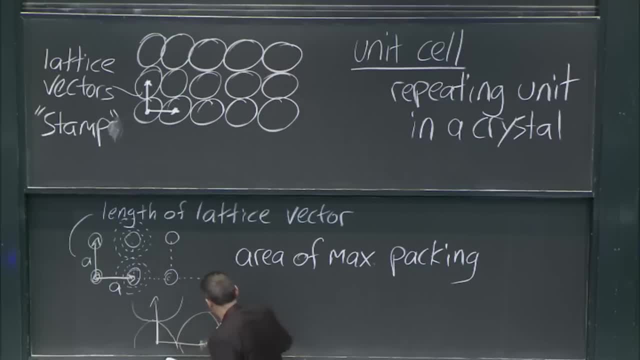 that's not a good circle, But anyway, You'll get the point here. You'll get the point here, which is that you know, if this is the lattice vector, is a a right, like I drew there, and I'm looking at the maximum packing. 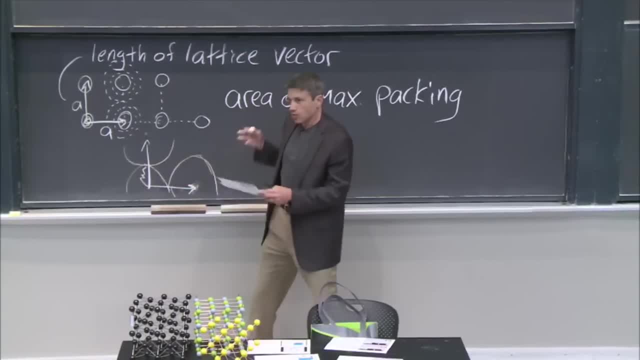 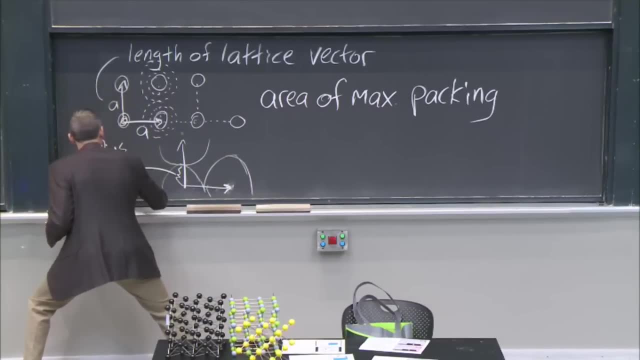 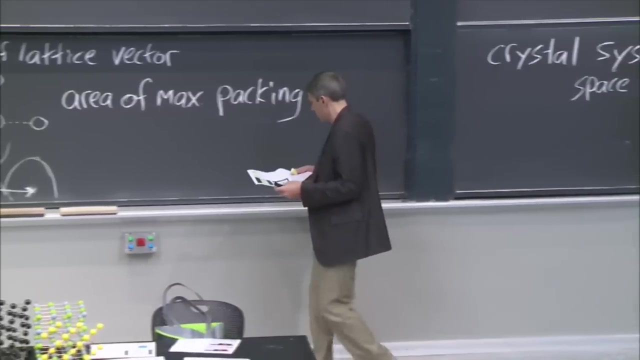 then you know already that the radius of the circle is a half a. So radius equals 1, half a right, I mean, if the radius of the circle is a half a, OK, if the radius of a circle is a half a. 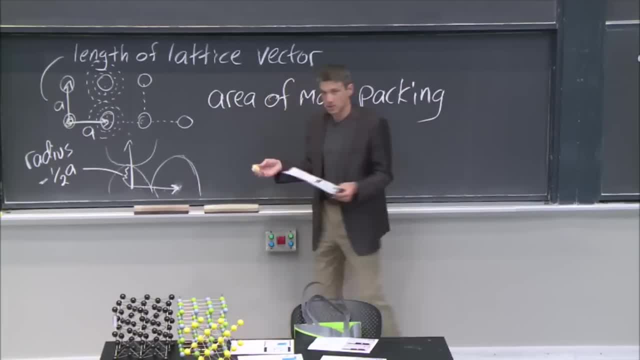 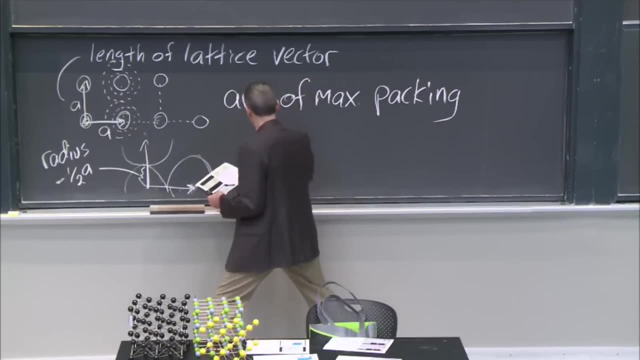 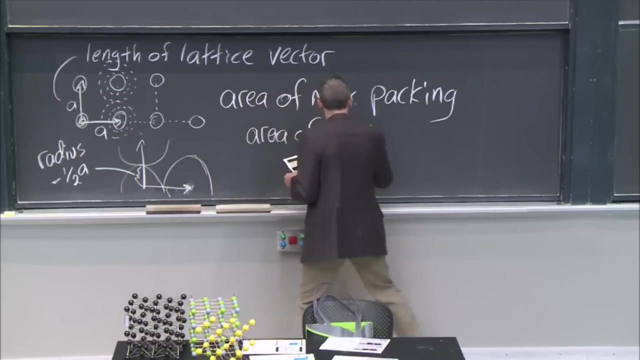 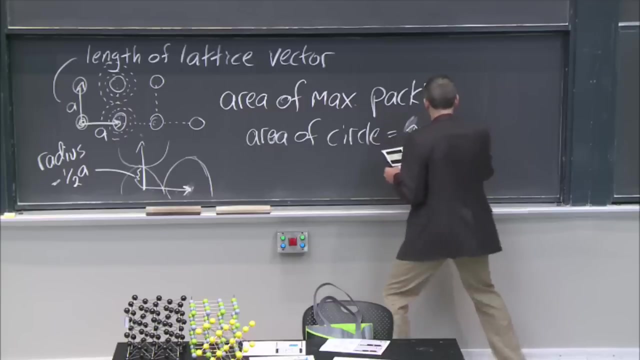 then you also know what the area is. I'm in 2D right now. I'm in 2D. So if I've maximized the packing of these circles on the square lattice, then the area, then the area, area of the circle, is 1: half. that's a pi times r squared. 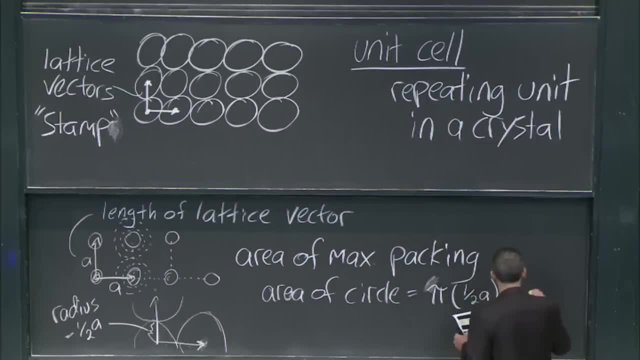 So 1 half a squared equals All right, Pi a squared over 4.. But see, I also know how much I packed it in, right? I'm doing this slowly on purpose, because we'll go faster when we do some of the other ones. 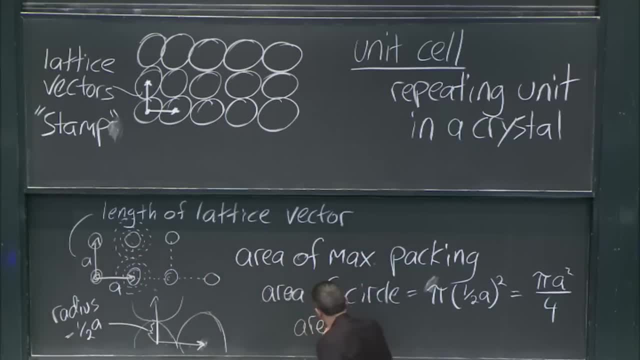 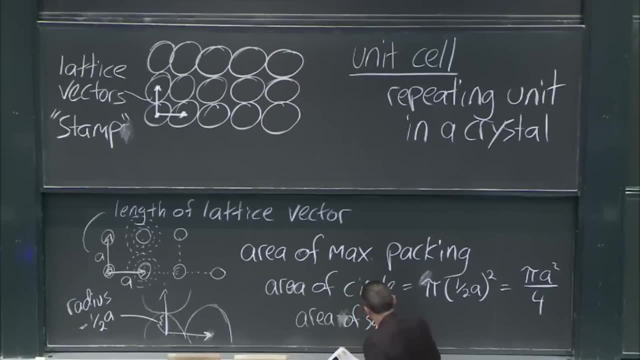 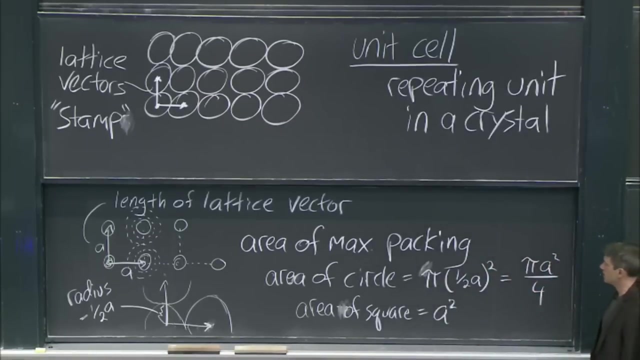 But I want to do the first one slow, because then we'll all be able to see what we're talking about. with the simplest case, The area of the square is a squared right, And so the pack- The area of max packing- is equal to OK. 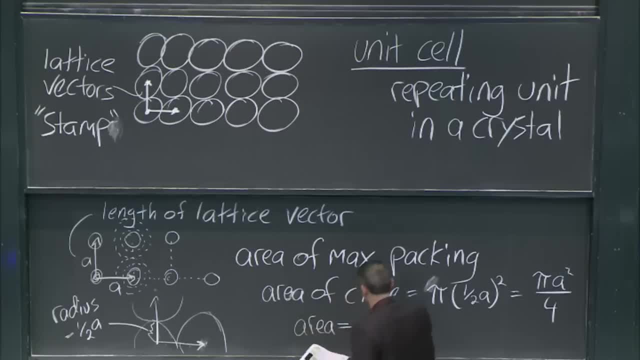 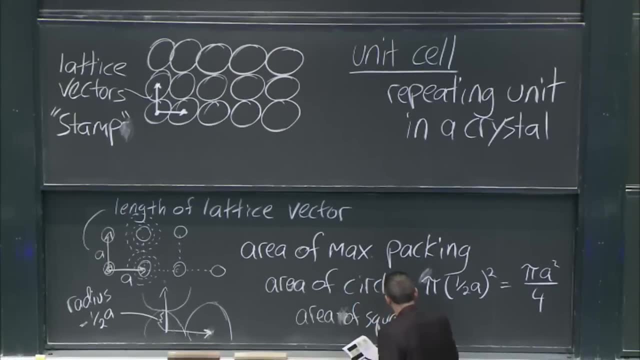 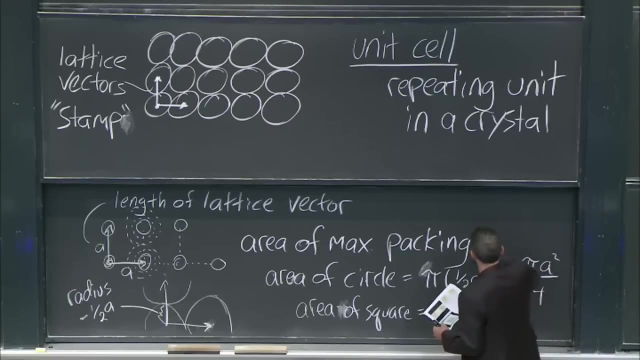 because then we'll all be able to see what we're talking about. with the simplest case, The area of the square is a squared right, And so the packing, the area of max packing, is equal to OK pi a squared over 4, over a squared. 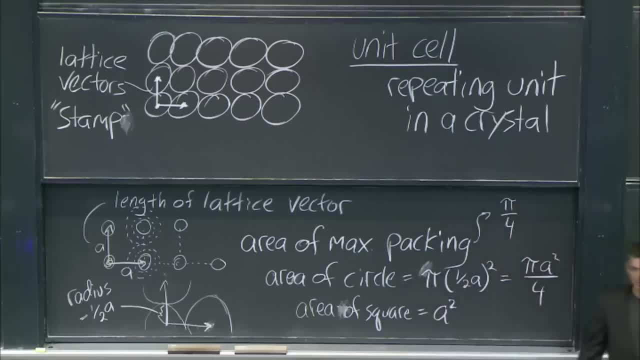 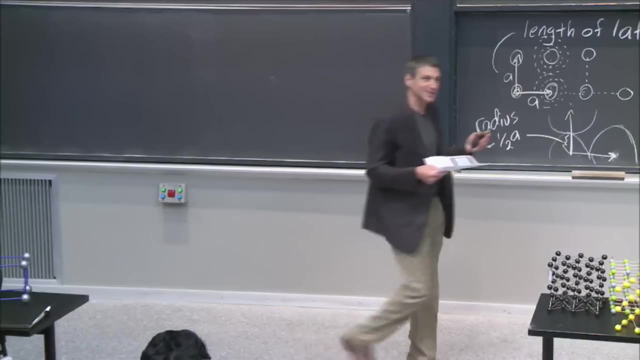 Pi over 4,. all right, because the a squareds cancel. All right, So it's 78%. This is what hook was in, But did I max it out or could I do something different? Could I pick a different lattice? 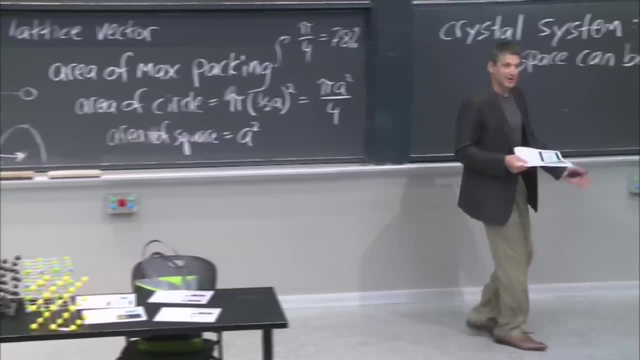 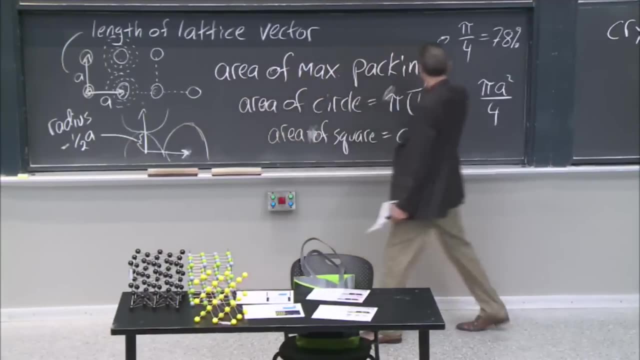 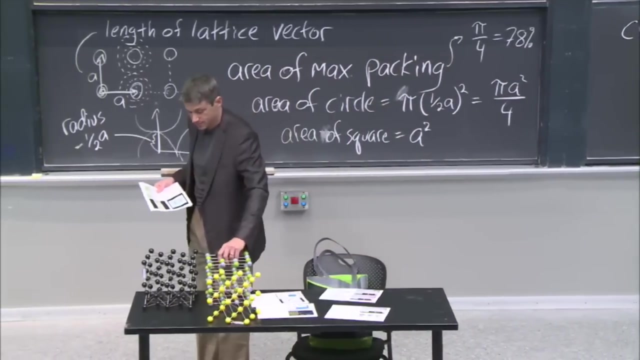 What if we made cancel? What if we made cannonballs into rectangles? Bad idea, No, he's stuck with spheres. But how do you pack them in? How can you arrange them in a way to change the max packing? That's what nature does with atoms, as we'll see. 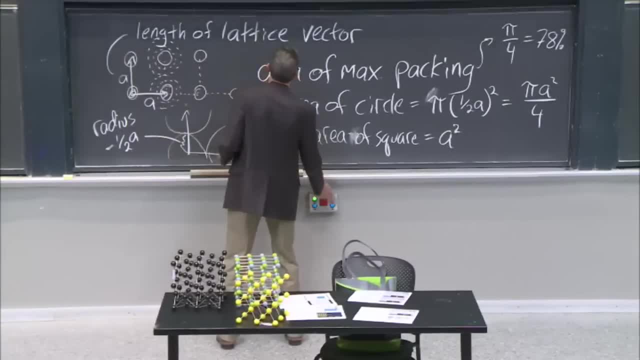 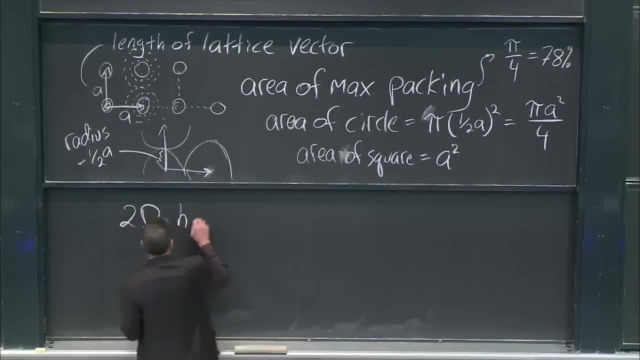 So, for example, if I had a 2D hexagonal lattice instead of my stamp being a square, so if it were a 2D hexagonal lattice, If I had a hexagonal lattice, I won't do this one out. 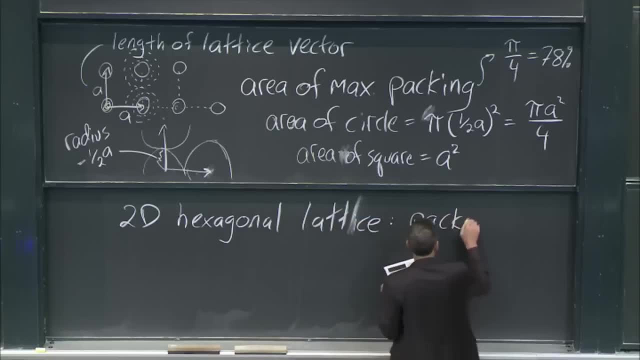 But then the packing, the max packing, goes all the way up to 91, 91%. That's a lot more per area, max packing, max packing, right. So this is something that we care a lot about. It's something that we care about because I mean, this is: 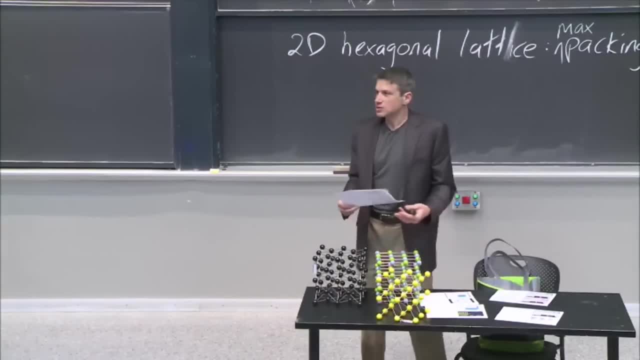 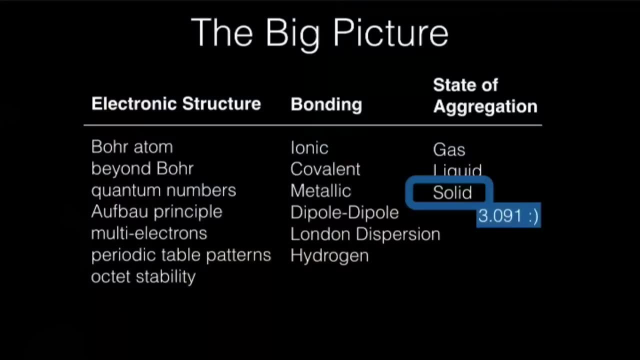 you know, when atoms see each other in a solid, what's the first thing they want to determine? The first thing they want to do is: they want to go back in here and they want to be like. which one of those can we do? 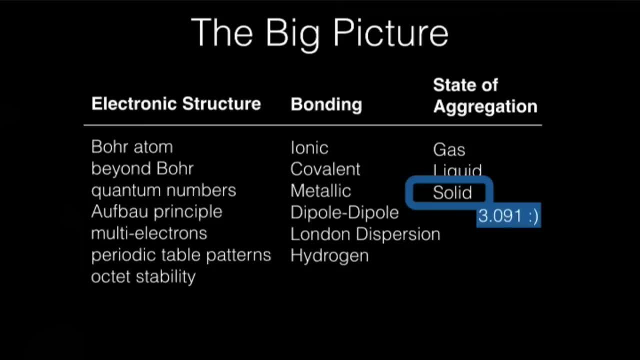 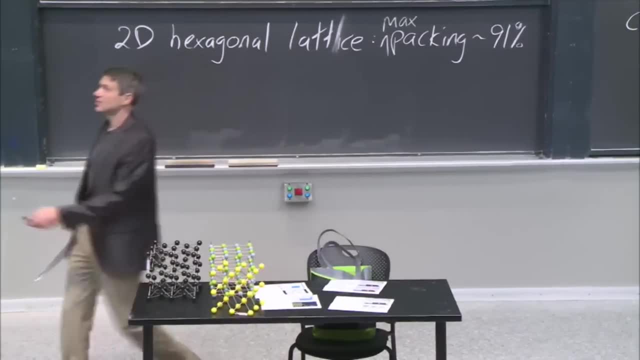 Can we find some way to bond? That's what atoms do, That's what everyone does. How can we bond together? What kind of relationship are we going to have? But they can't do that. They want to max that out, right. 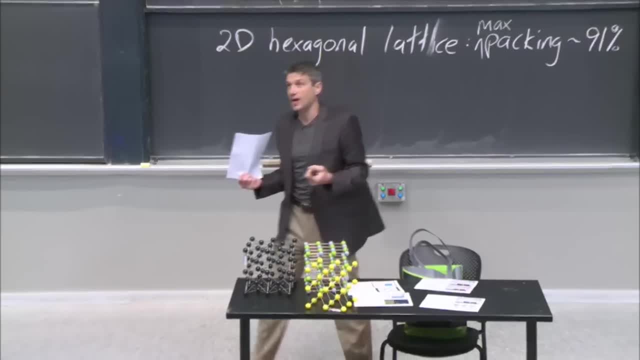 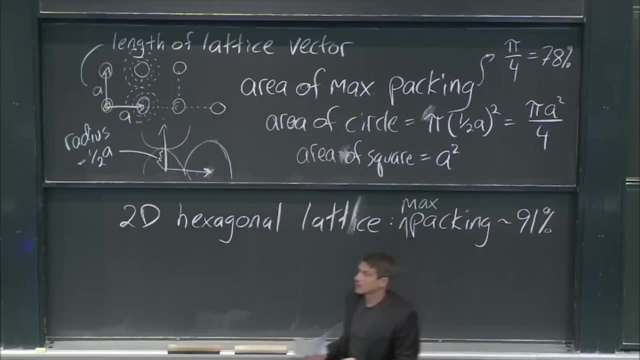 And so they want to try to pack. They want to pack in, given the bond that they're going to have, And that is what's going to dictate the kind of arrangement they can have in the crystal. OK, So, OK. So, here we are. 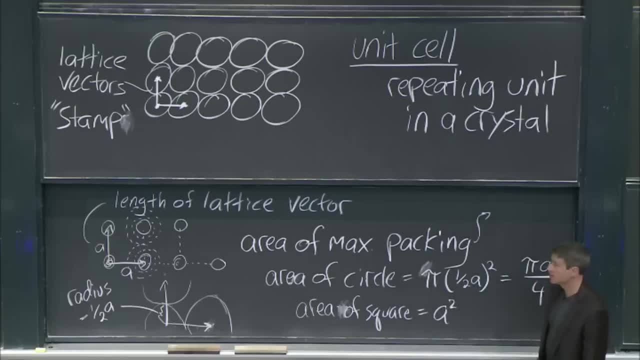 pi a squared over 4 over a squared Pi over 4, right, Because the a squareds cancel. So it's 78%. This is what hook was in, But did I max it out or could I do something different? 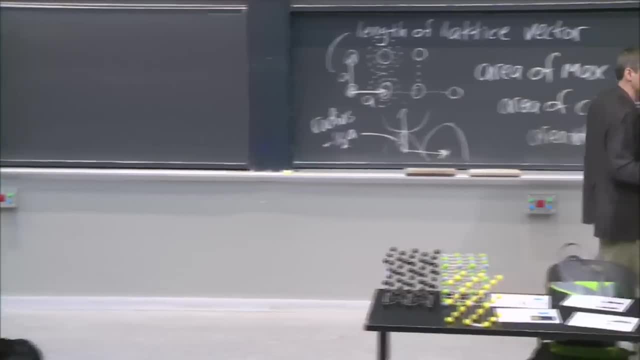 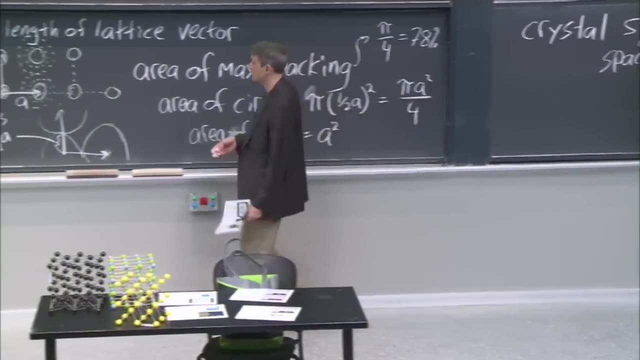 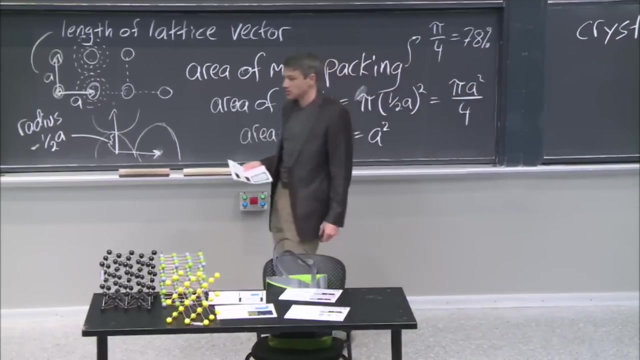 Could I pick a different lattice? What if we made cannonballs into rectangles? Bad idea, No, he's stuck with spheres. But how do you pack them in? How can you arrange them in a way to change the max packing? That's what nature does with atoms, as we'll see. 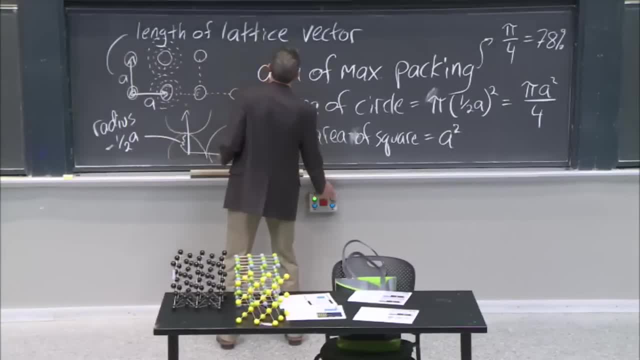 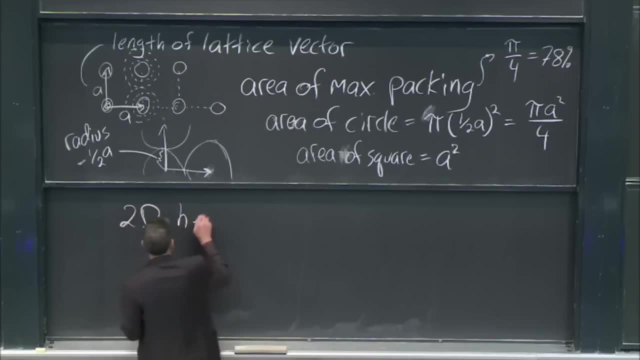 So, for example, if I had a 2D hexagonal lattice instead of my stamp being a square, So if it were a 2D hexagonal, hexagonal lattice, I won't do this one out. But then the packing, the max packing. 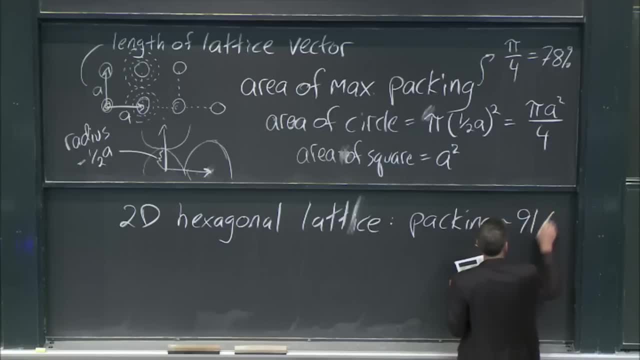 goes all the way up to 91, 91%. That's a lot more per area, max packing, max packing right. So this is something that we care a lot about. It's something that we care about because I mean: 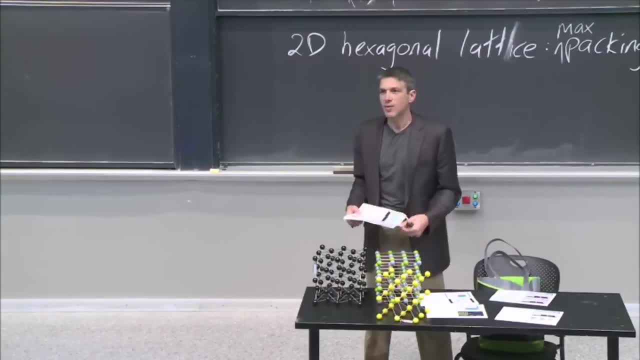 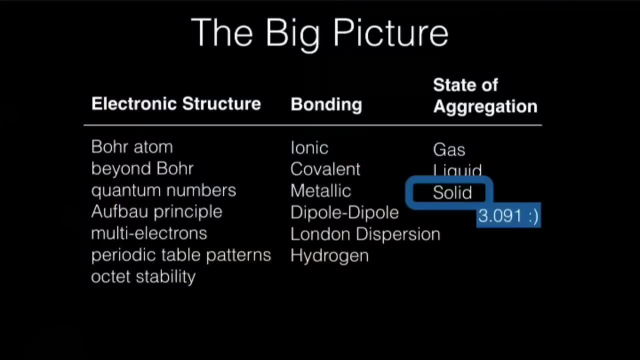 when atoms see each other in a solid, what's the first thing they want to determine? The first thing they want to do is: they want to go back in here and they want to be like. which one of those can we do? Can we find some way to bond? 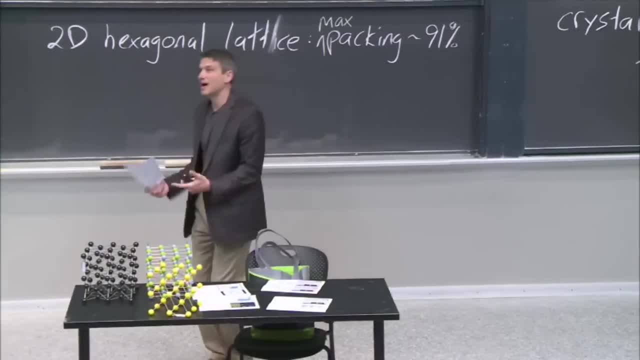 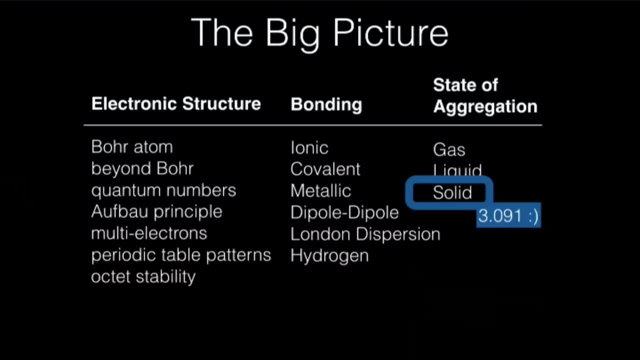 That's what atoms do, That's what everyone does. How can we bond together? What kind of relationship are we going to have? But They can't do that. They want to max that out right, And so they want to try to pack in. 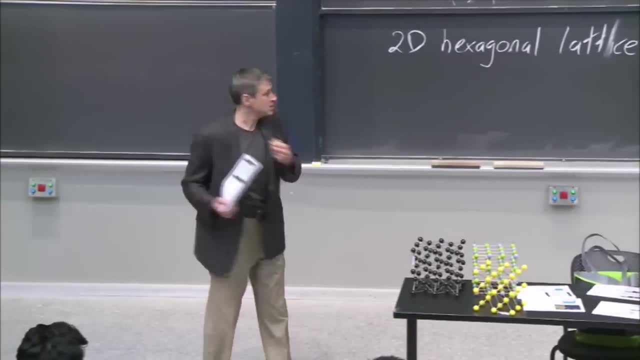 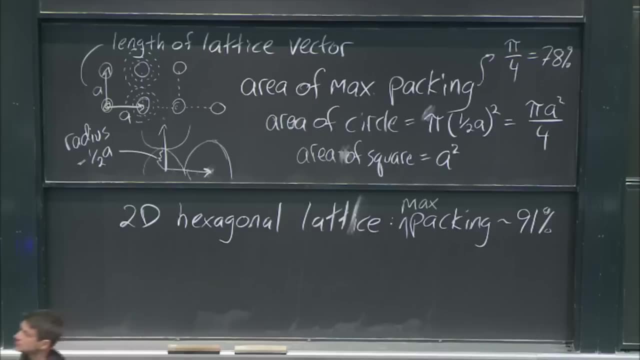 given the bond that they're going to have, And that is what's going to dictate the kind of arrangement they can have in the crystal. OK, So, OK. So, here we are, and we're going from 2D to 3D. 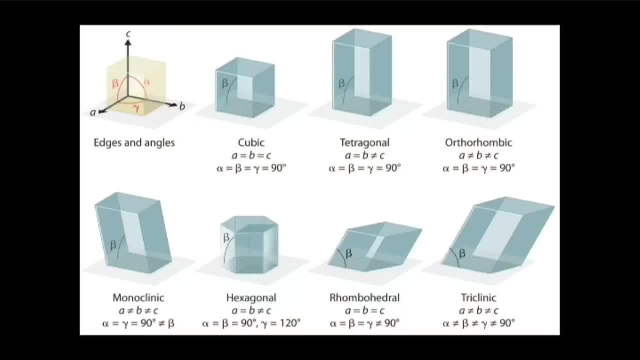 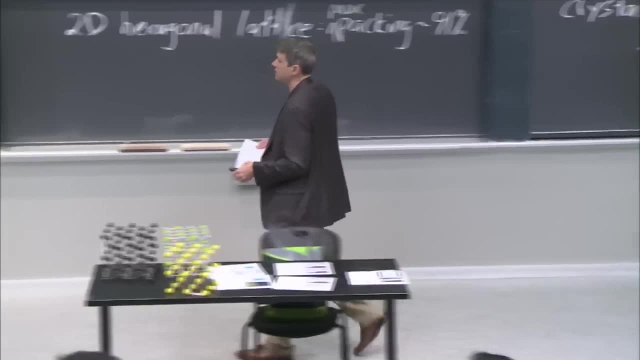 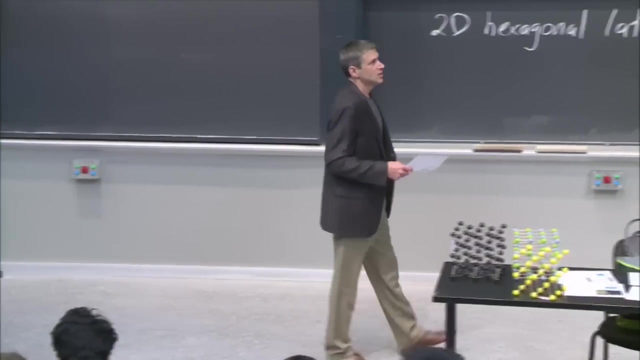 And we're going from 2D to 3D. Now the thing is, we will not, do you know, this is not going to be an in-depth dive into symmetry and space groups and group theory. Those are all great topics. 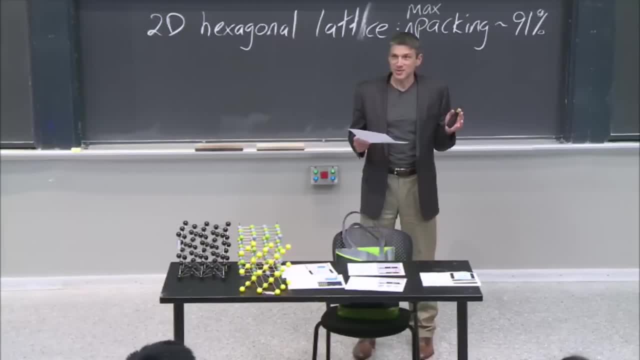 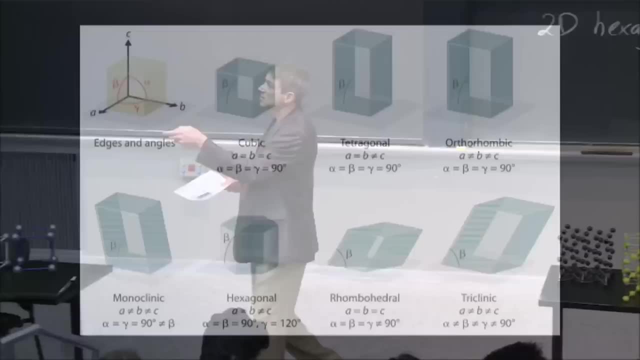 But I'm just going to tell you- and it's actually kind of cool, In 3D there are only seven unique crystal systems. There are only seven ways that you can do this. You can only pack in and have no voids and have no voids. 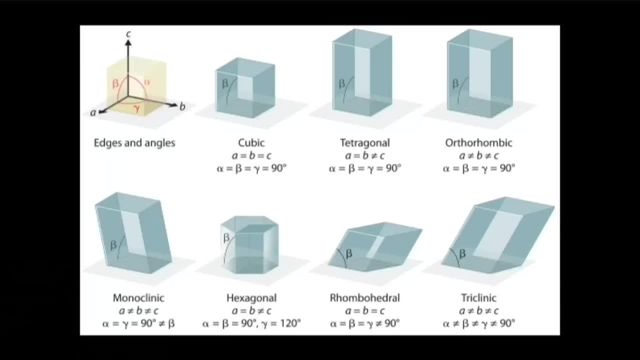 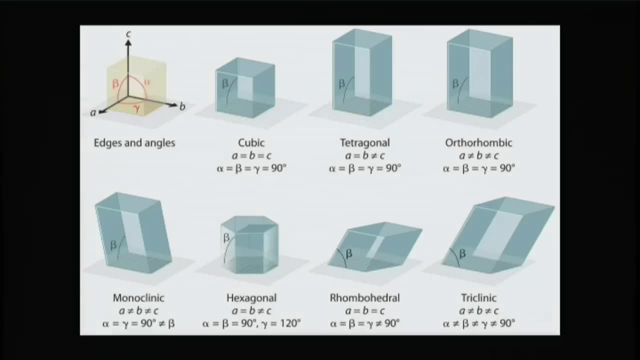 You can only pack in these seven different systems where, as you can see, what's changing here? Well, it's Cartesian coordinates. So you've got the length of each lattice vector and their relative angles. All right, That's all you're changing. 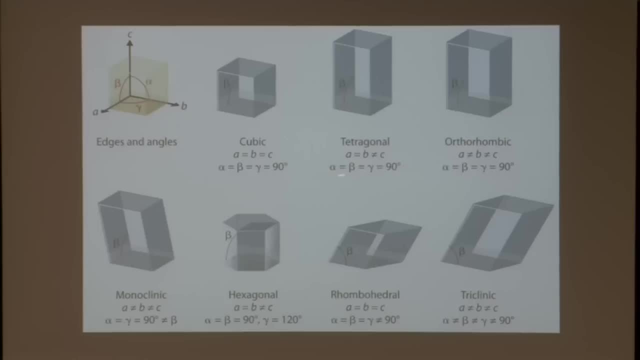 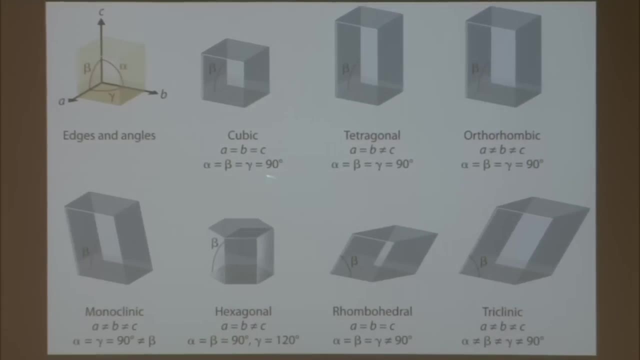 Well, you know, sometimes you change all the angles at once. OK, Sometimes you change only a few. Well, sometimes you change only a few of them, Sometimes you make them all the same, Sometimes you change a few, Sometimes you have all of them be even. 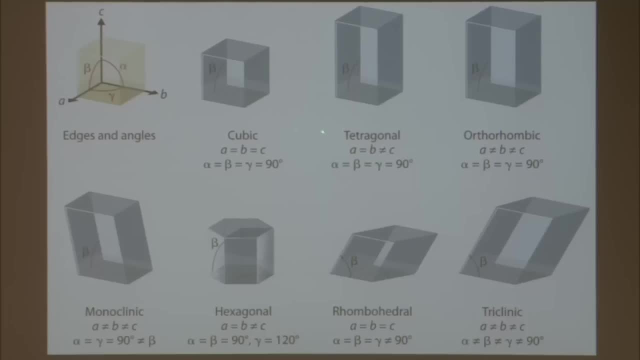 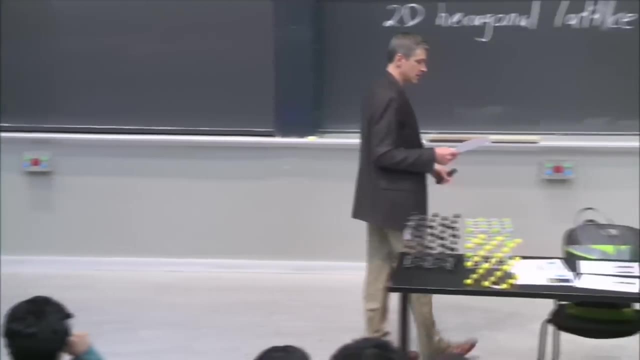 And sometimes some of them are equal. Some of the lattice lengths are equal, but another one is different. These are the seven ways that we can fill all of space, And there are only seven In this class. we're only going to focus on one. 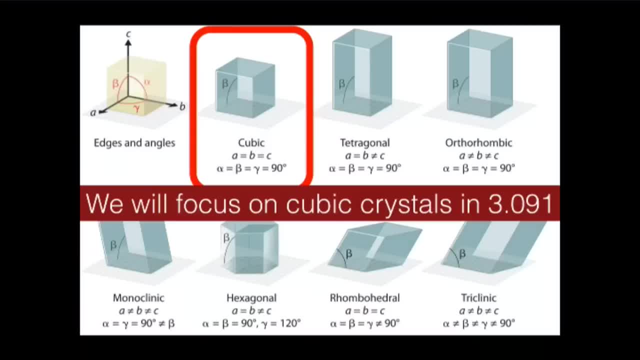 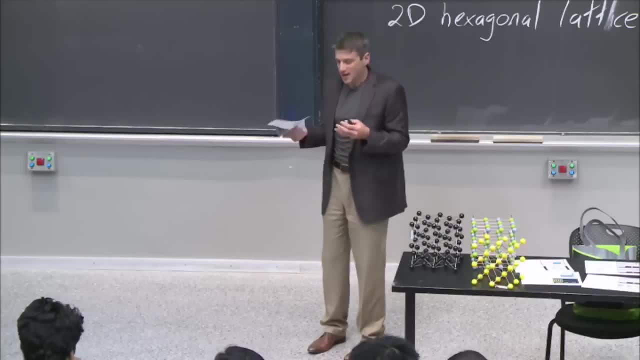 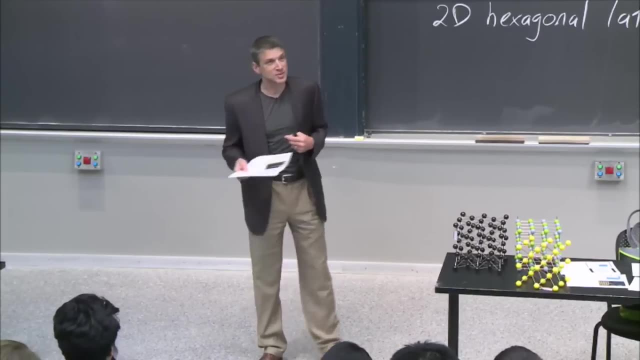 and that's the cubic system, And the reason is that this gives us plenty to work with to understand crystallography and how chemistry relates to crystallography, And there's the benefit of the fact that a lot of elements. take one of these three. 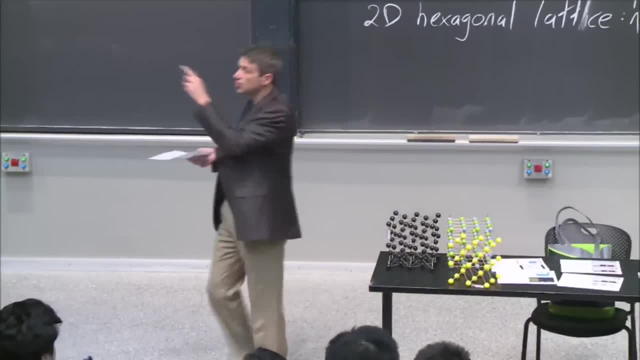 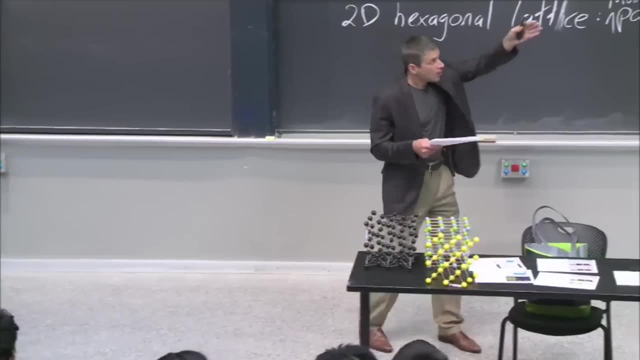 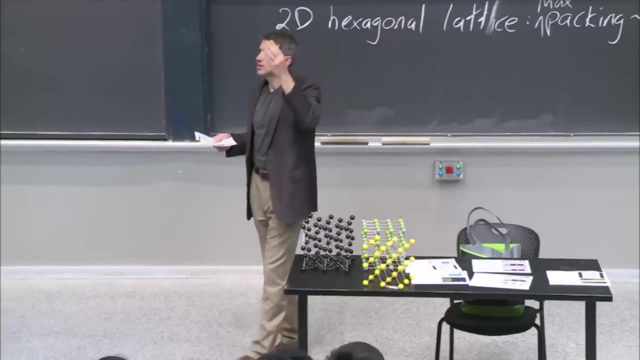 Actually only two, But they take cubic symmetry. What does that mean? Well, it means It means that all the lattice vectors are the same. Each one has a length, a. They're orthogonal to each other, which means that the angle is 90 degrees. 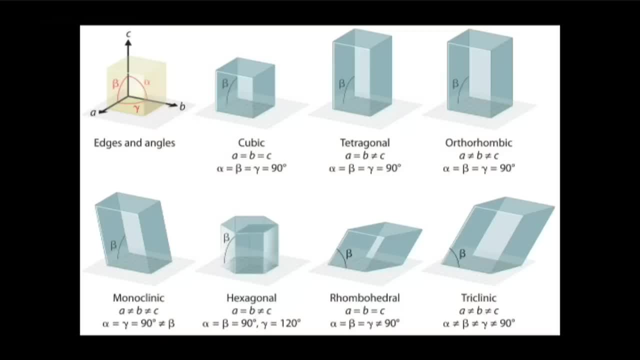 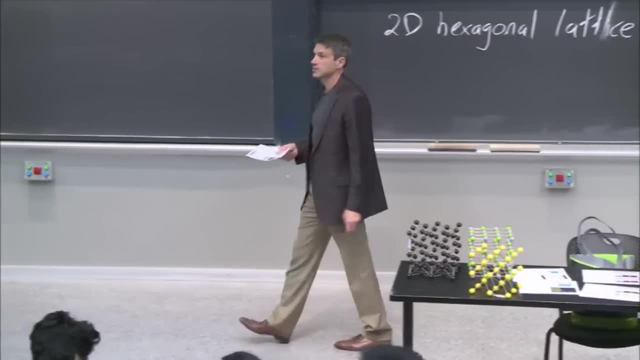 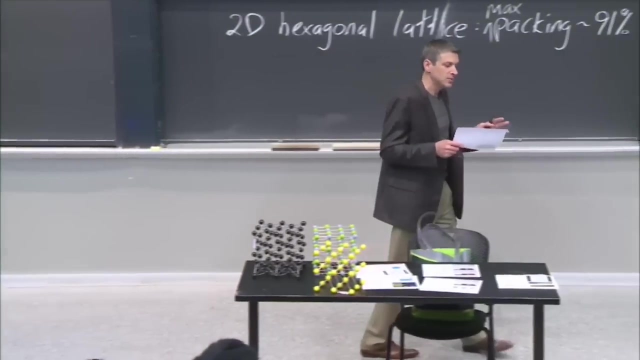 Now the thing is we will not do. you know, this is not going to be an in-depth dive into symmetry and space groups and group theory, Those are all great topics. But I'm just going to tell you, and it's actually kind of cool, 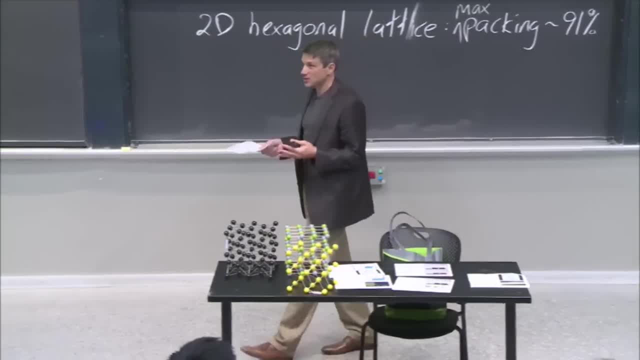 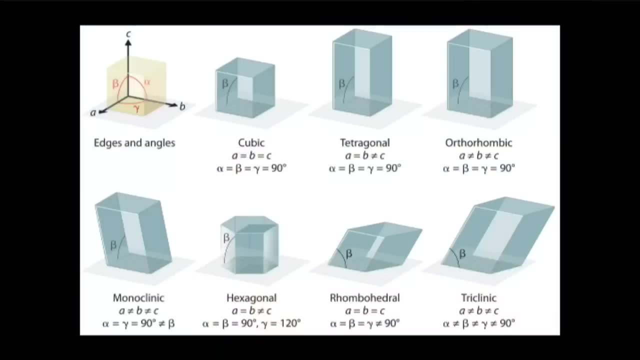 in 3D. there are only seven unique crystal systems. There are only seven ways that you can do this. You can only pack in and have no voids and have no voids. You can only pack in these seven different systems where. 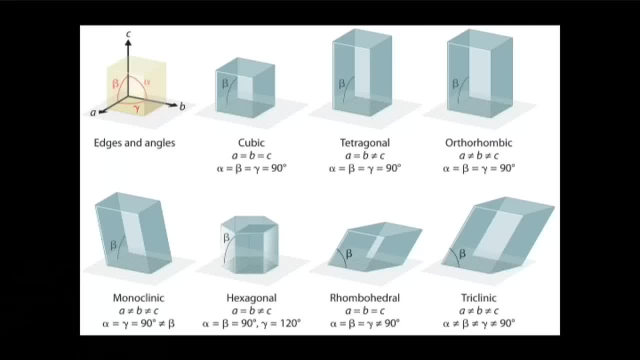 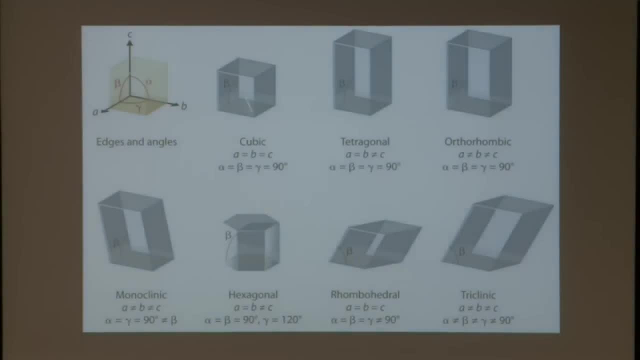 as you can see what's changing here. Well, it's Cartesian coordinates. so you've got the length of the crystal, the length of each lattice vector and their relative angles. That's all you're changing. Well, you know, sometimes you change all the angles at once. 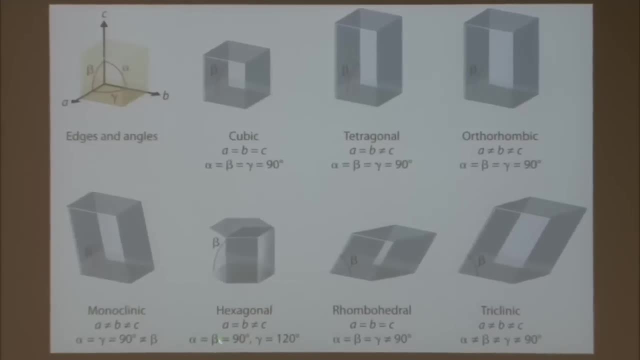 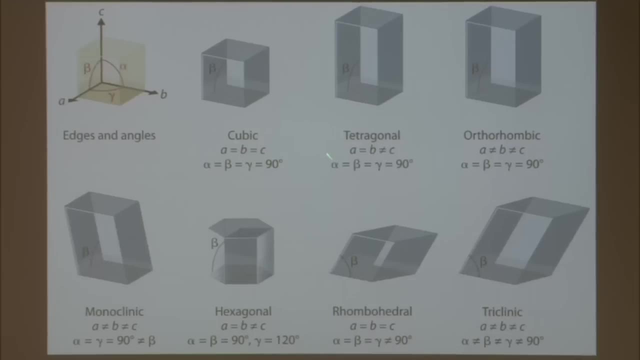 Sometimes you change only a few of them, Sometimes you make them all the same, Sometimes you change a few, Sometimes you have all of them be even, And sometimes some of them are equal. Some of the lattice lengths are equal, but another one is different. 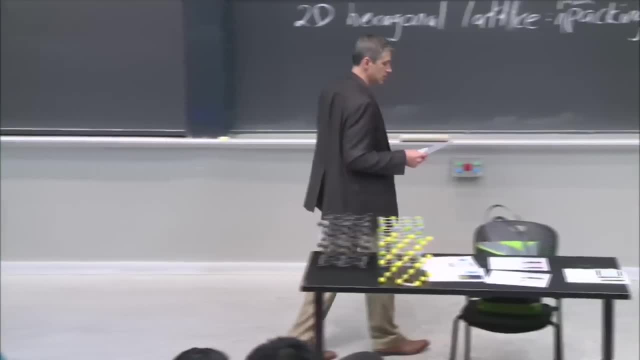 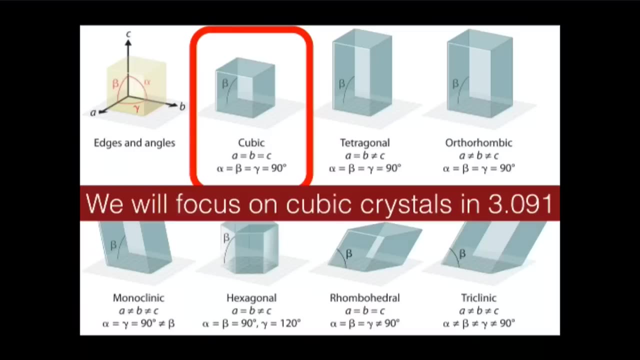 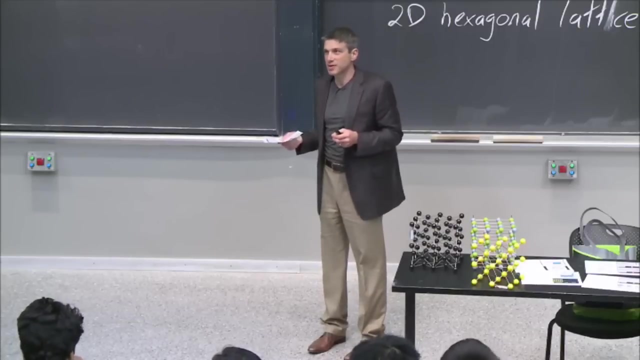 These are the seven ways that we can fill all of space, And there are only seven In this class. we're only going to focus on one, and that's the cubic system, And the reason is that this gives us plenty to work with to understand crystallography. 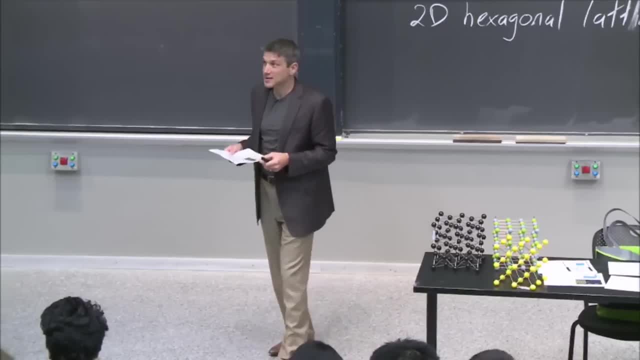 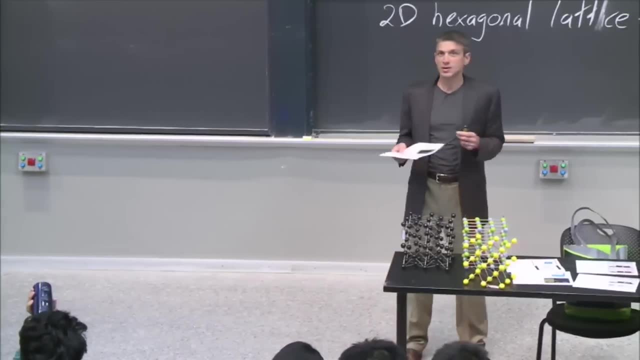 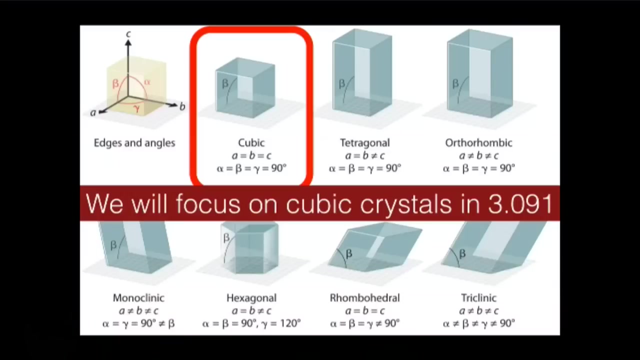 and how chemistry relates to crystallography. And there's the benefit of the fact that a lot of elements take one of these three, Actually, only two, But they take cubic elements: Symmetry. What does that mean? Well, it means that all the lattice vectors are the same. 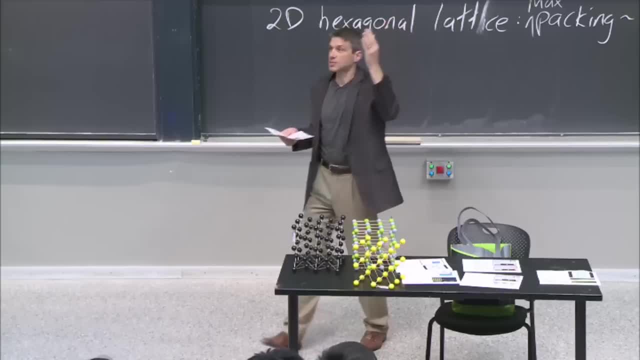 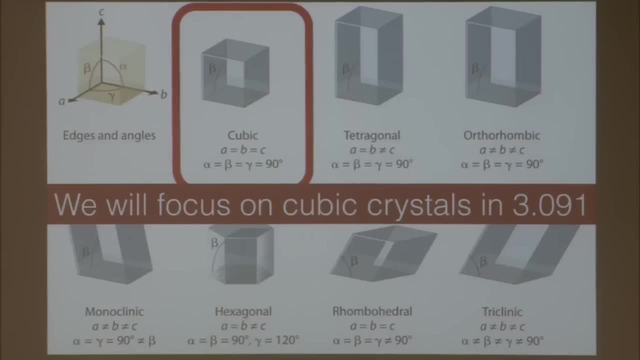 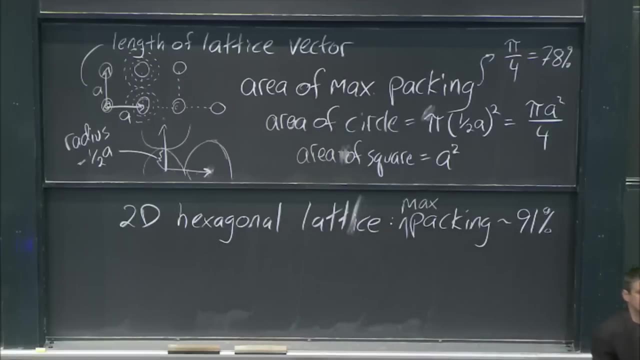 Each one has a length, a. They're orthogonal to each other, which means that the angle is 90 degrees. So we've got a cube. Now it turns out that now you say: well, how do you pack? How can I pack things together in the cubic system? 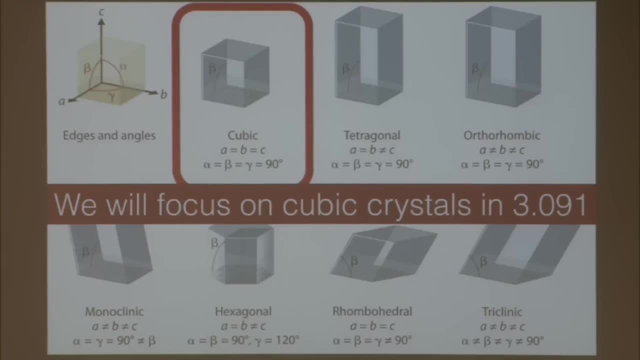 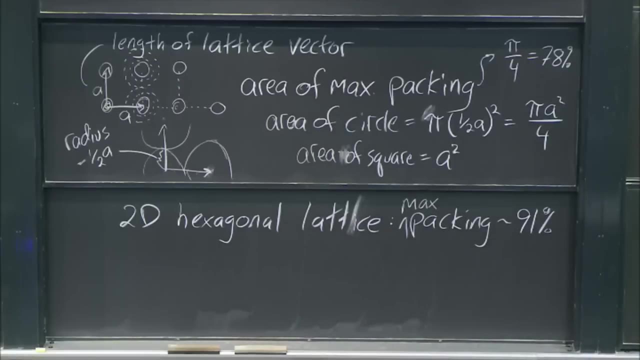 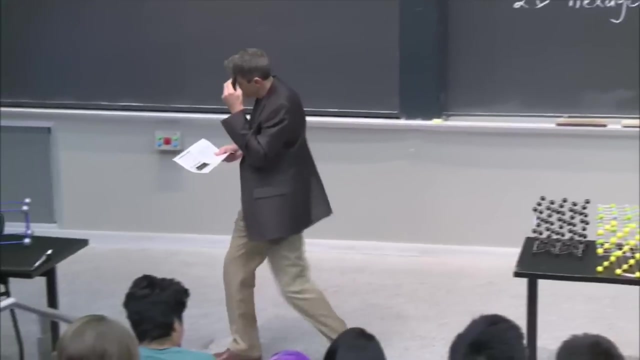 So we've got a cube. Now it turns out that now we say, well, how do you pack? How can I pack things together in the cubic system? And there there's three different ways to do it. So what this is is it's more symmetry and more group theory. 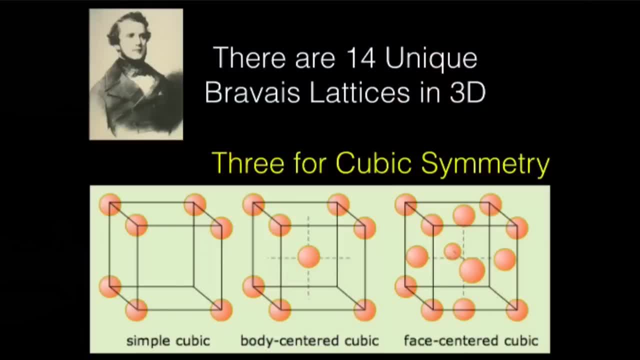 and math that goes into this- that Bravais figured out, And so we call these Bravais lattices. Now, what Bravais figured out, and again, you don't need to know all the math behind this, but I want you to know these three cubic lattices. 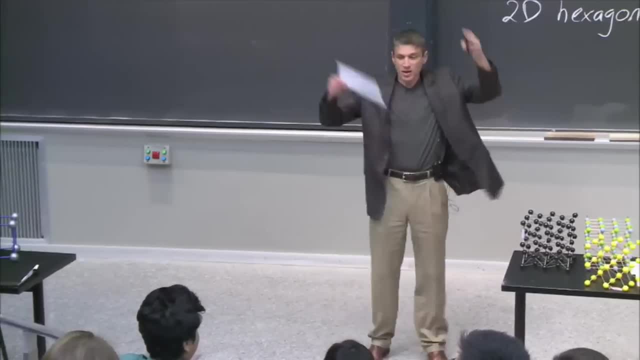 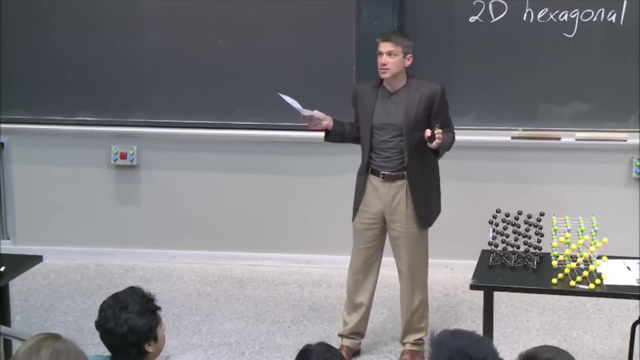 What he figured out is that from the seven crystal systems, there are only 14 ways to pack. There are 14 ways to pack. There are 14 ways to pack. That's it, No more. That's pretty cool. There's no 15.. 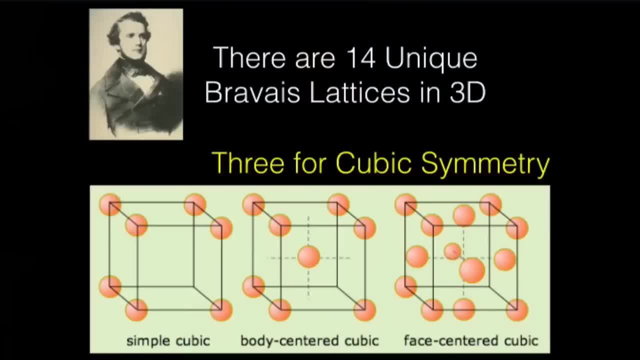 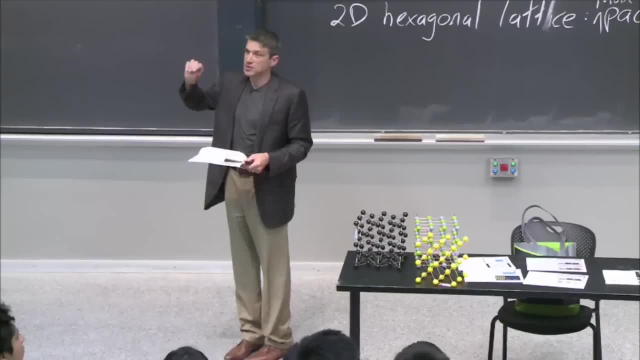 There's no 16.. There's 14, exactly 14 ways that you can: by having a lattice, which means a stamp. there are only 14 ways you can do it for the seven crystal systems And for the cubic system. there's only three. 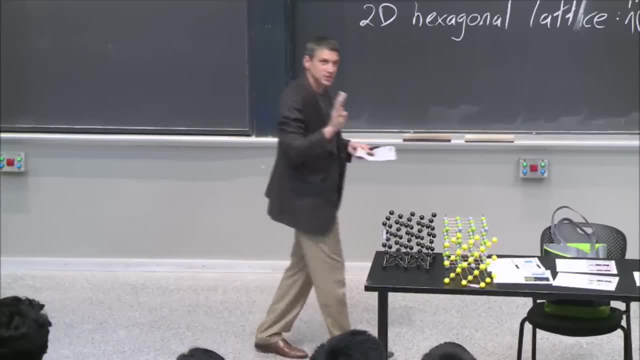 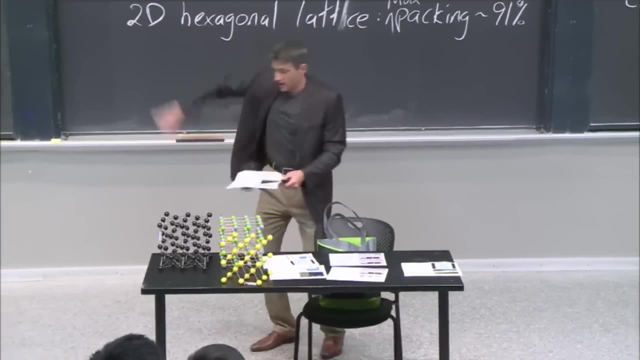 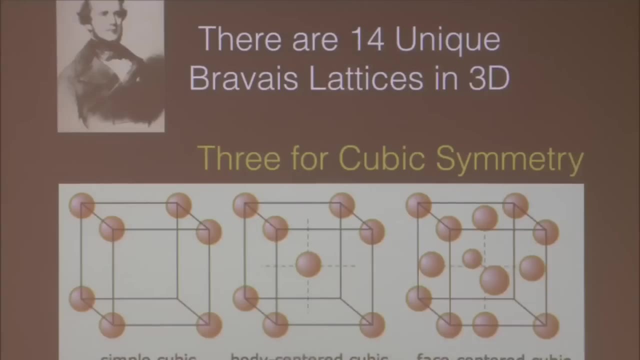 So I have three types of stamp. That's what it means. Three types of stamps where I leave no voids. Right, I leave no voids, So I can tile all of 3D space and it forms a cubic unit cell. 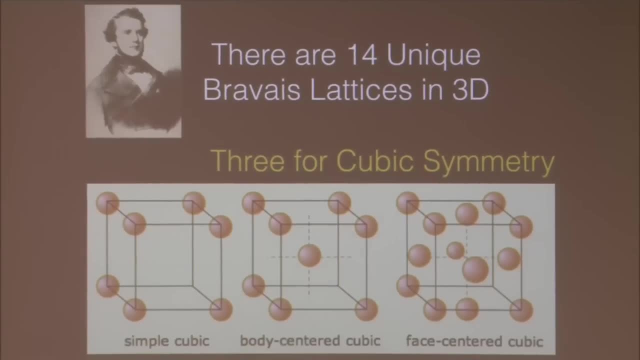 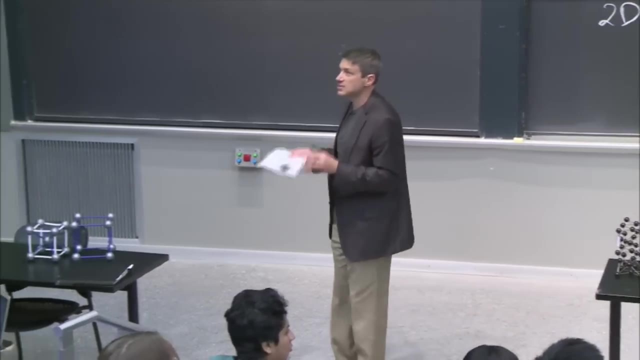 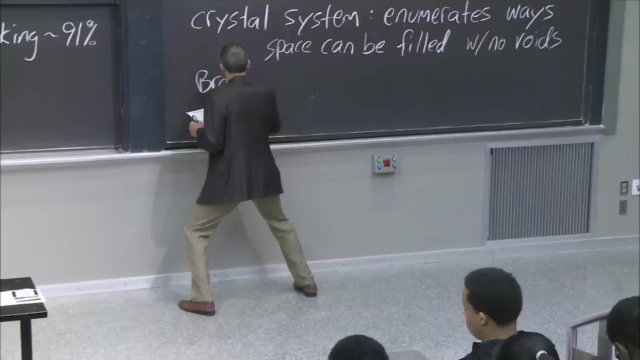 Cubic unit cell. These are the three ways: A simple cubic, a body-centered cubic and a face-centered cubic. These are the three types of lattices that have cubic symmetry. They're the only three. So in a Bravais lattice the difference is. in a Bravais 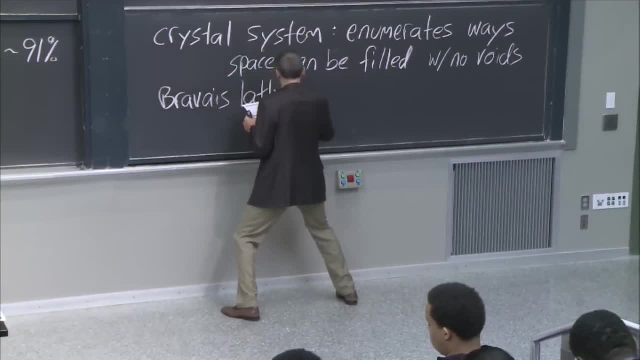 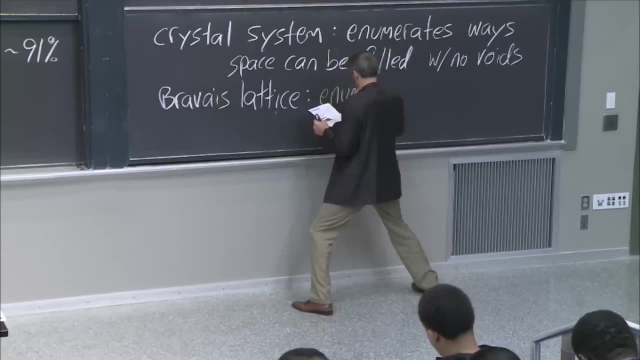 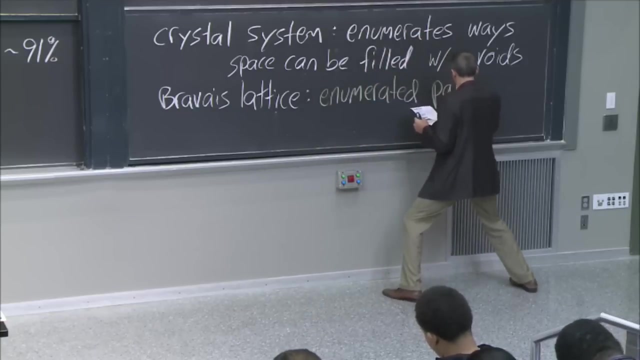 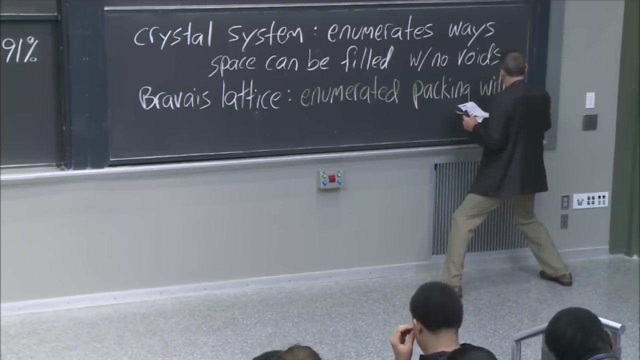 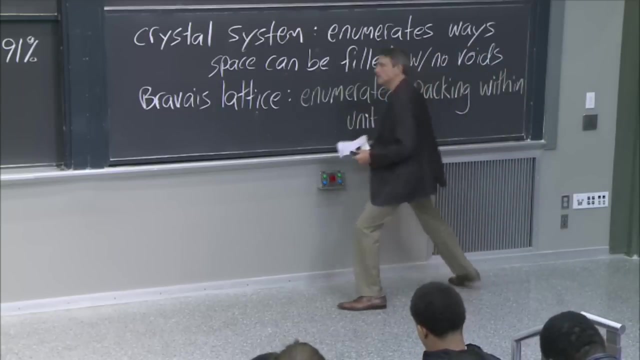 lattice. What Bravais did was he enumerated. So here we enumerate the way space can be filled. He enumerated the packing, all the ways that the space can be packed with, for example, packing within the unit cell. So there's three distinct ways to pack. 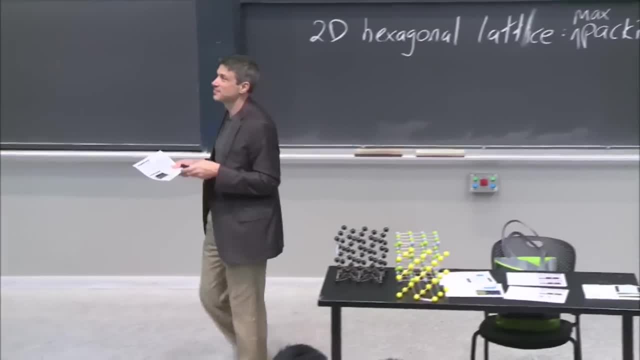 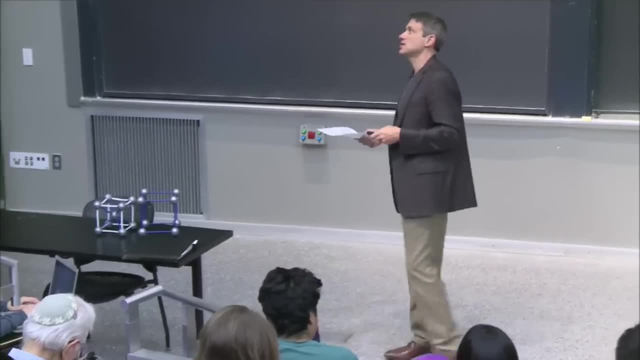 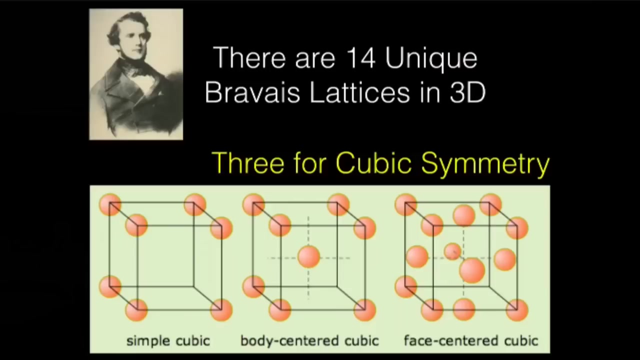 And there there's three different ways to do it. So what this is is it's more symmetry and more group theory and math that goes into this. that Bravais figured out, And so we call these Bravais lattices. Now, what Bravais figured out, and again: 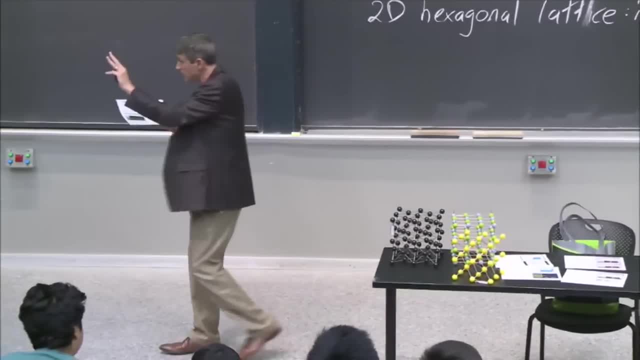 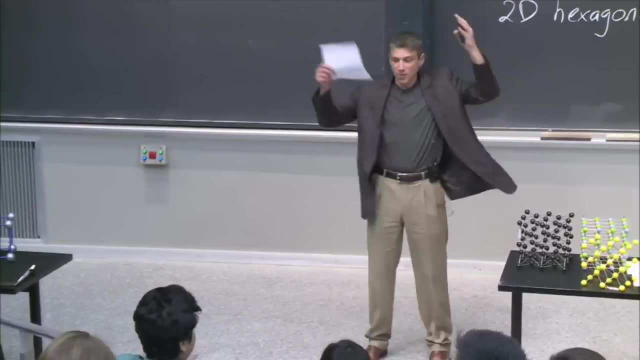 you don't need to know all the math behind this, but I want you to know these three cubic lattices. What he figured out is that from the seven crystal systems, there are only 14 ways to pack. There are 14 ways to pack. 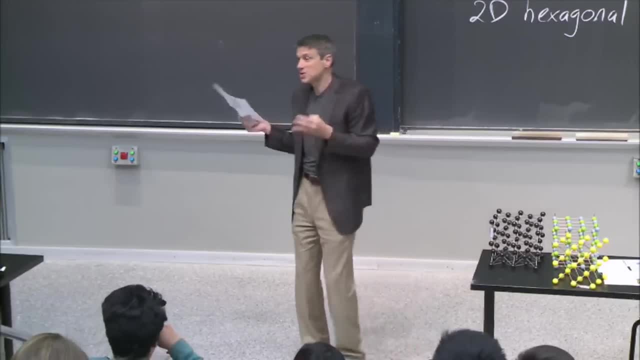 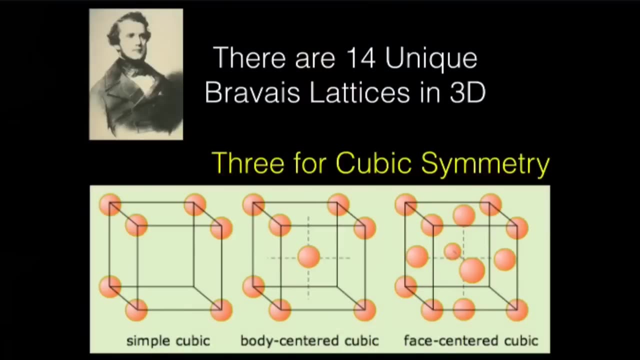 That's it, No more. That's pretty cool. There's no 15.. There's no 16.. There's 14, exactly 14 ways that you can by having a lattice, which means a stamp. there are only 14 ways you can do it. 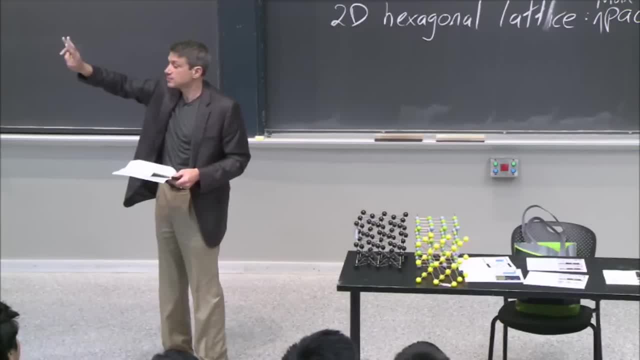 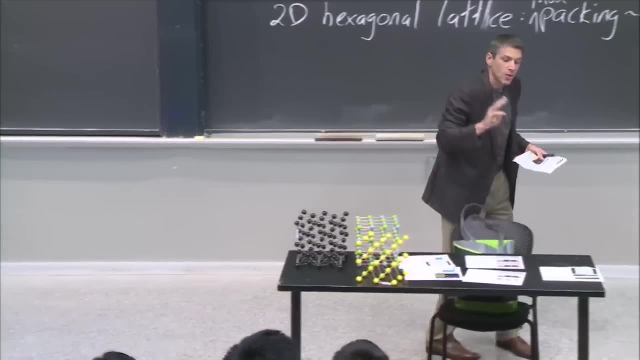 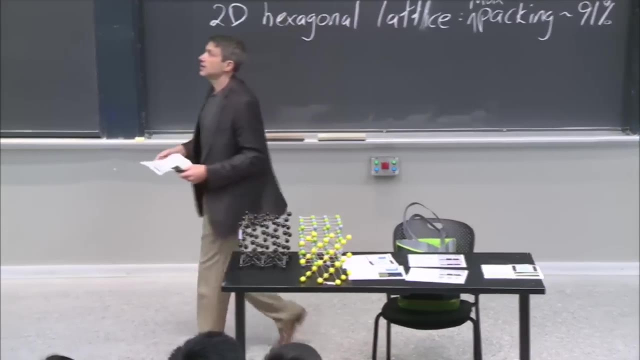 for the seven crystal systems And for the cubic system. there's only three. So I have three types of stamp. That's what it means. Three types of stamps Where I leave no voids. I leave no voids so I can tile all the 3D space. 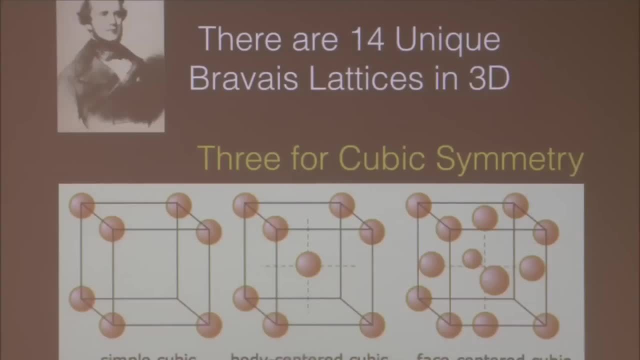 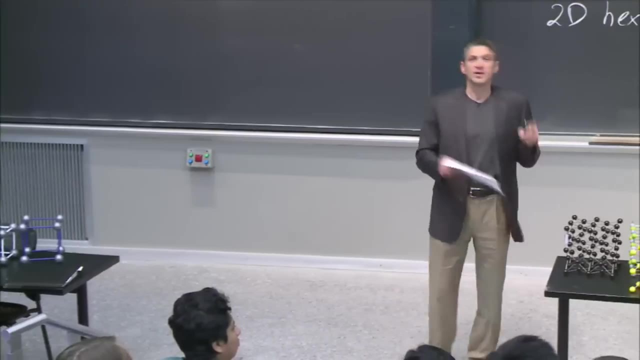 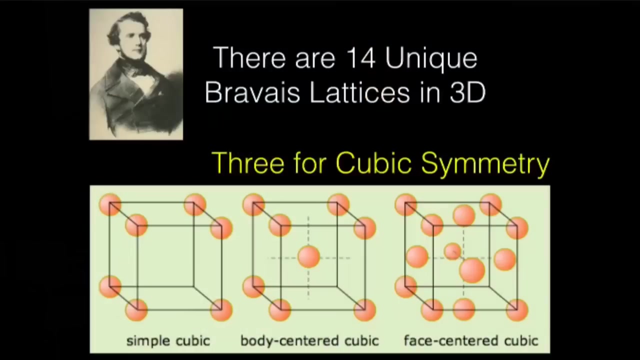 And it forms a cubic unit cell. cubic unit cell. These are the three ways: a simple cubic, a body-centered cubic and a face-centered cubic. These are the three types of lattices that have cubic symmetry. They're the only three. 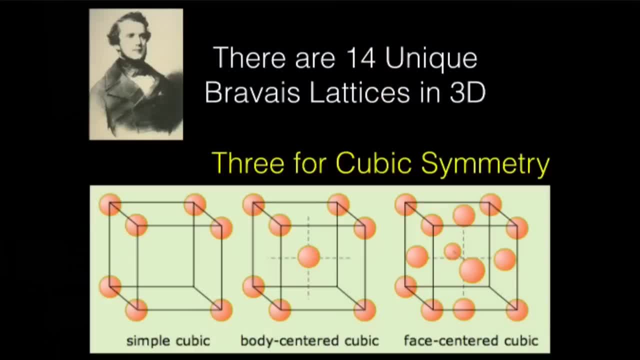 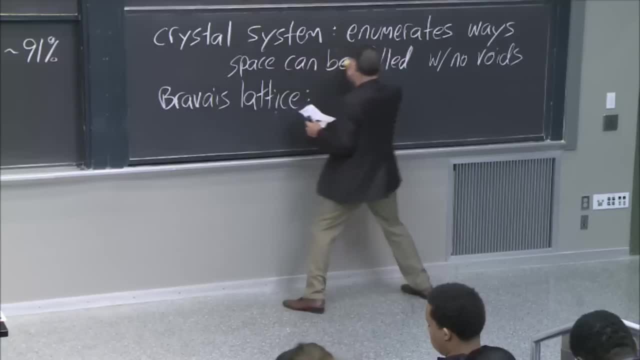 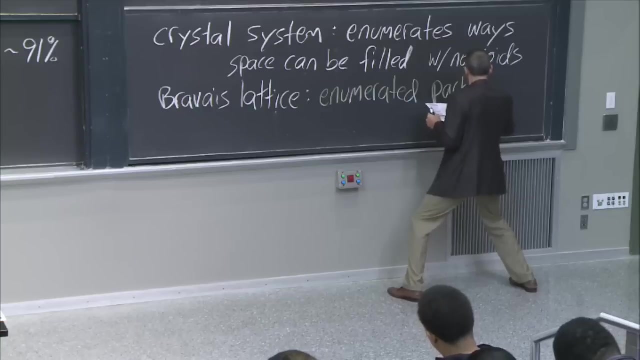 So in a Bravais lattice the difference is. in a Bravais lattice what Bravais did was he enumerated. So here we enumerate the ways space can be filled. He enumerated the packing, all the ways that the space can be packed with. for example, 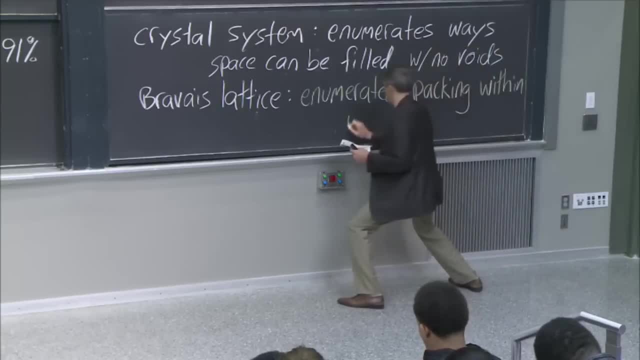 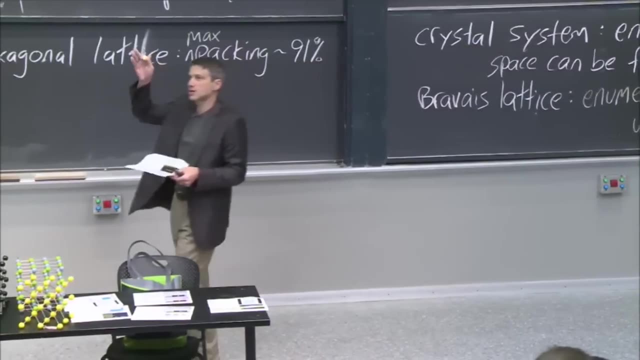 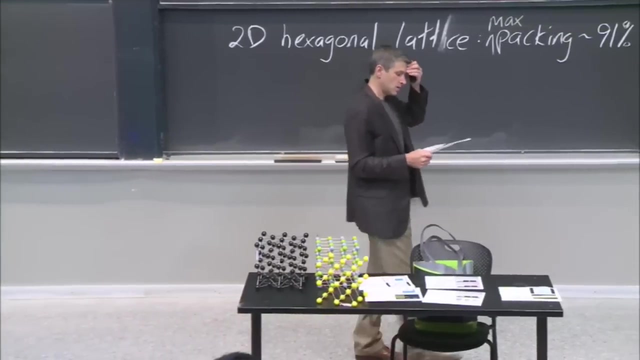 packing within the unit cell. So there's three distinct ways to pack within a cubic unit cell. So that's what we're going to bring to life today and we'll talk more about on Wednesday as well, And what I want to do is I want to go through each one. 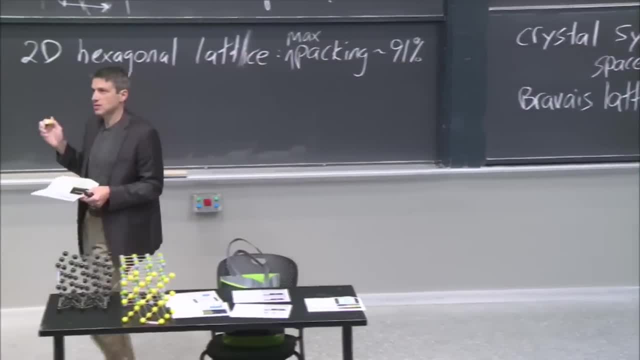 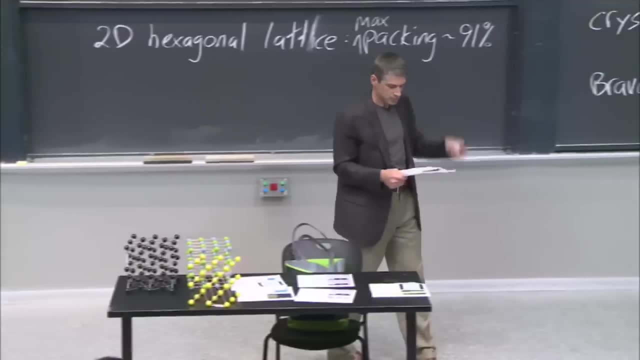 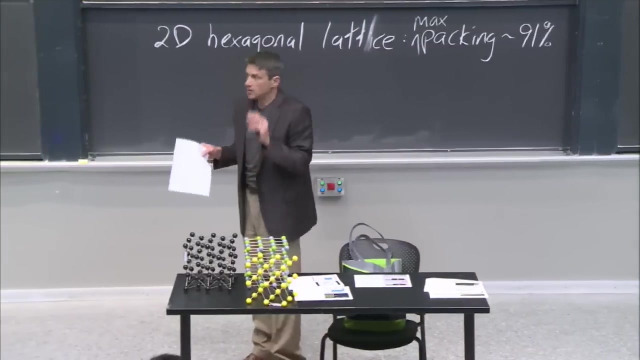 within a cubic unit cell. That's what we're going to bring to life today and we'll talk more about on Wednesday as well, And what I want to do is I want to go through each one. So we're going to go through simple cubic, body-centered. 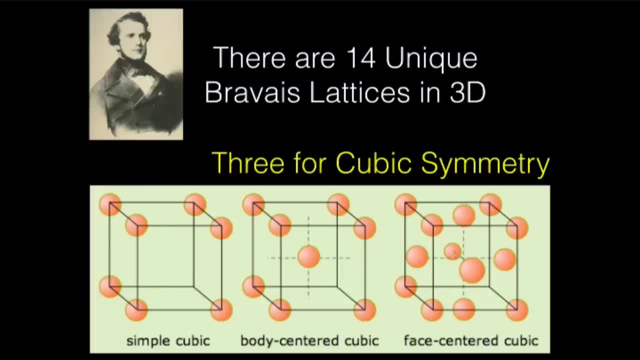 cubic, face-centered cubic, And then, with each one, I'm going to talk, I'm going to go through each one. I'm going to go through each one, I'm going to go through each one, I'm going to talk about it for a minute. 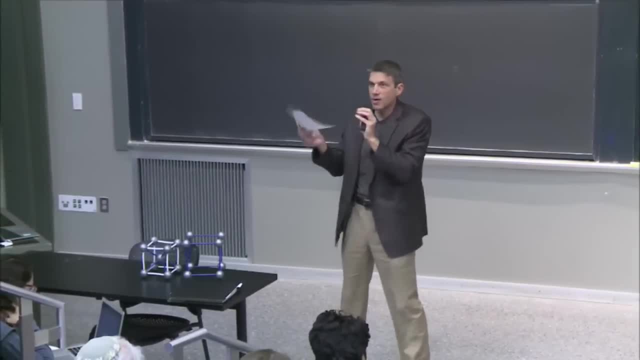 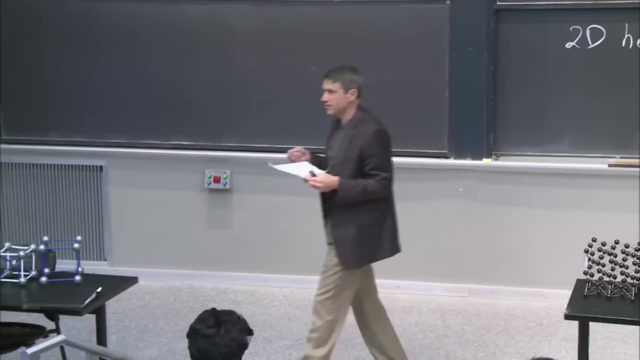 And then I'm going to show you a little video so that we can really see how the unit cell gets sliced up. And there's a razor that comes in and slices it. It's really cool, And so you can really see and feel what we're talking about. 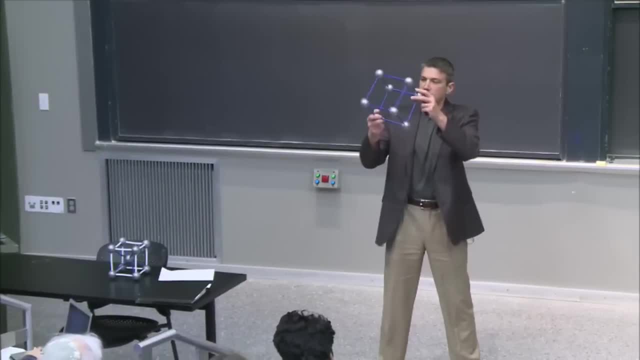 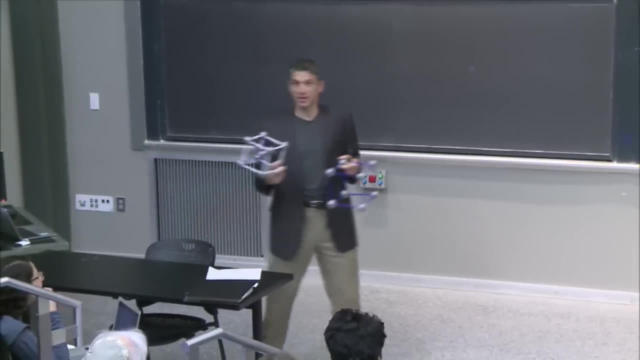 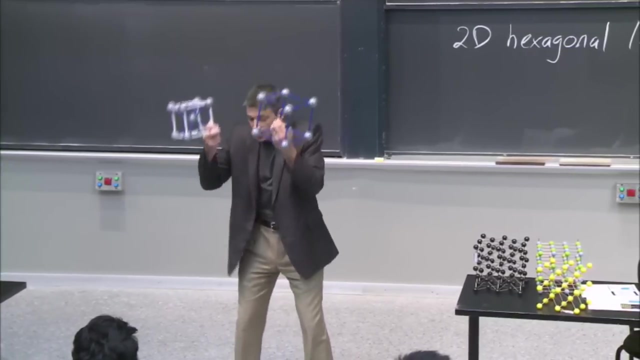 And speaking of seeing and feeling, so I have these And I had wanted for these to be what go in your goodie bag, But apparently $100,000 is too much or whatever. So you have smaller versions of these And I encourage you. there's no better way. 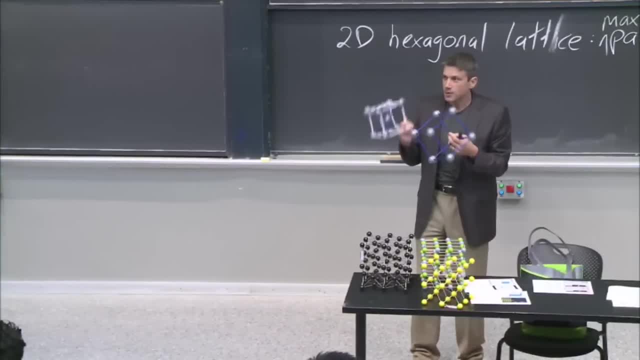 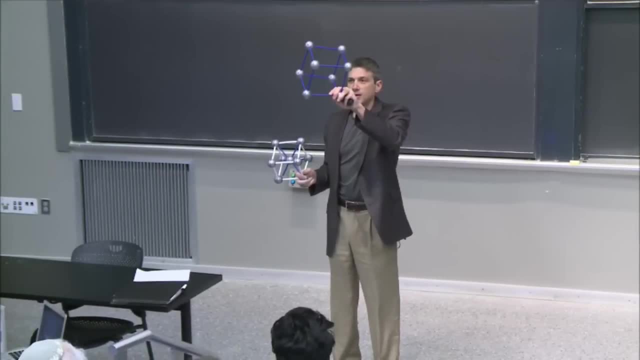 to think about crystallography than to build stuff and see it. You got to do that. It's really cool, And so this is the simple cubic. OK, so we'll pass that around, And this is the body-centered cubic. 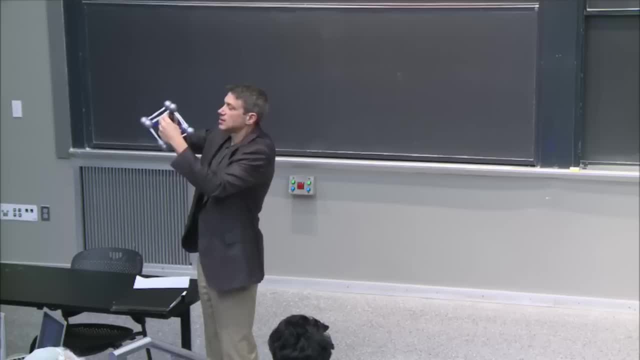 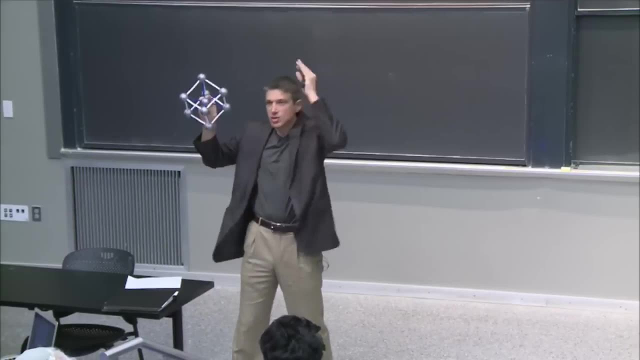 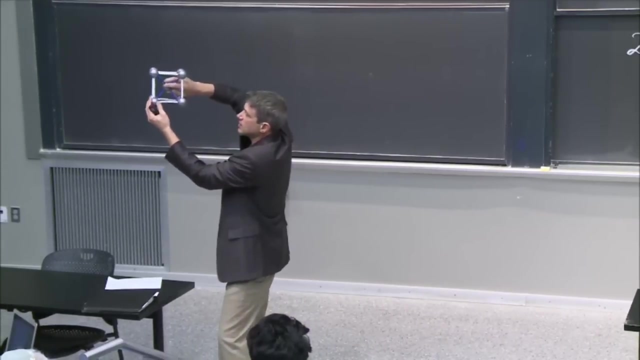 And here you have spheres, right. That's fine, But all we've done so far is set up a lattice. This could be anything. It's a repeat lattice, It's a lattice. No, that's what a lattice is. The lattice just defines that this is the same as this. 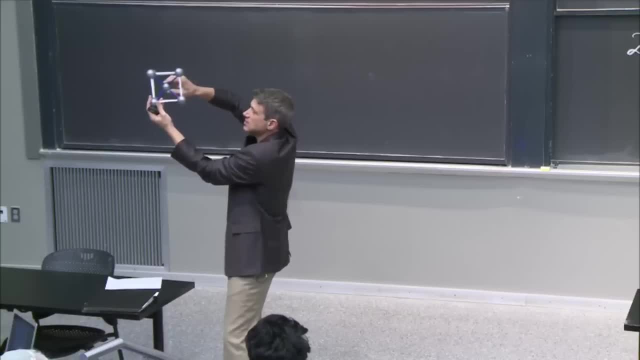 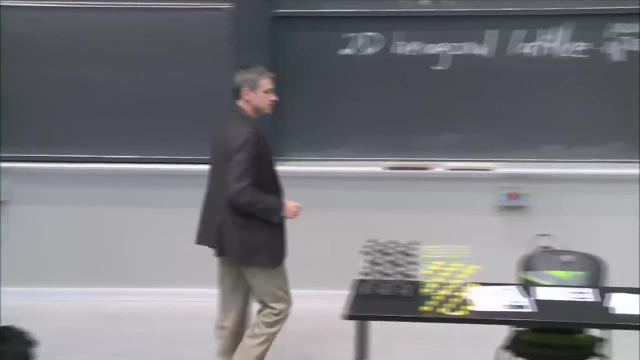 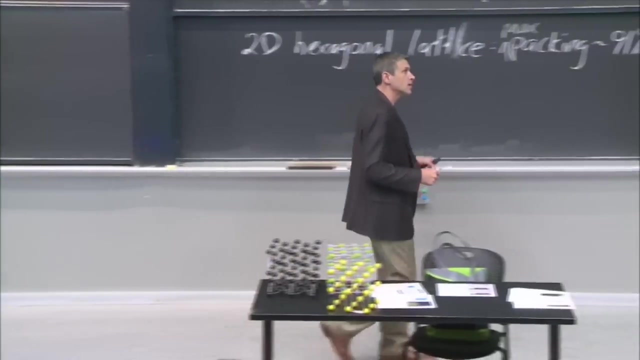 Whatever is here is the same, is the same as this, is the same as this. That's what we're defining here, OK, OK, all right. Now let's talk about these three. This is a picture from April. These are the three systems I just talked about. 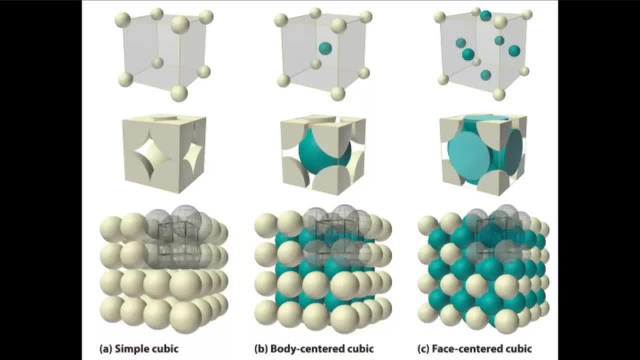 the three Bravais lattices, three different ways to pack In a cubic symmetric cell And notice there's three ways of looking at it right. So here is sort of a ball and stick model which is easy. It makes it easy to see the bonding and the atoms. 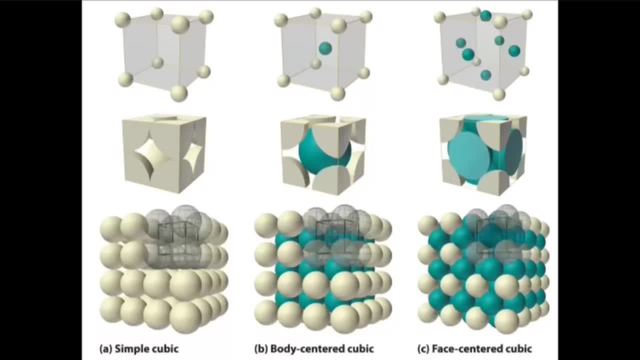 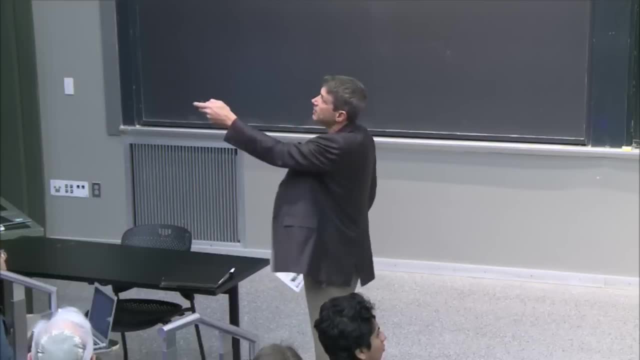 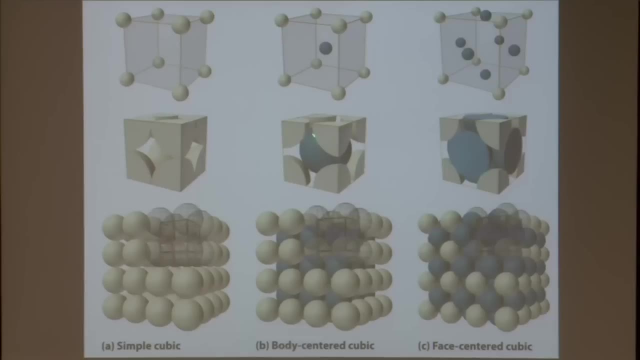 But the space-filling model is really important here, because the space-filling model lets us think about the maximum packing. That's really important. Remember the maximum packing because, remember, these are bonding Really, These are bonding together Right. 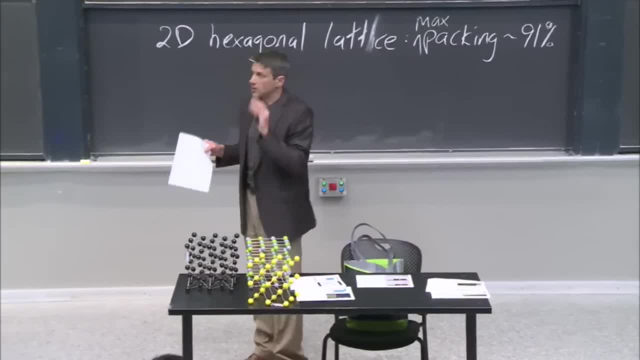 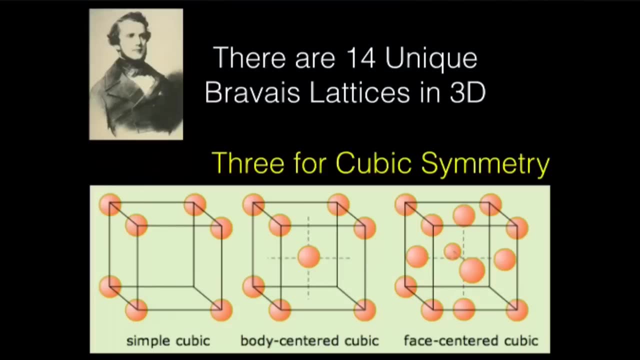 So we're going to go through simple cubic, body-centered cubic, face-centered cubic, And then with each one I'm going to talk about it for a minute. And then I'm going to talk about it for a minute And then I'm going to show you a little video so that we can. 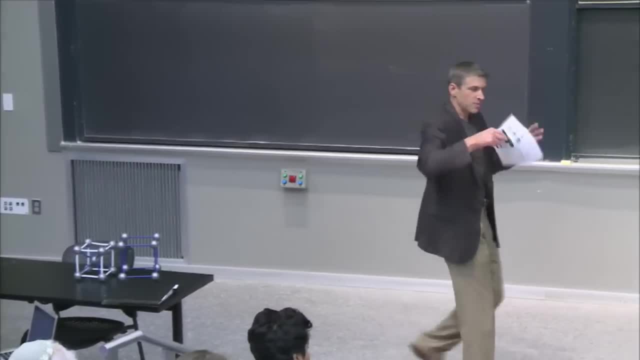 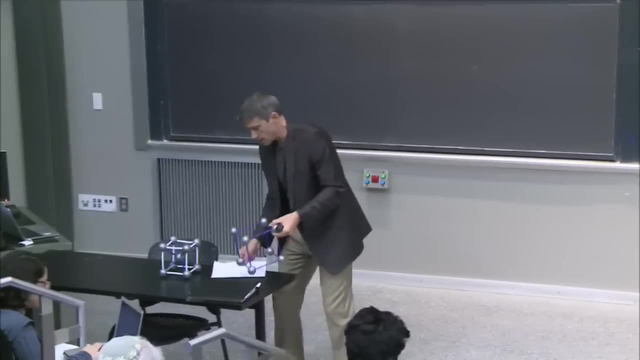 really see how the unit cell gets kind of sliced up And there's like a razor that comes in and slices it. It's really cool And so you can really see and feel what we're talking about. And speaking of seeing and feeling, so I have these. 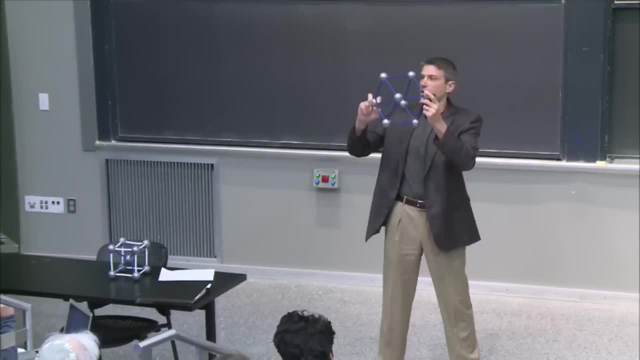 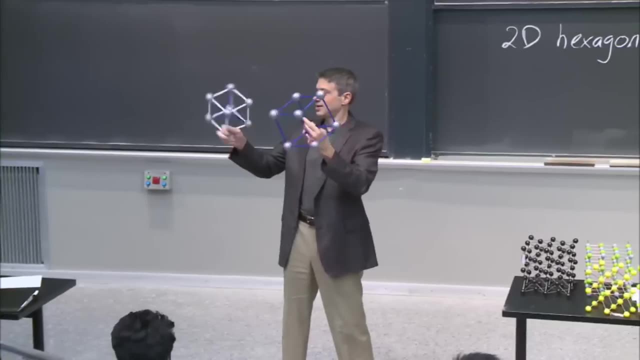 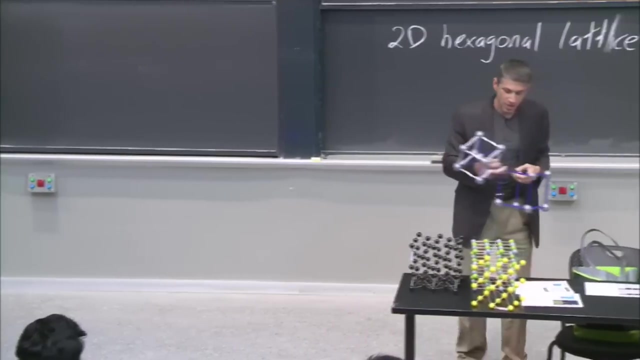 And I had wanted for these to be what go in your goodie bag, But apparently $100,000 is too much or whatever. So you have smaller versions of these And I encourage you. there's no better way to think about crystallography than to build stuff and see it. 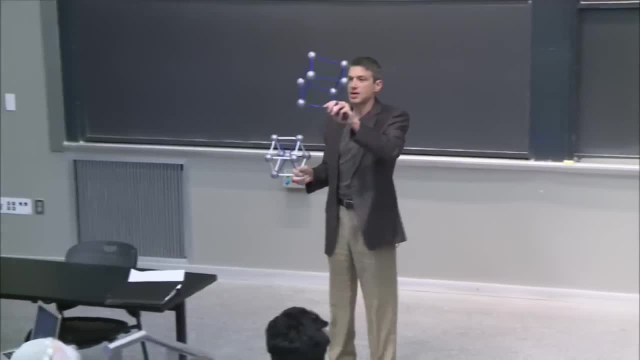 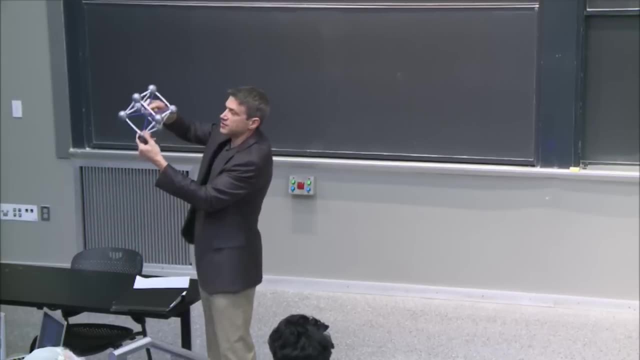 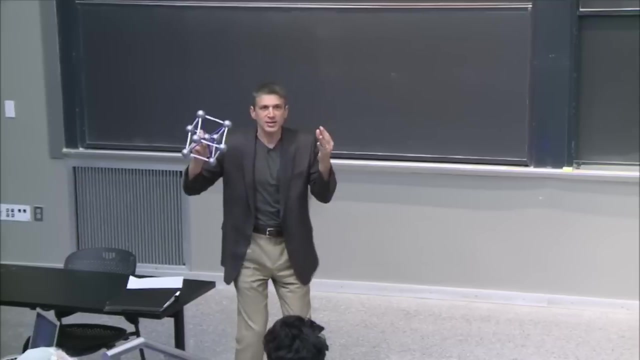 You've got to do that. It's really cool, And so this is the simple cubic. OK, so we'll pass that around, And this is the body-centered cubic, And here you have spheres. right, That's fine, But all we've done so far is set up a lattice. 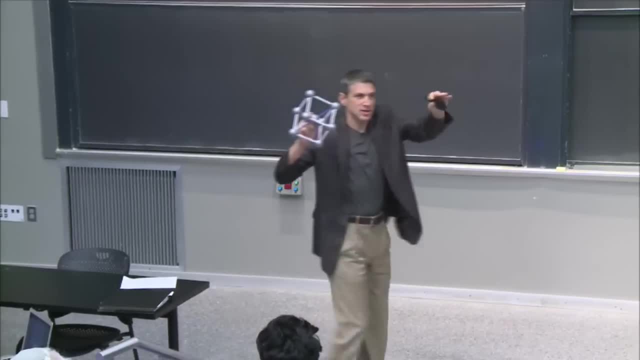 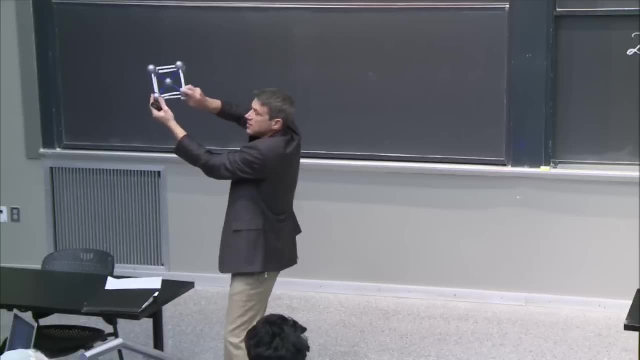 This could be anything. It's a repeat lattice. It's a lattice. No, that's what a lattice is. The lattice just defines that this is the same as this. Whatever is here is the same is the same as this is the same as this. 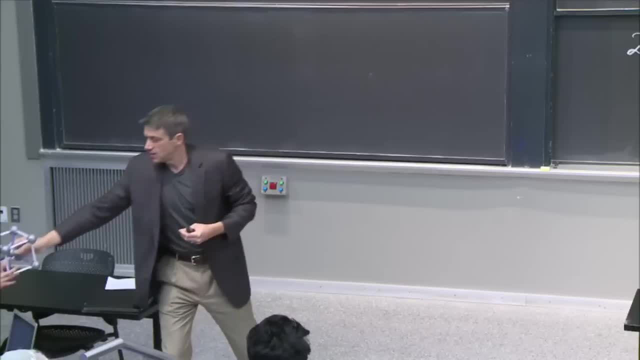 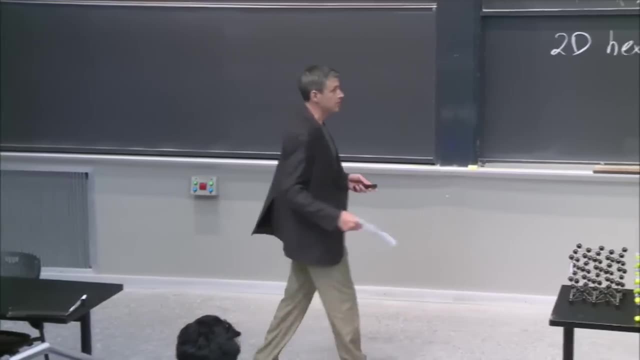 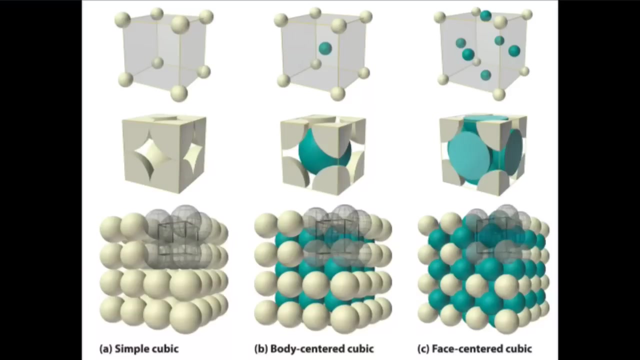 That's what we're defining here, OK, OK, all right, Now let's talk about these three. This is a picture from April. These are the three systems I just talked about, the three Bravais, lattices, three different ways. 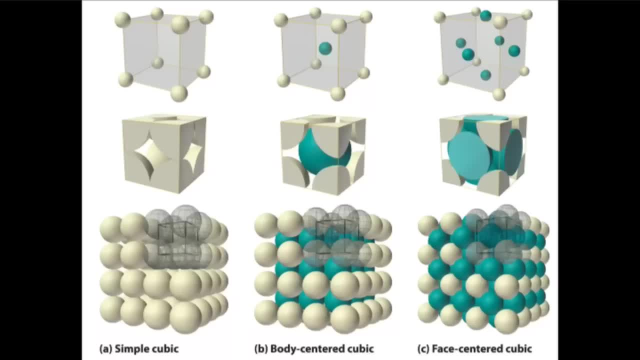 to pack in a cubic symmetric cell And notice there's three ways of looking at it, right. So here is sort of a ball and stick model, which is easy. It makes it easy to see the bonding and the atoms. But the space-filling model is really important here. 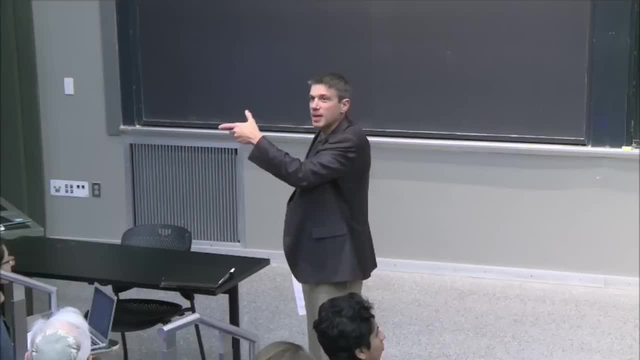 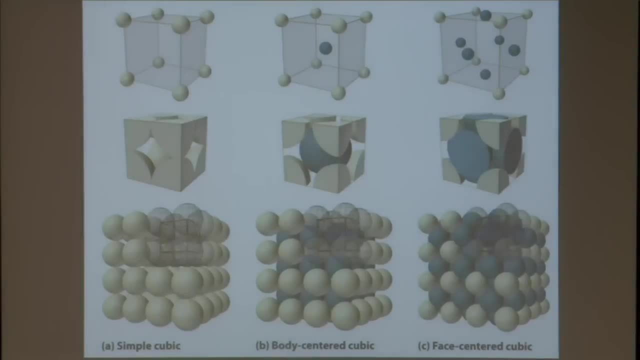 Because the space-filling model lets us think about the maximum packing. That's really important. Remember the maximum packing Because, remember, these are bonding Really. Yes, These are bonding. These are bonding together, right, So drawing them all the way up to where they touch. 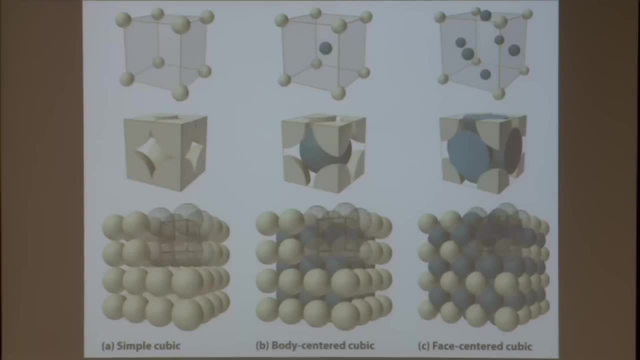 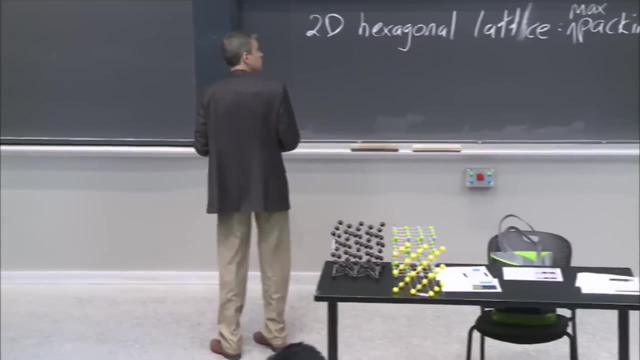 So drawing them all the way up to where they touch right, That's going to help us understand how they pack in, what their maximum packing can be. So let's look at that for the simple cubic. OK, So for the simple cubic, we'll do that here. 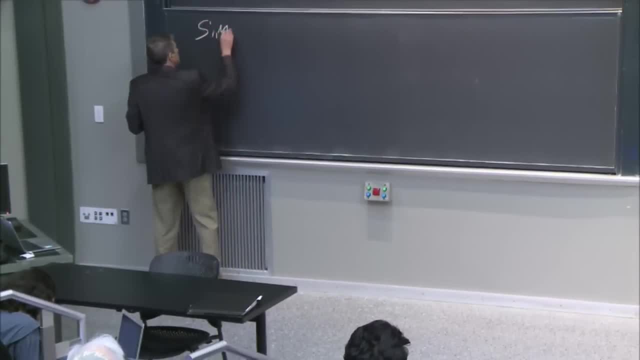 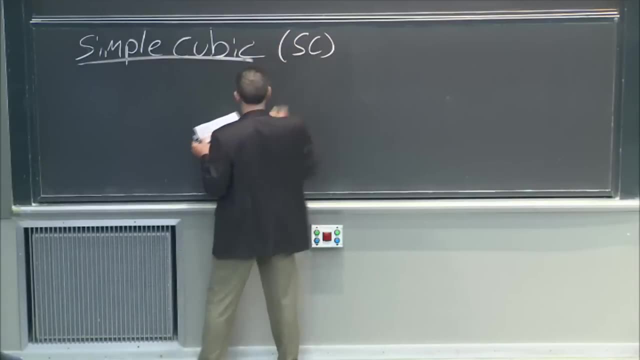 Simple cubic. OK, simple cubic. Oh, let's just call it SC for short. Why not? Now? one of the things you want to think about is how many of these are going to be the nearest neighbors to each other. How many nearest neighbors do I have? 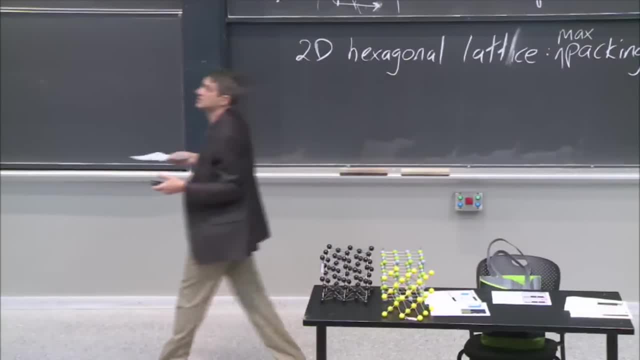 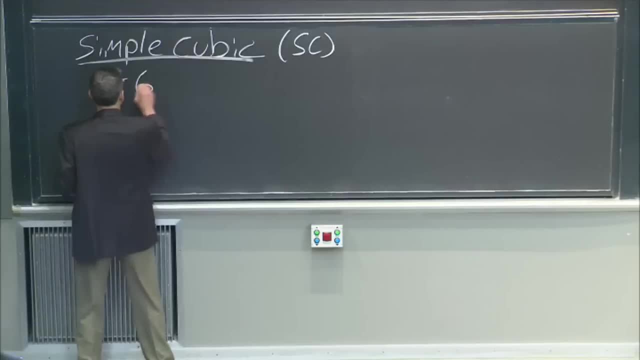 And I lost the thing. So you can see. look at the edge and think about how many nearest neighbors. Well, you know you got six right. If you're in the corner there of the cube, in your simple cubic, you've got six nearest neighbors. 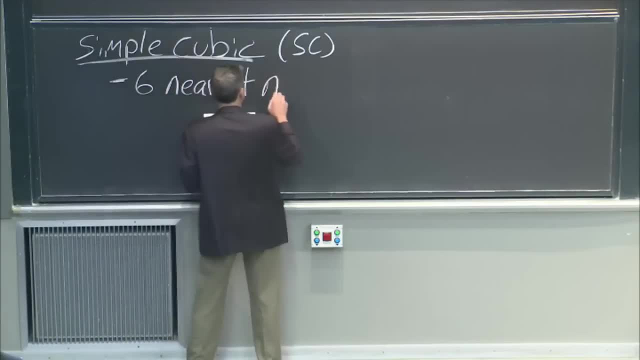 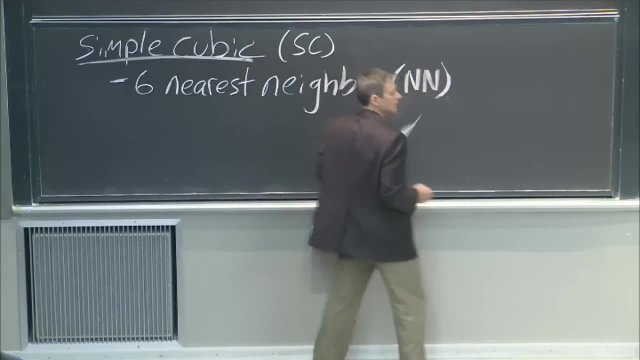 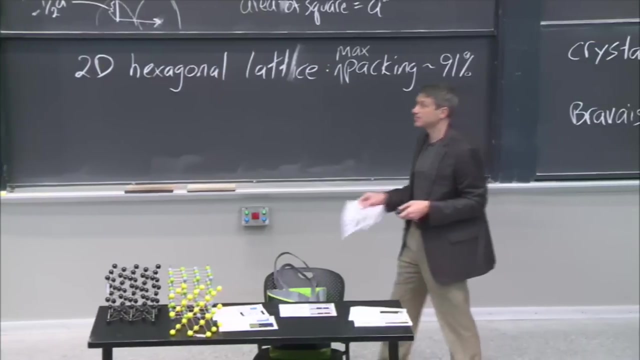 OK, that's important, right? Six nearest neighbors Those are. why is that important? Well, it's important because that's how many bonds, that's how many other atoms you could bond with in this solid? OK, But the other thing we want to know is the packing. 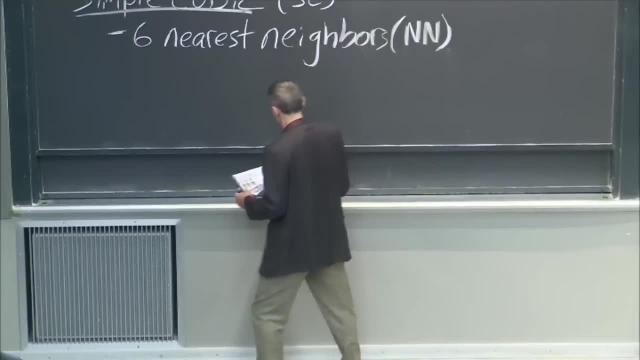 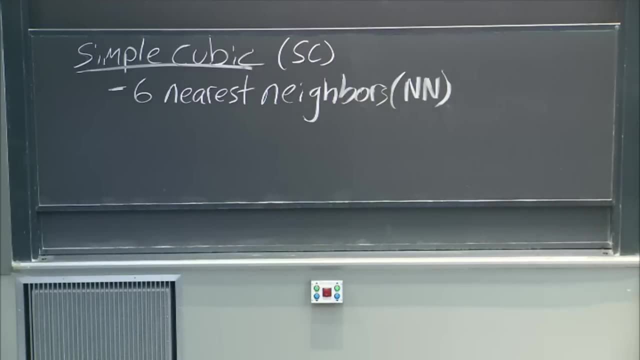 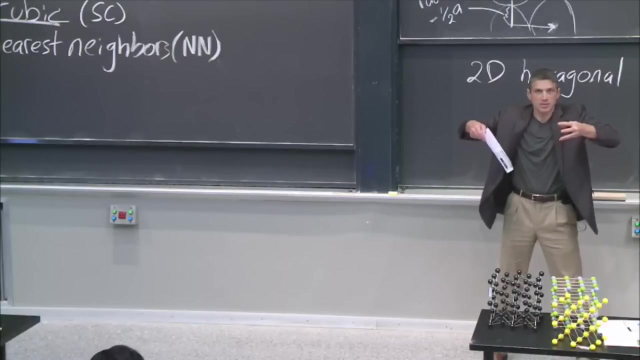 Now again, what you want to do to figure out the maximum packing is. you want to think about it in the same way we did here. Think about putting something at each of the lattice points and then growing it out right until they can't grow anymore. 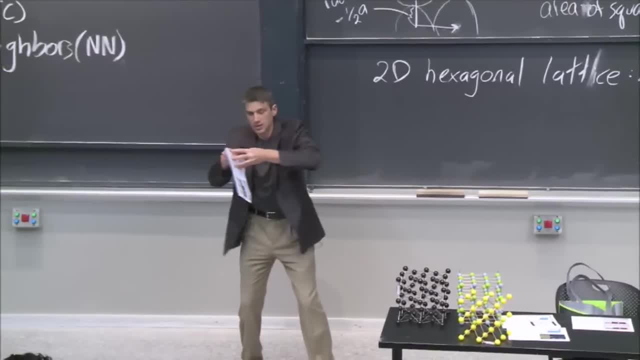 That's a good way to think about it. OK, And in this case, we're going to take spheres. We're going to be taking spheres because that's how we're going to represent atoms. OK, so we're going to be taking spheres. 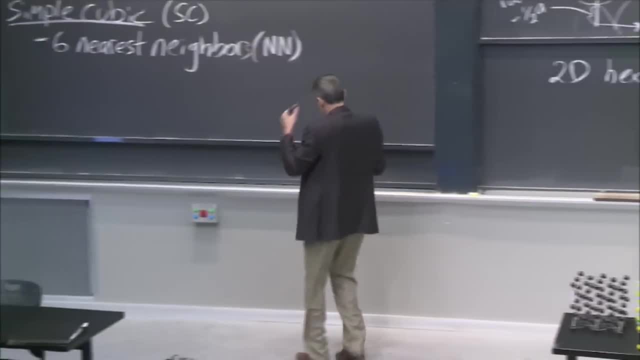 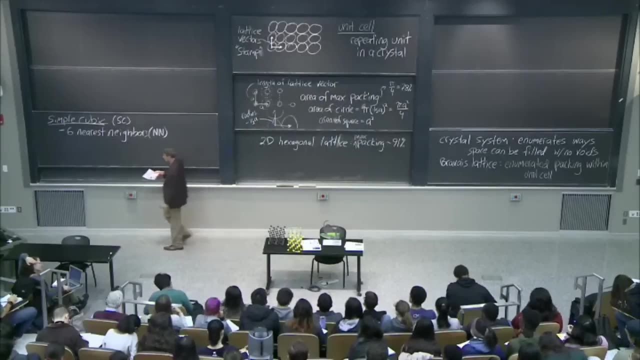 And we're going to grow them out and see what the packing is. Yeah, but I got to do the same trick. I did here. I got to do the same trick I did here. I got to write the radius of the atom in terms of the unit cell. 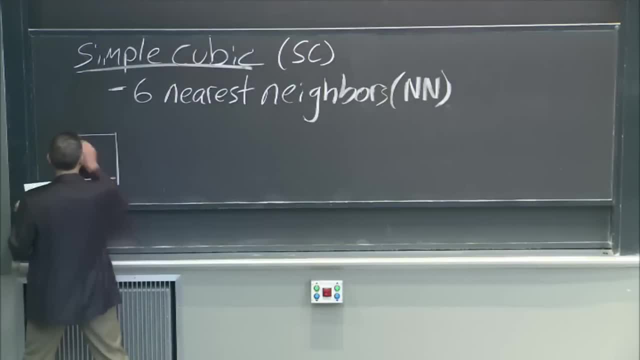 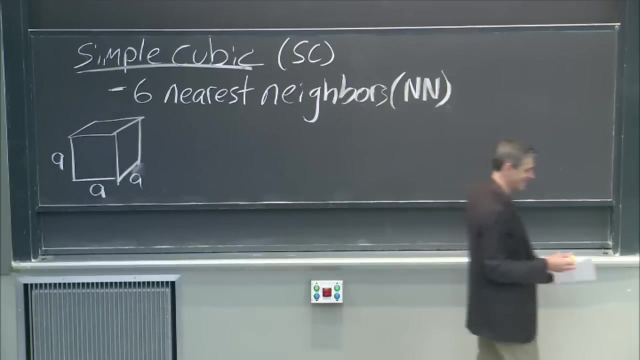 So if the unit cell- oh boy, I'm going to be drawing a 3D structure- Danger, Danger, A, A, A. It's a cube. All the sides are A. I just made myself very happy: It's a cube. 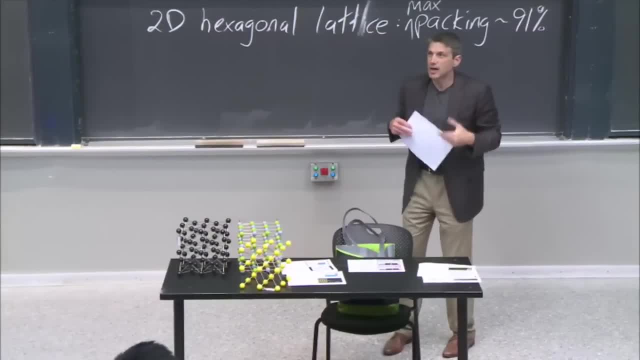 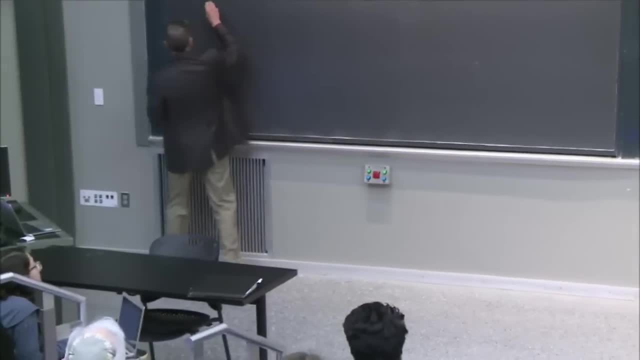 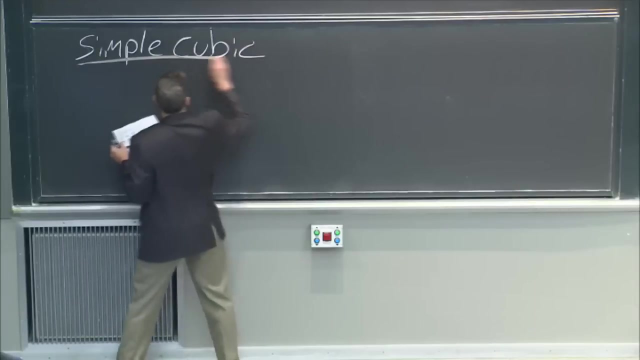 that's going to help us understand how they pack in, what their maximum packing can be. So let's look at that for the simple cubic, OK. So for the simple cubic, we'll do that here. Simple cubic, OK, Simple cubic. 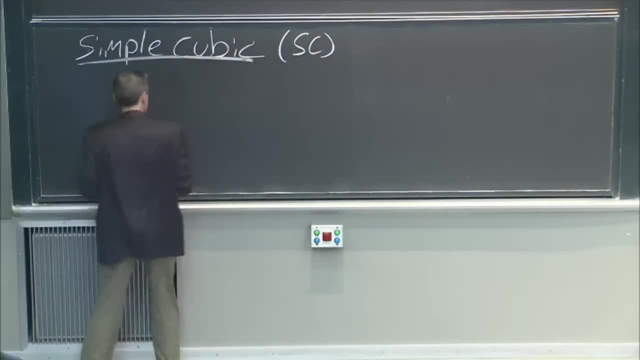 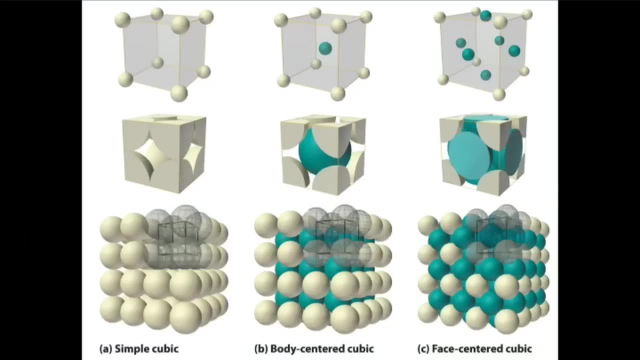 Oh, let's just call it SC for short. Why not Now? one of the things you want to think about is how many nearest neighbors do I have And I lost the thing, So you can see, look at the edge and think about. 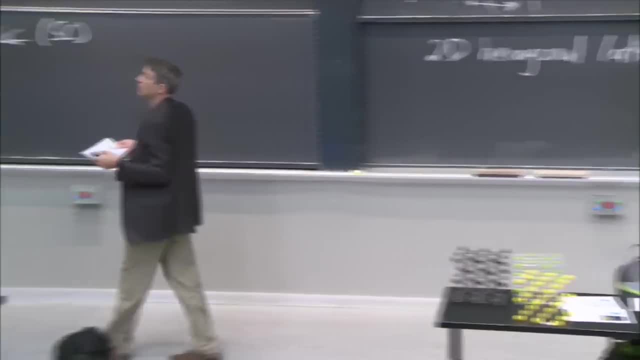 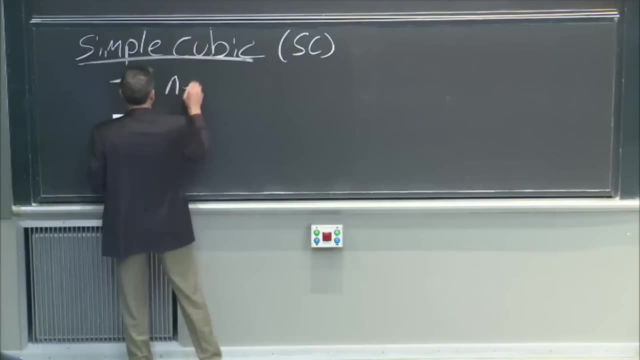 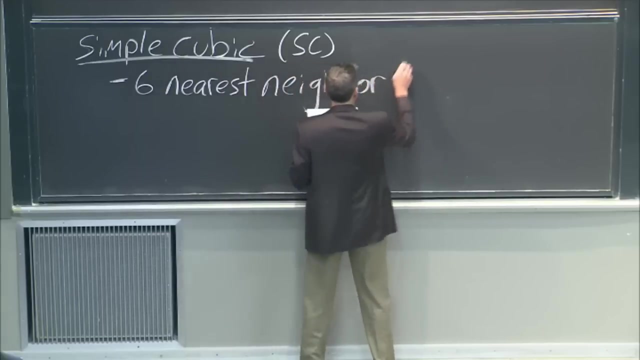 how many nearest neighbors? Well, you know, you got six right. If you're in the corner there of the cube, in your simple cubic, you've got six nearest neighbors. OK, that's important, right, Six nearest neighbors Those are. why is that important? 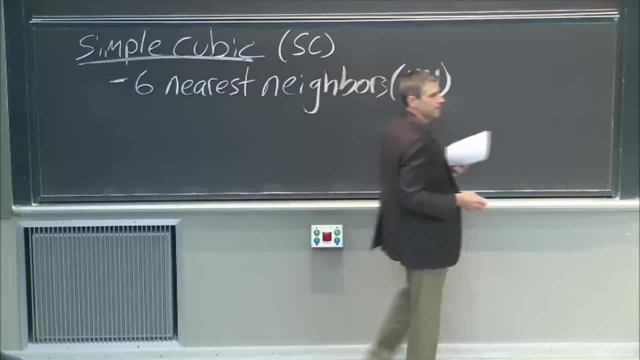 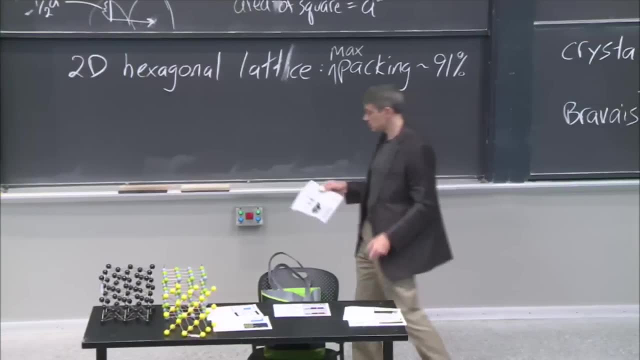 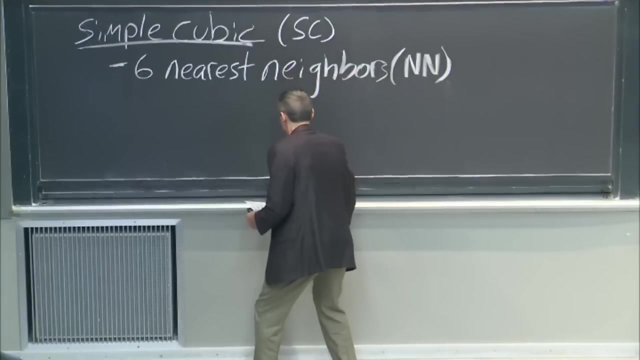 Well, it's important because that's how many bonds, that's how many aldehydes, Those are atoms you could bond with in this solid, OK, But the other thing we want to know is the packing Now again, what you want to do to figure out. 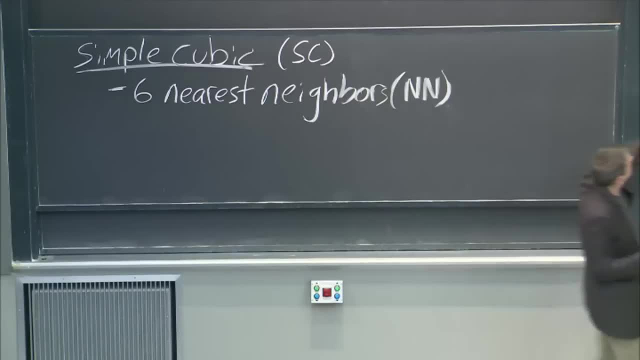 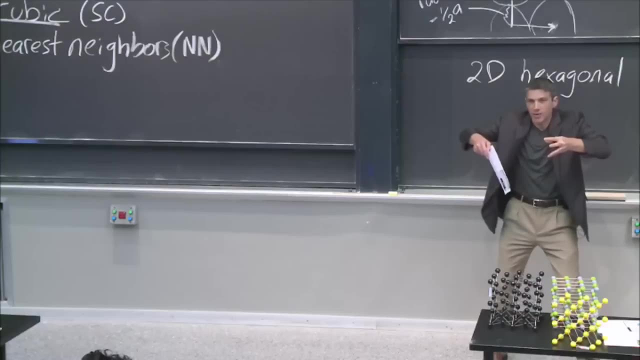 the maximum packing is. you want to think about it in the same way we did here. Think about putting something at each of the lattice points and then growing it out right until they can't grow anymore. That's a good way to think about it. 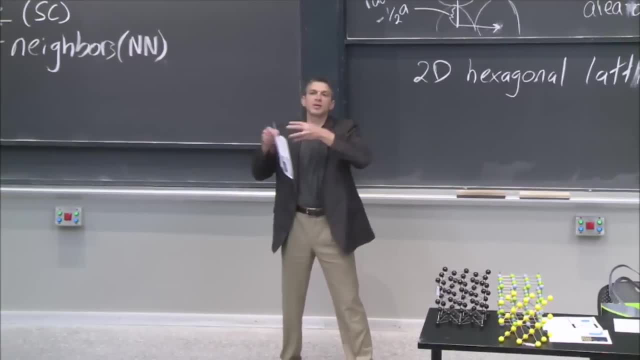 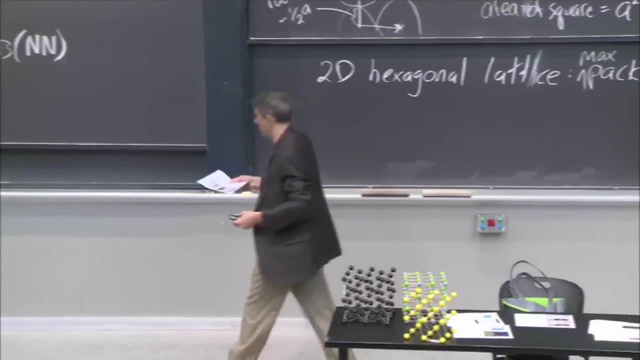 And in this case, we're going to take spheres. We're going to be taking spheres because that's how we're going to represent atoms. OK, so we're going to be taking spheres And we're going to grow them out and see what the packing is. 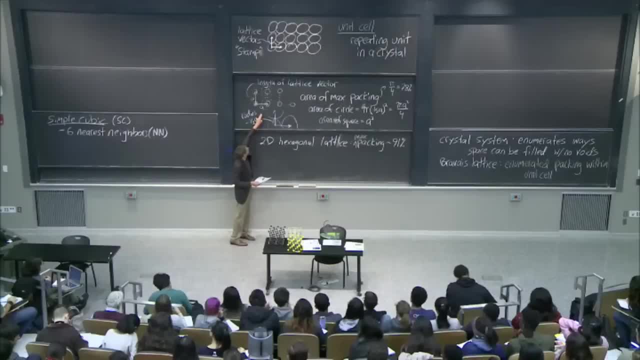 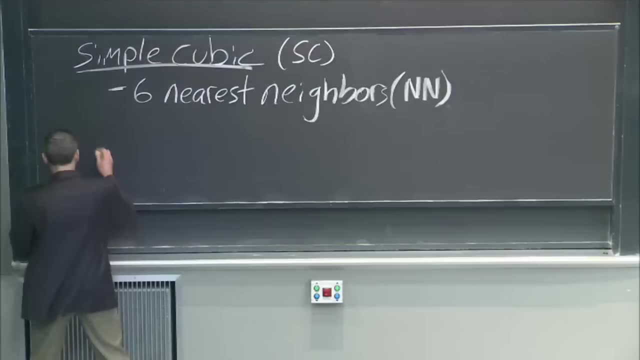 Yeah, but I got to do the same trick. I did here. I got to do the same trick I did here. I got to write the radius of the atom in terms of the unit cell. So if the unit cell, oh boy, I'm going. 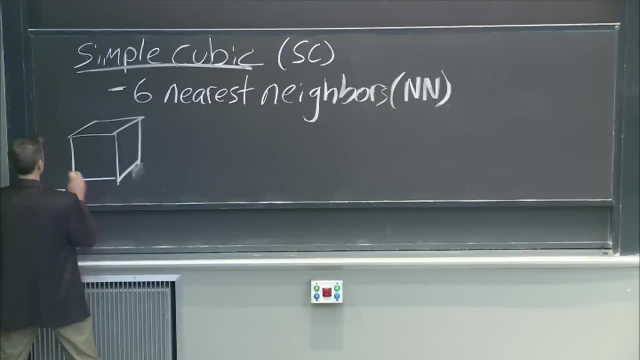 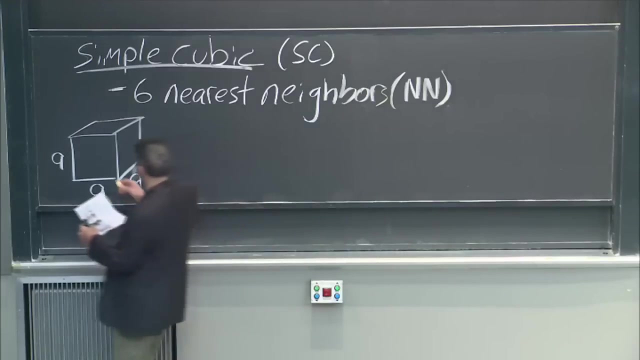 to be drawing a 3D structure. Dang Danger, A, A, A. It's a cube. All the sides are A. I just made myself very happy. It's a cube Now, oh so, but we have a cubic. 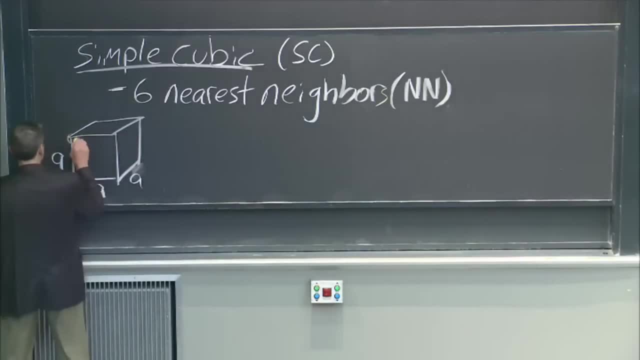 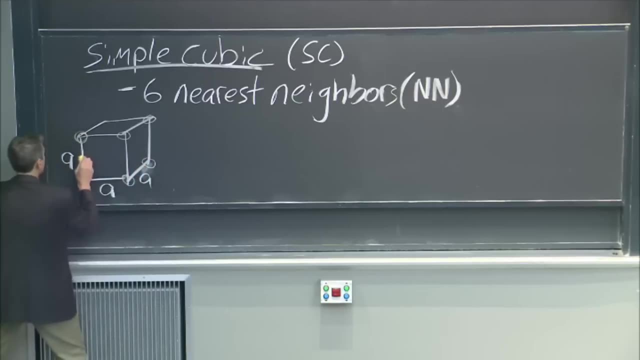 Now, oh so, but we have a cubic Now, OK, here we go. This one, Oh, but see, I want maximum packing, So I'm going to grow them out And you can see what's going to happen, right as I do that. 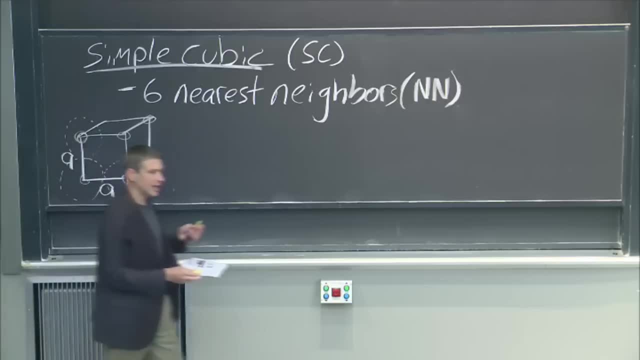 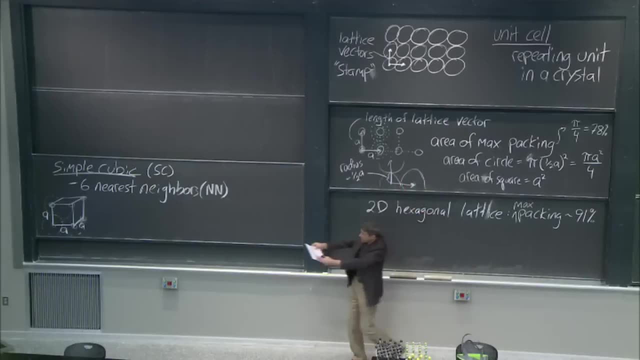 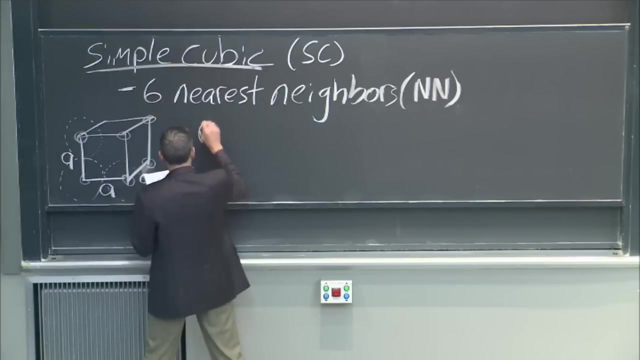 And so you can see that in the case of a simple cubic lattice, it's just like in the square lattice. It's just like in the square lattice, right, When I've grown out the sphere, the radius of that sphere, the radius is r- equals now, oh, wait a second. 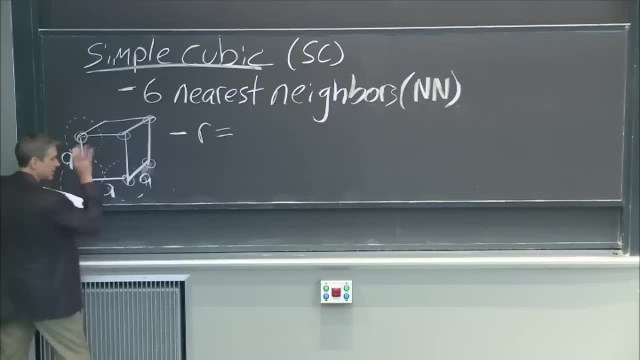 OK, so I have 4 thirds pi or q? OK, but it doesn't matter. yet Don't do volume. Think about the radius. OK, the radius is just going to be a half. The radius is just going to be a half. the lattice right. 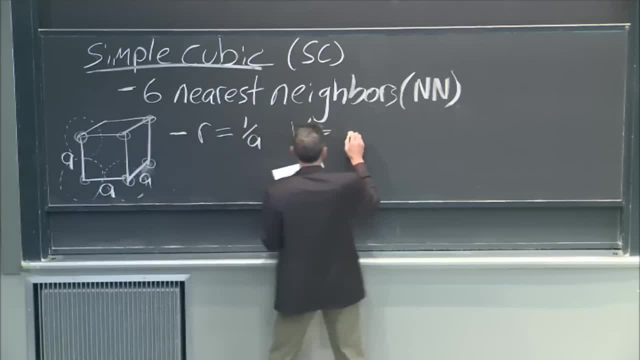 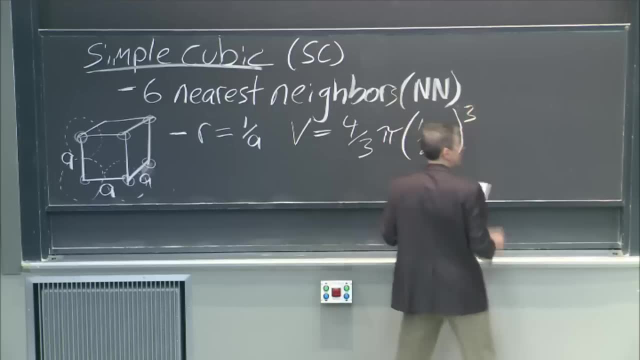 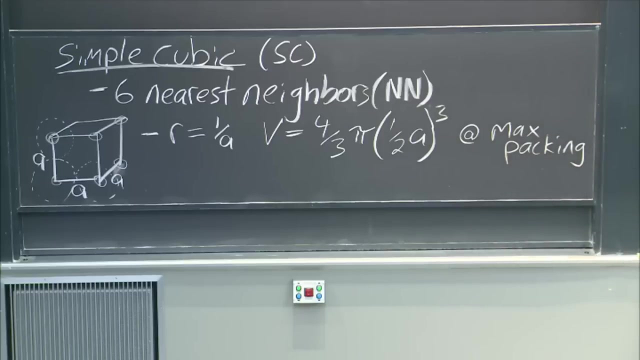 So radius is a half A, Volume is 4 thirds pi a half A cubed. All right, Now, this is important- That is at the max packing, OK. So I've grown these volumes out And I've seen what the packing can be. 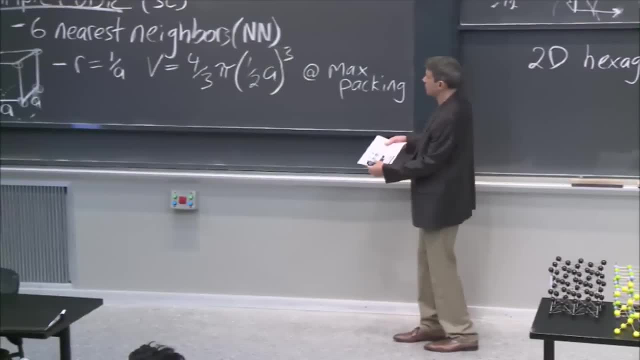 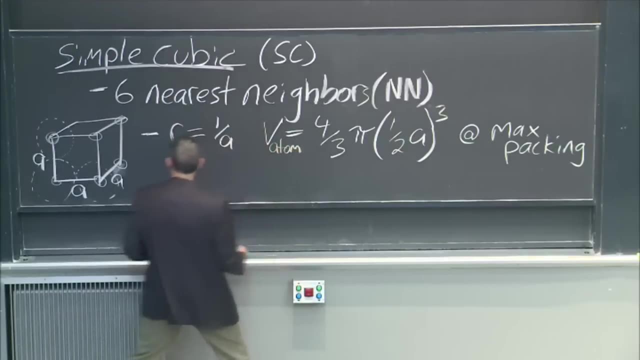 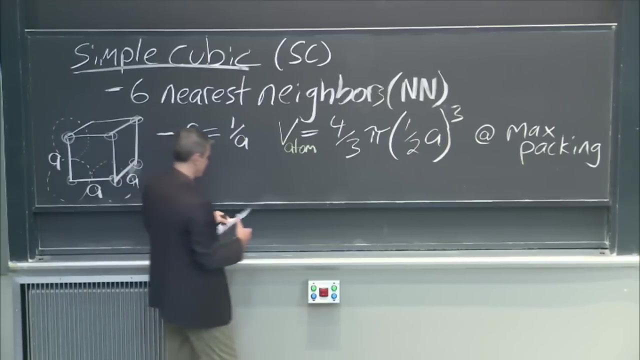 Now we actually call this Now. so now I've got the volume of an atom. I'm pretending that these are atoms now. No, I'm not pretending anymore, It's real. These spheres are now atoms, And OK, so that's the volume of the atom, right? 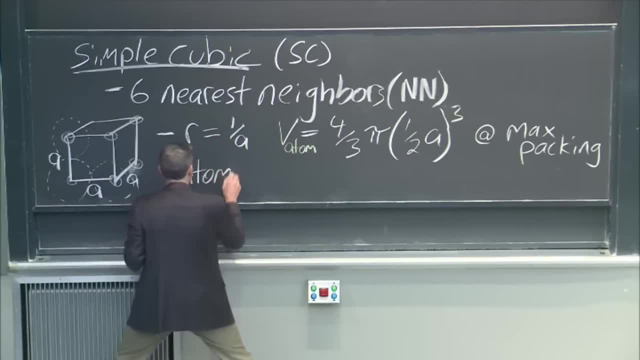 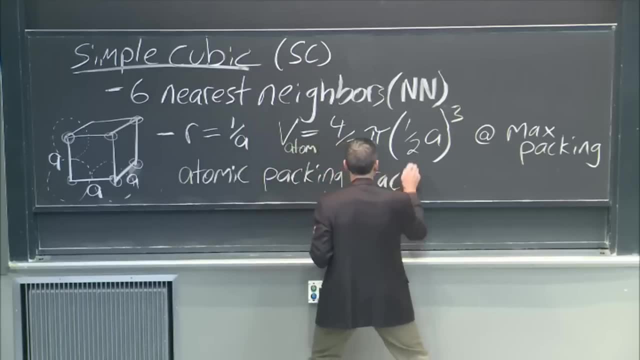 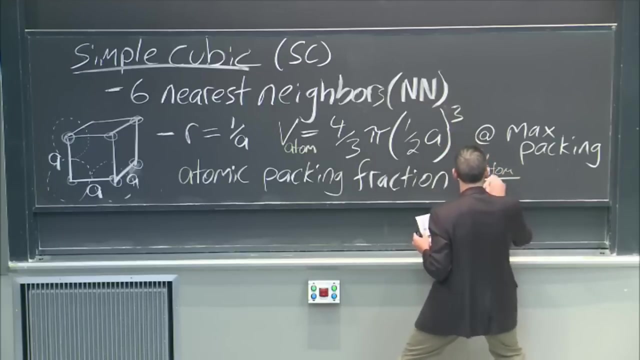 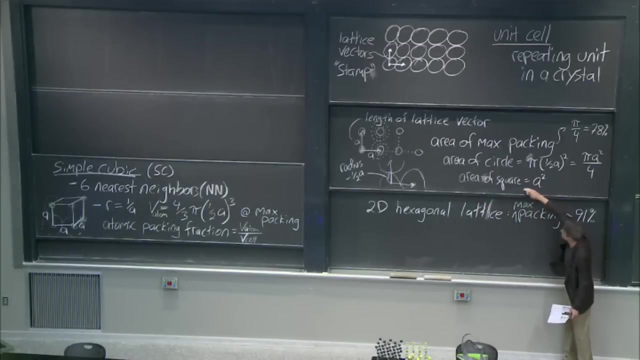 And so we can write: atomic packing fraction. Atomic packing fraction now Right, As the volume of the atom over the volume of the cell. Well, that's exactly what I did up here, right? That's how we got the area of the square. 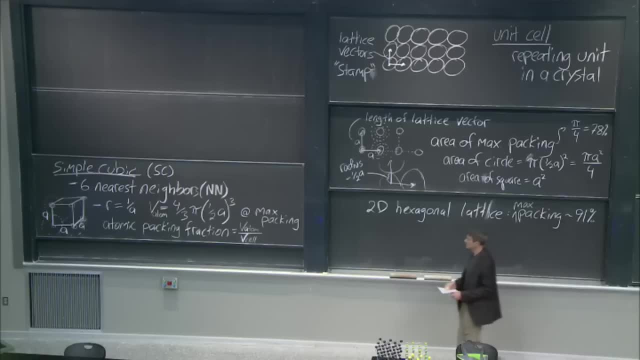 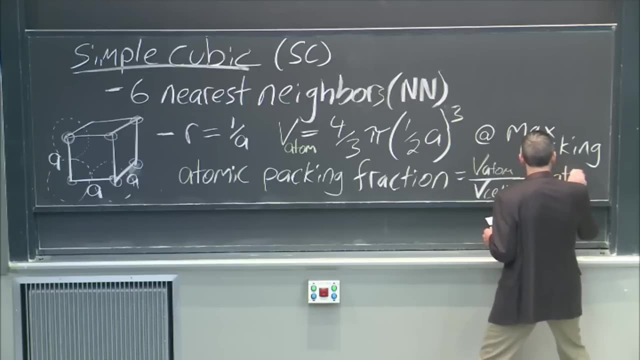 the area of the circle right. But there's one more thing that's really important, which is it has to be times the number of atoms in the cell. When I say cell, I mean unit cell, Right, It has to be times the number of atoms in the unit cell. 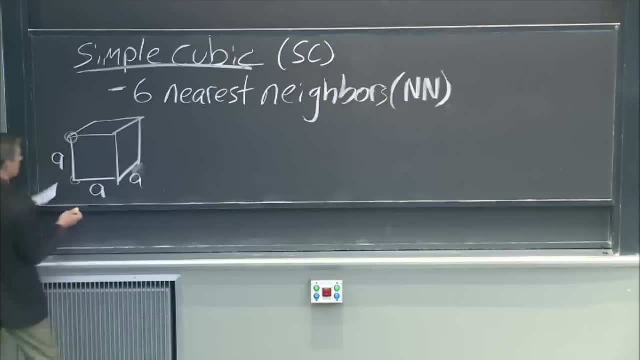 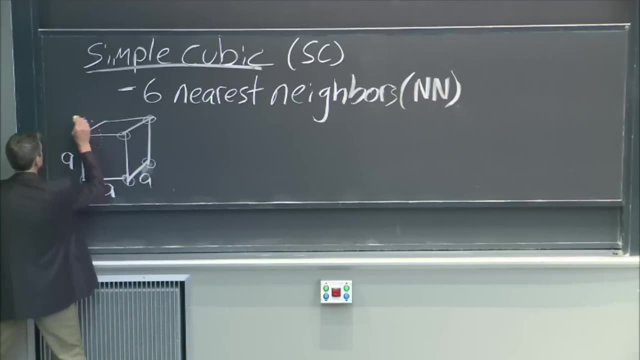 Now, OK, here we go, This one. Oh, but see, I want maximum packing, So I'm going to grow them out And you can see what's going to happen right as I do that. And so you can see that in the case of a simple cubic lattice. 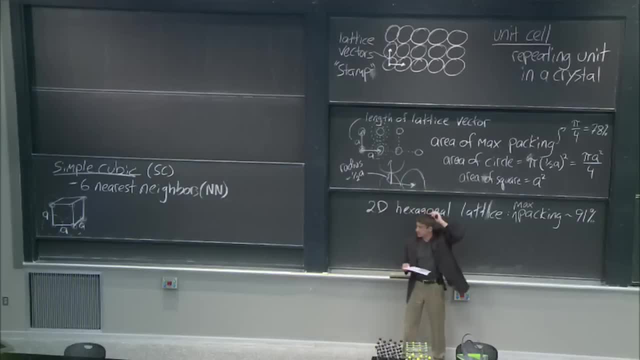 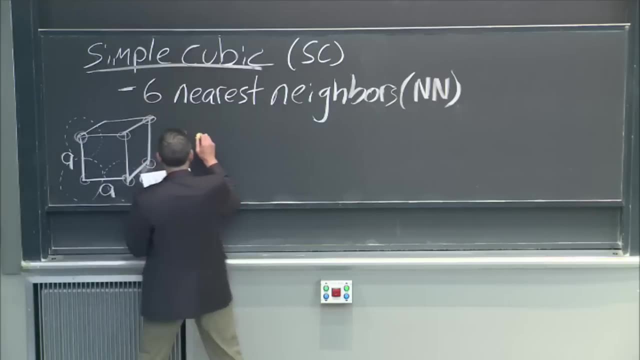 it's just like in the square lattice. It's just like in the square lattice right, When I've grown out the sphere, the radius of that sphere, the radius is r equals now, oh, wait, a second. OK, so I have 4 thirds pi or q. 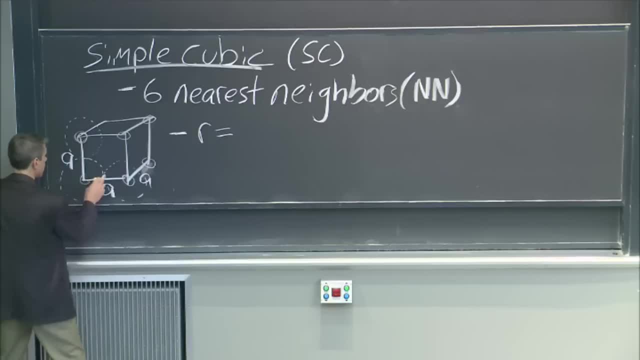 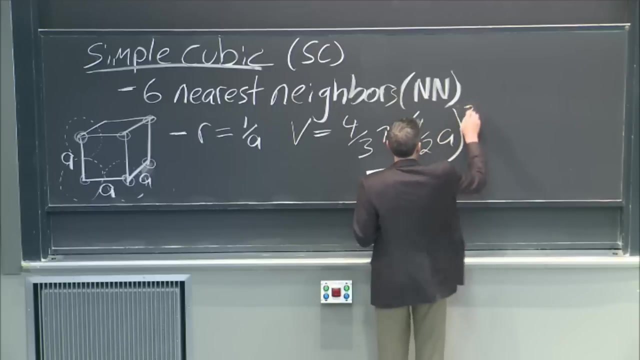 OK, but it doesn't matter yet. Don't do volume. Think about the radius. OK, the radius is just going to be a half, It's going to be a half the lattice right. So radius is a half A Volume is 4 thirds pi a half A cubed. 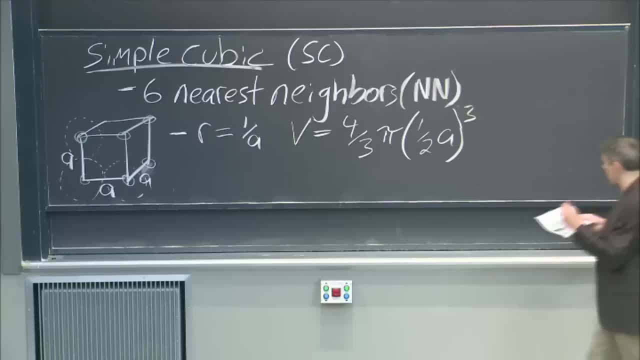 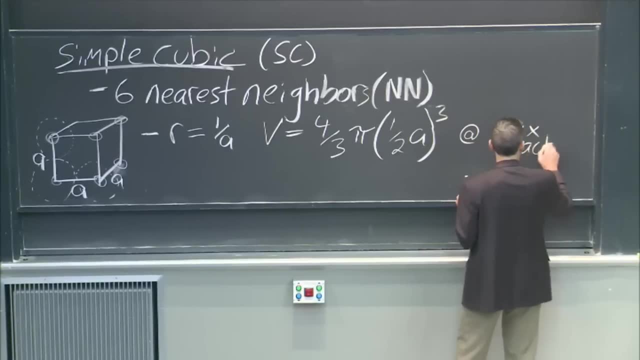 All right, Now, this is important. That is at the max packing, OK. So I've grown these volumes out And I've seen what the packing can be. Now we actually call this Now. so now I've got the volume of an atom. 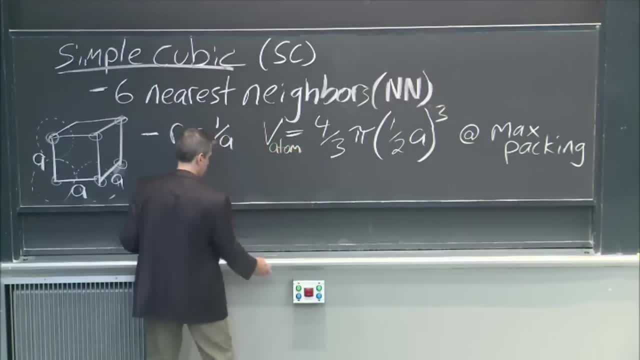 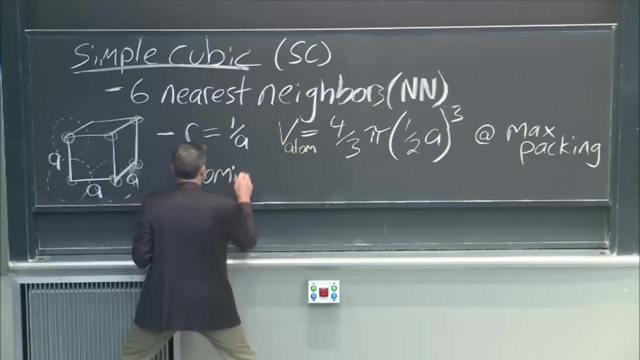 I'm pretending that these are atoms now. No, I'm not pretending anymore. It's real. These spheres are now atoms, And OK, so that's the volume of the atom, right? And so we can write: atomic packing fraction: atomic packing fraction now. 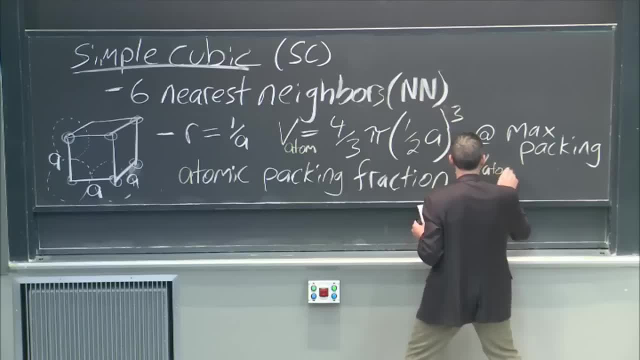 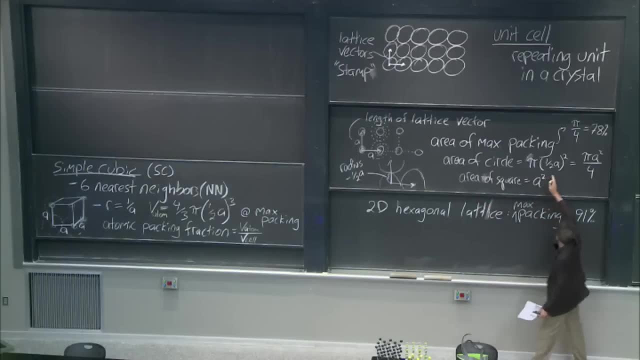 Right as the volume of the atom over the volume of the cell. Well, that's exactly what I did up here, right? That's how we got right the area of the square right, the area of the circle right. 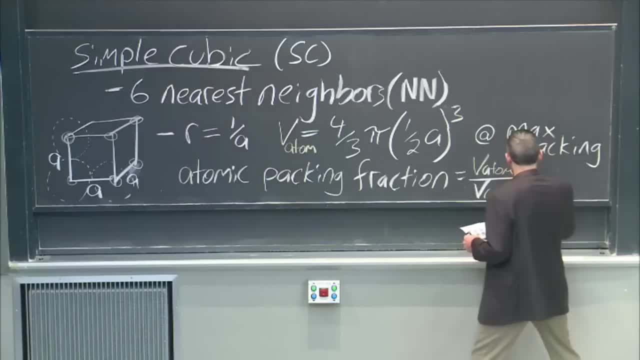 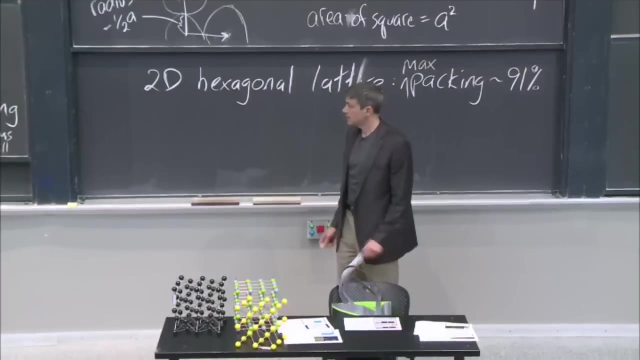 But there's one more thing that's really important, which is it has to be times the number of atoms in the cell. When I say cell, I mean unit cell. It has to be times the number of atoms in the unit cell, right. 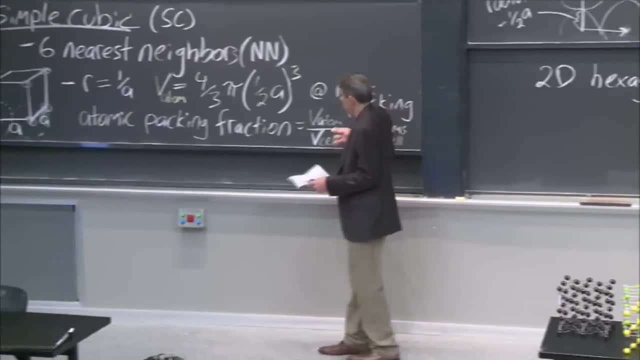 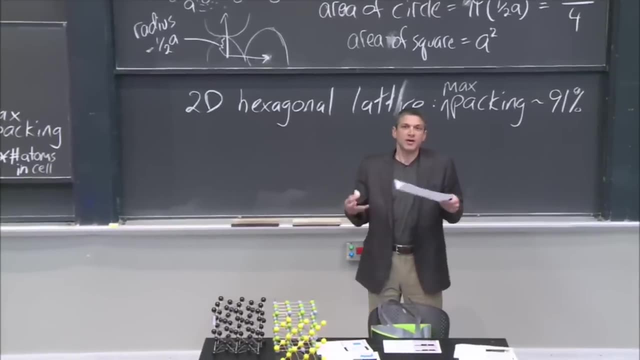 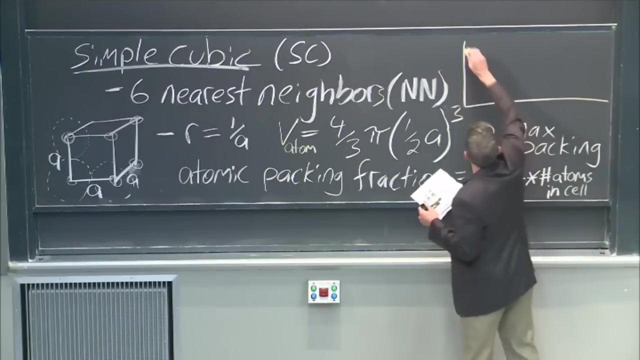 Right. So it's however many atoms I have, times the volume of the atom. OK, that's good. That's how much is inside of the cell divided by the volume of the cell And that gives me the atomic packing fraction. So in the case of a simple cubic, the APF, right. 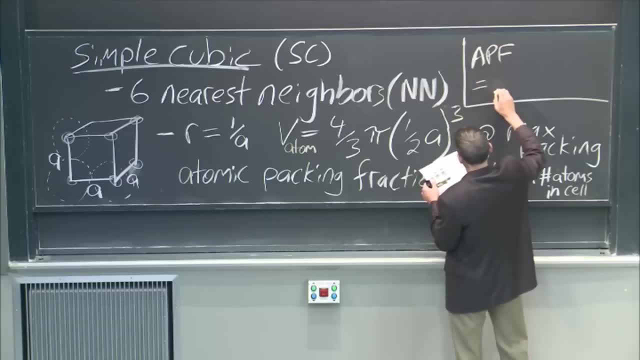 the atomic packing fraction is equal to, let's say, pi over 6,, which is 52%. That's not very good, All right, That's not well. I mean, it's relative. We don't know yet. 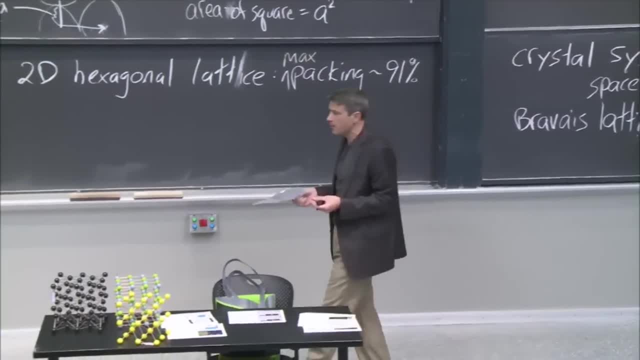 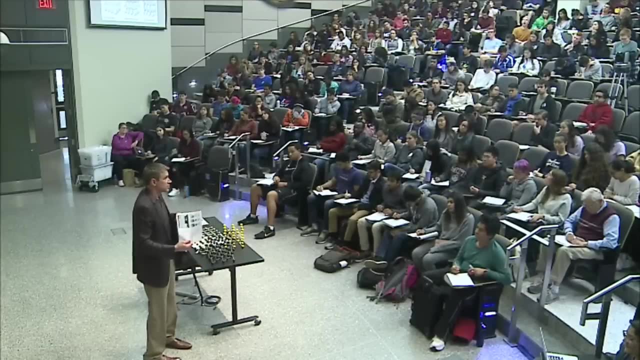 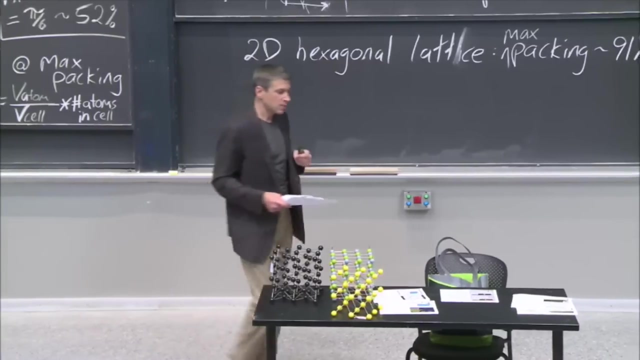 But it feels kind of low: 52%. So with a simple cubic lattice all I can do in my wildest dreams is cover 52% of that volume. That's not very that doesn't feel like a lot And in fact when you look at the periodic table, 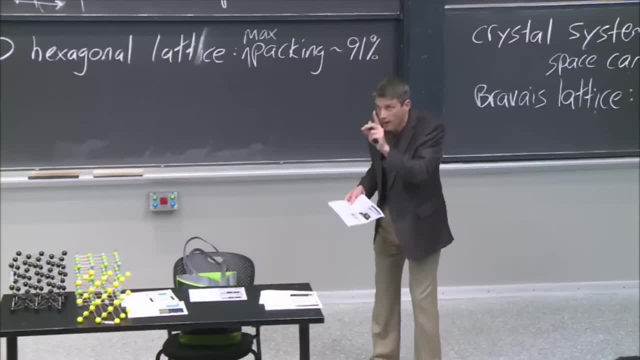 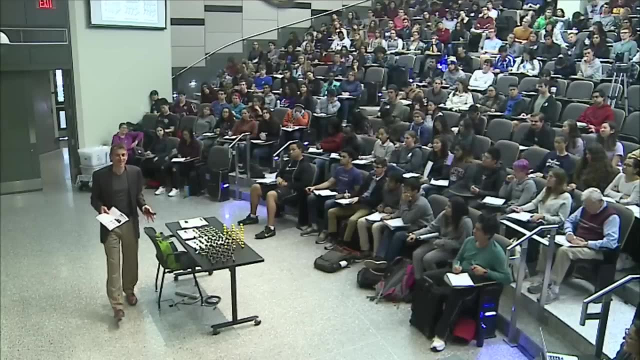 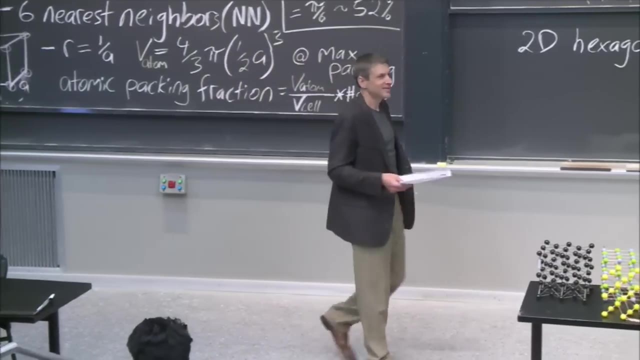 what you find is that there's only one element, one that takes the simple cubic lattice. Anybody know what it is? Of course It's polonium. Of course That's a really good conversation starter. I'm just saying. 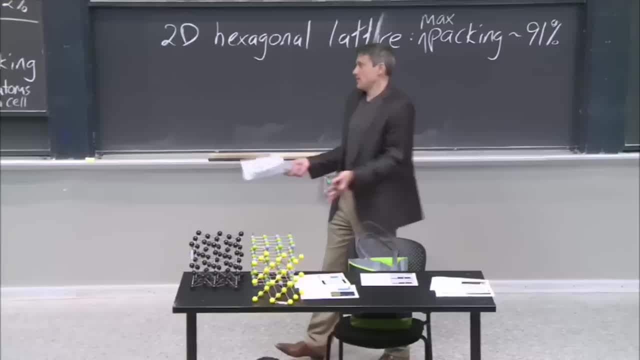 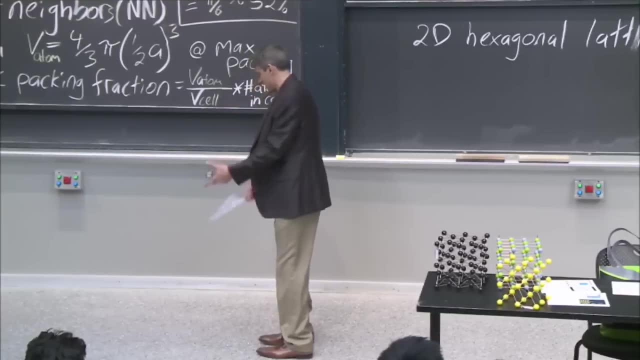 That is a great way to meet people. Which one? It's polonium. Why Relativity? Relativistic In polonium, those electrons, they're so high energy, Literally, they're so high energy, they're like close to the speed of light. 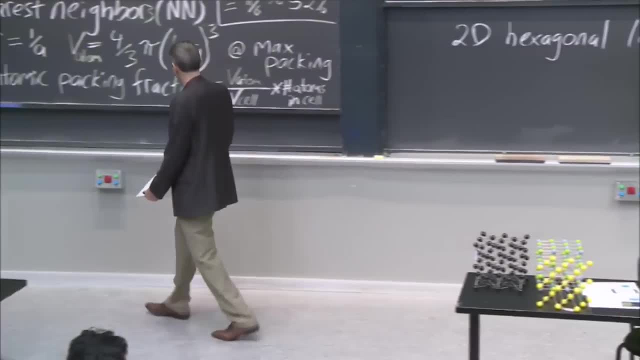 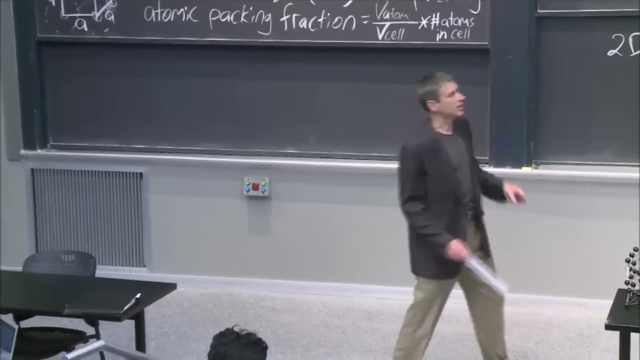 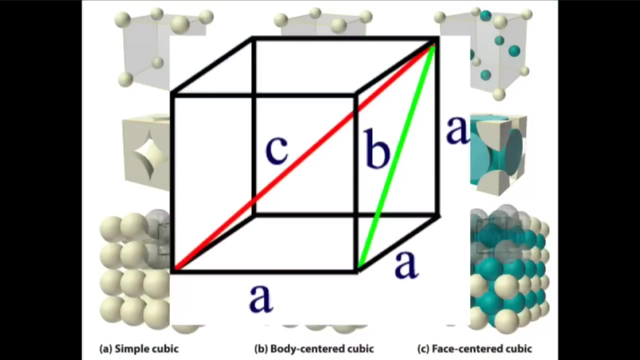 They're relativistic, Their mass is heavier. All sorts of interesting things happen. Polonium's the only one that goes simple cubic. I promised a video. Oh, there's a. oh, ha, a, a, a, There's a diagonal. 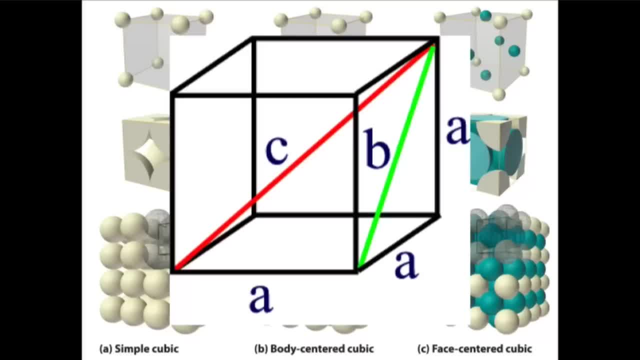 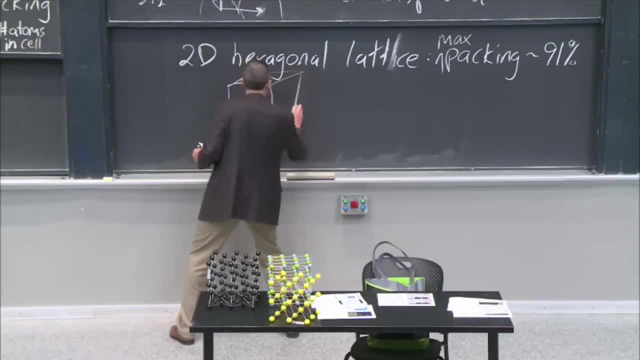 There's another diagonal. Oh, we're going to come back, We're going to come back to this. Let's draw that Because that might be important, right? So if I have a cube, then this diagonal, if that's a. 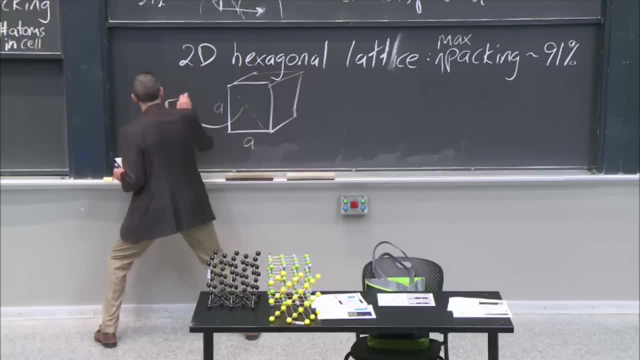 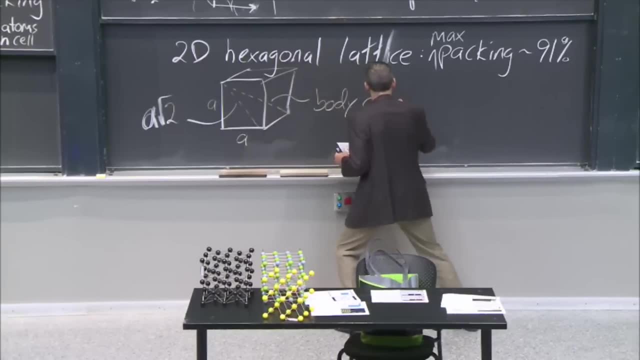 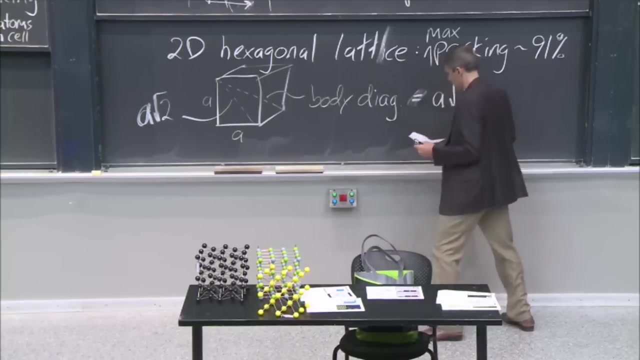 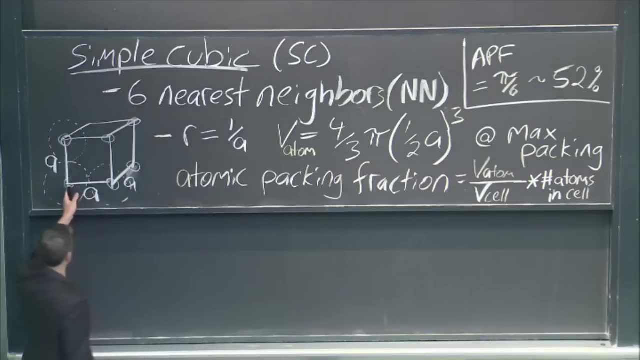 and that's a, then that is a root 2.. And the body diagonal- that's the body diagonal- is a root 3, not equals a root 3, right, OK, We'll come back. Oh, I didn't need that because this is just a over 2.. 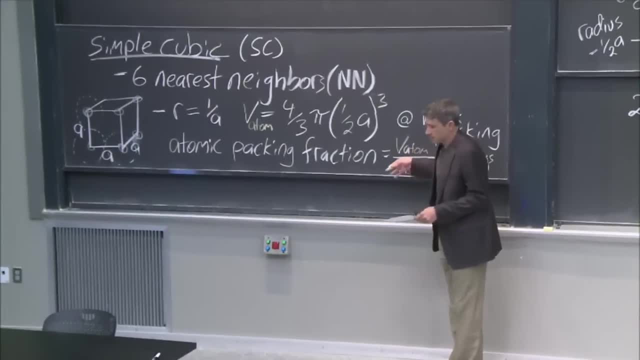 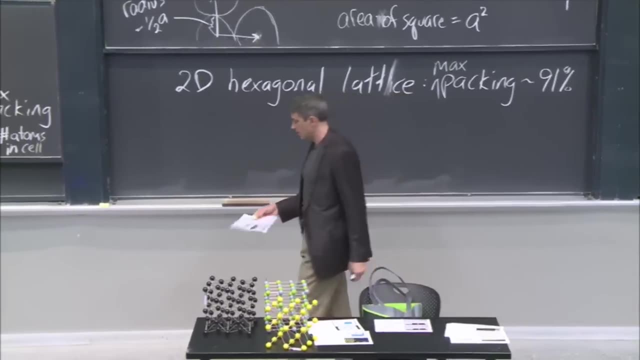 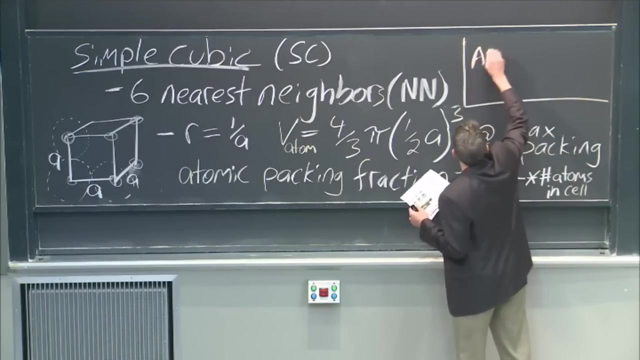 So it's however many atoms I have, times the volume of the atom. OK, that's good. That's how much is inside of the cell divided by the volume of the cell And that gives me the atomic packing fraction. So in the case of a simple cubic, the APF right. 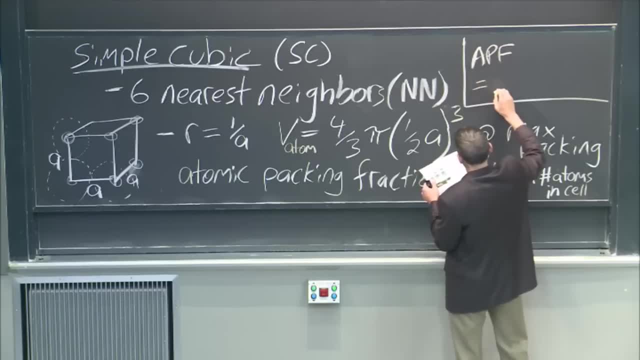 the atomic packing fraction is equal to ah pi over 6,, which is 52%. That's not very good. all right, That's not well. I mean it's relative, We don't know yet, but it feels kind of low, 52%. 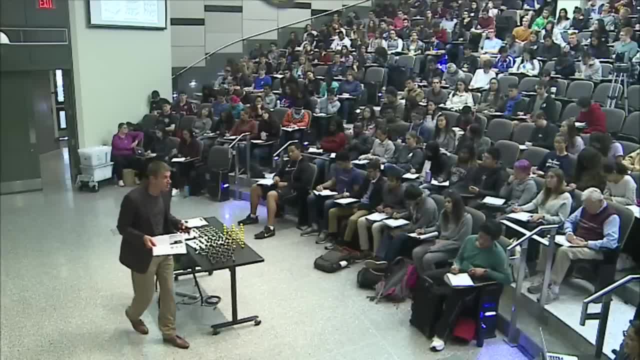 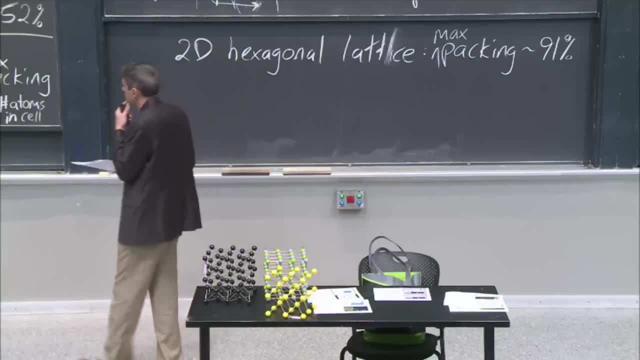 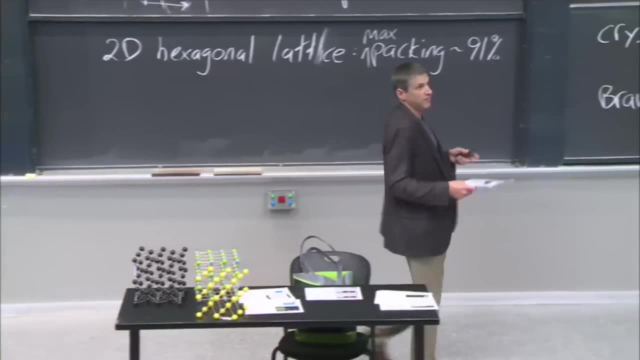 So with a simple cubic lattice, all I can do in my wildest dreams is cover 52% of that volume. That's not very. that doesn't feel like a lot, And in fact, when you look at the periodic table, what you find is that there's only one element, one. 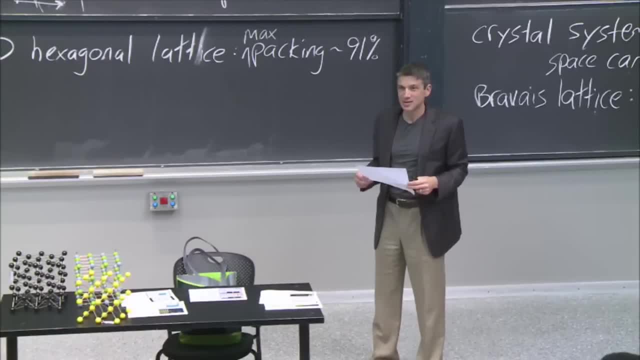 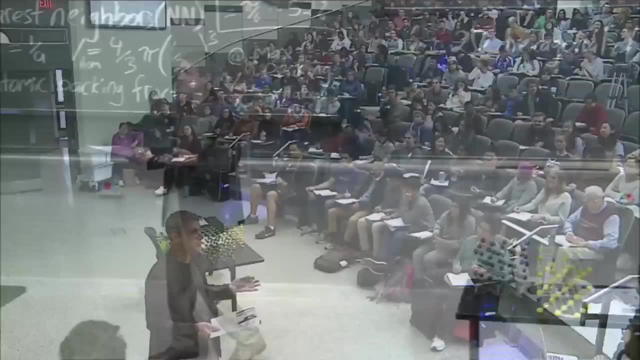 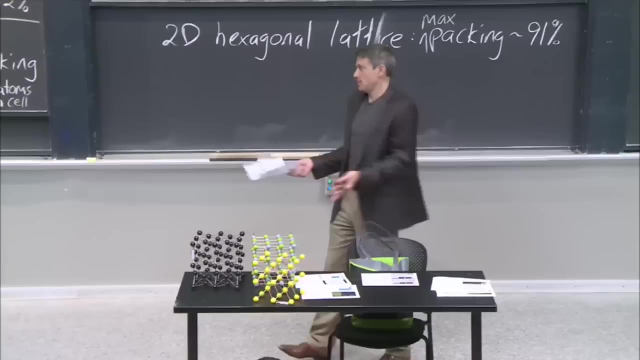 that takes the simple cubic lattice. Anybody know what it is. Of course It's polonium. Of course That's a really good conversation starter. I'm just saying That is a great way to meet people. Which one? It's polonium. 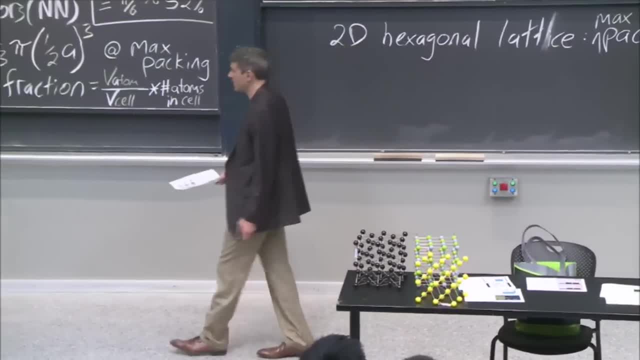 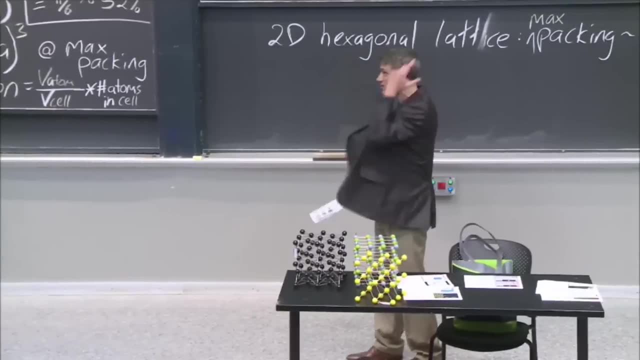 Why Relativity? Relativistic In polonium, those electrons, they're so high energy, Literally they're so high energy, they're like close to the speed of light. They're relativistic. Their mass is heavier. 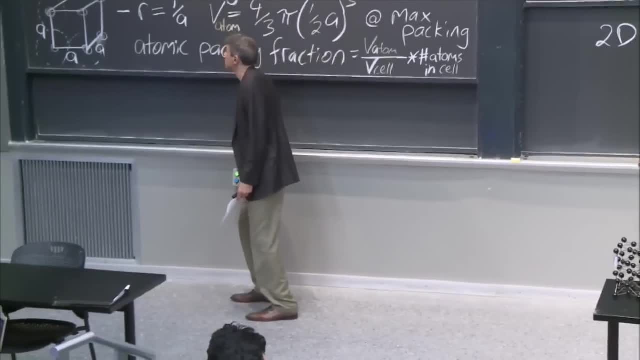 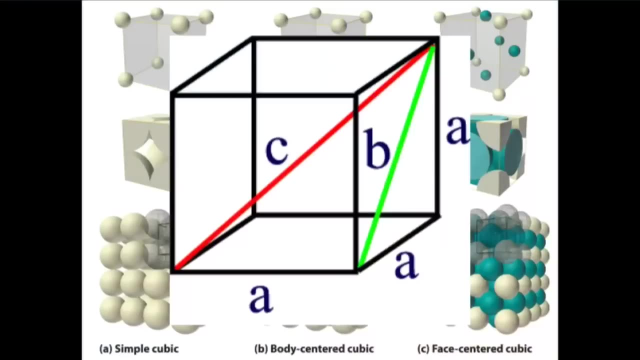 All sorts of interesting things happen. Polonium's the only one that goes simple, cubic. I promised a video. Oh, there's a, oh, ha, a, a, a. There's a diagonal, There's another diagonal, Oh. 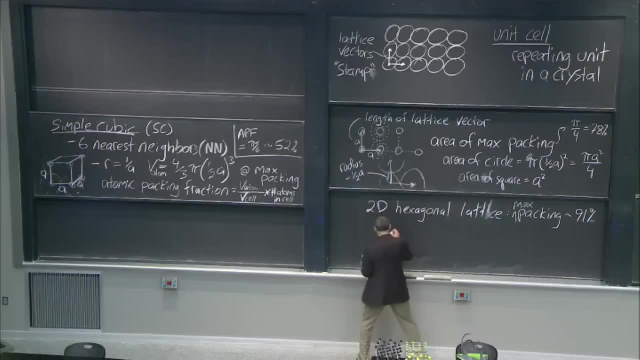 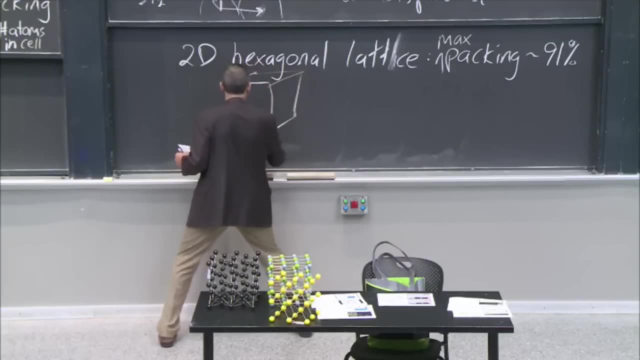 We're going to come back to this. Let's draw that Because that might be important, right? So if I have a cube, then this diagonal, if that's a and that's a, then that is a root. 2. And the body diagonal, that's the body diagonal. 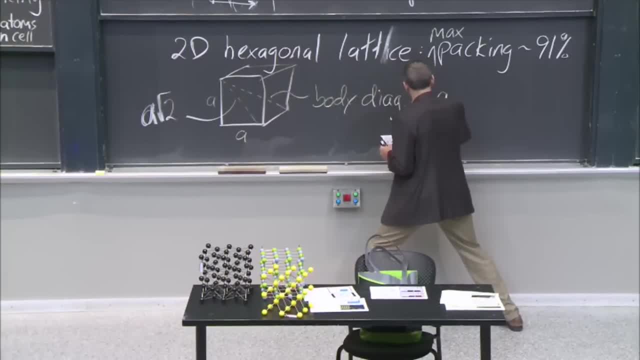 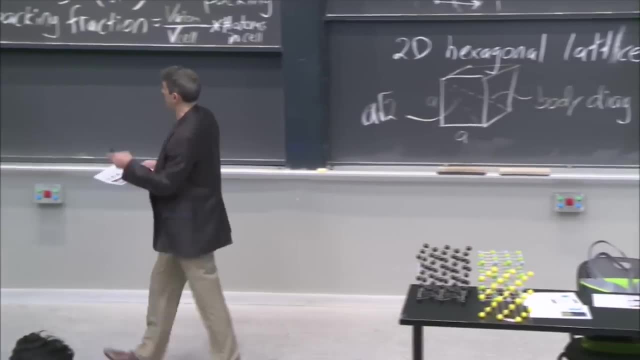 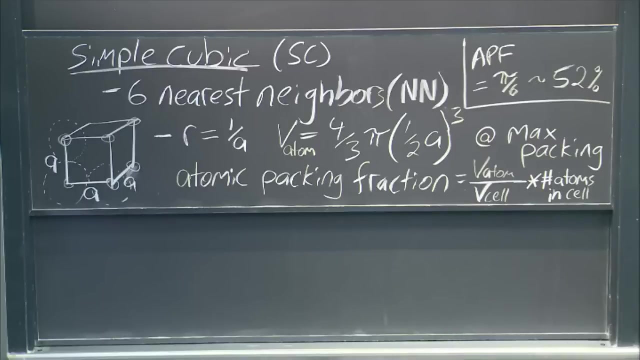 is a root 3, not equals a root 3, right, OK, We'll come back. Oh, I didn't need that because this is just a over 2.. But hold on, We're coming to it, But I promised a video first. 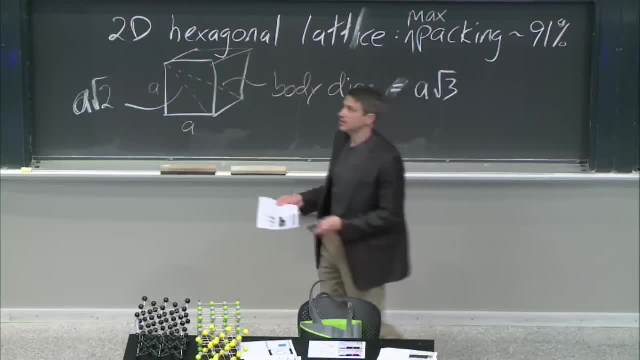 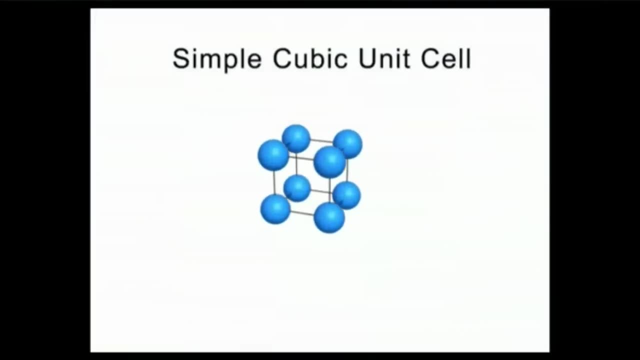 So here's a video with the laser coming in And you're going to really see this will come to life a little bit. Unique cells have particles at the corners of a cube. The simple or primitive cubic unit cell has particles at the corners only. 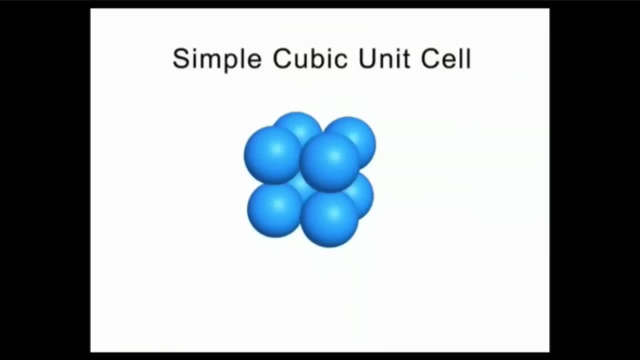 In reality, the particles lie as close to each other as possible. Note that the particles touch along the cube edges, but not along a diagonal in the face or along a diagonal through the body. By slicing away parts that belong to neighboring unit cells, we see that the actual unit cell consists. 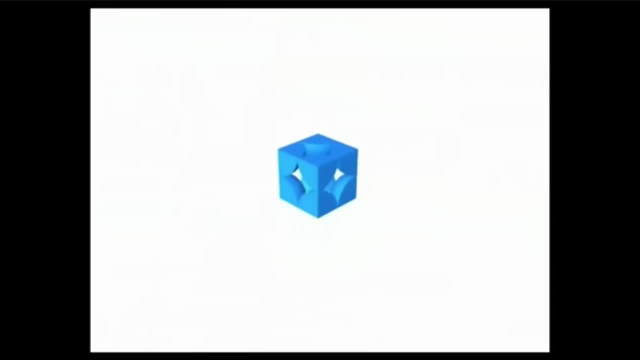 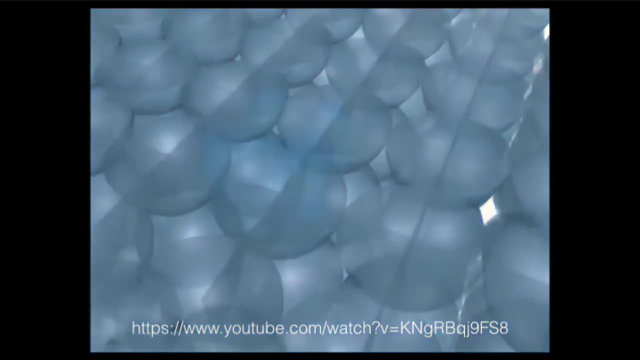 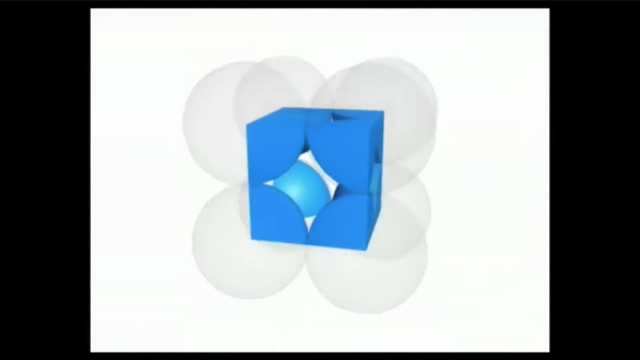 of portions of the particles. When the cells pack next to each other in all three dimensions, we obtain the crystal. If we fade the others out, we obtain the crystal. Note: you can see the original group of eight particles within the array and the unit cell within that group. 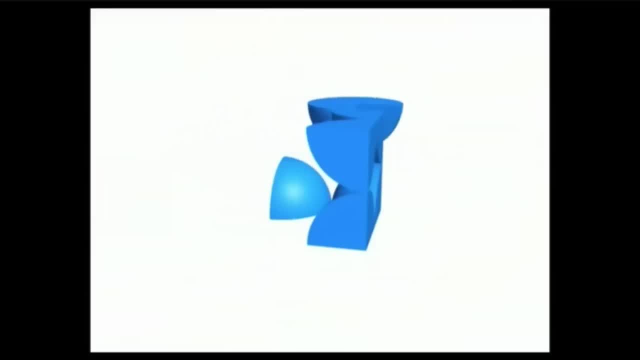 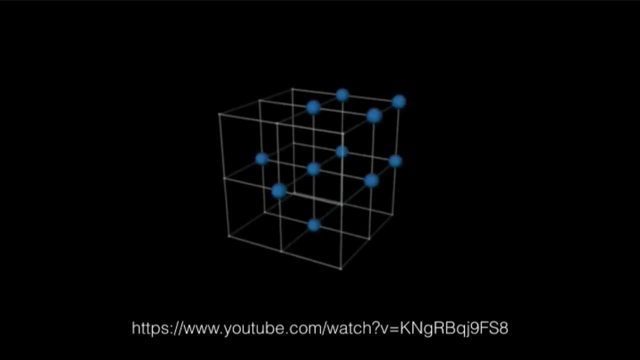 We find the number of particles in one unit cell by combining all the particles' portions In the simple cubic unit cell. eight corners, each of which is 1 eighth of a particle, combine to give one particle A key feature of a crystal structure. 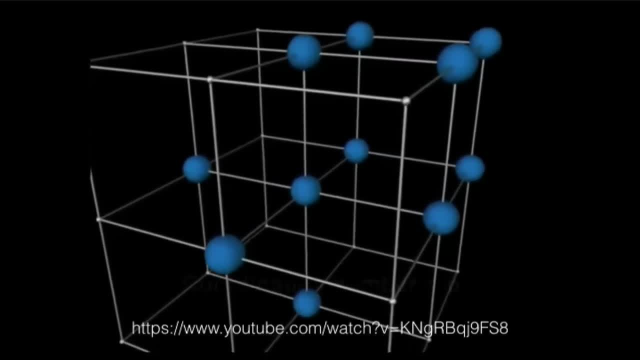 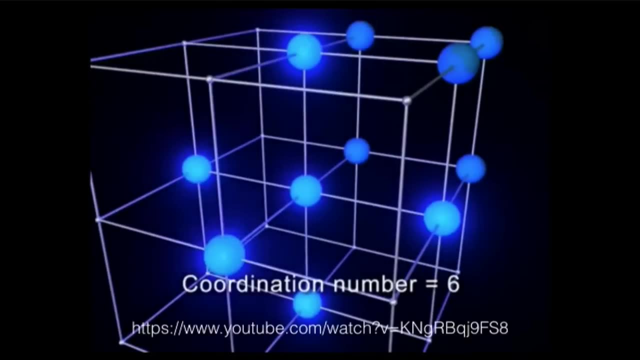 is its coordination number, the number of the nearest neighbors surrounding each particle. In a simple cubic array, any given particle has a neighboring particle above, below, to the right, to the left, in front and in back of it, for a total of six nearest neighbors. 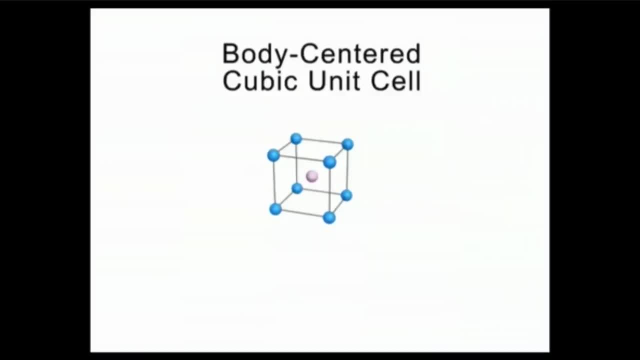 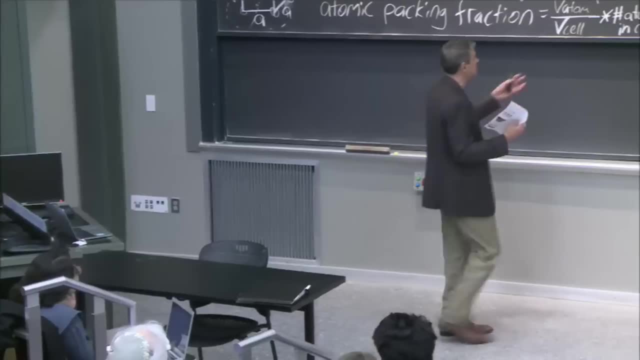 The body-centered cubic unit cell has a? OK. so you see how that's so cool, right? And you're figuring out how many atoms are in the cell, right? Well, Why don't you just put the atom in the middle? 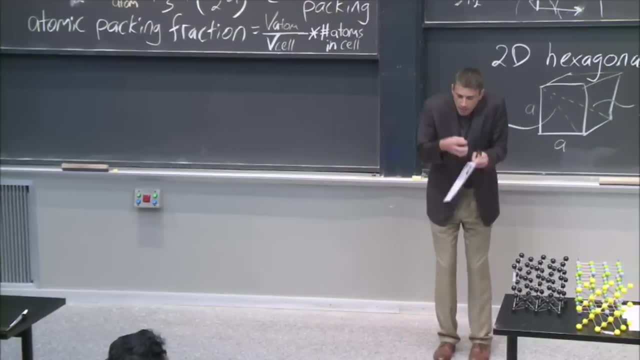 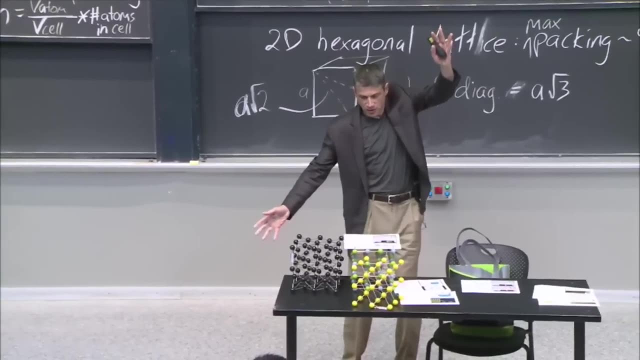 You can do that, but then it's not at the point, right. So you've got to understand. the concept of the lattice is that whatever I put here, wherever my vectors go, that's what I put there, right And there and then there. 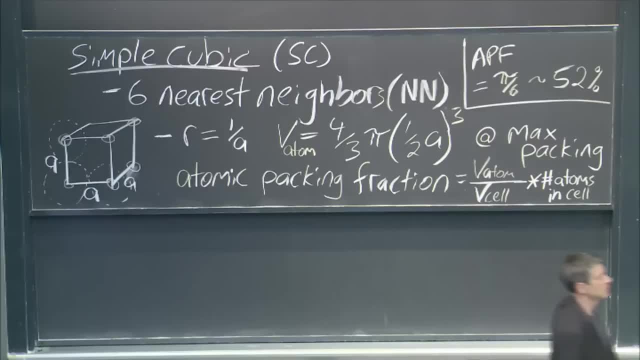 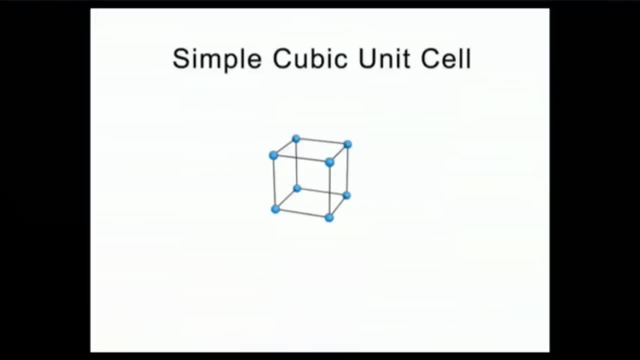 But hold on, We're coming to it, But I promised a video first, So here's a video with the laser coming in And you're going to really see this will come to life a little bit. Unique cells have particles at the corners of a cube. 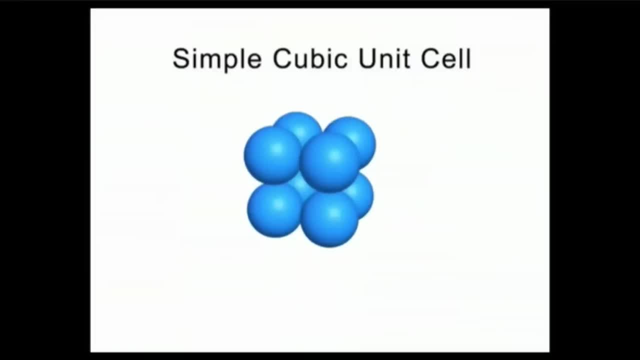 The simple or primitive cubic unit cell has particles at the corners only. In reality, the particles lie as close to each other as possible. Note that the particles touch along the cube edges but not along a diagonal in the face or along a diagonal through the body. 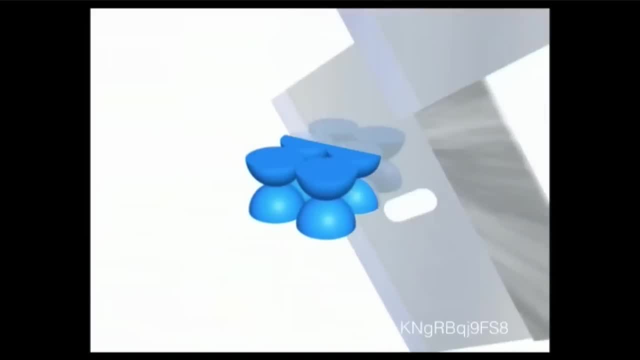 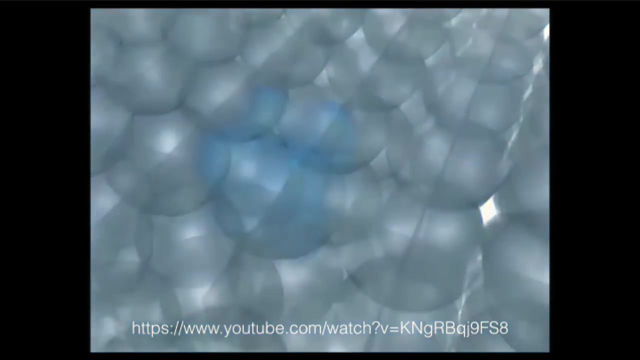 By slicing away parts that belong to neighboring unit cells, we see that the actual unit cell consists of portions of the particles. When the cells pack next to each other in all three dimensions, we obtain the crystal. If we fade the others out, you can. 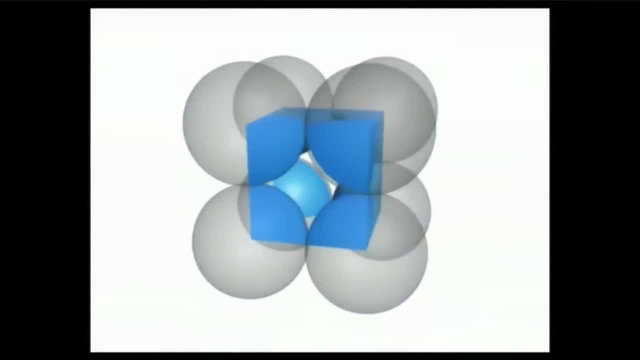 see the original group of eight particles within the array and the unit cell. within that group We find the number of particles in one unit cell by combining all the particles' portions In the simple cubic unit cell. eight corners, each of which is 1 eighth of a particle, combine to give one particle. 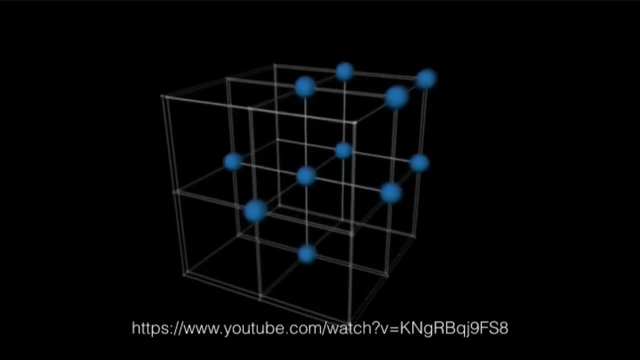 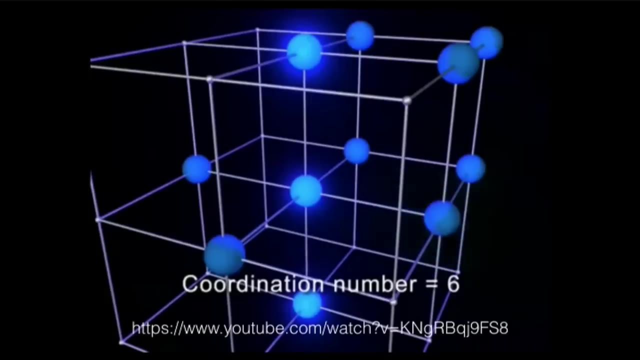 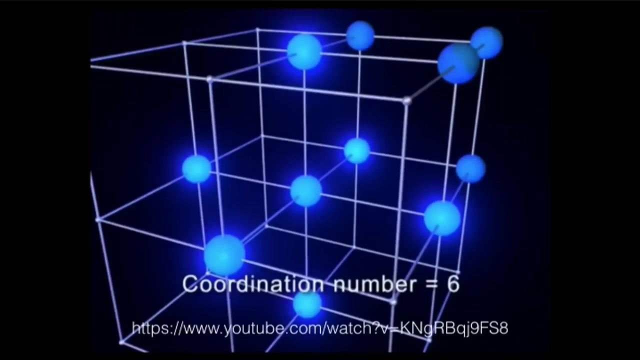 A key feature of a crystal structure is its coordination number, the number of the nearest neighbors surrounding each particle. In a simple cubic array, any given particle has a neighboring particle above, below, to the right, to the left, in front and in back of it. 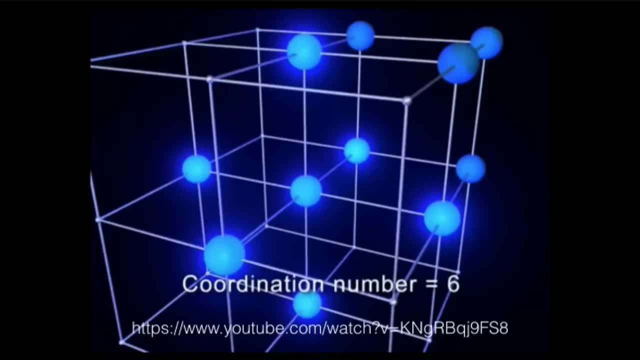 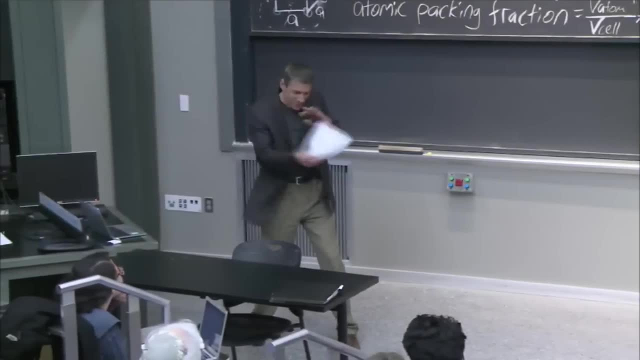 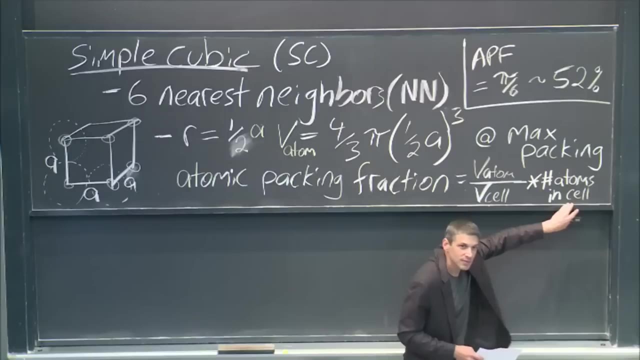 for a total of six nearest neighbors. The body-centered cubic unit cell has a OK. so you see how that's so cool, right? And you're figuring out how many atoms are in the cell, Right? Well, why didn't you just put the atoms in the cell? 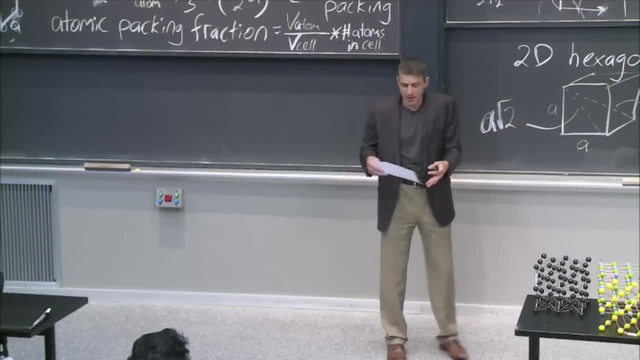 Why didn't you just put the atoms in the cell? Why didn't you just put the atom in the middle? You can do that, but then it's not at the point right. So you've got to understand the concept of the lattice. 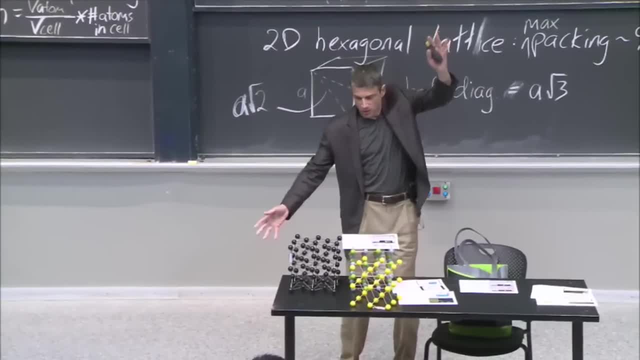 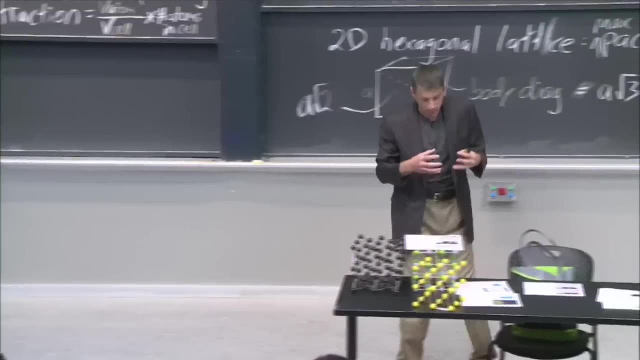 is that whatever I put here, wherever my vectors go, that's what I put there, right And there and then there. And so we often, as a standard, we say, well, OK, what did I put there? I put an atom right. 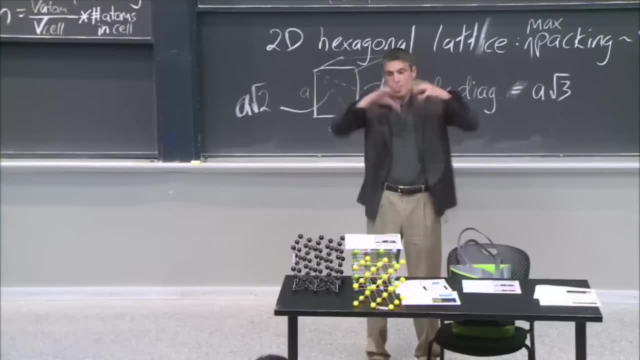 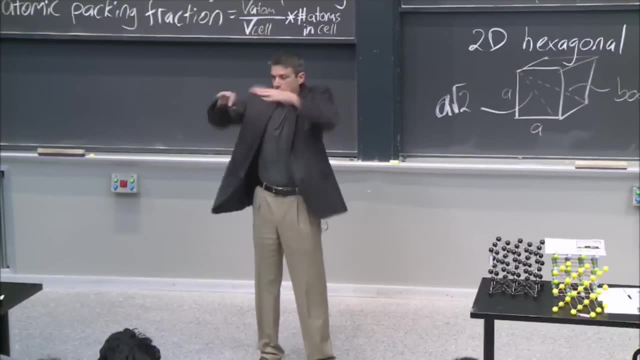 And so we often, as a standard, we say, well, OK, what did I put there? I put an atom right And then I put another atom, But then your unit cell is that cube. And so we cut the unit cell and you're like: well. 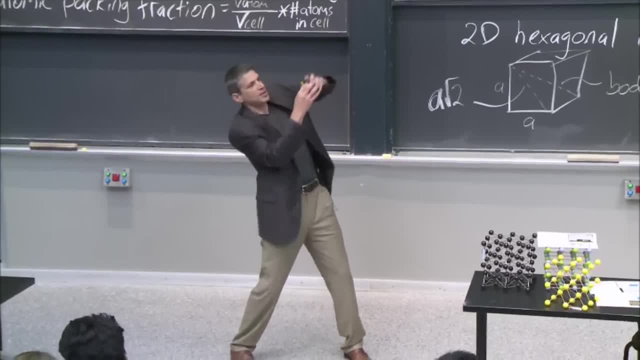 how many atoms do I have in it? Well, let's see, I got one here, but it's shared with all these other cubes. So there's an eighth of an atom there, right, And an eighth of an atom there. we add them all up. 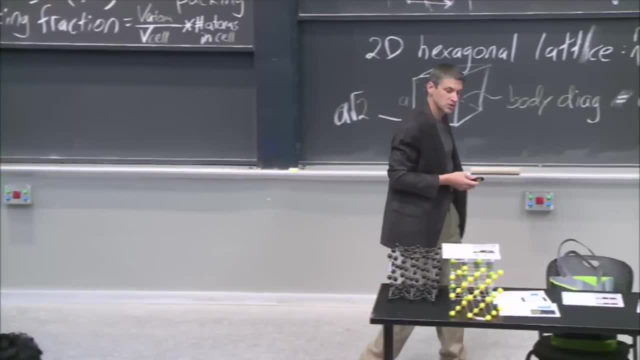 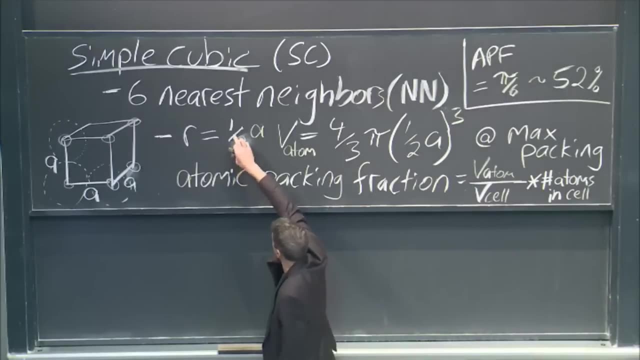 and you get one atom right back, which you knew, Which you knew, And, by the way, this was not 1 over a, It was. I wrote it mistakenly as 1 over a. The radius is a half a OK over there. 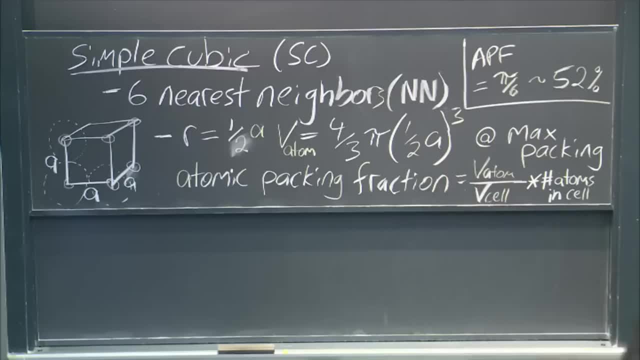 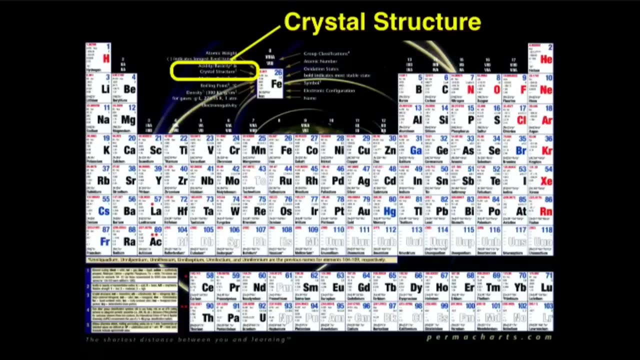 All right, which is correct here. OK, good, Now next crystal structure. Oh look, How do you know what crystal structure? And there it is. right there, It's the periodic table. To the rescue again. He had it right there. 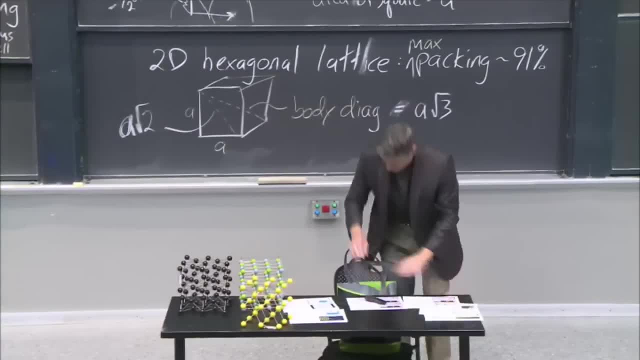 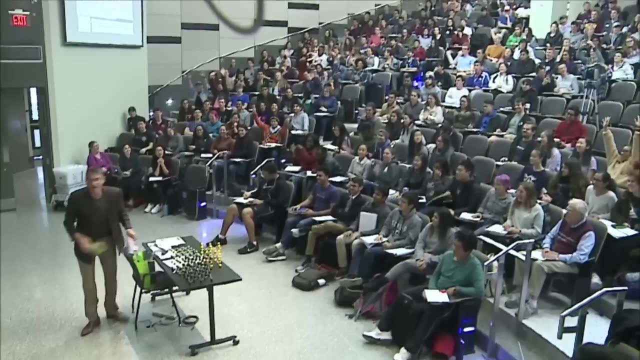 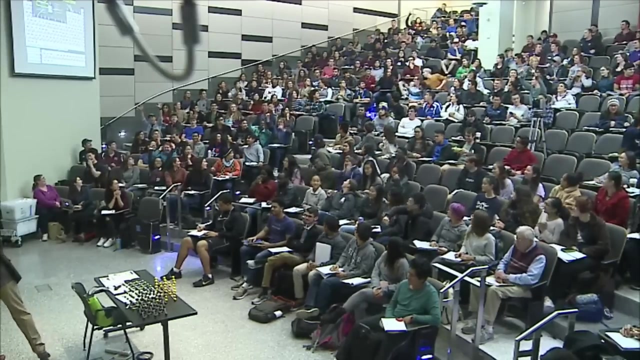 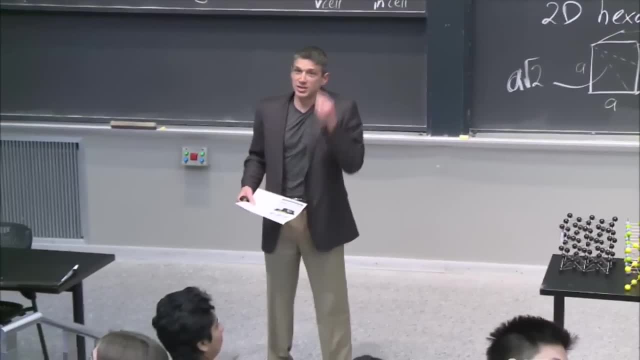 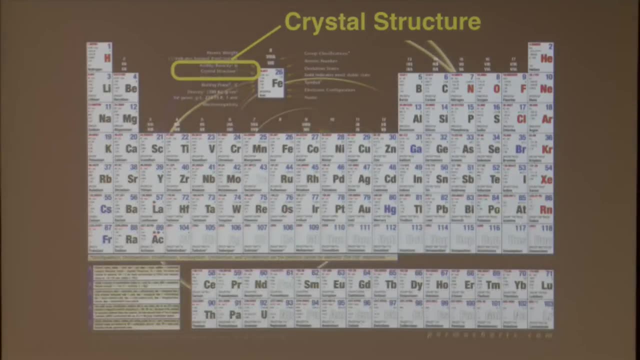 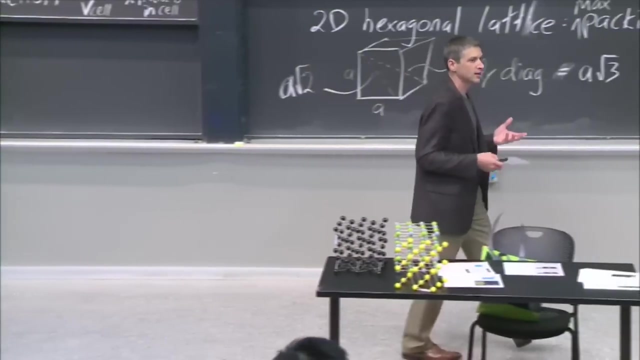 I know Which one is: simple cubic Polonium. It's only polonium. There it is Polonium. Thank you for being representative of simple cubic crystals, But now we're talking about the next kind, which is body-centered cubic. 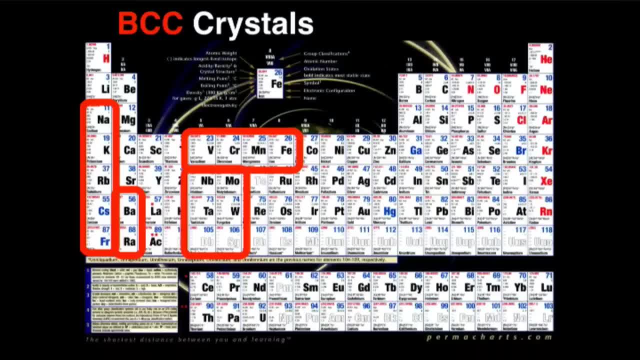 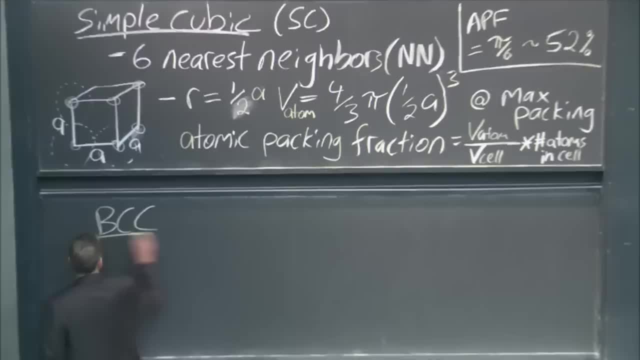 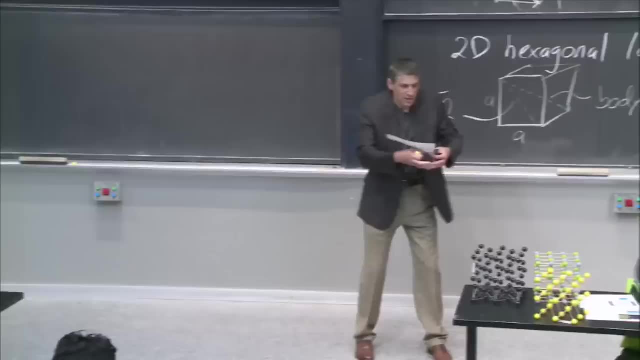 And look A lot more. I have a body-centered cubic And here here, OK, so if it's BCC, body-centered cubic, well now you know, if I take these atoms at these corners and I add: now there's a lattice that takes me to the middle. 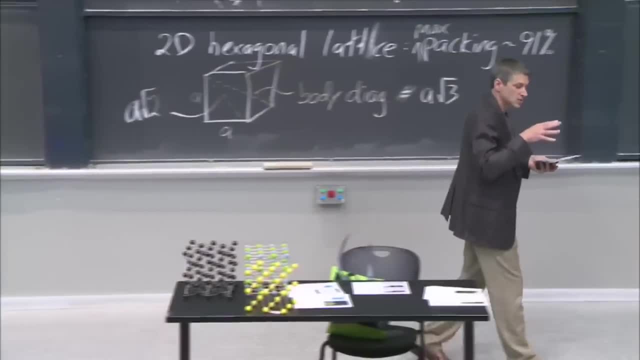 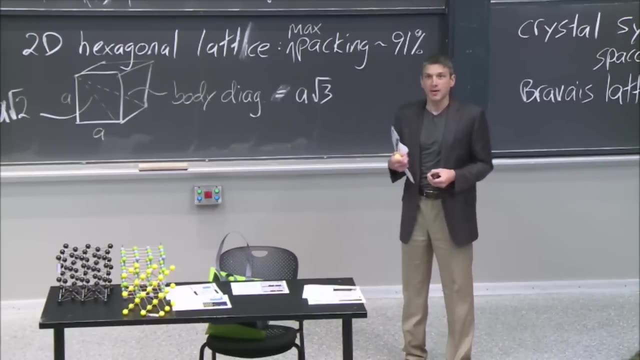 Remember, my lattice is giving me this symmetry. My lattice is giving me this. So it means: whatever I put here, I put it all the corners and I put it in the middle. right, That's BCC. That's what BCC means. 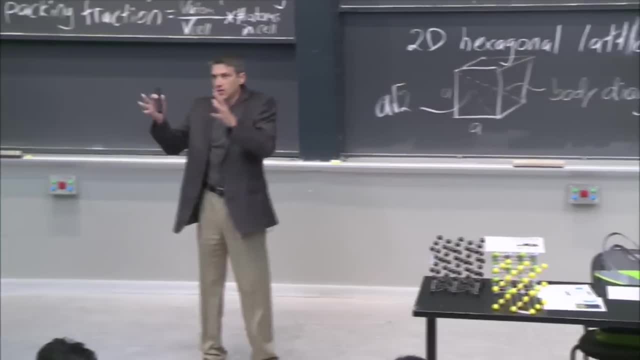 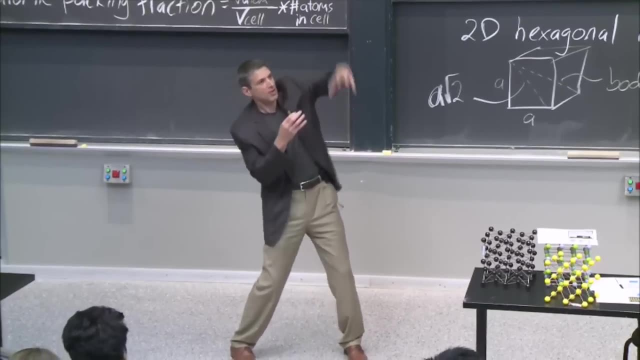 And then I put another atom, But then your unit cell is that cube, And so we cut the unit cell and you're like: well, how many atoms do I have in it? Well, let's see, I've got one here, but it's shared. 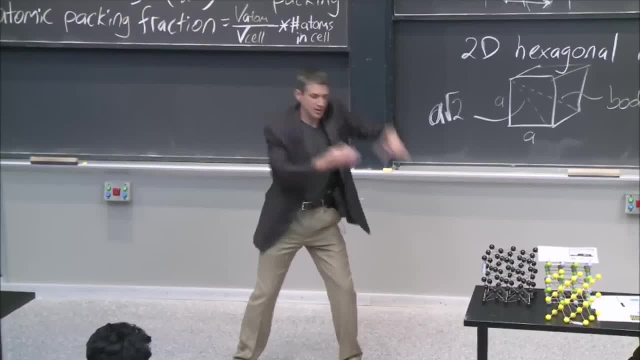 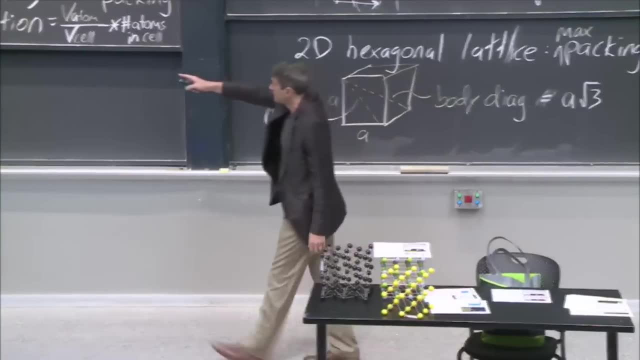 with all these other cubes. so there's an eighth of an atom there right And an eighth of an atom there. we add them all up and you get one atom right back, which you knew, Which you knew. And, by the way, this was not 1 over a. 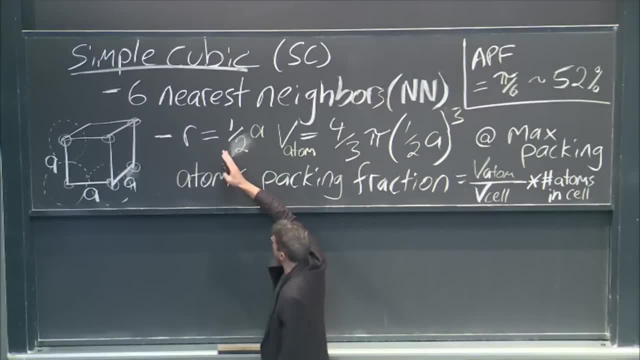 It was. I wrote it mistakenly as 1 over a. The radius is a half a. OK, over there. All right, which is correct here? OK, good, Now next crystal structure. Oh look, How do you know what crystal structure? 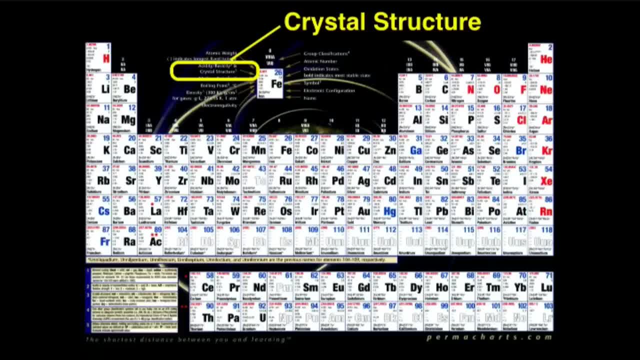 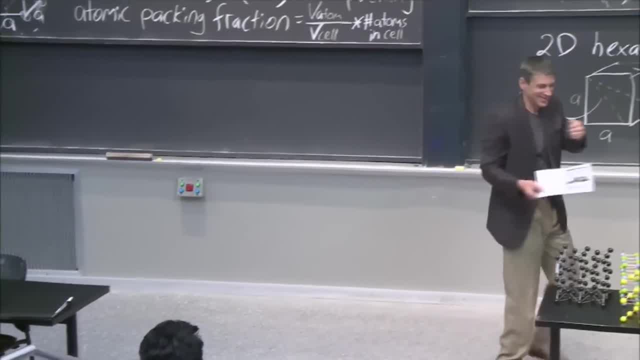 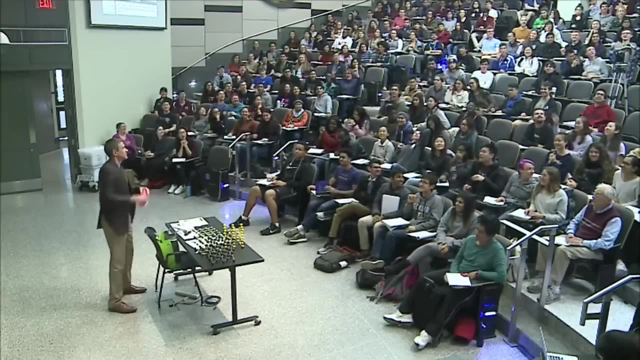 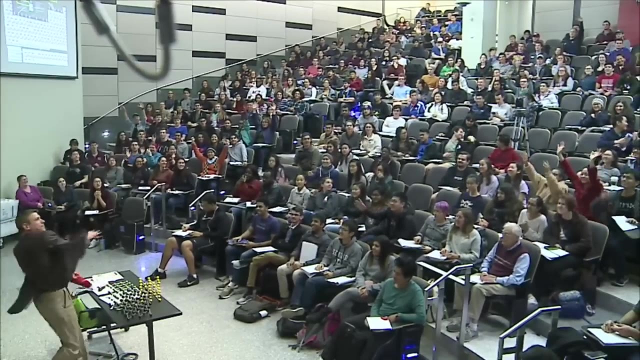 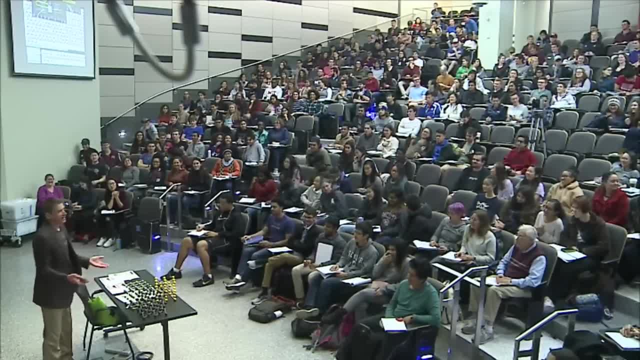 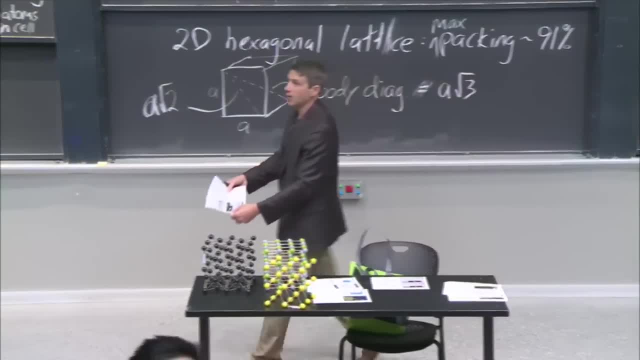 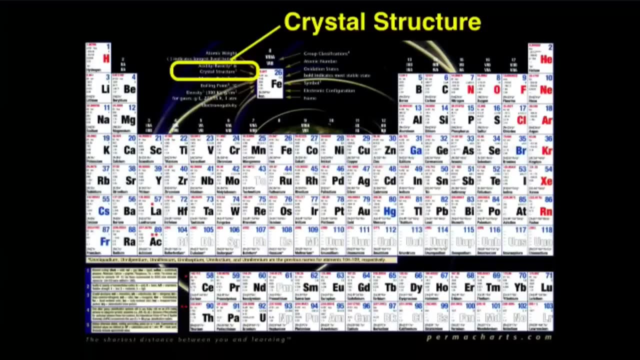 and up there We'll bring more. You bring a periodic table like that. what is a crystal symmetry? I know Which one is simple cubic Polonium. It's only polonium. There, it is polonium. Thank you for being representative. 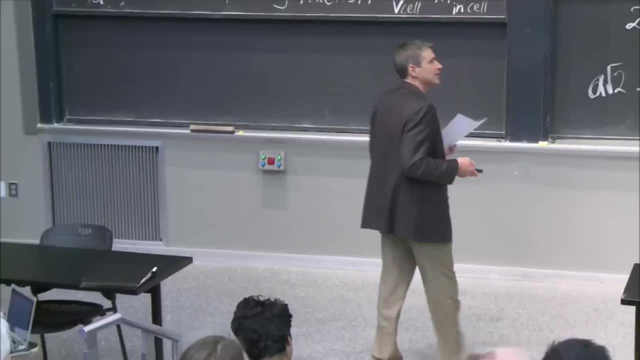 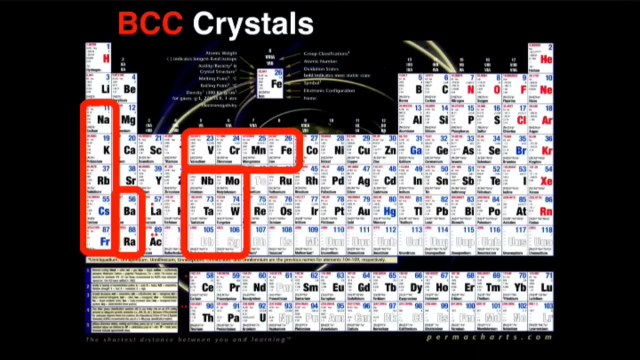 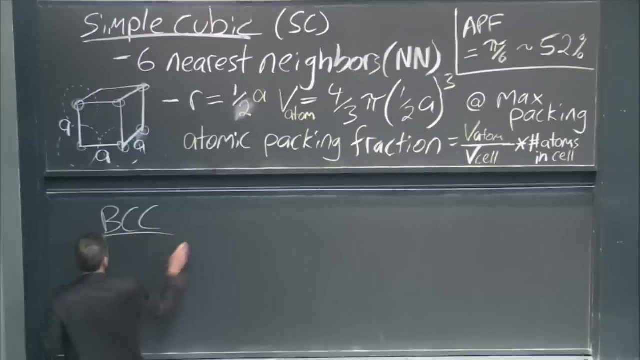 of simple cubic crystals, But now we're talking about the next kind, which is body-centered cubic. And look a lot more. I have a body-centered cubic and here here: OK, so if it's BCC- body-centered cubic, well now 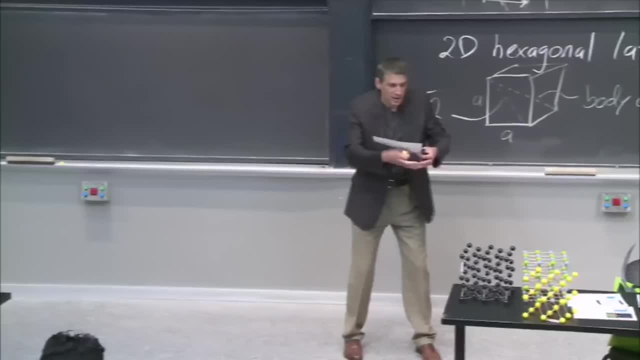 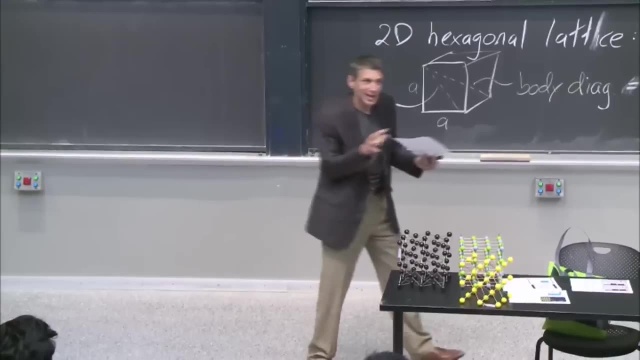 you know, if I take these atoms at these corners and I add: now there's a lattice that takes me to the middle, Remember, my lattice is giving me this symmetry, My lattice is giving me this. So it means whatever I put here. 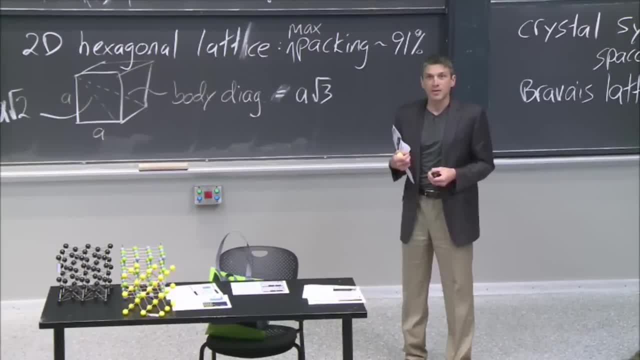 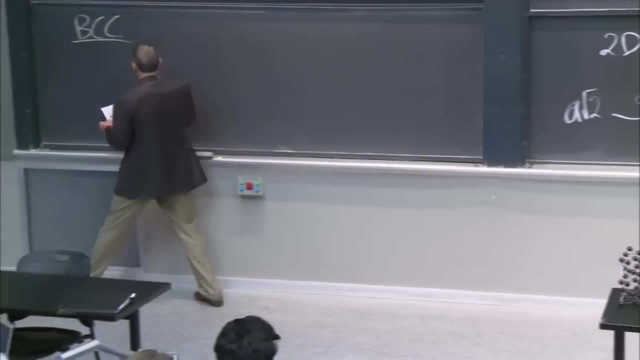 I put it all the corners and I put it in the middle, right, That's BCC. That's what BCC means. Well, if you grow that, OK, so first of all, eight nearest neighbors, right, Eight nearest neighbors. 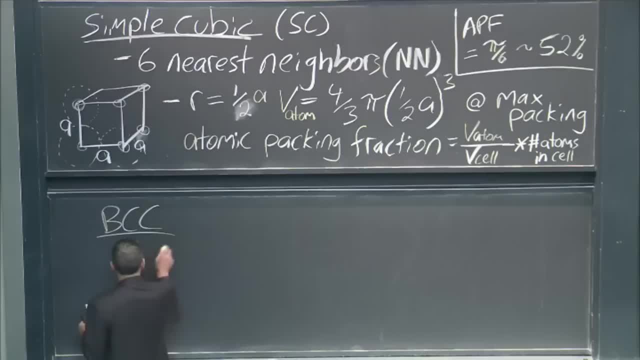 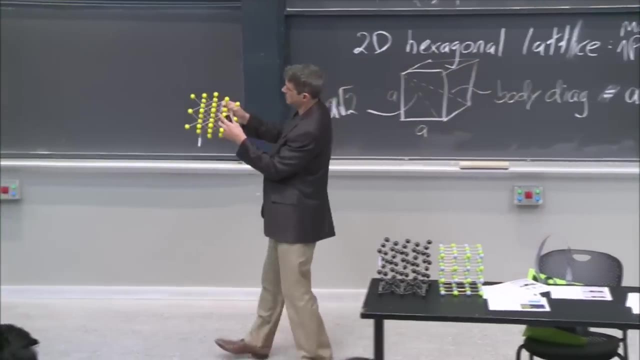 Well, if you grow that, OK, so first of all, eight nearest neighbors, right, Eight nearest neighbors? Well, you can see that, because I've got the six, but then I've got these ones here, right, I've got. actually it's not the six. 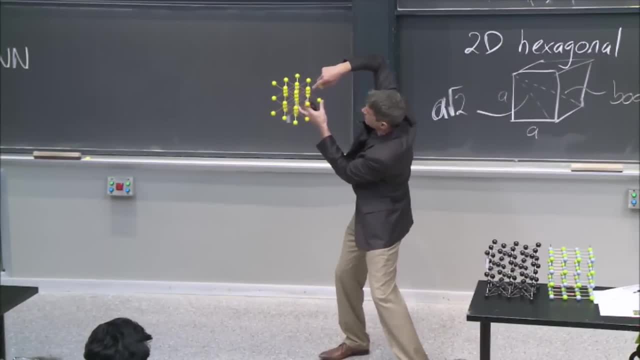 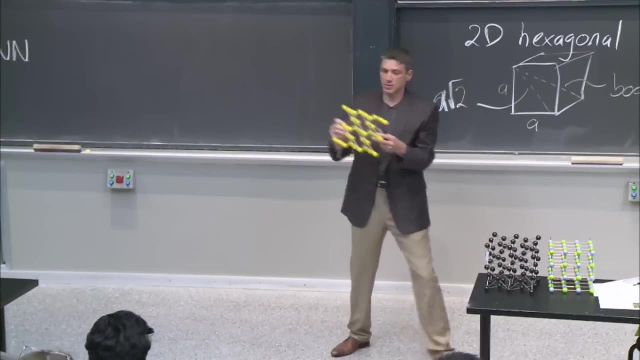 I've got the one along the diagonal, which is kind of the point I wanted to make. next This: oh, this is BCC, This is BCC right Now. how do you see that it's BCC? Because you stare at it and you stare at it. 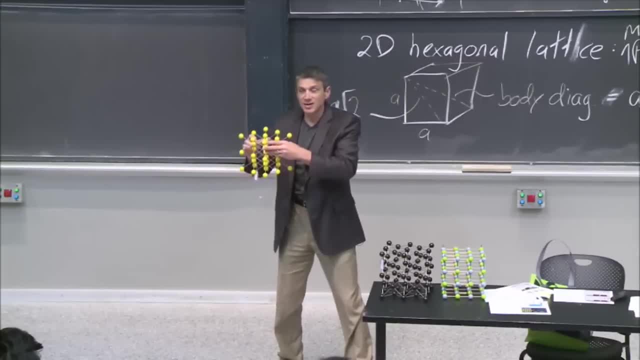 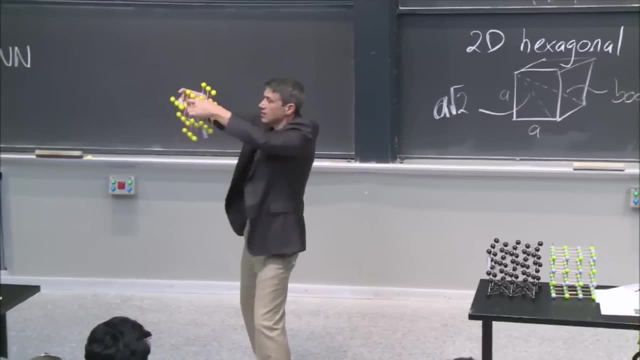 You build it, You get together with friends, You get together with friends and you build even more And you see how much you can build. And then you look and you see, look, here it is, There's my square right. 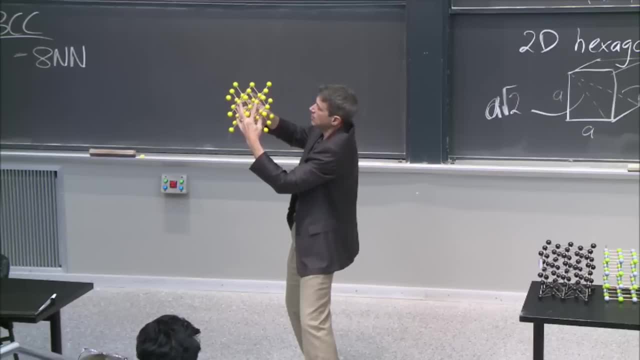 OK, and there's another square and that's my cube, And you go like this. And then you're like: oh look, and there's an atom in the middle, That's BCC, and they're all the same. 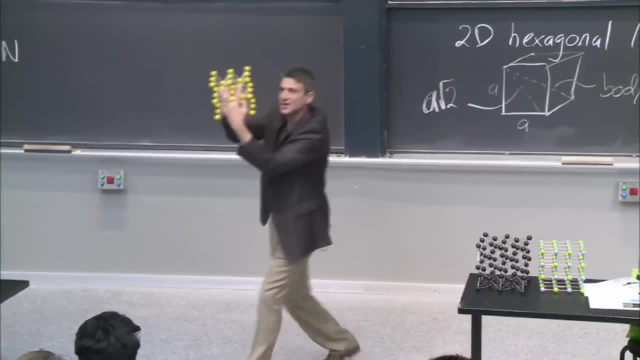 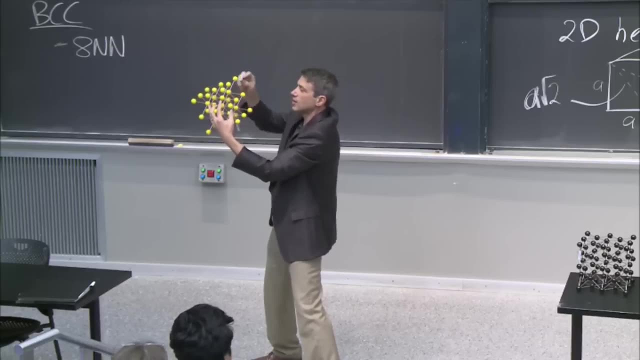 That's BCC right. But see, because this is defined by the lattice, I could have made my square anywhere. This didn't have to be the middle atom. I could move it over, and then this would be the middle atom, or this right. 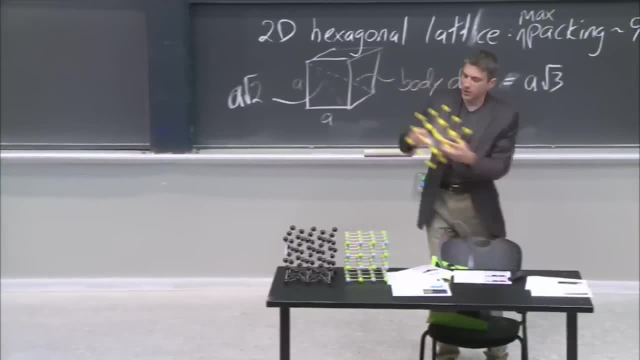 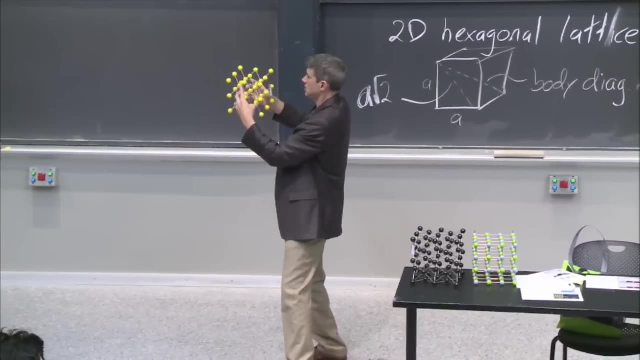 They're all equivalent. It's a lattice. Now, if you look at this and you take that square or that cube, ah, Then what you'll find is that if you go along the body diagonal- see, now, I'm going to take each of these- 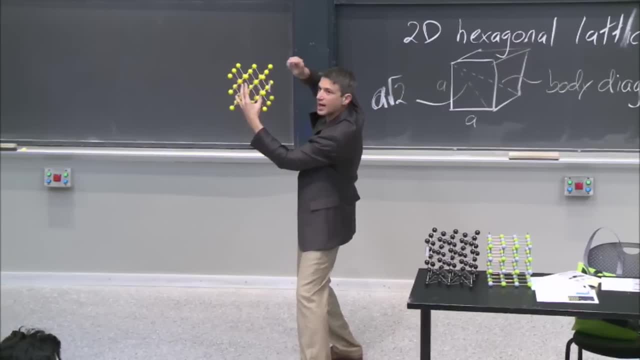 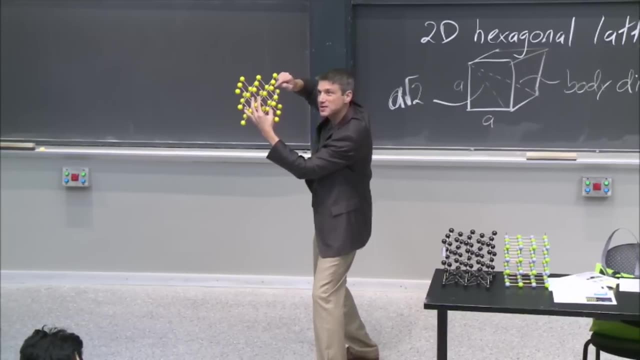 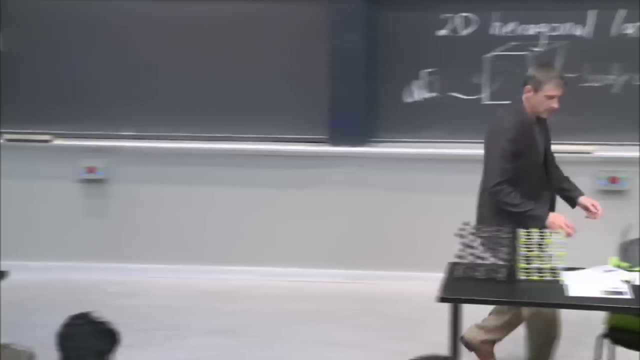 and I'm going to grow them. Where do the atoms touch? If I grow the atoms in a BCC crystal, they touch along the body diagonal first. Now, that's really important. Let's pass this one around too. That's really important, OK. 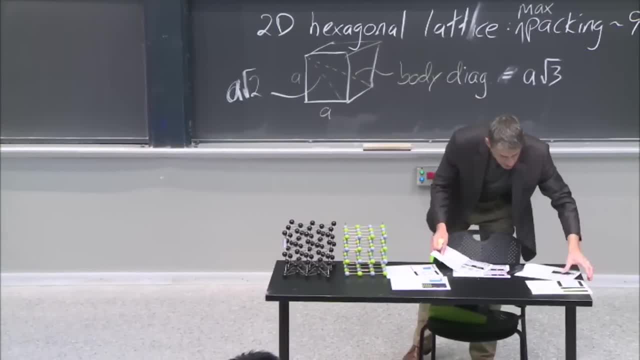 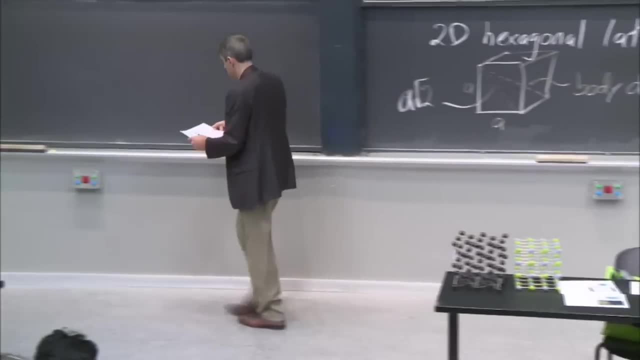 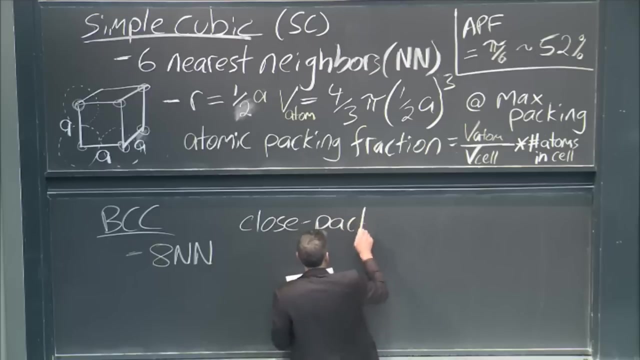 Because now we have this concept that again is also very important, which is the closed-packed direction. Closed-packed direction And for the BCC structure it's the body diagonal Over here, it's the cube edge. For a simple cubic it's the cube edge. 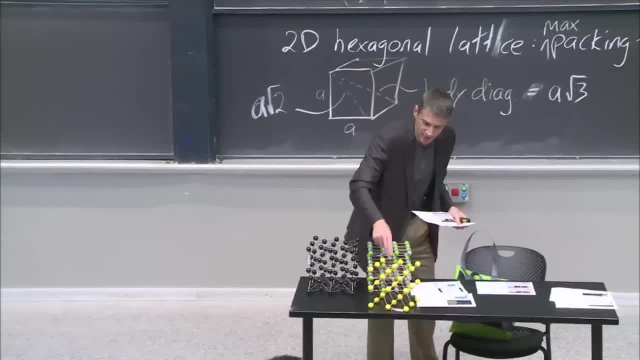 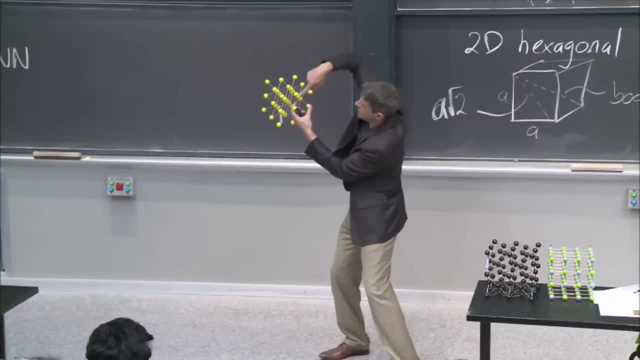 Well, you can see that because I've got the six, but then I've got these ones here, right, I've got- actually it's not the six, I've got the one along the diagonal, which is kind of the point I wanted to make. next, 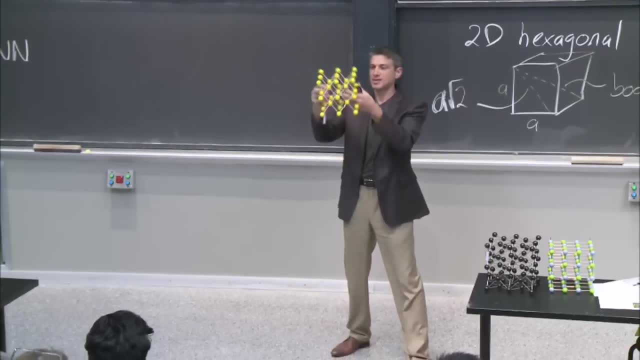 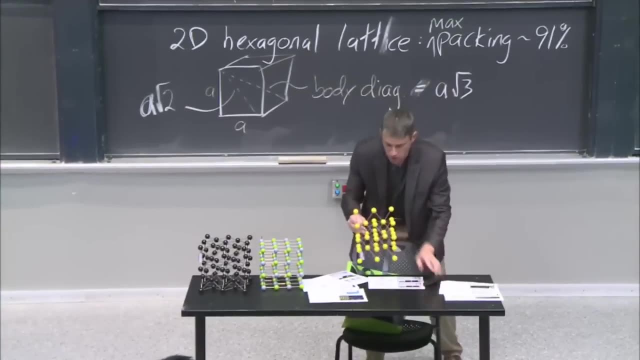 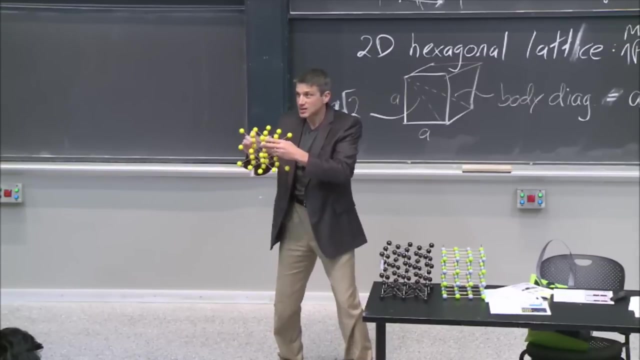 This, oh, this is BCC. This is BCC right Now. how do you see that it's BCC? Because you stare at it and you stare at it, You build it, You get together with friends, You get together with friends and you build even more. 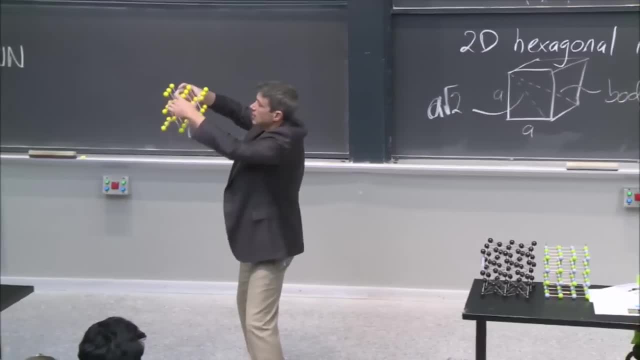 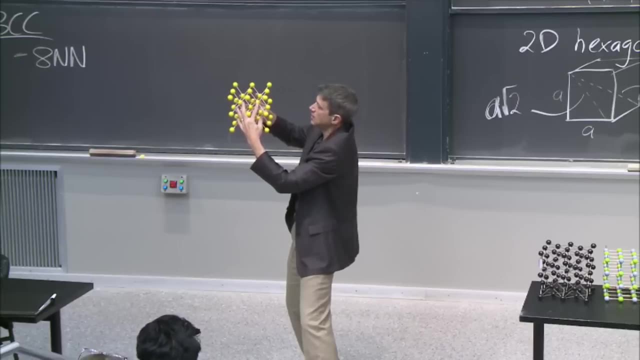 And you see how much you can build. And then you look and you see: look, here it is, There's my square, right, OK, and there's another square and that's my cube. And you go like this: 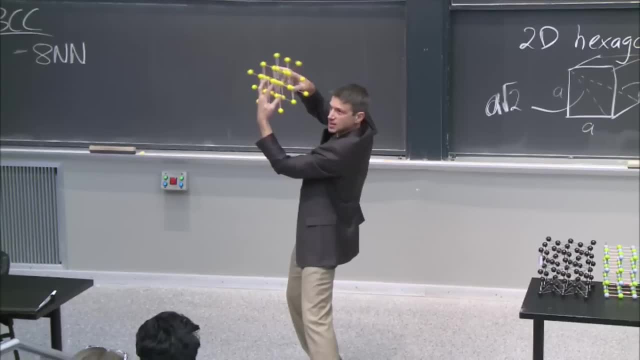 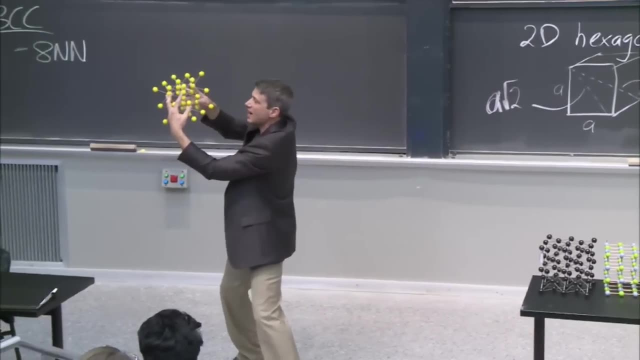 And then you're like, oh look, and there's an atom in the middle, That's BCC, and they're all the same. That's BCC, right, But see, because this is defined by the lattice, I could have made my square anywhere. 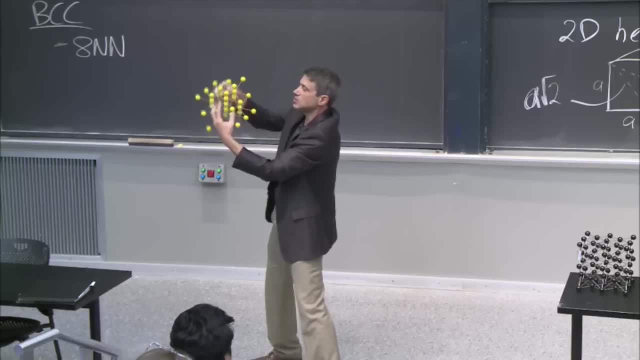 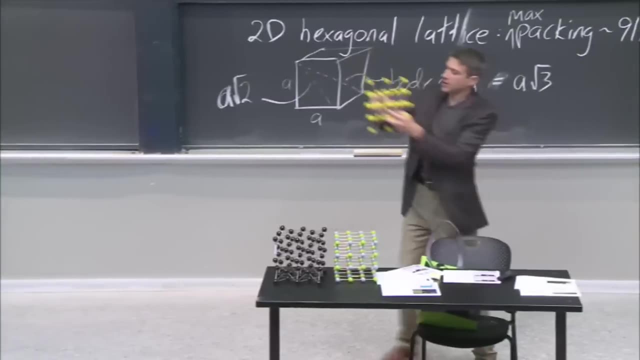 This didn't have to be the middle atom. I could move it over and then this would be the middle atom or this, right, They're all equivalent. It's a lattice Now if you look at this and you take that square. 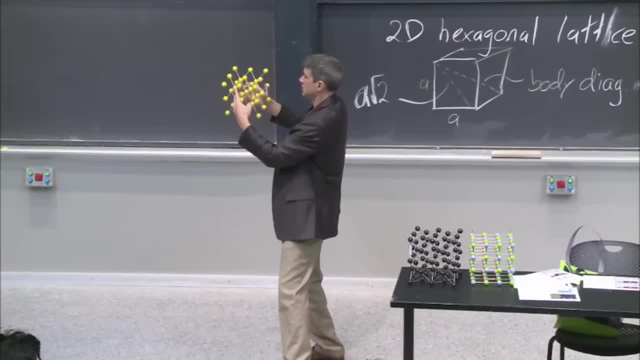 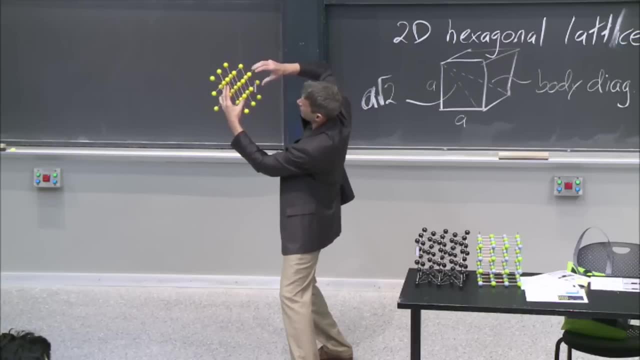 or that cube- Then what you'll find is that if you go along the body diagonal- see, now I'm going to take each of these and I'm going to grow them- Where do the atoms touch? If I grow the atoms in a BCC crystal? 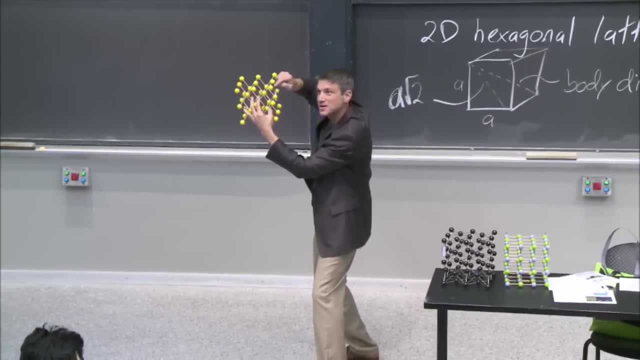 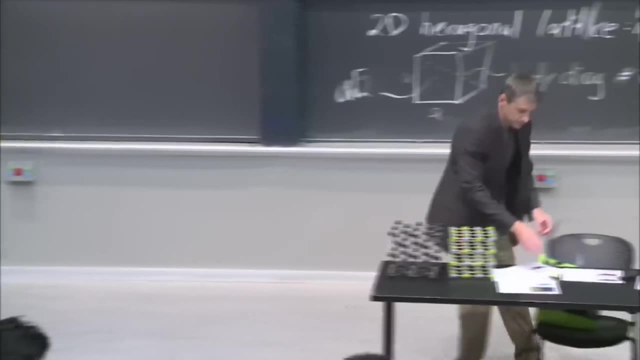 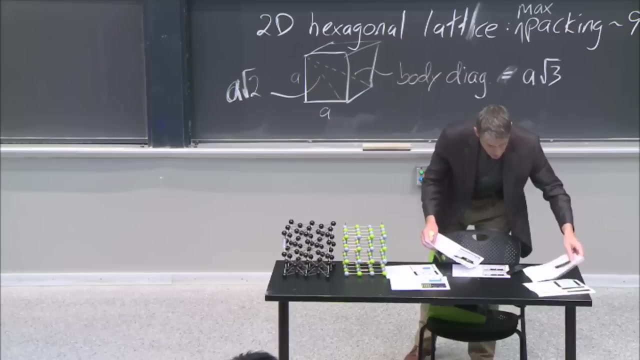 they touch along the body diagonal first. Now, that's really important. Let's pass this one around too. That's really important, OK, Because now we have this concept That is also very important, which is the closed-packed direction. 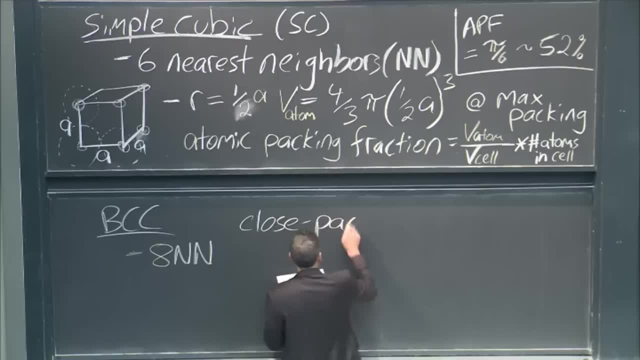 Closed-packed direction. And for the BCC structure it's the body diagonal Over here. it's the cube edge. For a simple cubic it's the cube edge. Cube edge is the closed-packed. OK, how's that going to work? 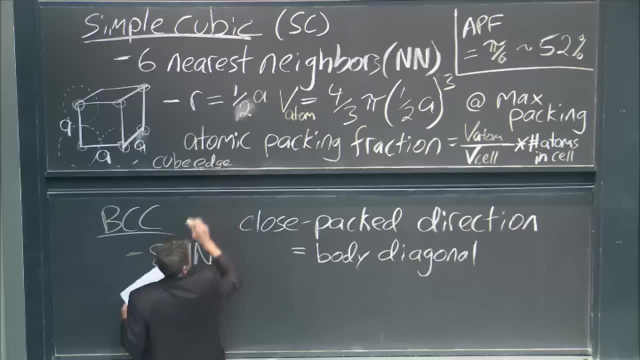 Cube edge is the closed-packed. OK, how's that going to work? I'll do this That. No, that's going to be confusing. Cube edge closed-packed- Oh, that's really small, But you get my point. Closed-packed direction. 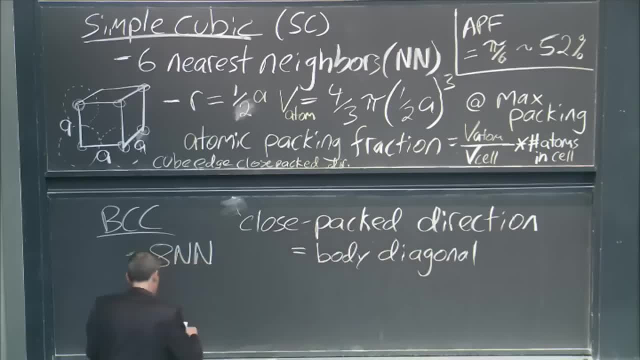 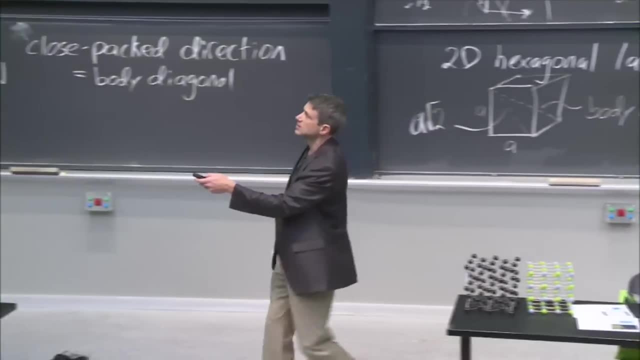 Closed-packed direction: body diagonal. Now, what that means is that- And you can see it right here If you go back all the way back to this, there it is. Let's see as I grow these, these are the same. 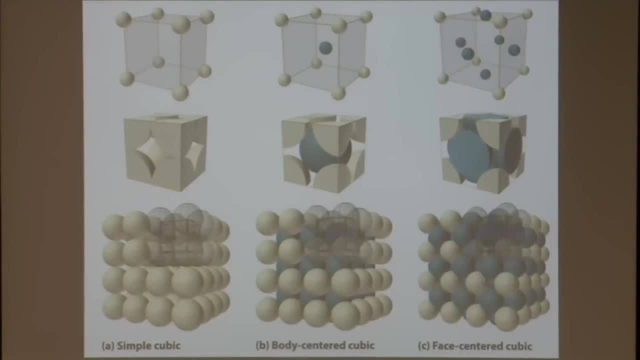 They're colored blue just for clarity, just so you can see. But these are the same because it's a BCC lattice And as I grow them, these all have the same radius. These are the ones that touch first along the diagonal. 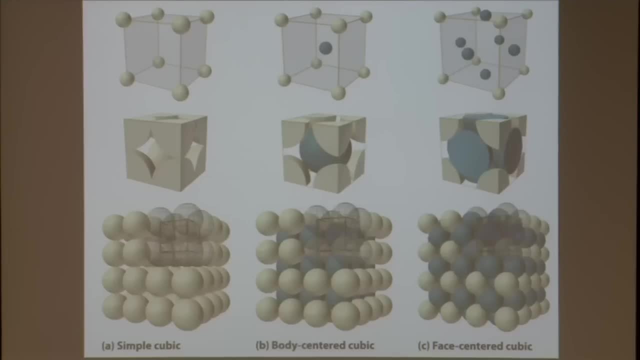 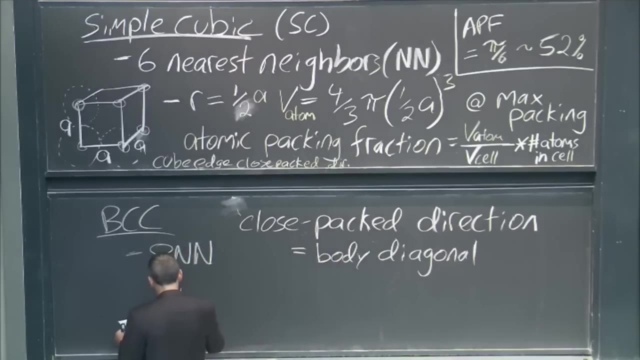 not those, Not those. And that feeds into what the radius is of the atom. I do the same trick And the APF is going to be OK: 4 thirds pi, And now I've got my a root: 3 over 4.. 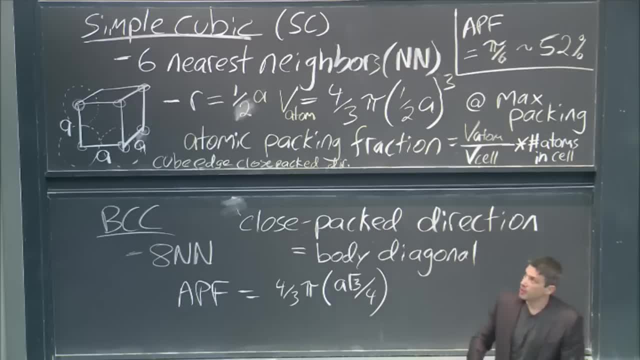 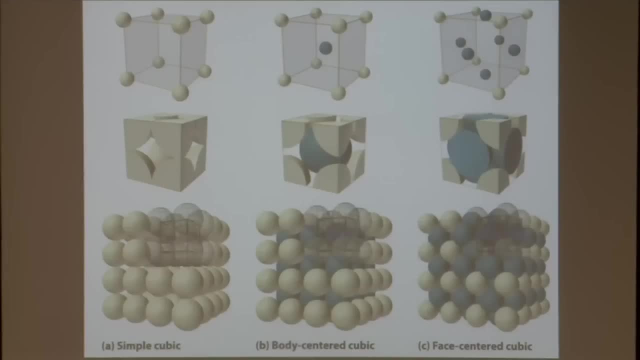 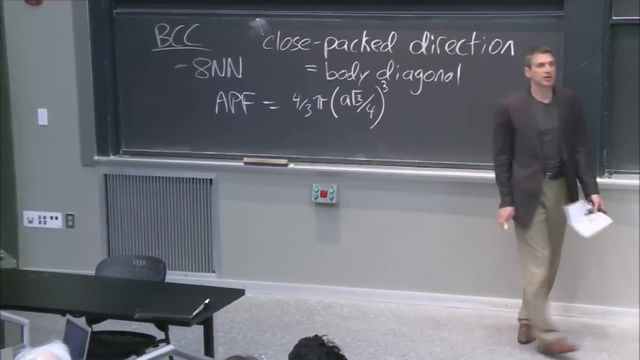 Why? Because a is the length of the cube And you can see here I've got four radii right. Two diameters of the sphere go down the body diagonal, So r cubed 4 thirds pi r cubed is going to be the volume of a maximally packed. 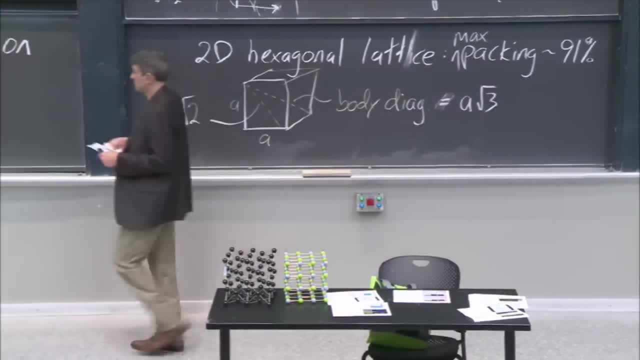 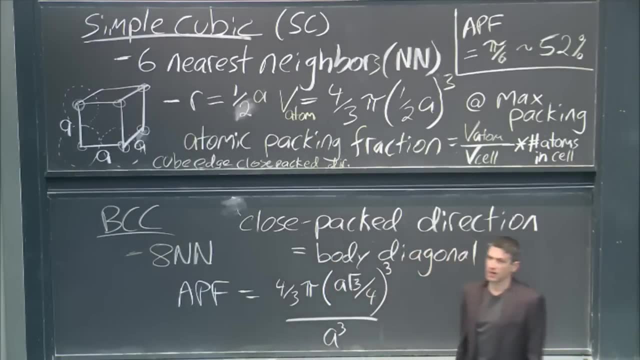 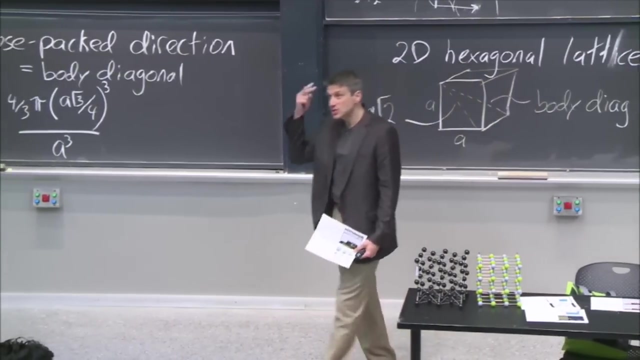 sphere in a BCC lattice. So this has to be divided by the whole volume, which is a cubed. But I'm missing something, because there's not just one, There's not just one, There's another one. There's actually two atoms in a unit cell. 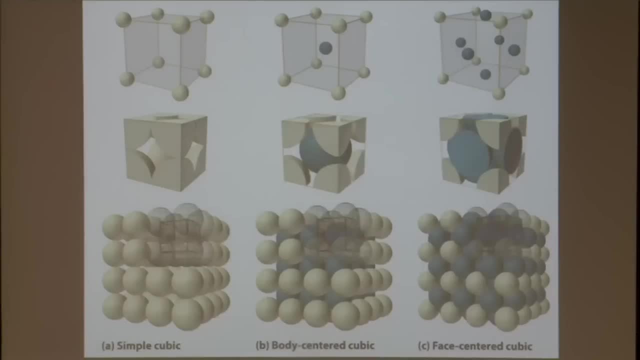 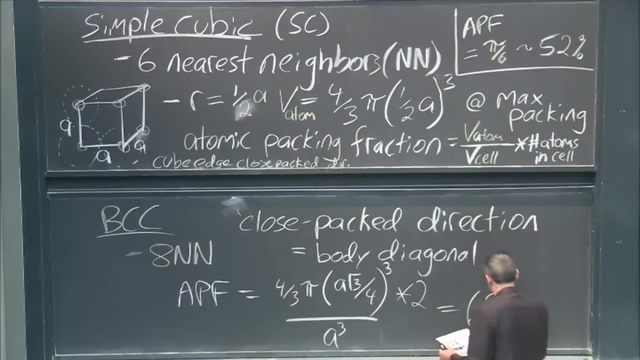 There's two of these. You can see that- one in the middle and then the eighth, eighth, eighth, eighth, eighth. You've got two, So I've got to multiply it by 2. And it gives you 68%. is the APF. 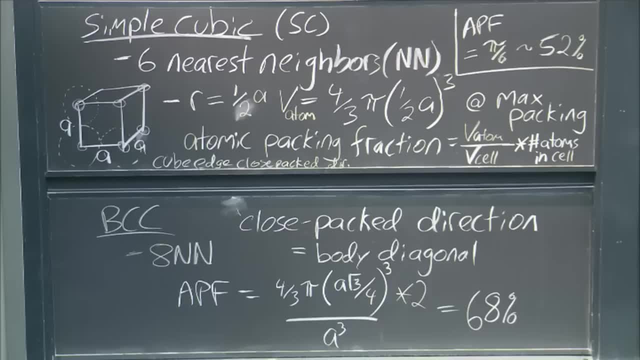 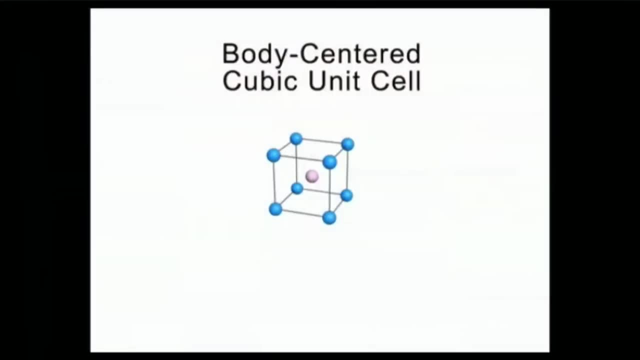 And that's why so many more structures, especially metals, are happy to be BCC. Let's watch the video again, or a different video: this one on BCC Particle at each corner and one in the center which is colored pink to make it easier to see. 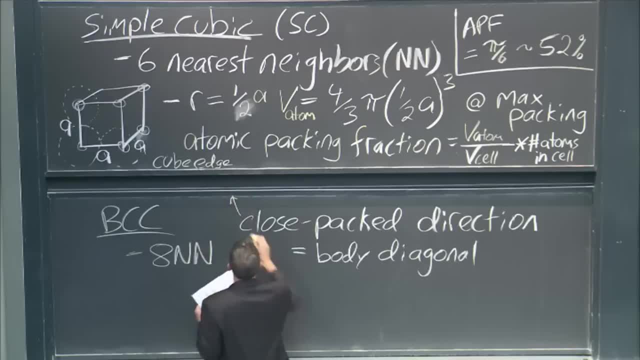 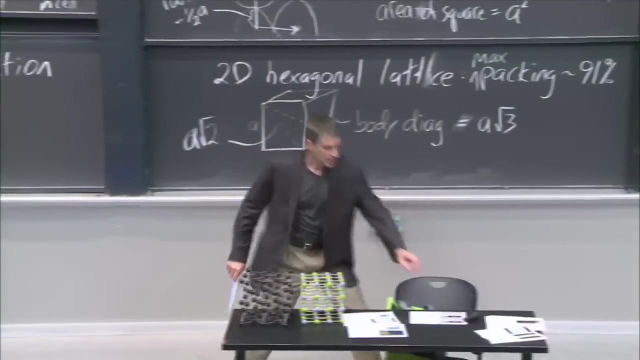 I'll do this, That. No, that's going to be confusing. Cube edge: closed-packed- Oh, that's really small, But you get my point. Closed-packed direction. Closed-packed direction, body diagonal. What that means is that- and you can see it right here: 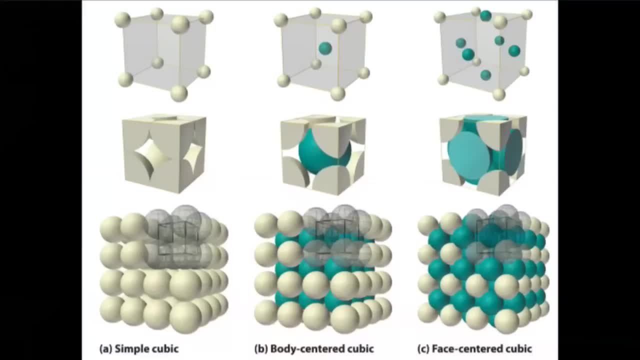 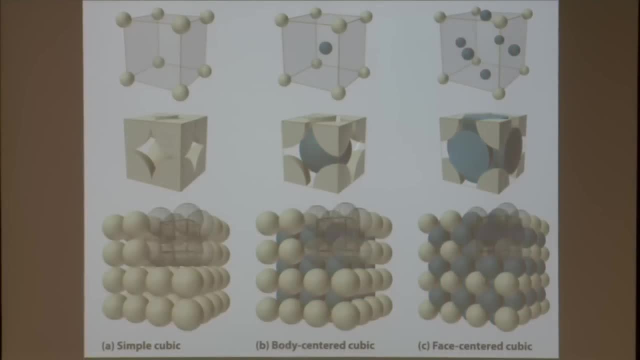 If you go back all the way back to this. there it is. Let's see as I grow these. these are the same. They're colored blue just for clarity, just so you can see. But these are the same because it's a BCC lattice. 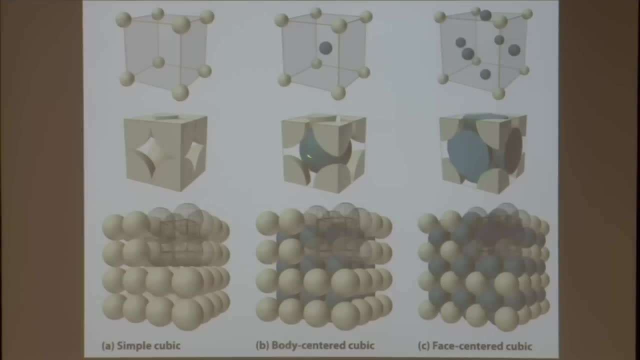 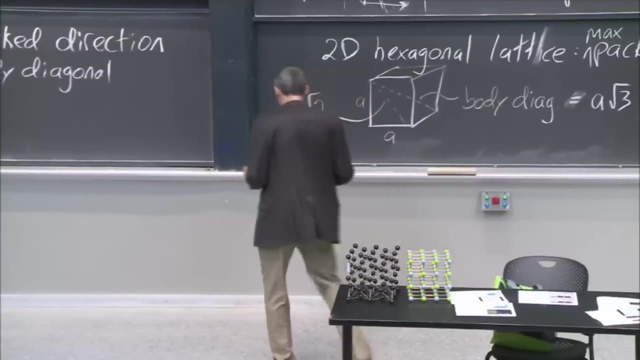 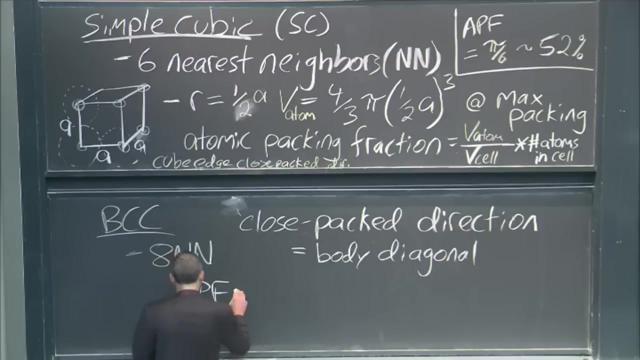 And, as I grow them, these all have the same radius. These are the ones that touch first along the diagonal, not those right, Not those, And that feeds into what. the radius is OK, The atom- I do the same trick, and the APF is going to be OK. 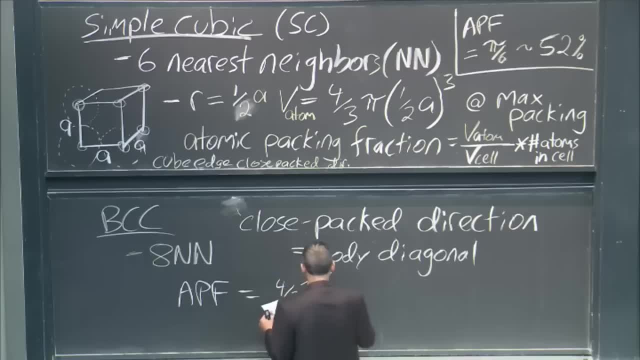 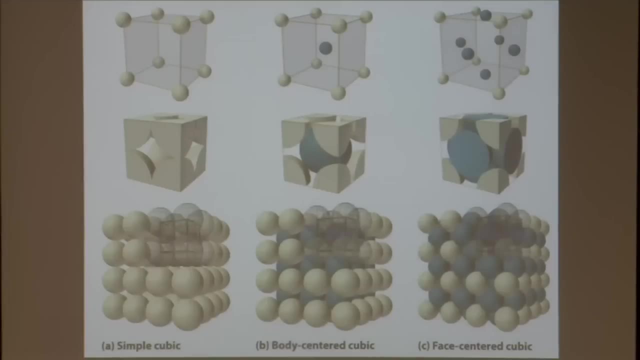 4 thirds pi. And now I've got my a root 3 over 4.. Why? Because a is the length of the cube And you can see here I've got four radii right. Two diameters of the sphere go down the body diagonal. 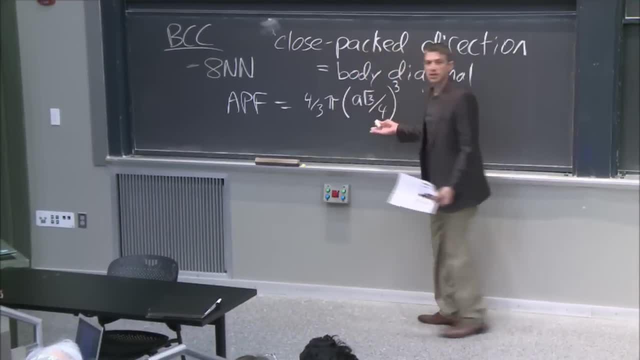 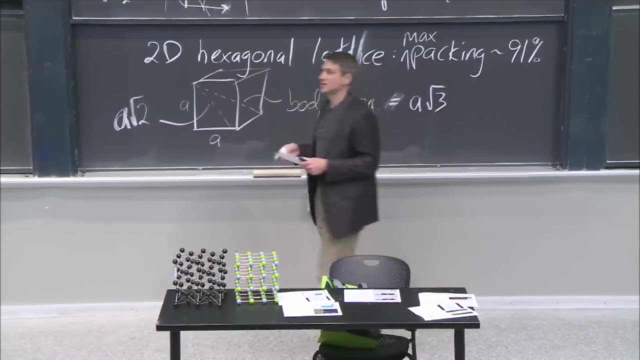 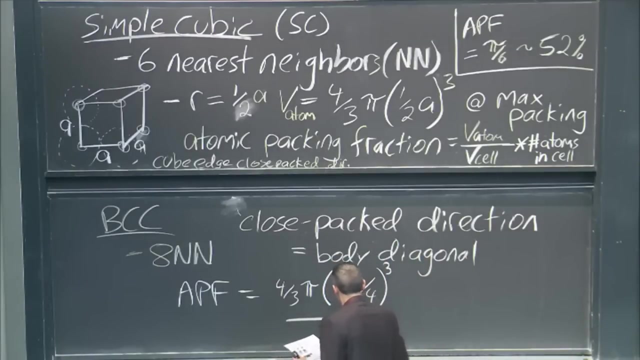 So r cubed, 4 thirds pi? r cubed is going to be the volume of a maximally packed sphere in a BCC lattice. So this has to be divided by the whole volume which is a cubed. But I'm missing something. 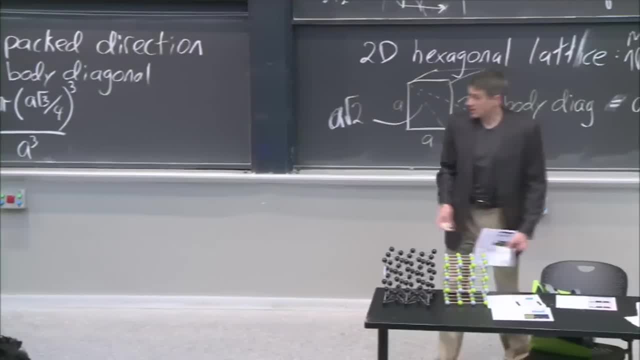 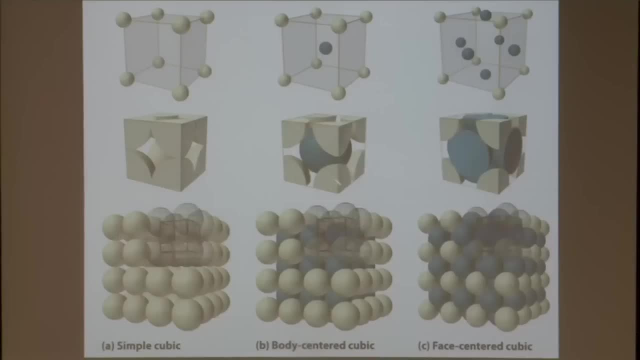 Because there's not just one, right, There's not just one, There's another one. There's actually two atoms in a unit cell. There's two of these. You can see that one in the middle, and then the eighth and eighth, eighth, eighth, eighth, eighth. you've got two. 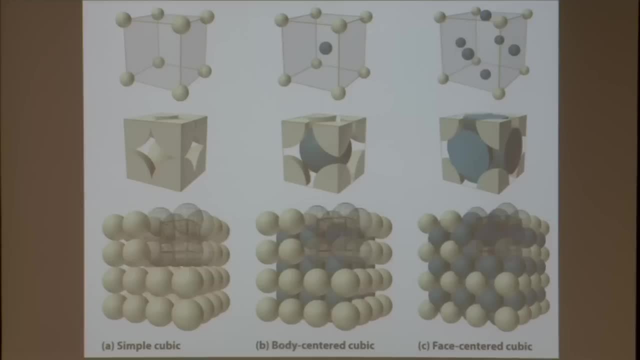 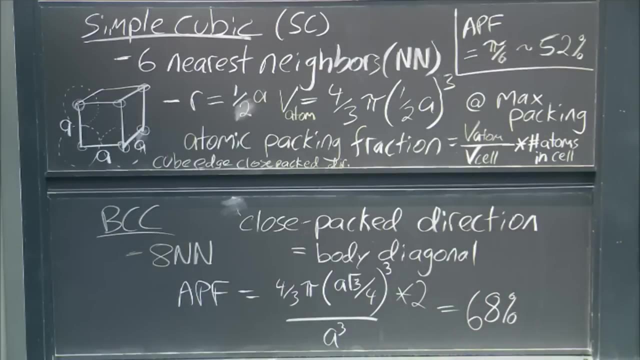 So I've got to multiply it by 2, and it gives you 68% is the APF, And that's why so many more structures, especially metals, are happy to be BCC. Let's watch the video again. Or a different video, this one on BCC. 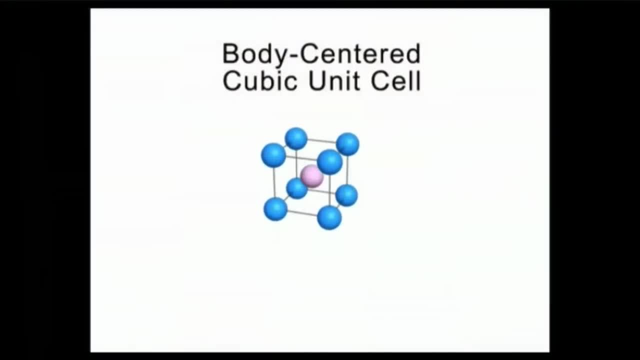 Particle at each corner and one in the center, which is colored pink to make it easier to see With full size spheres, you can see that the particles don't touch along the edges of the cube, But each corner particle does touch the one in the center. 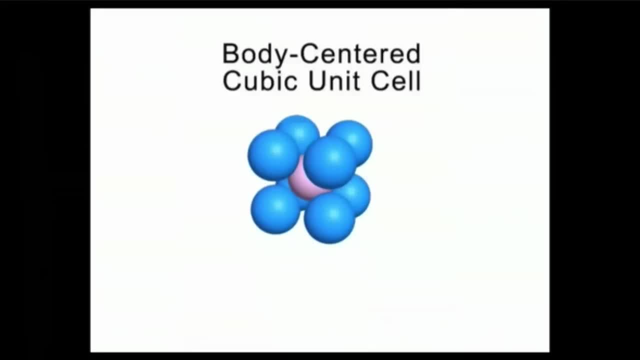 With full size spheres you can see that the particles don't touch along the edges of the cube, But each corner particle does touch the one in the center. The actual unit cell consists of portions of the corner particles and the whole one in the center. 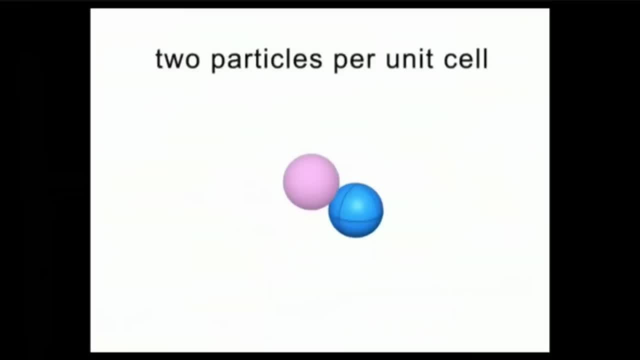 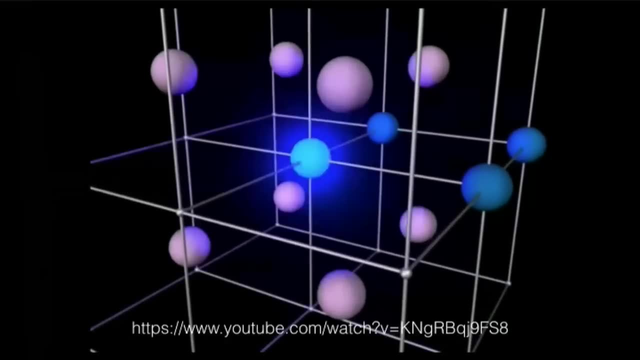 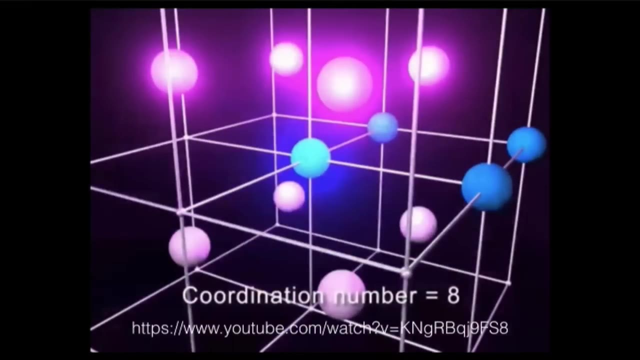 Eight eighths give one particle and the one in the center gives another, for a total of two particles. In this tiny portion of a body-centered cubic array, you can see that any given particle has four nearest neighbors above and four below, for a total of eight. 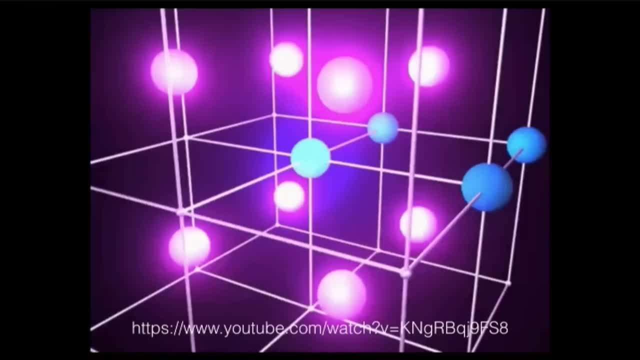 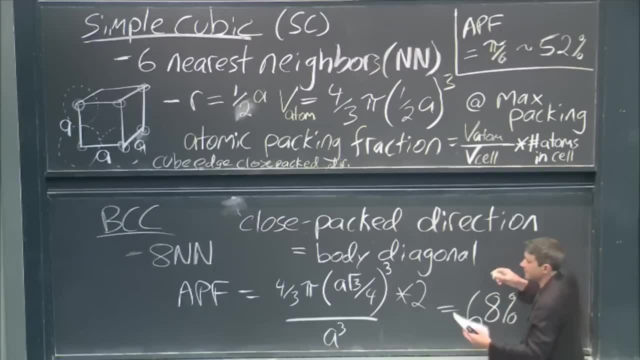 nearest neighbors. OK, now it's really important, right? That's just so you see, conceptually, visually, how we got this. The closed-pack direction for BCC is four times the radius. I want to write that: four times the radius. 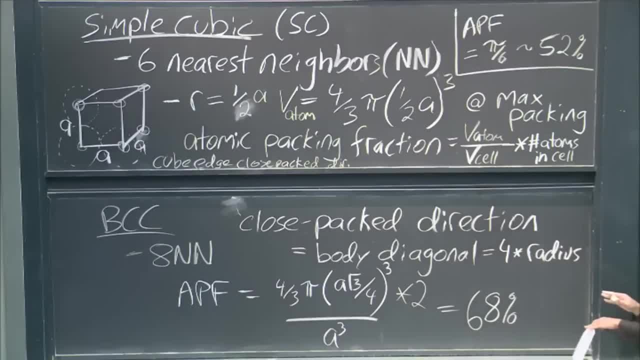 And it's that thing that we're doing now a couple of times, right where you've got the radius of this sphere that you're packing in with a given symmetry. but I've got to write that in terms of the lattice vectors, which are, in this case, all A right. 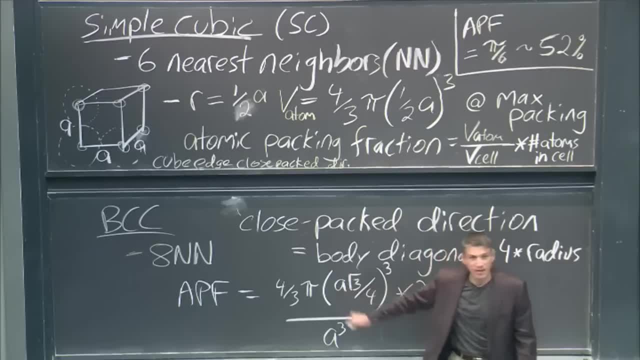 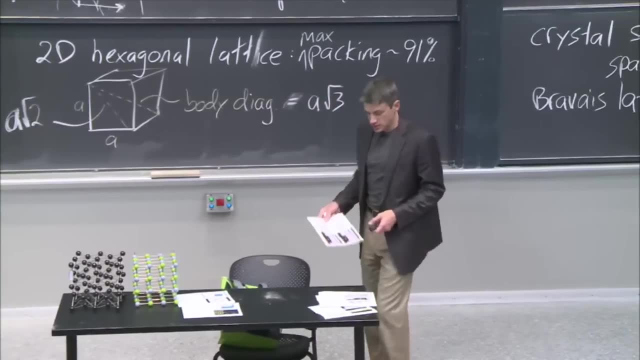 So it's really easy, but they're all A, So I've got to write it in terms of the length of the lattice. That's how you get the atomic packing. OK, Good. Now the last one is FCC. Look at how many elements take the FCC form. 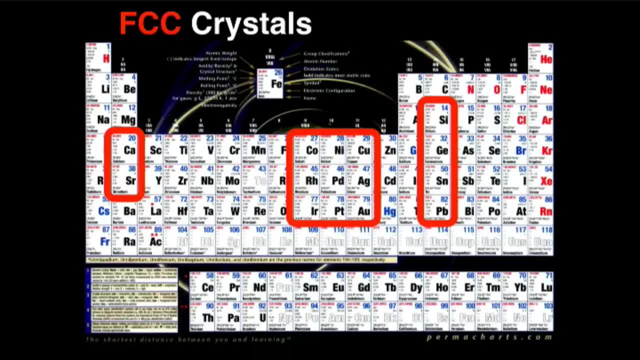 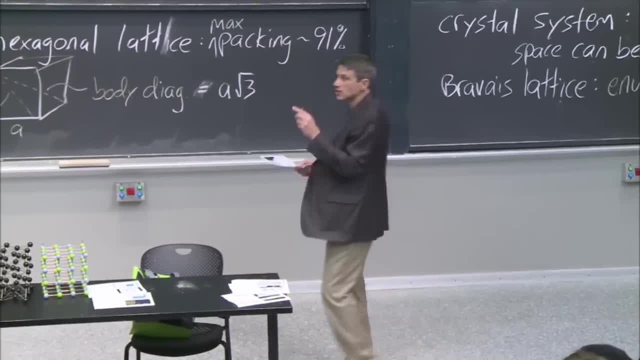 How do you know? You bring out the periodic table and you look it up. Now some of these, many of these elements, can take different crystal symmetries. The ones that are listed are the ones that are often always the most stable one, right, the most stable one. 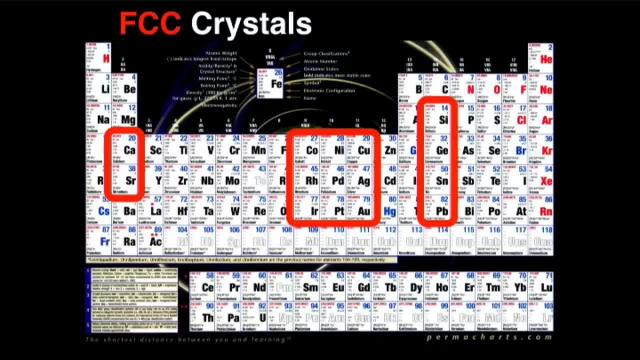 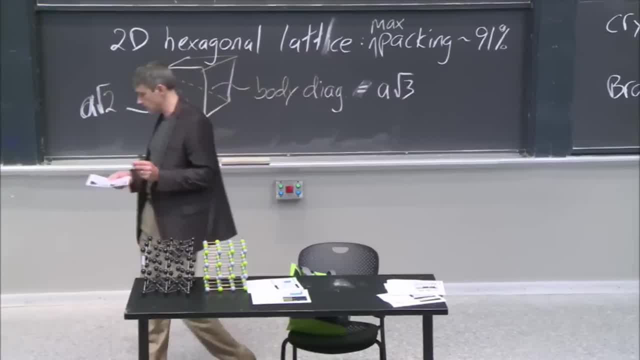 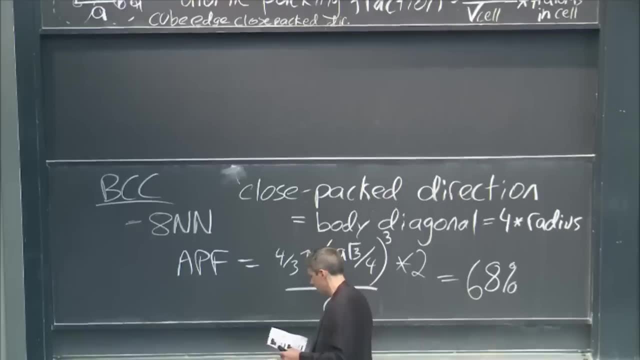 But sometimes they can take many different symmetries. if you do something like add temperature or pressure or other things to the system, What's in the periodic table is the most stable one. Now, the FCC is the last one that we're going to care about. 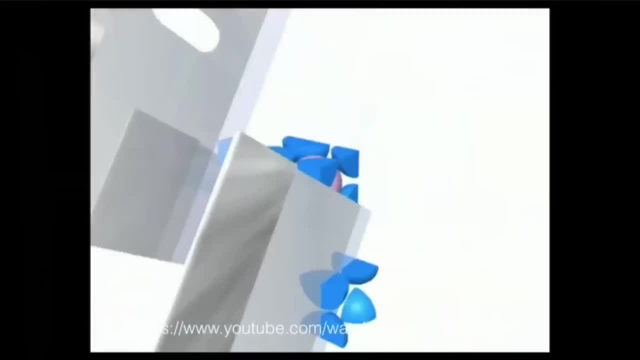 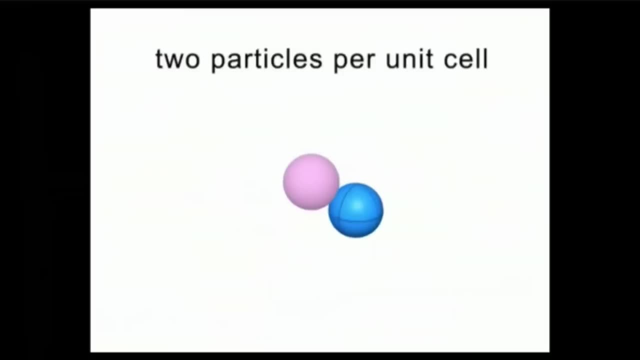 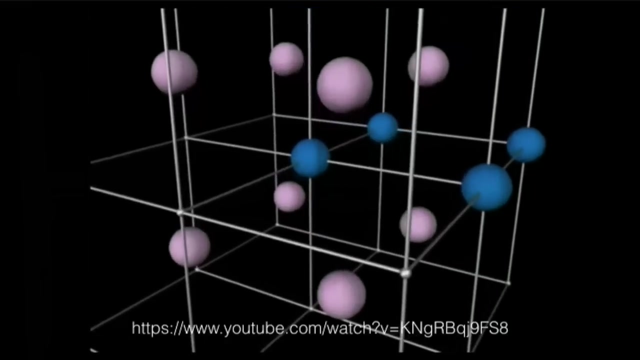 The actual unit cell consists of portions of the corner particles and the whole one in the center. Eight eighths give one particle and the one in the center gives another, for a total of two particles In this tiny portion of a body-centered cubic array. 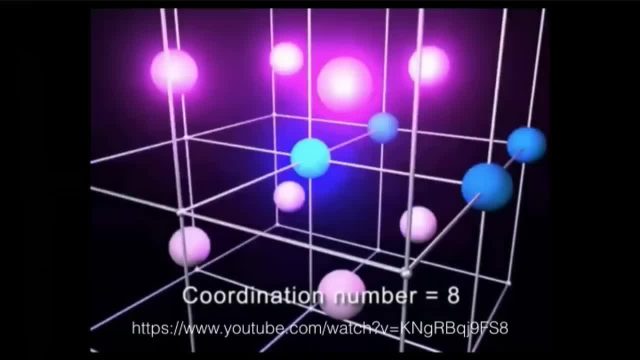 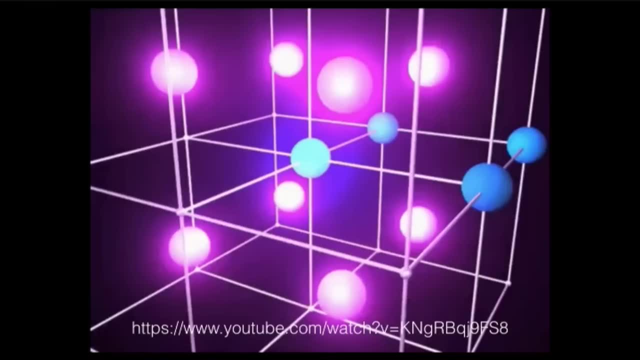 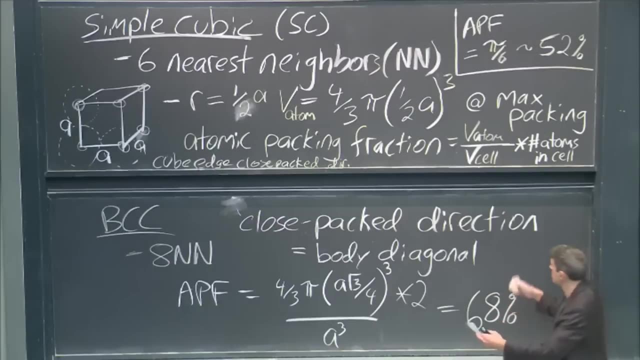 you can see that any given particle has four nearest neighbors above and four below, for a total of eight nearest neighbors. OK, now it's really important, right? Just so you see, conceptually, visually, how we got this. The closed-pack direction for BCC is four times the radius. 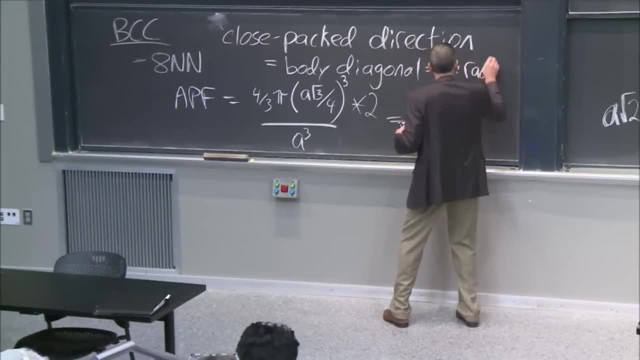 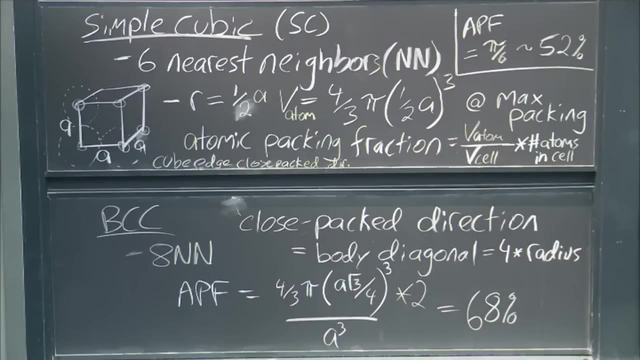 I want to write that four times the radius- And it's that thing that we're doing now- a couple times, right where you've got the radius of this sphere that you're packing in with a given sphere, And I want to write that in terms of the lattice vectors. 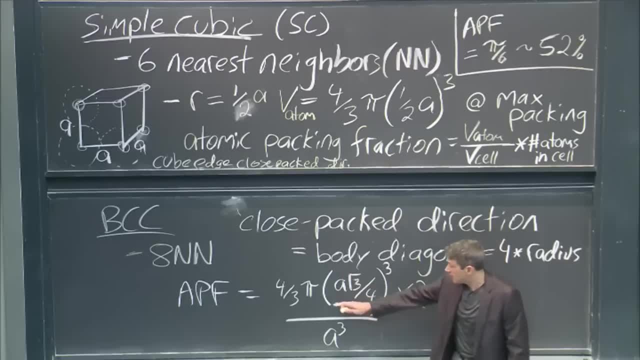 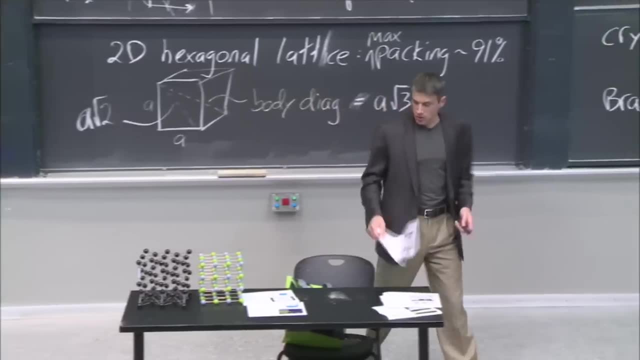 which are, in this case, all A right. So it's really easy, but they're all A, So I've got to write it in terms of the length of the lattice. That's how you get the atomic packing OK, good. 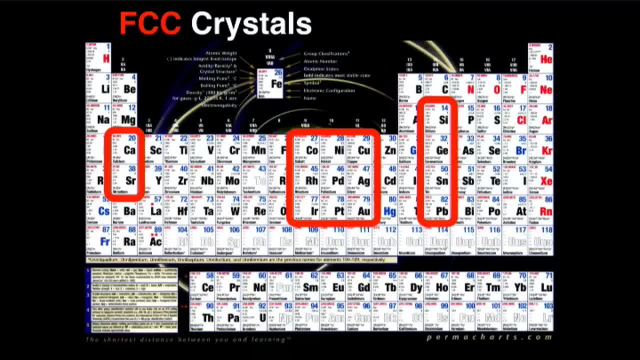 Now the last one is FCC. Look at how many elements take the FCC form. How do you know? You bring out the periodic table and you look it up. Now some of these many of these elements can take different crystal symmetry. 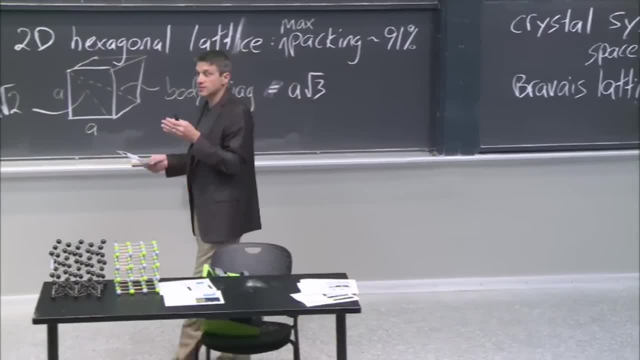 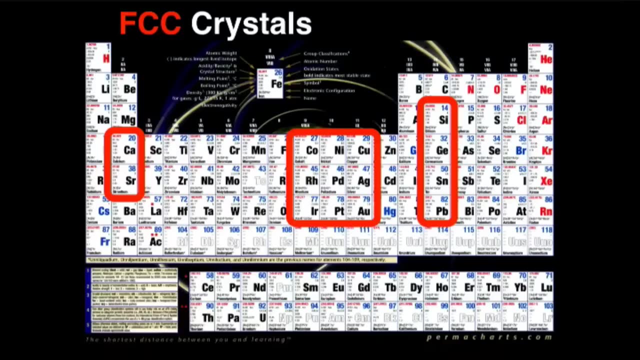 The ones that are listed are the ones that are often- oh, it's the most stable one, right, the most stable one, But sometimes they can take many different symmetries if you do something like add temperature or pressure or other things to the system. 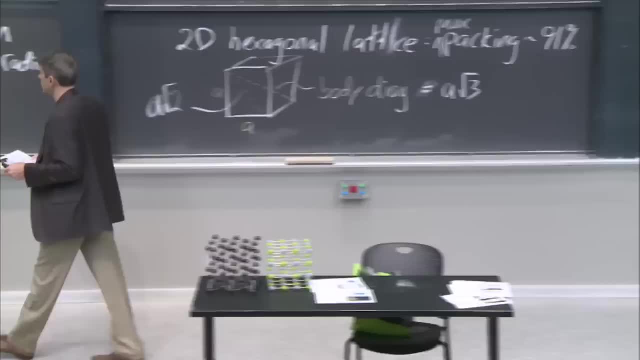 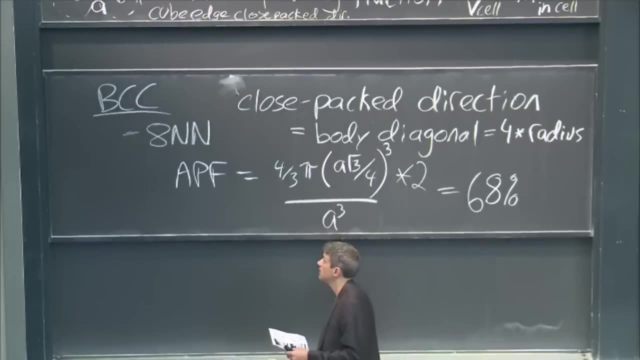 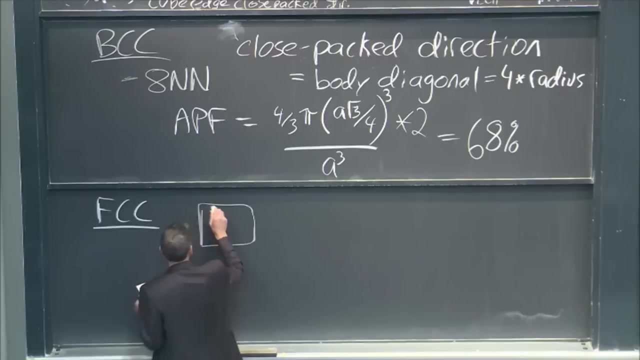 What's in the periodic table is the most stable one. Now the FCC is the last one that we're going to care about, And it is the FCC. It's the face-centered cubic. Now this is OK. so on this one we've got an atom. 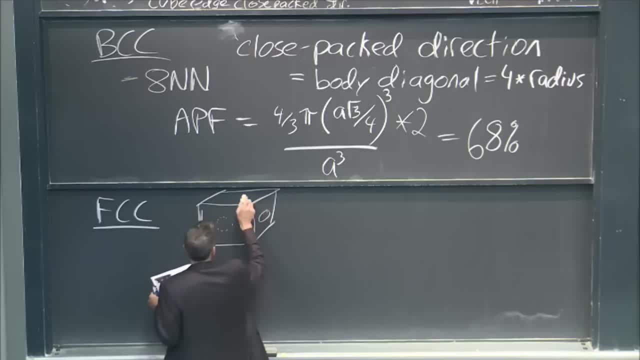 This is the face, right. So we've got these atoms that are sharing across the face, And then we've got these atoms here right at the corners. There's nothing in the middle now, but they're on the faces and sorry. 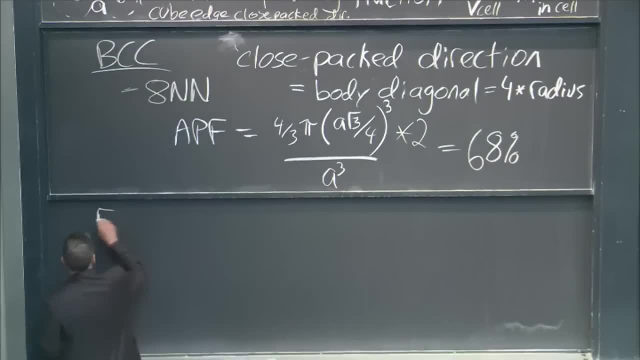 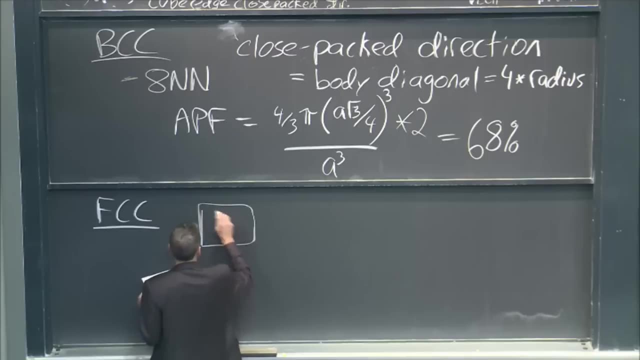 And it is the face center, It's the cubic. Now, this is OK. so on this one, we've got an atom. This is the face right. So we've got these atoms that are sharing across the face. And then we've got these atoms here right at the corners. 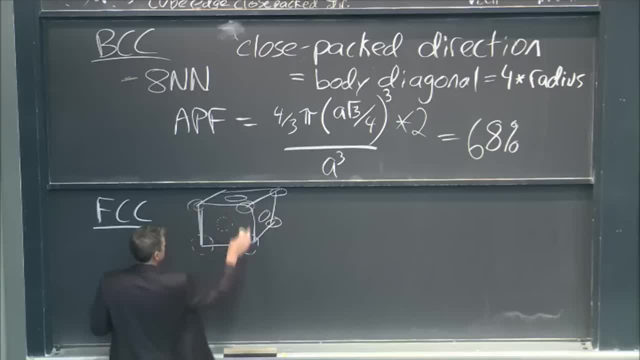 There's nothing in the middle now, but they're on the faces and, sorry, the corners and the faces right. And so, if you look at this, what you can see from looking at this, and you've got to look at it. 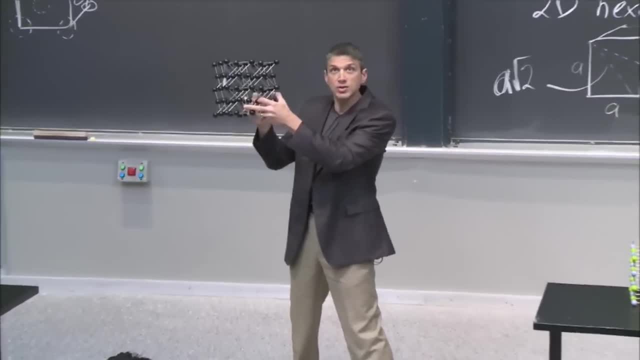 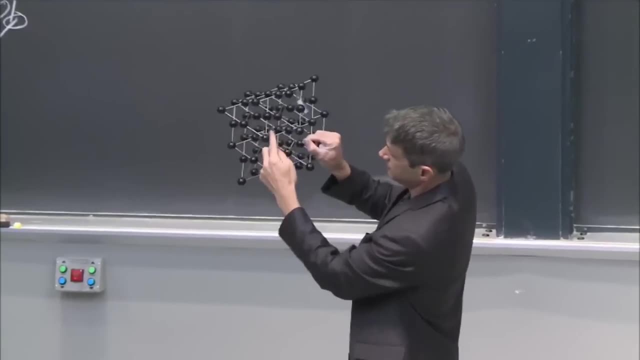 Where's my cube? Where's my unit cell? You now know it's called the unit cell, right? Oh, and I see. and then there's the face atom, right, There's a square there and there's the atom in the face. 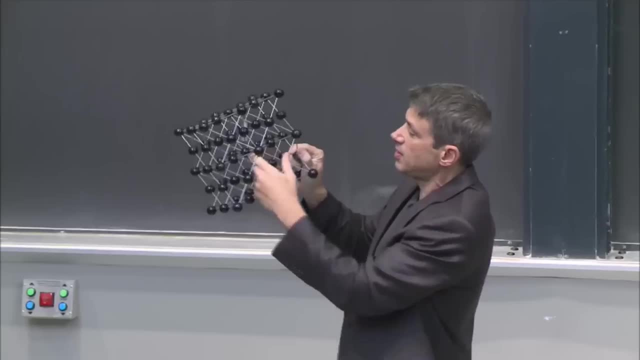 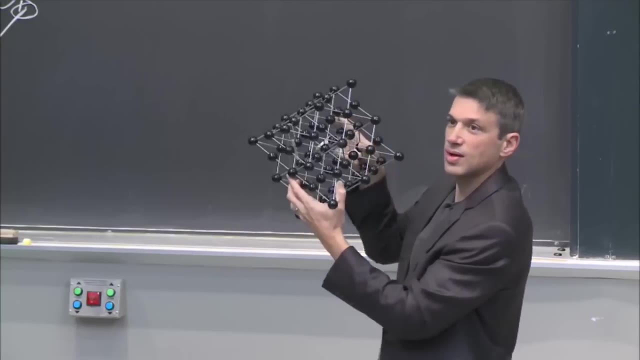 And there's nothing in the middle. It's not BCC, right? But if I look at another edge of that, ah right, there's the atom in that face, and so on and so on. right Now, what's really cool about FCC? 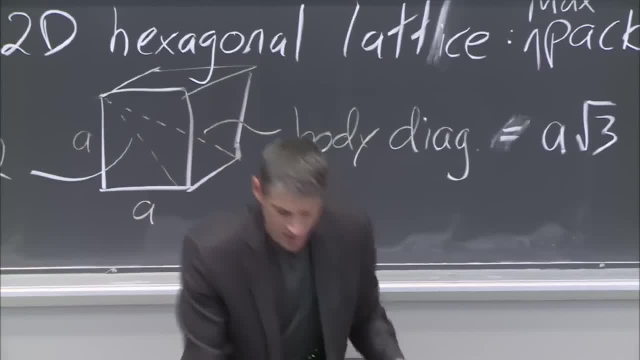 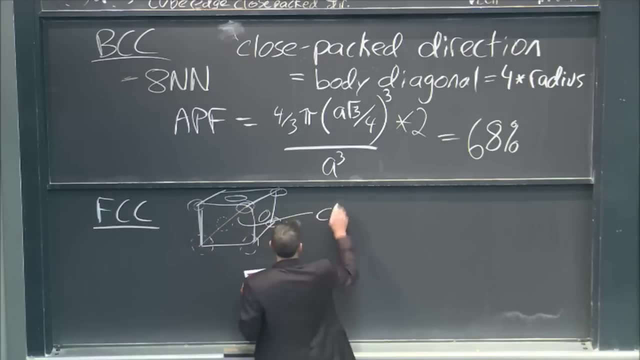 is that it's got a lot of neighbors and it's got more packing. So for FCC, this is the closed-pack direction. Closed-pack direction is the face, is the. did I write down? I didn't write down. OK, that's fine. 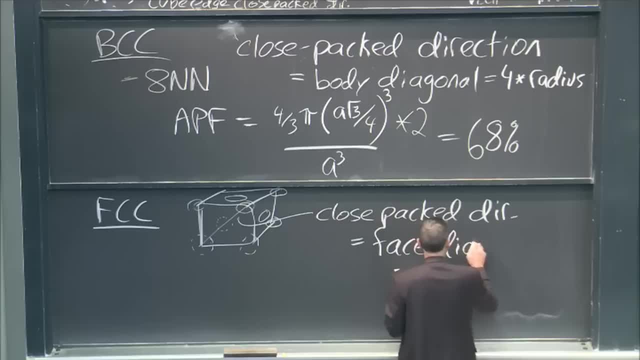 It's the face diagonal, Face diagonal Right, Which is a root 2 in length, And so the atomic packing, so the nearest neighbors, is 12.. And the atomic packing fraction for FCC is 4 thirds pi times. And now here we go, right. 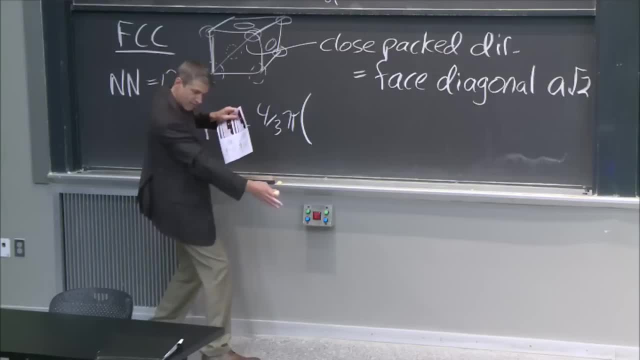 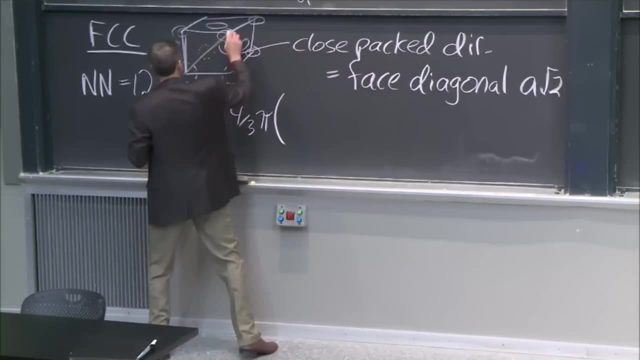 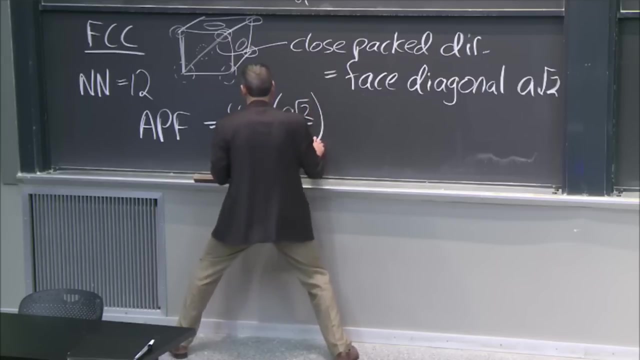 That's when I expand them. it's along the face that they're going to touch, right. So that's the closed-pack direction: face diagonal. That's this one here, right. So it's root. it's a root: 2 over 4, right. 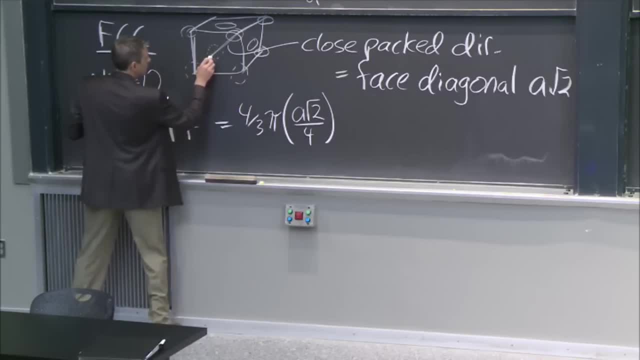 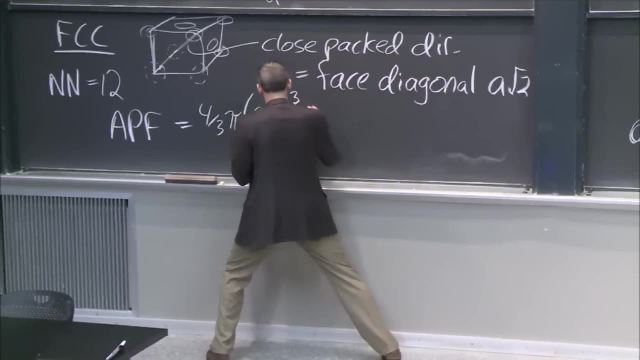 Because again I've got a radius and another, and another, and another. I can you know, there's two diameters worth that go across that face, And so that's going to be cubed. Yeah, OK, Divided by a cubed. 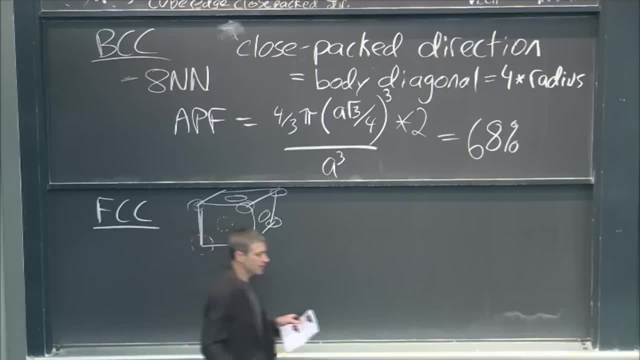 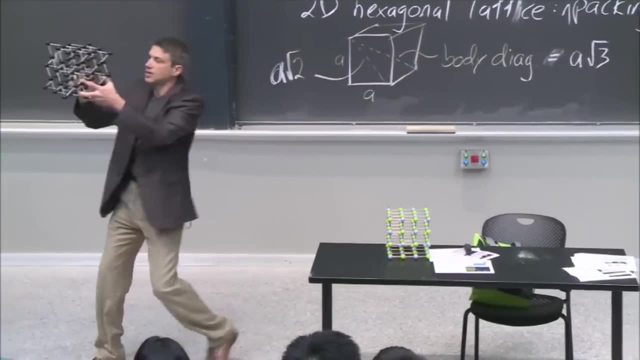 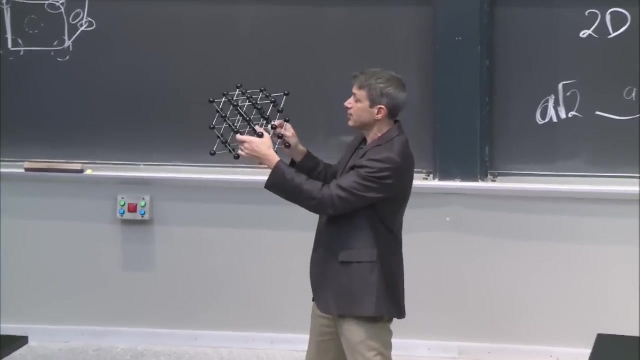 the corners and the faces right, And so, if you look at this, what you can see from looking at this, and you've got to look at it- where's my cube? Where's my unit cell? You now know it's called the unit cell right. 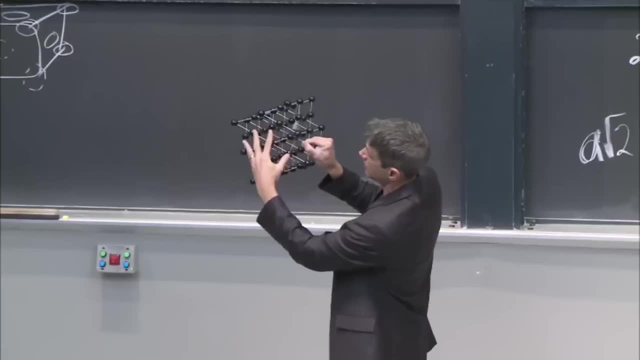 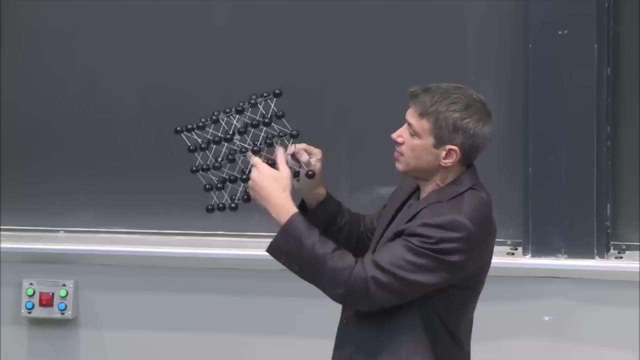 Oh, and I see. and then there's the face atom right, There's a square there and there's the atom in the face And there's nothing in the middle. It's not BCC, right? But if I look at another edge of that, ah right. 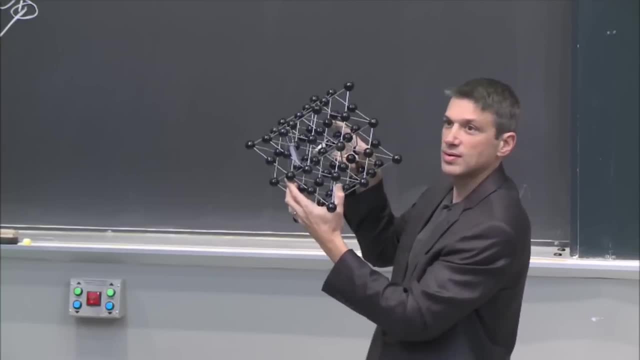 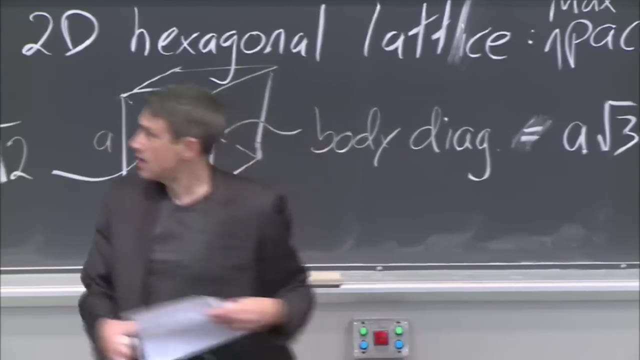 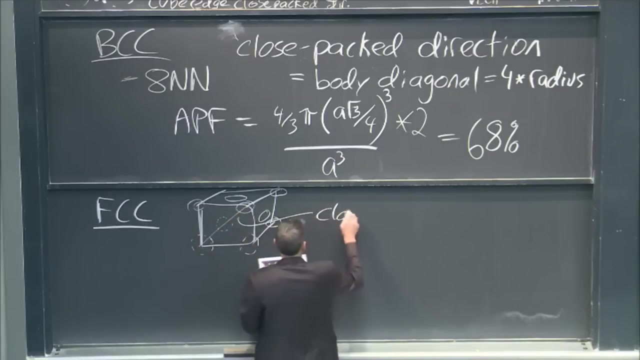 there's the atom in that face and so on and so on. right Now, what's really cool about FCC is that it's got a lot of neighbors and it's got more packing. So for FCC, this is the closed-pack direction. 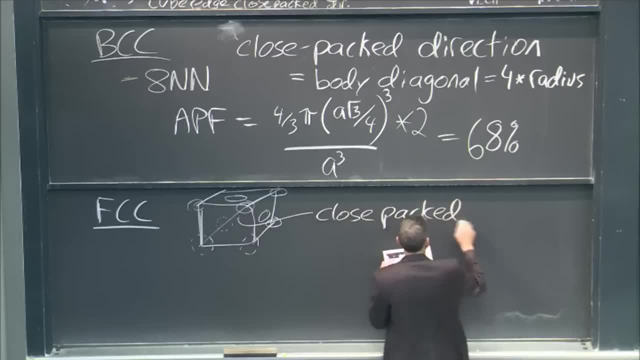 Closed-pack. direction is the face, is the- did I write down? I didn't write down? OK, that's fine, It's the face diagonal Face diagonal Face diagonal right, which is a root 2 in length, And so the atomic packing, so the nearest neighbors, is 12.. 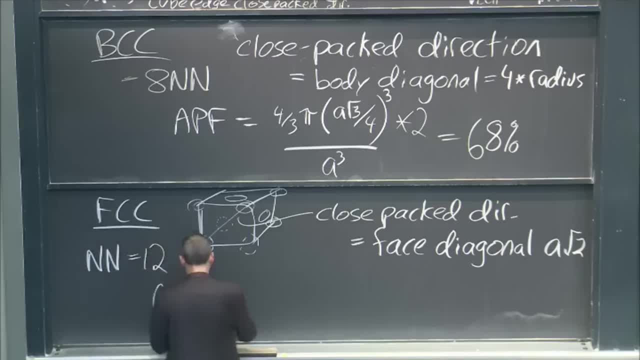 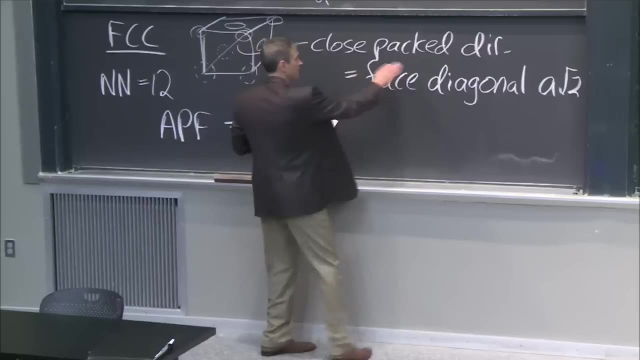 And the atomic packing fraction for FCC is 4 thirds pi times. And now here we go. right, That's when I expand them, it's along the face that they're going to touch, right. So that's the closed-pack direction. 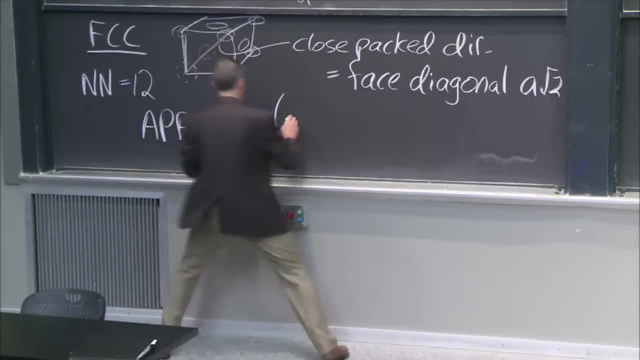 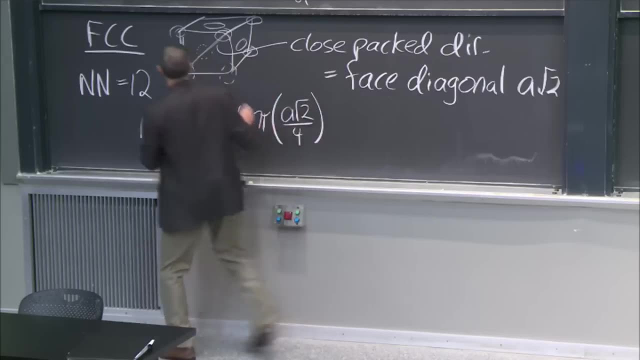 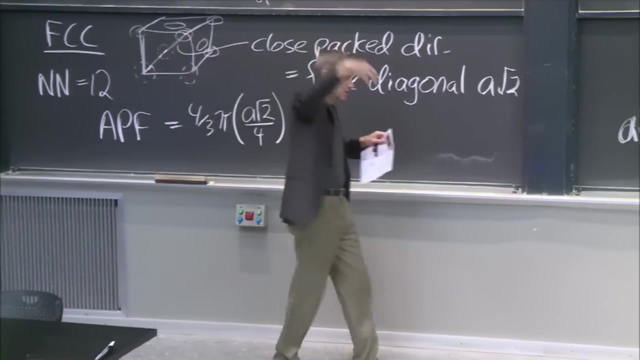 Face diagonal. that's this one here, right? So it's root 2 over 4, right? Because again I've got a radius and another, and another and another. There's two diameters worth that go across that face And so that's going to be cubed. 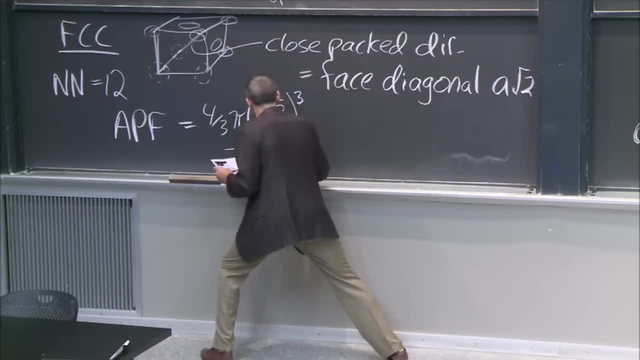 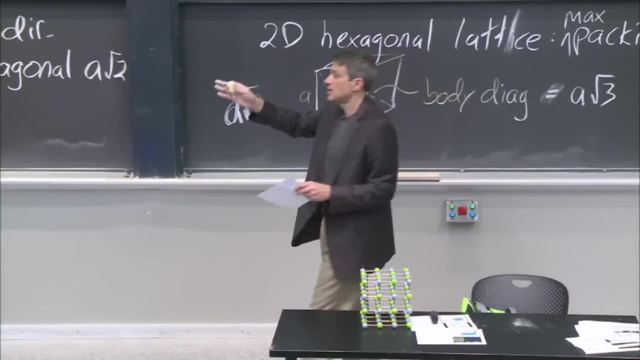 Yeah, OK, divided by a cubed. Now is there something missing? Yes, the number of atoms. The number of atoms. If you look at it, it's a square. If you look at a FCC crystal and you look at the corners. 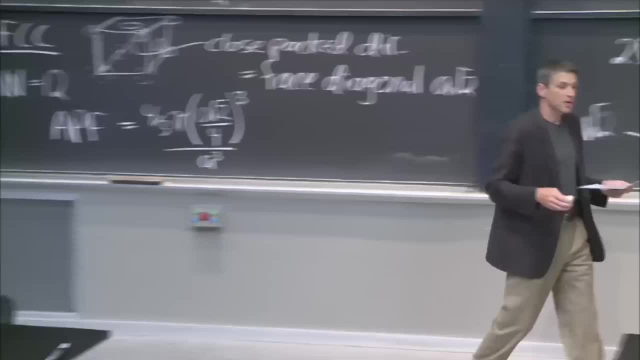 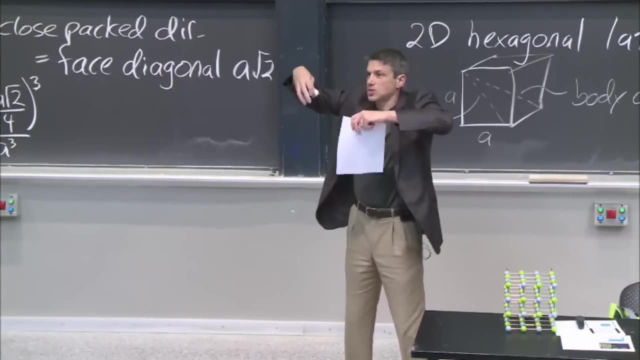 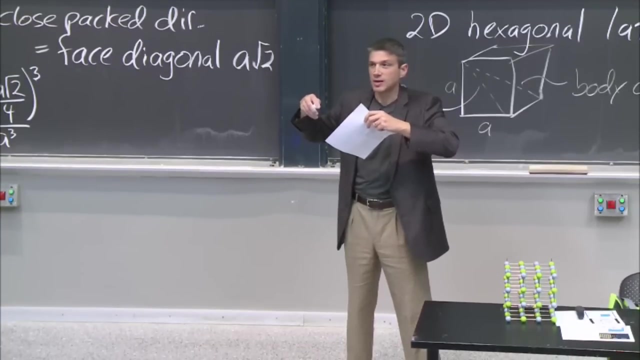 Now, is there something missing? Yes, The number of atoms. If you look at a FCC crystal And you look at the corners, each one of those shares with eight other unit cells, So there's an eighth. That gives you the one, like in our simple cubic. 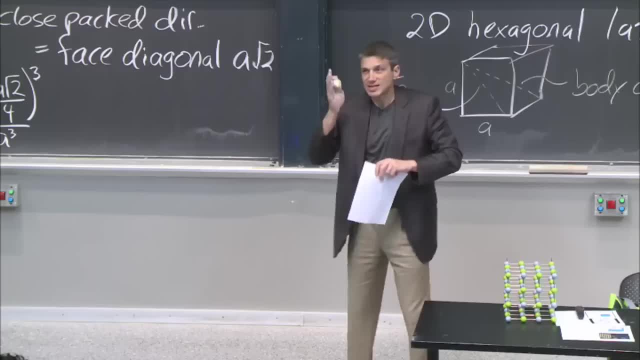 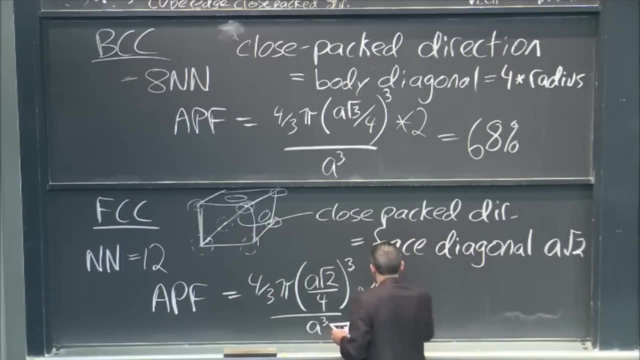 But now you've got all these ones sharing across faces. You've got six of those, each one sharing a half atom. So that's three more, So there's four, And this gives you a very nice packing of 74%, 74%. 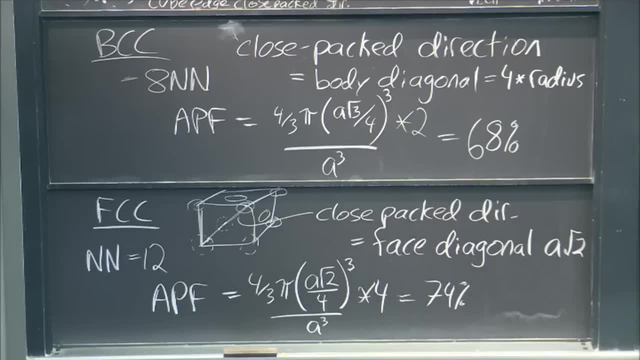 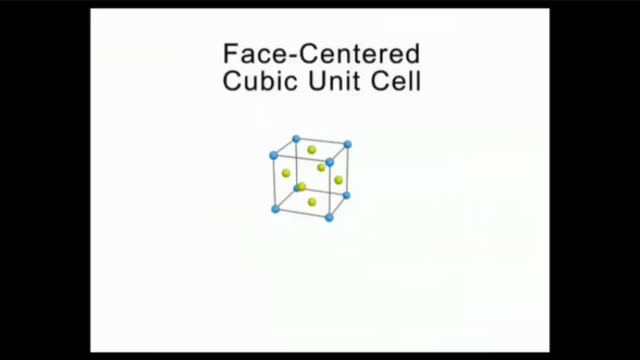 Let's see what our video guy says about FCC. The face-centered cubic unit cell has a particle at each corner and in each face which are colored yellow here but none in the center. The corner particles don't touch each other, But each corner does touch a particle in the face. 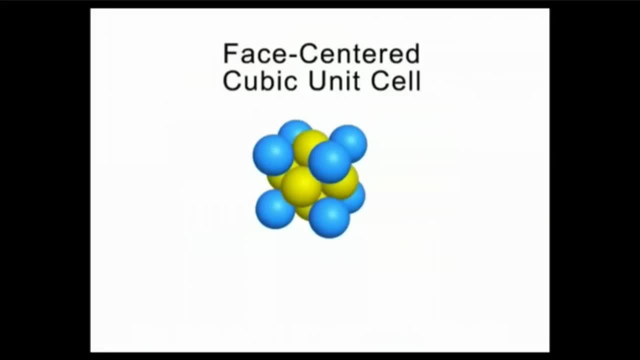 And those in the faces touch each other as well. The actual unit cell consists of portions of particles: particles at the corners and in the faces. Eight-eighths at the corners gives one particle And half a particle in each of six faces gives three more, for a total of four particles. 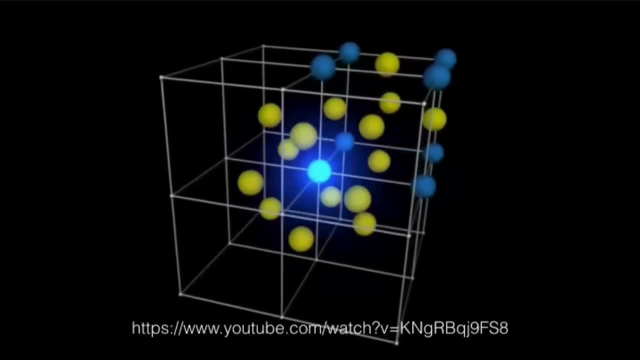 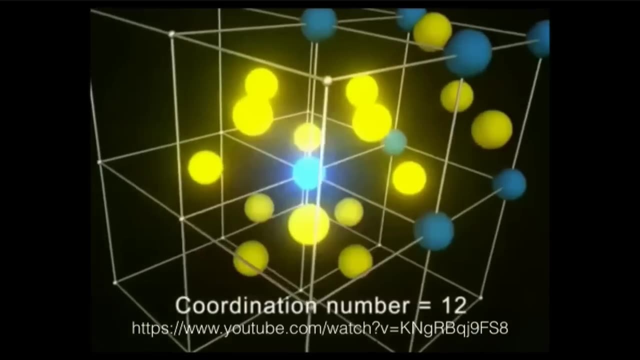 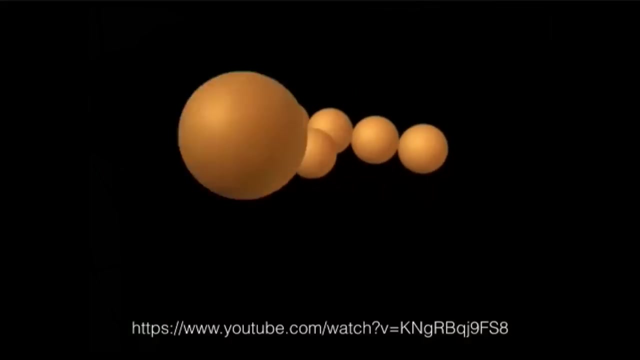 In this tiny portion of a face-centered cubic array, notice that a given particle has four nearest neighbors around it, four more above and four more below, for a total of 12 nearest neighbors- Stacking spheres. Stacking spheres shows how the three cubic unit cells arise. 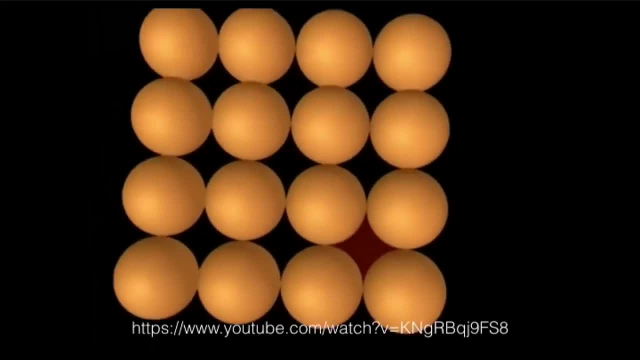 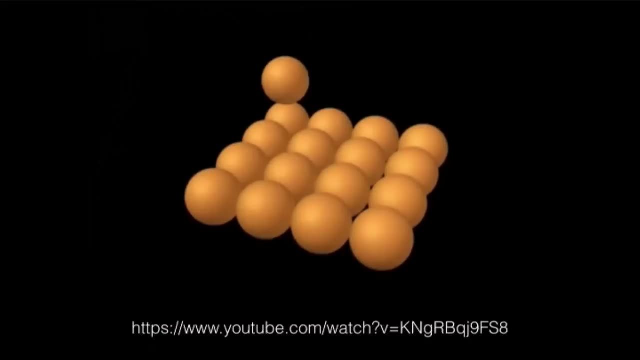 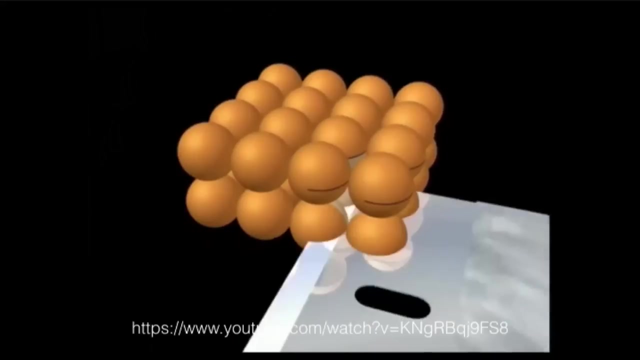 Now we're talking about packing. Arrange a layer of spheres in horizontal and vertical rows. Note the large diamond-shaped space among the particles. Placing the next layer directly over the first gives a structure based on the simple cubic unit cell. Those larger spaces mean an inefficient use of space. 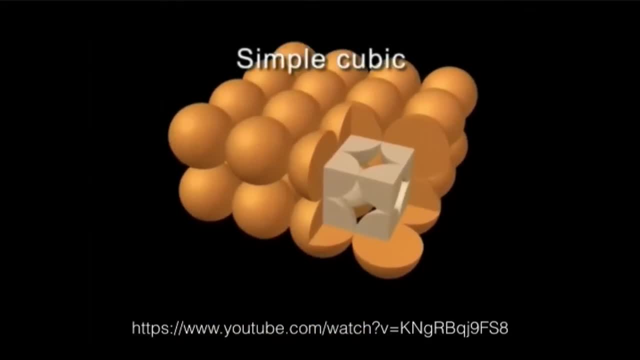 In fact, only 52% of the available volume is actually used. In fact, only 52% of the available volume is actually used. In fact, only 52% of the available volume is actually used. In fact, only 52% of the available volume is actually occupied by spheres. 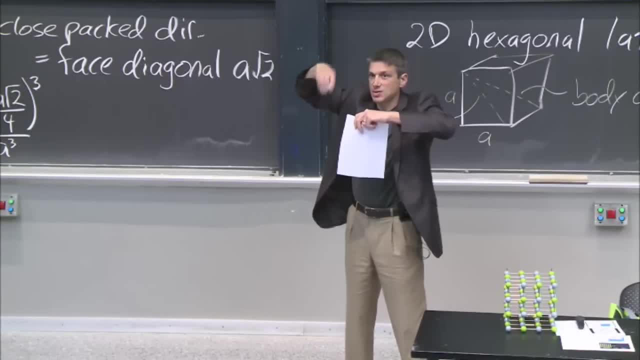 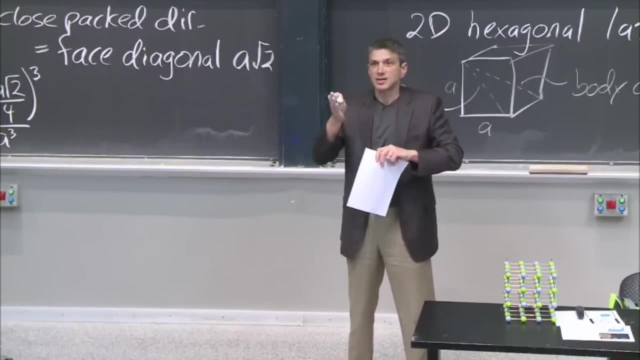 each one of those shares with eight other unit cells, So there's an eighth. That gives you the one, like in our simple cubic. But now you've got all these ones sharing across faces. You've got six of those, each one sharing a half atom. 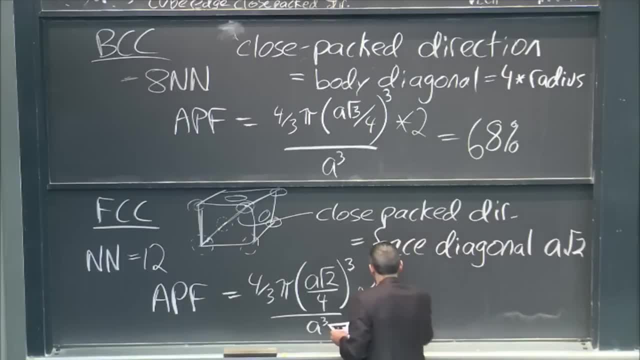 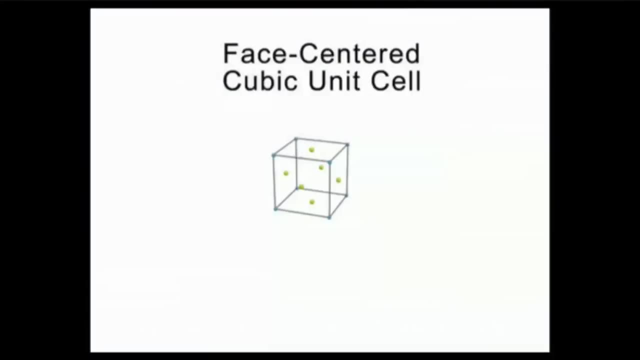 So that's three more, So there's four, And this gives you a very nice packing of 74%- 74%. Let's see what our video guy says about FCC. The face-centered cubic unit cell has a particle at each corner and in each face. 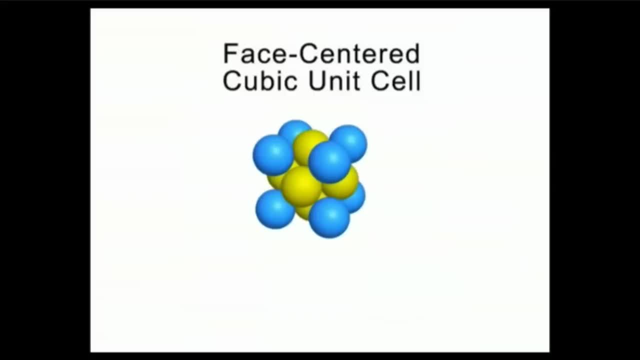 which are colored yellow here, but none in the center. The corner particles don't touch each other, But each corner does touch a particle in the face And those in the faces touch each other as well. The actual unit cell consists of the particles which, by the way, 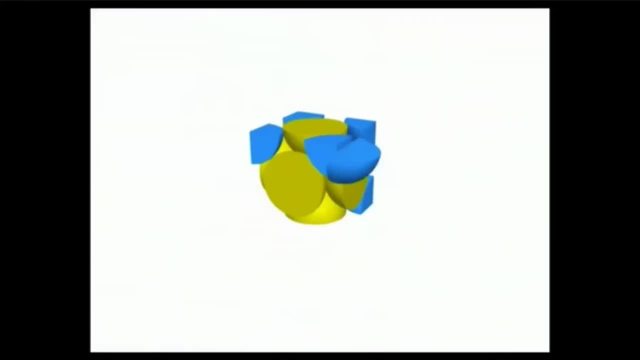 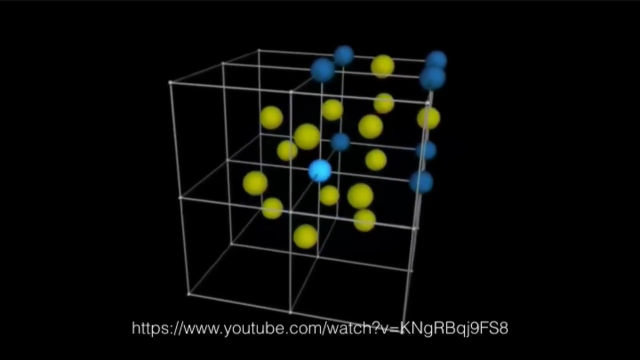 of portions of particles at the corners and in the faces. Eight-eighths at the corners gives one particle and half a particle in each of six faces gives three more, for a total of four particles In this tiny portion of a face-centered cubic array. 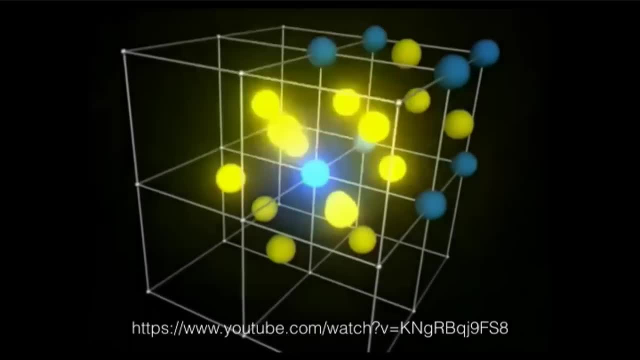 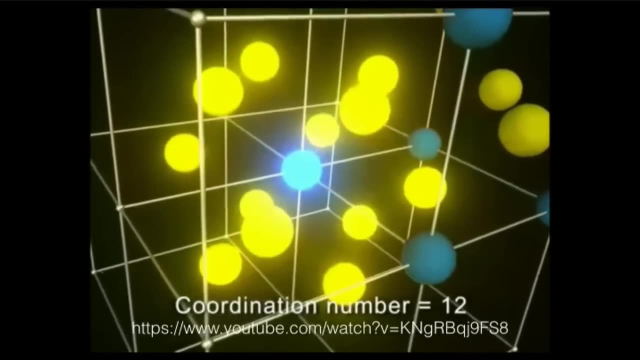 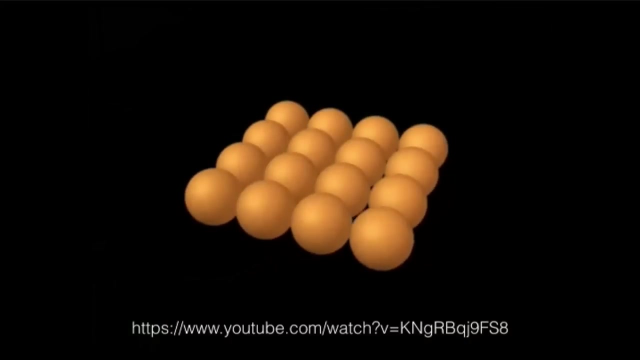 notice that a given particle has four nearest neighbors around it, four more above and four more below, for a total of 12 nearest neighbors. Stacking spheres shows how the three cubic unit cells arise. Now we're talking about packing. Arrange a layer of spheres in horizontal and vertical rows. 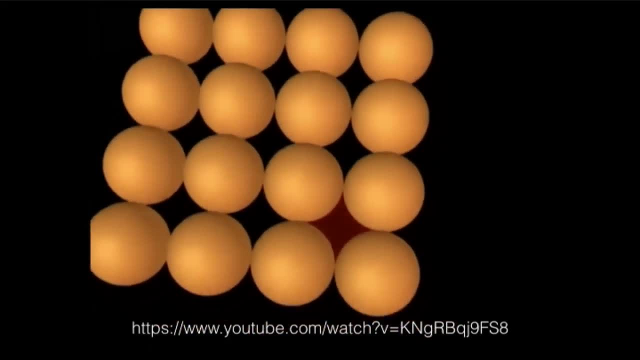 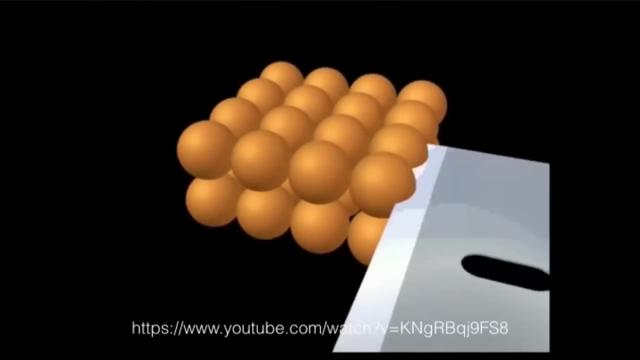 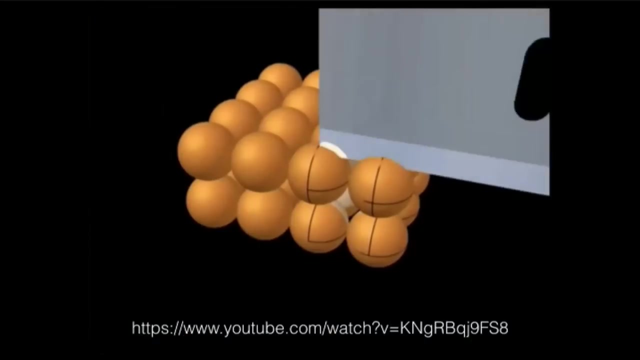 Note the large diamond-shaped space among the particles. Placing the next layer directly over the first gives a structure based on the simple cubic unit cell. Those larger spaces mean an inefficient use of space. In fact, only 52% of the available space. 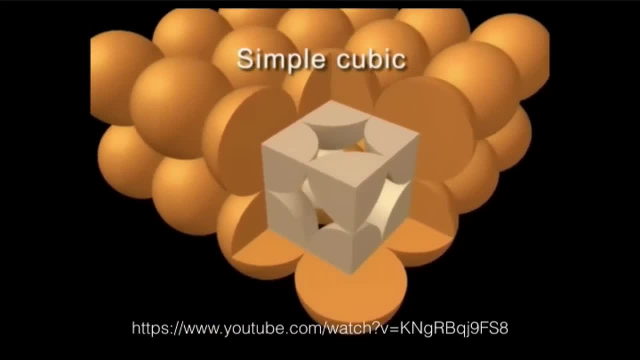 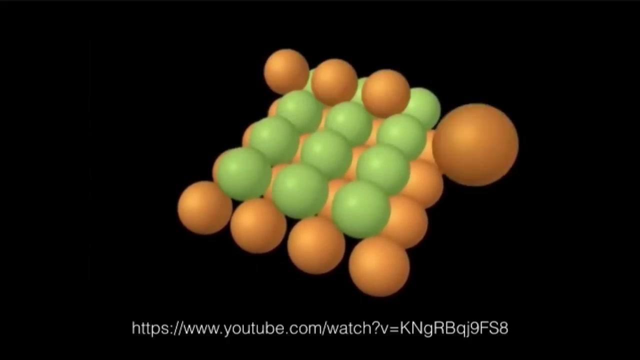 is actually occupied by spheres. Because of this inefficiency, the simple cubic unit cell is seen rarely in nature. Polonium A. more efficient stacking occurs if we place the second layer over the spaces formed by the first layer and the third layer over the spaces formed by the second. 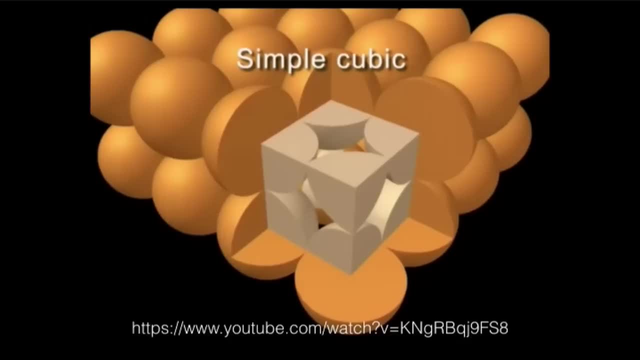 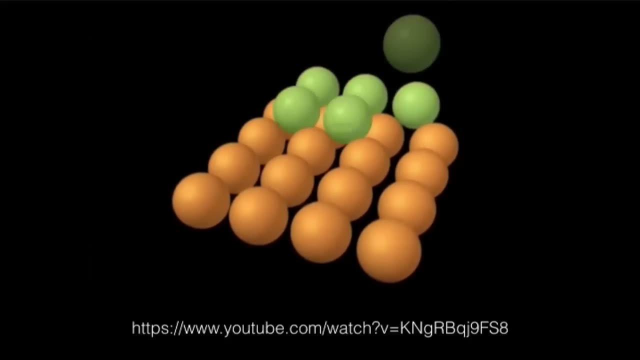 Because of this inefficiency, the simple cubic unit cell is seen rarely in nature. Polonium A. more efficient stacking occurs if we place the second layer over the spaces formed by the first layer and the third layer over the spaces formed by the second. 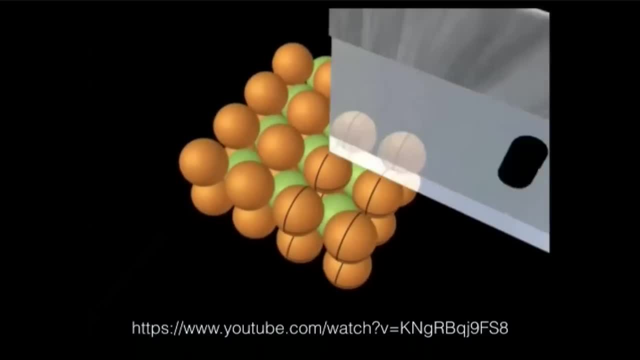 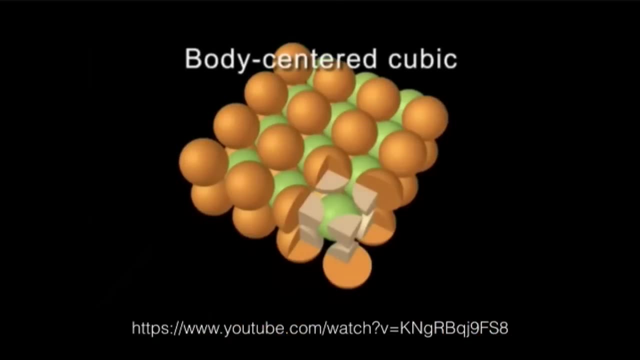 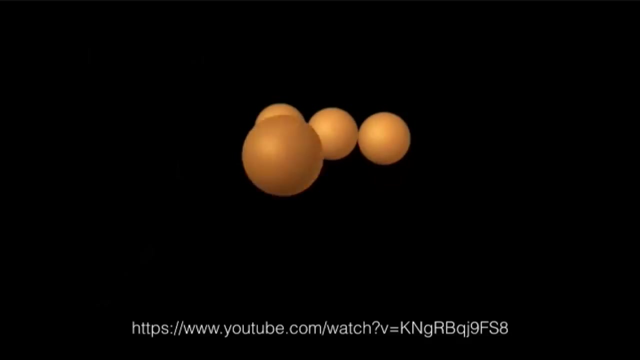 That simple change leads to 68% of the available volume occupied by the spheres and a structure based on the body-centered cubic unit cell. Many metals, including all the alkali metals, adopt this arrangement For the most efficient stacking. shift every other row. 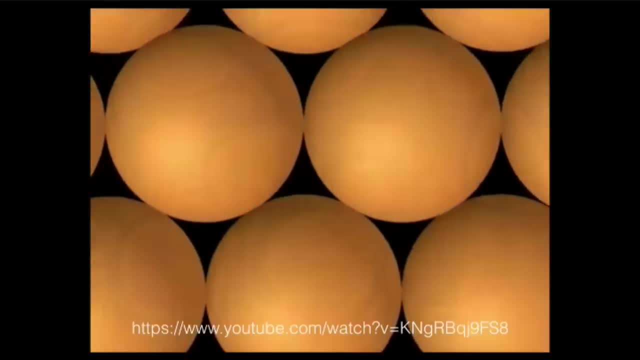 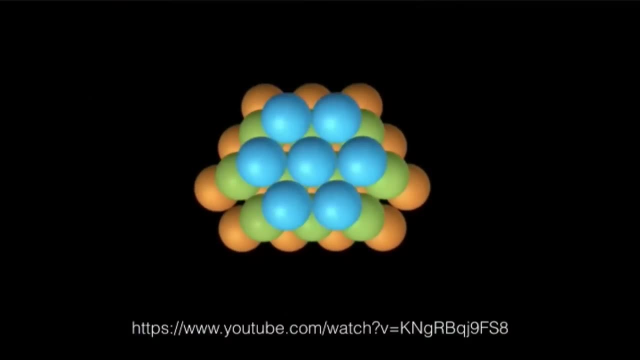 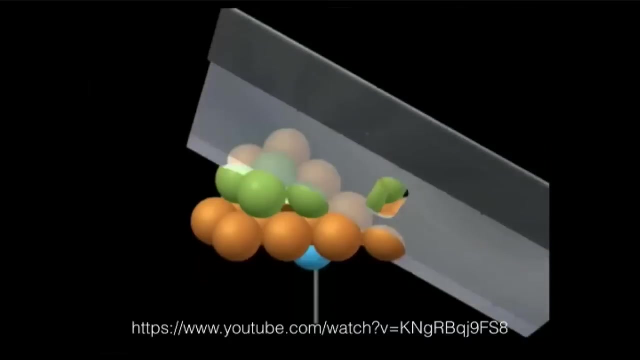 in the first layer. so the large diamond-shaped spaces become smaller triangular spaces and place the second layer over them. Then the third layer goes over the holes visible through the first and second layers. In this arrangement called cubic, closest packing spheres are occupied by 74% of the volume. 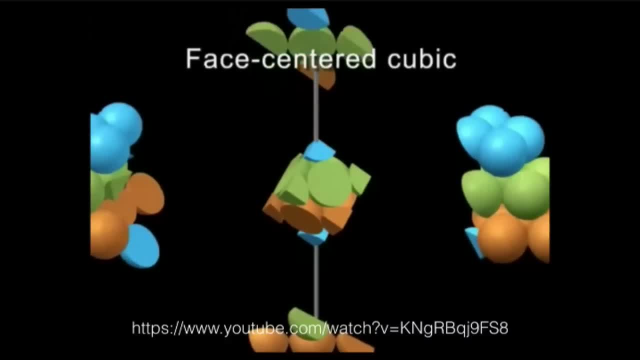 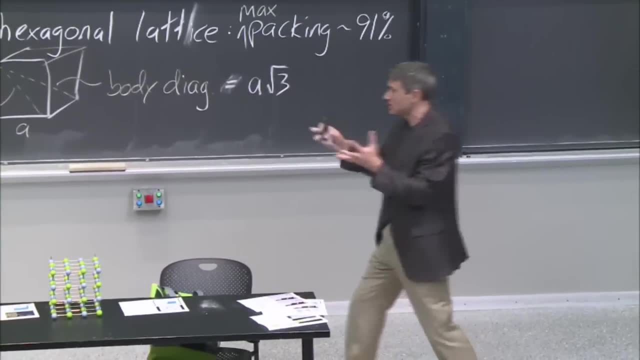 Note that it is based on the FCC crystal Bravais lattice. That's what he meant to say there. And you really see it come to life right? I wish I could do this somehow with the 3D models, But you stare at the 3D models and you see that. 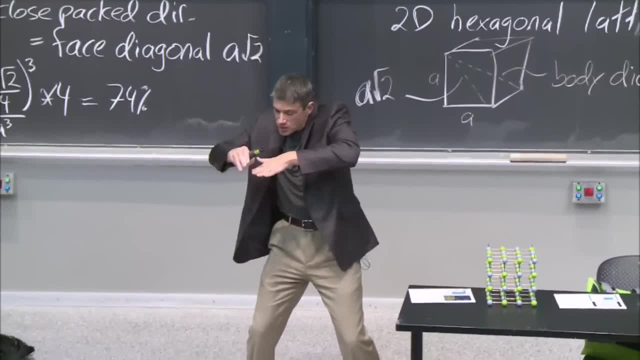 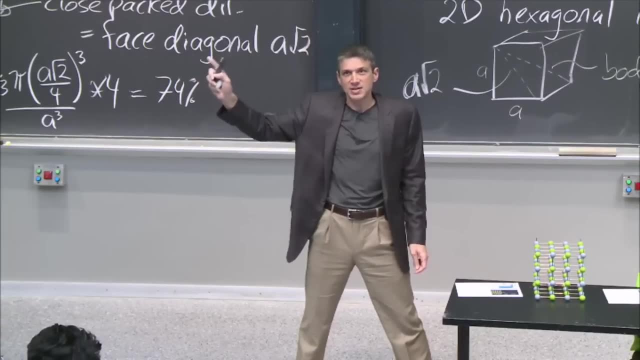 You know, what's interesting is the way you put it. This is what Hooke did with the cannonballs: You slide that base layer and then you can stack them differently, But it's still a cubic system. FCC- all right. 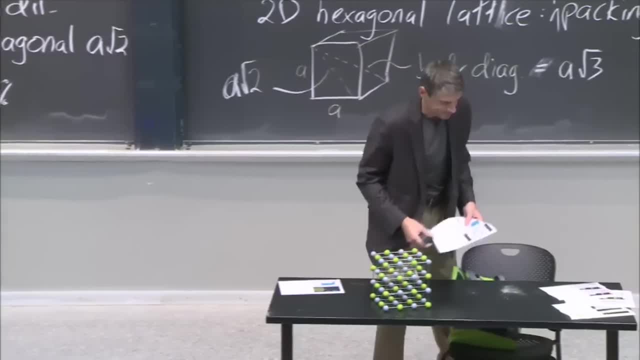 All right, We'll pick up on this on Wednesday. 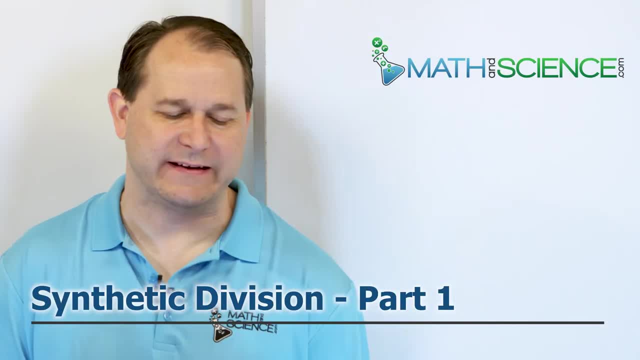 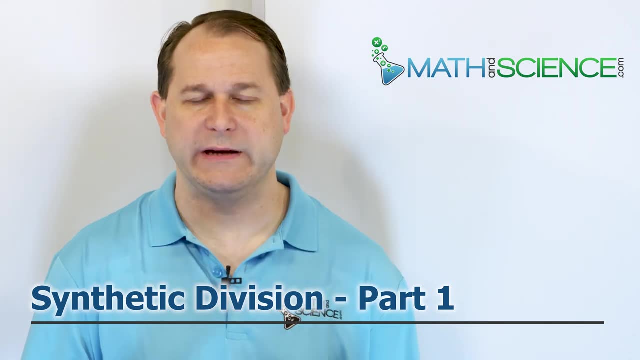 Hello, welcome back to Algebra. The title of this lesson is called Synthetic Division, Part 1.. We're going to have several lessons here, increasing the problem complexity, but the most important point here in the beginning is to really understand what synthetic division is. 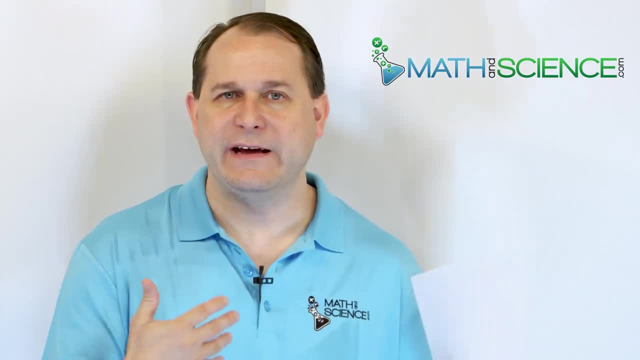 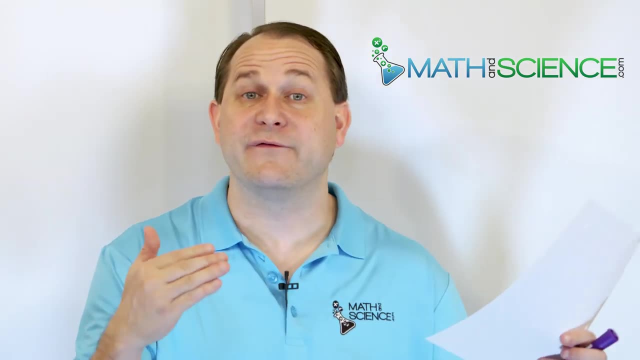 why we use it and to understand where it comes from. I could just give you the procedure and you could do it, but I want you to know where it's actually coming from. So in the last few lessons, we learned how to divide polynomials And if you're anything like me or like most,